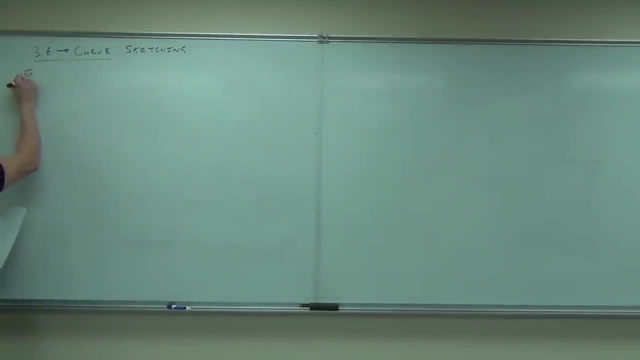 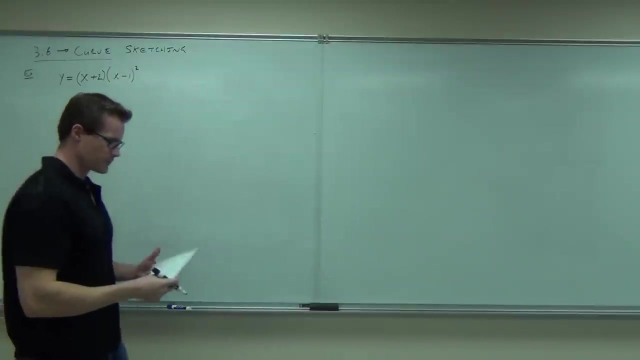 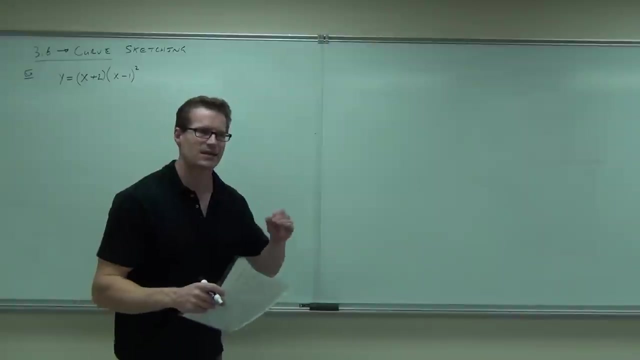 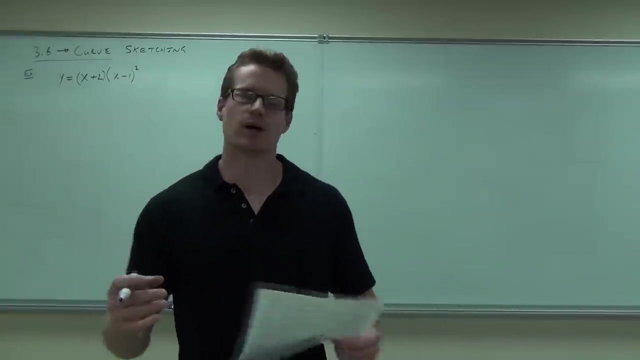 So here's your example. Here's your example, And I'll tell you how to do this problem verbatim, just exactly like you should. all right, with every single step. Step number one, when you're graphing any curve, is: well, you want to find out as many intercepts as you can. 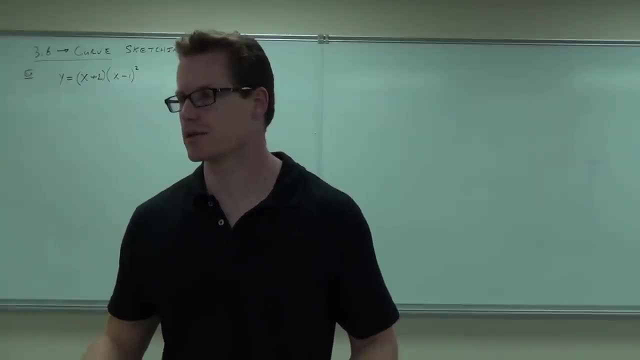 X intercepts and Y intercepts. That's always a good thing to do, right? Because in most cases that gives you at least an approximation of what you're talking about where you're crossing the Y axis, where you're crossing the X axis. 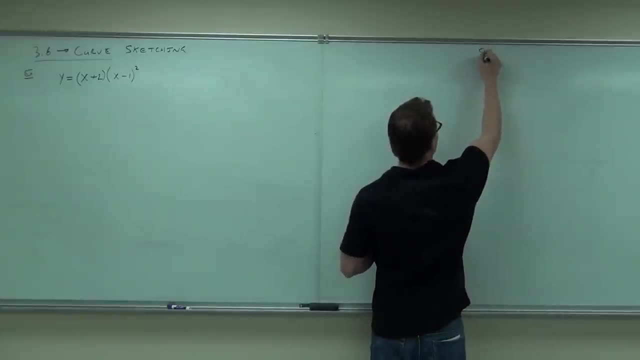 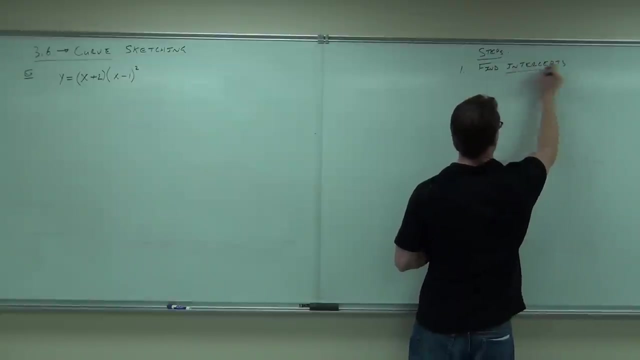 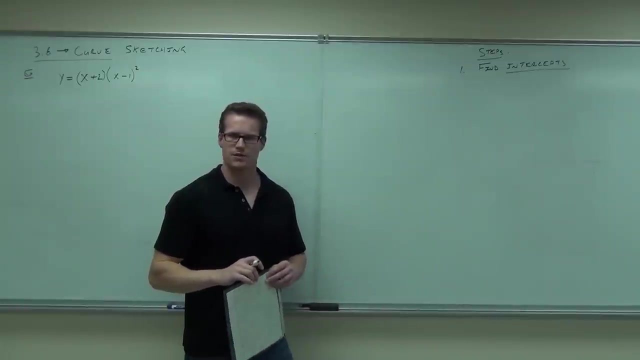 So step number one every time you're gonna find the intercepts. By the way, how do you find X- x intercepts? how do you find x intercepts? Y equals zero. Say it: Y equals zero, Y equals zero. 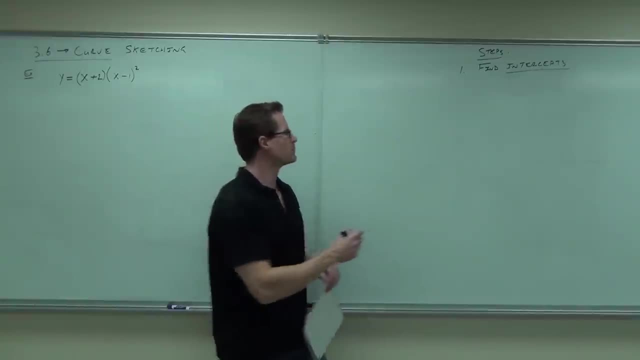 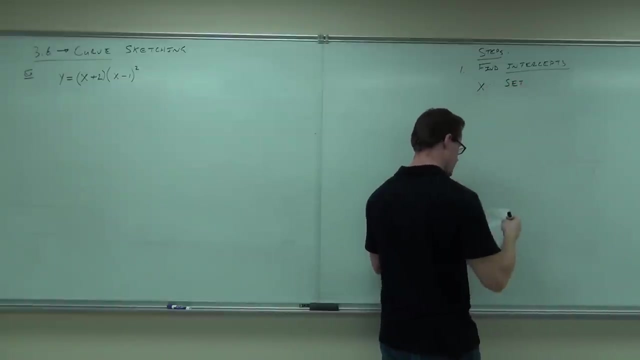 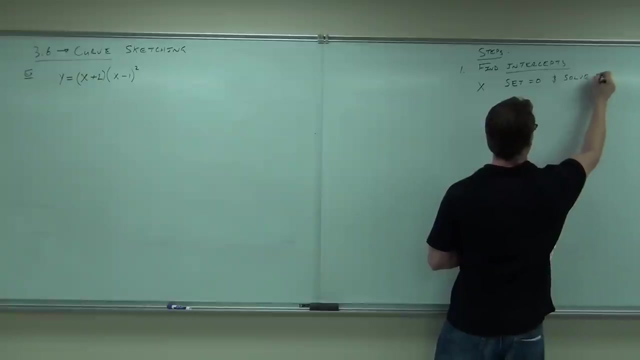 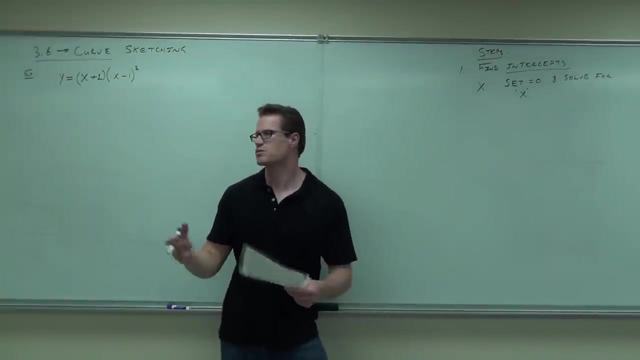 So set the equation equal to zero. that's how you find x intercepts. You set equal to zero, you solve for x. That's gonna give you any roots. That's what a root was right When you set the function equal to zero. 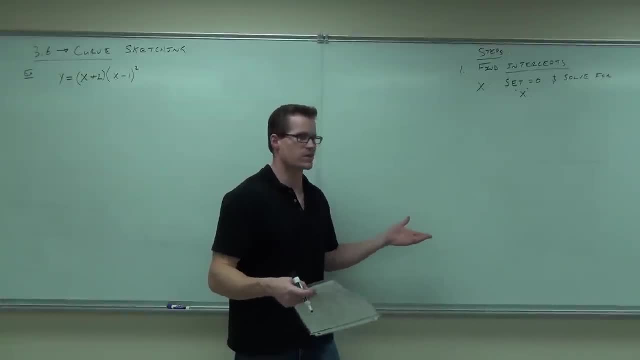 and you solve for x, you find out where it's crossing the x axis. That's a whole exact idea. Should make sense, right? Because if you set y equal to zero, that means you're gonna find out everywhere you cross that x axis. 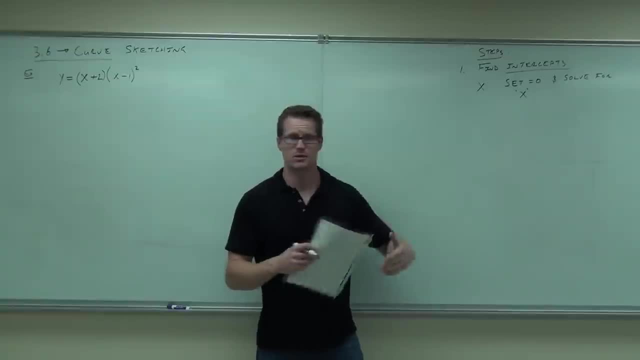 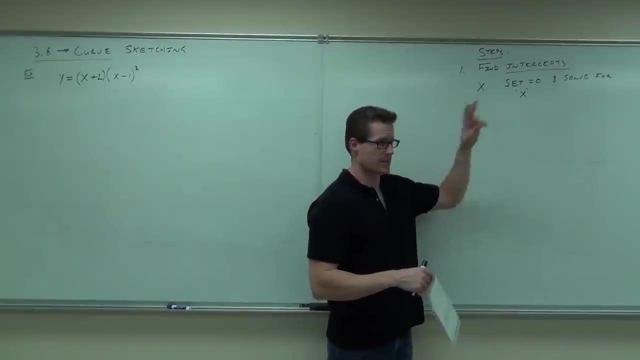 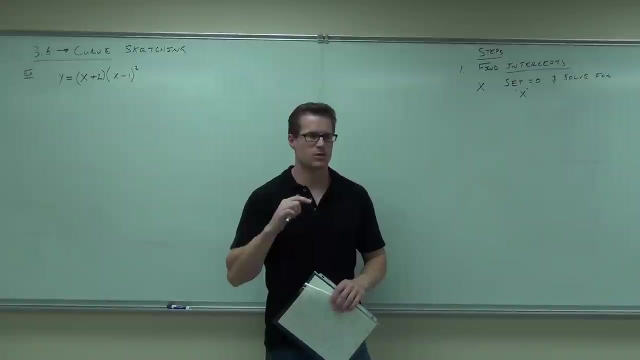 Can you believe me? Now, the y intercept is quite a bit easier, By the way. you only do this step if it's easy. Easy, easy means it's quadratic or lower, or it's already factored for you. Okay, so, cubics, don't spend your time factoring them. 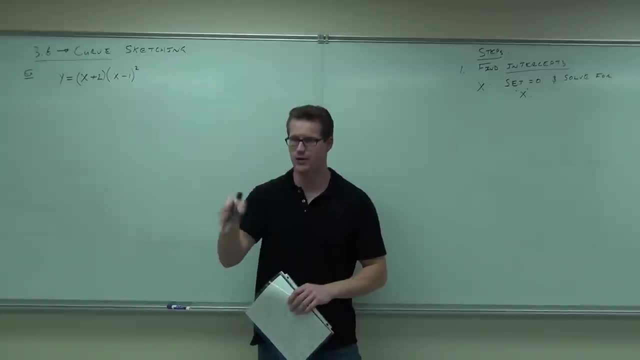 If I give that to you on a test, I'll just give you the x intercepts. I'll say: here are your three x intercepts. You follow me on that. So if it's easy, do that. Easy means so I know this is recorded. 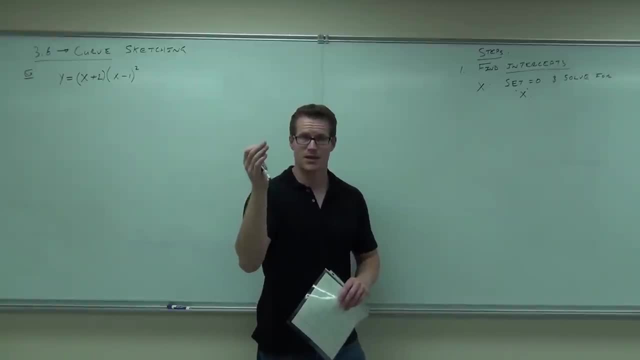 so you don't cheat me. Easy means quadratic, linear, or if it's already factored for you, that's easy. Everything else- cubic or higher- is hard. Unless you can just see a root right off the bat, that would be considered easy. 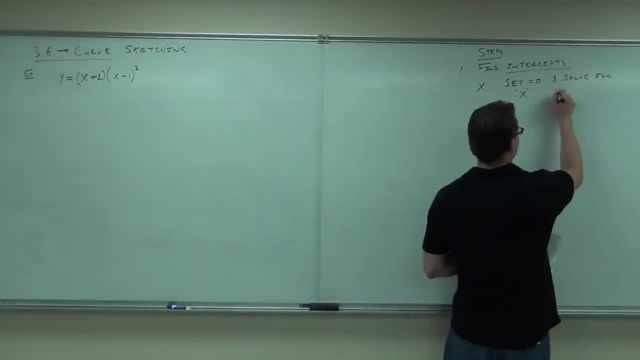 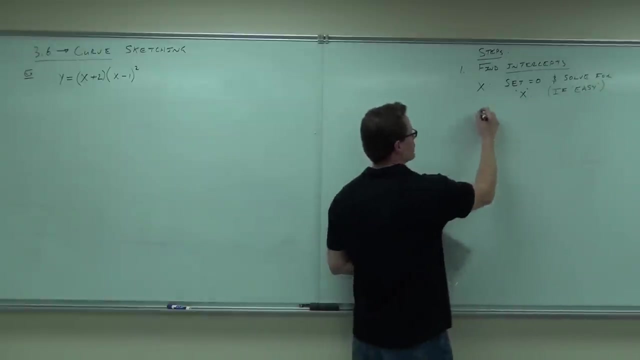 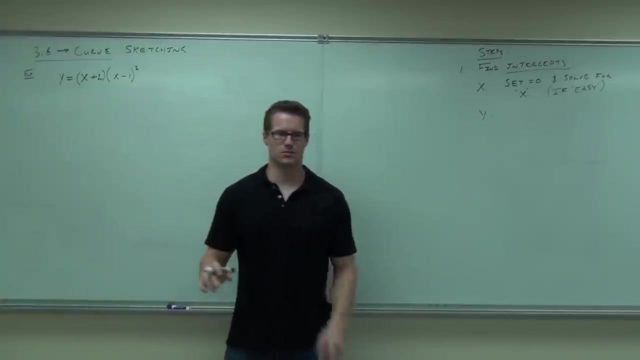 Believe me, Okay, okay, If it's easy For y intercepts, how do you find y intercept Easy? really easy to do: X equal to zero, Set x to plug in zero. You plug in zero for x and it'll give you y intercept. 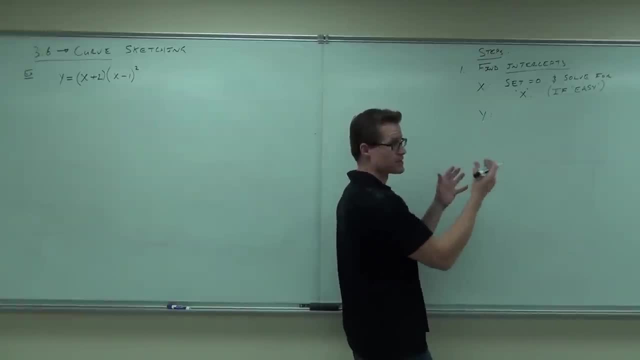 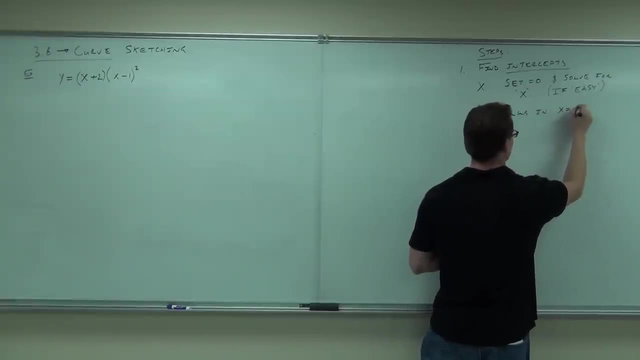 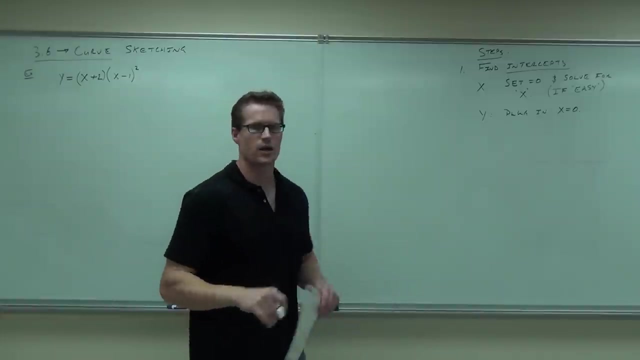 That's the easy one, That's nice. You all need to find that for every single one of these, if they exist, Let's try it, Let's try it. So this will be step number one. I'll try to write out every step for you. 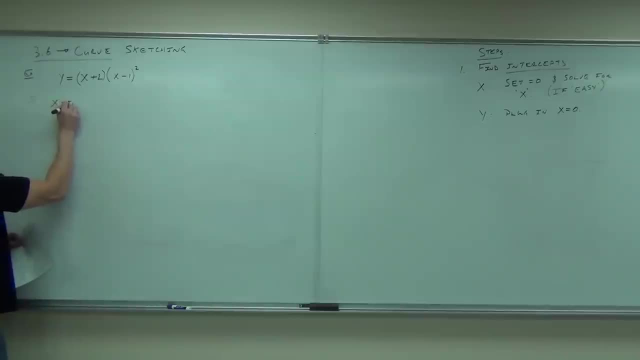 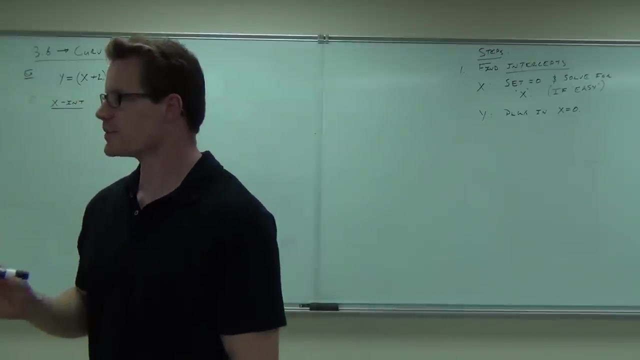 Step number one: Solving for x intercept. How do you solve for the x intercept? Well, this is just basic algebra. You're gonna take your function, you're gonna set it equal to zero and you're gonna solve for x. 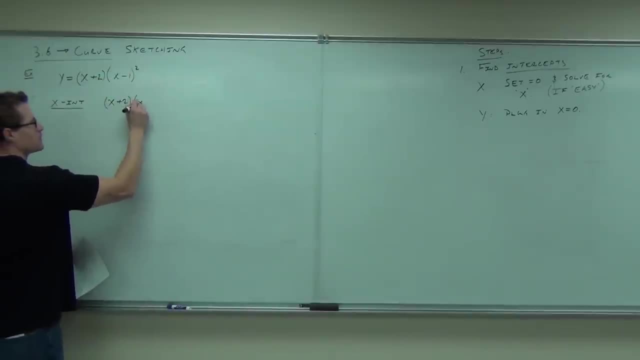 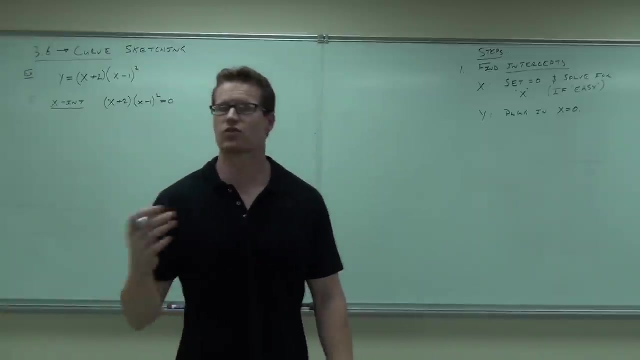 So we will have x plus two, x minus one, squared equal to zero. Can you find your x intercepts from right there? That's great. That's great. That's great because it's already factored for you. Can you tell me what's one of your x intercepts? 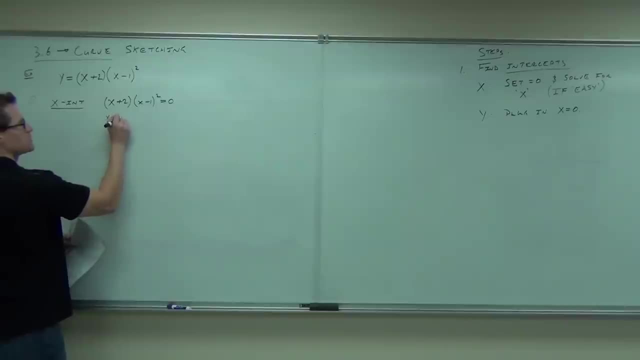 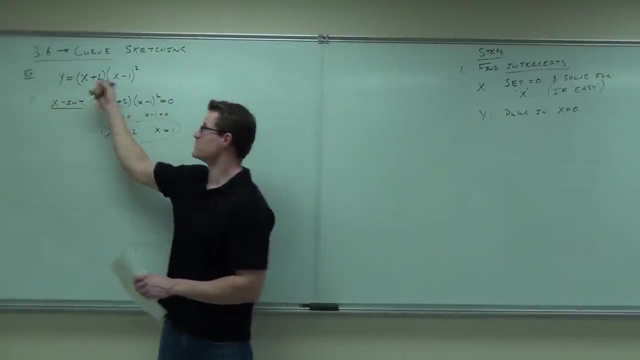 You have: x plus two equals zero, x minus one equals zero, because it's zero product property. So x equals negative two, very good, and x equals one. You have two x intercepts, Richard. I feel okay with that If this hadn't been factored for you. 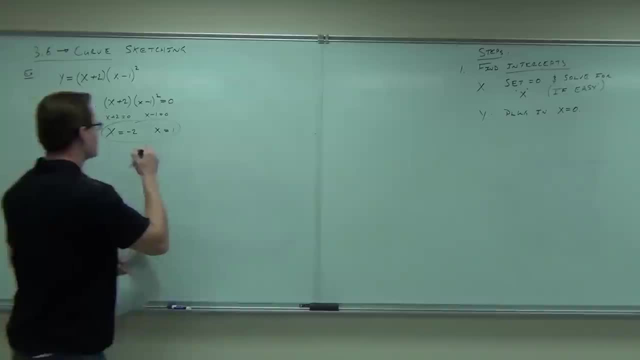 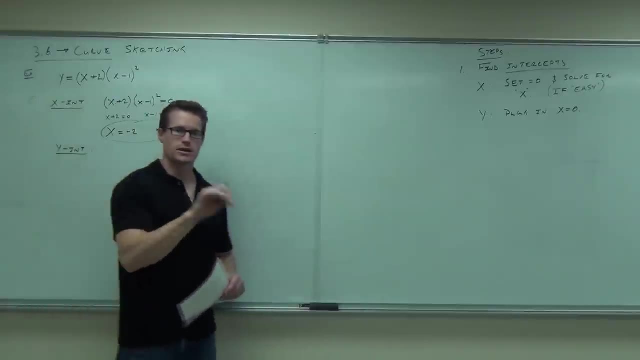 you'd just skip it. I'd give them to you, okay? Part two of step number one. Step number one is find your y-intercept. Y-intercept says you need to plug in zero for x and see what you have. 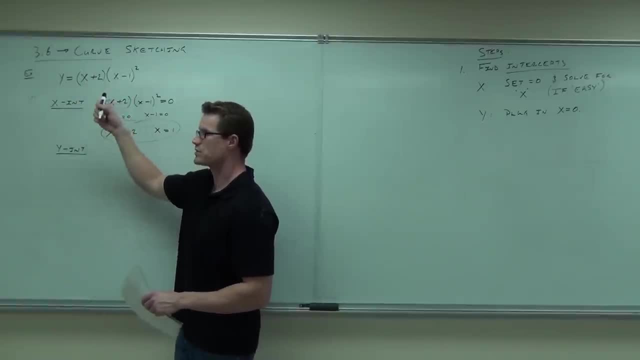 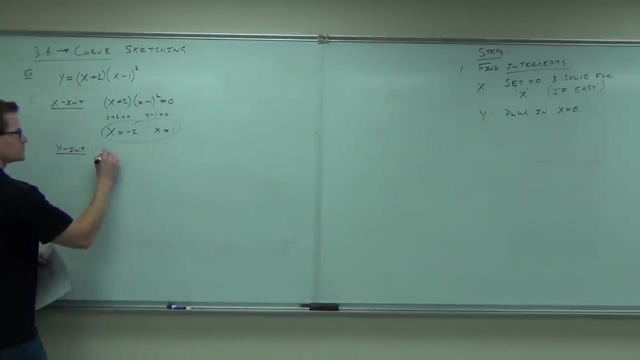 So I'm gonna take zero plus two times zero minus one squared- Don't forget squared before you multiply. What is zero minus one Negative one? Negative one squared One Times Two Is Two. You get two. The y-intercept is two. 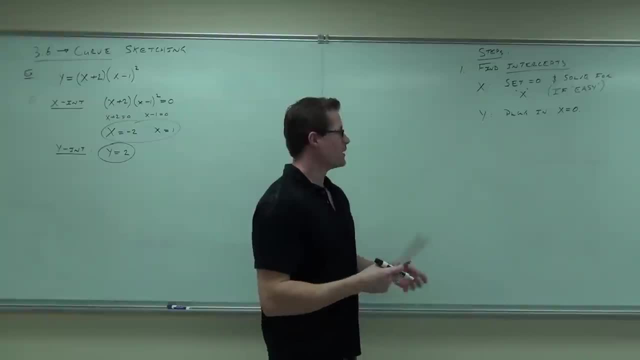 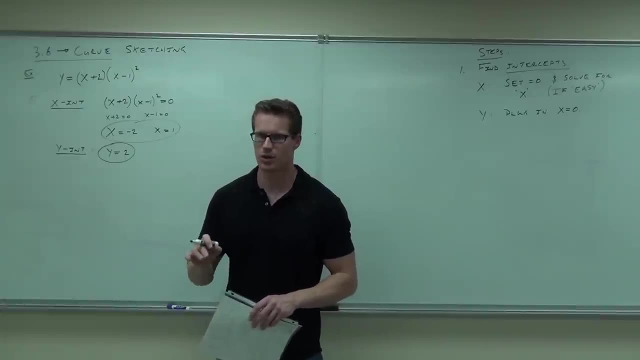 Do you feel okay for this? so far? All right. step number two. Step number two applies only to rational functions. It does not apply to polynomials. because polynomials do not have this, I'm gonna put step number two and a little asterisk. 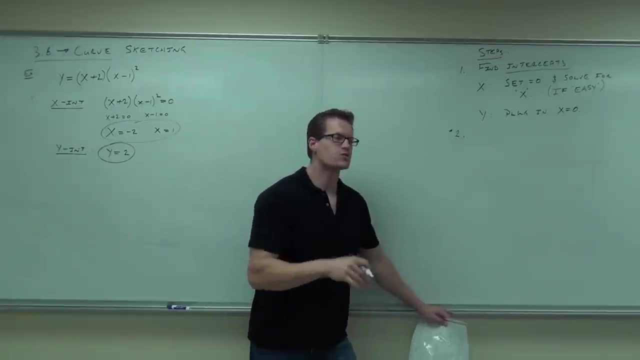 The asterisk means for rational functions, only For rational functions. a lot of times with rational functions you're gonna get some asymptotes, right, You're gonna get some holes. So for rational polynomials, don't have those. It's continuous everywhere. 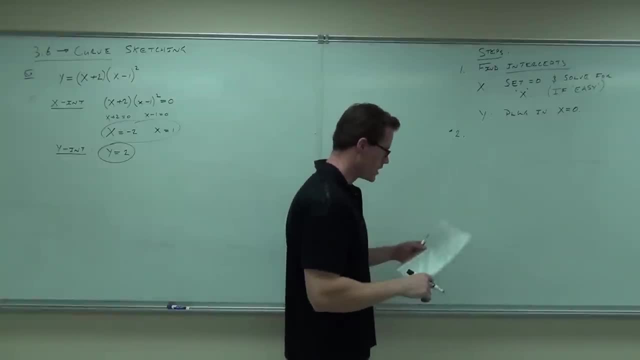 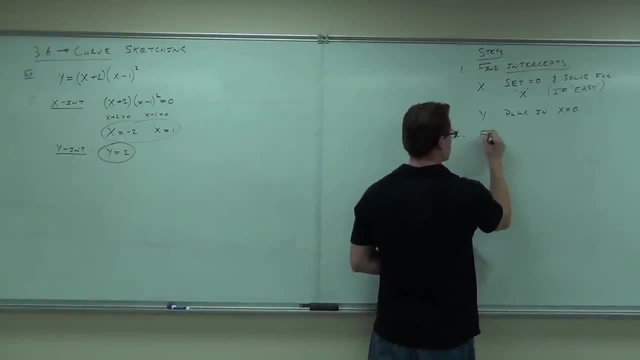 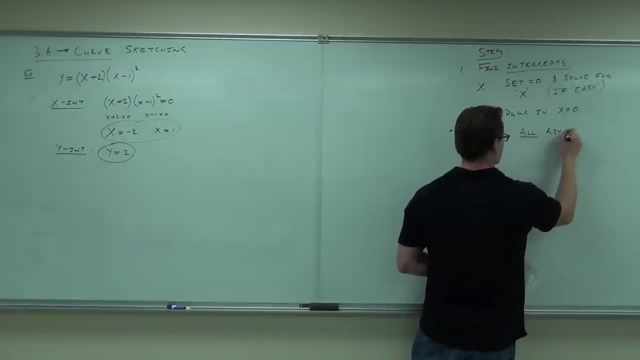 You don't have asymptotes, you don't have holes. So this is why it's only for rational functions. You're gonna find all the asymptotes, vertical and horizontal, and any holes. Okay, Do you remember when vertical asymptotes exist? 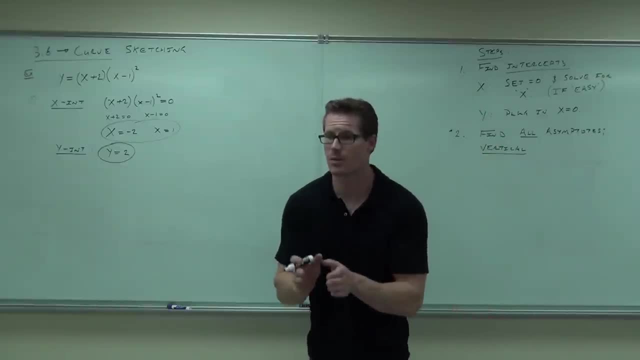 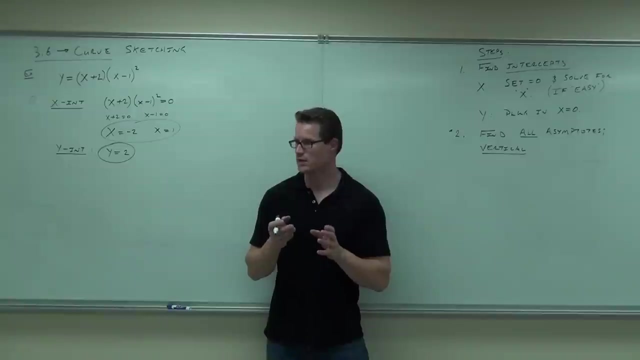 Denominator equals what? And you can't. when do holes exist? When you can't cross it out? Okay, so denominator equals zero gives you asymptotes or holes. If you can cross it out, it's a hole, If you can't cross it out, it's asymptotic. 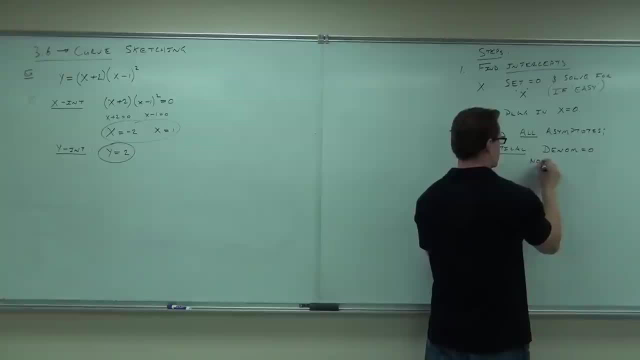 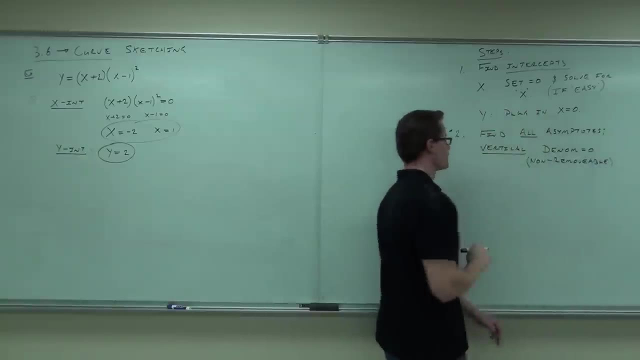 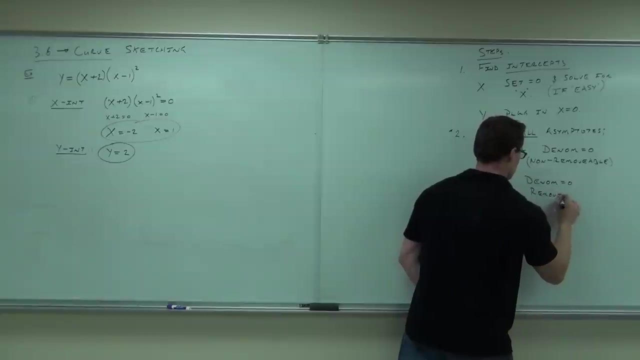 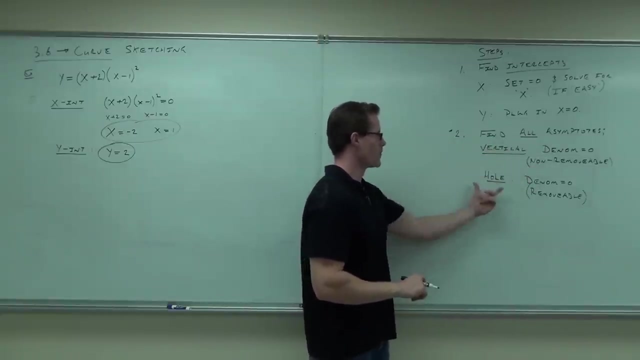 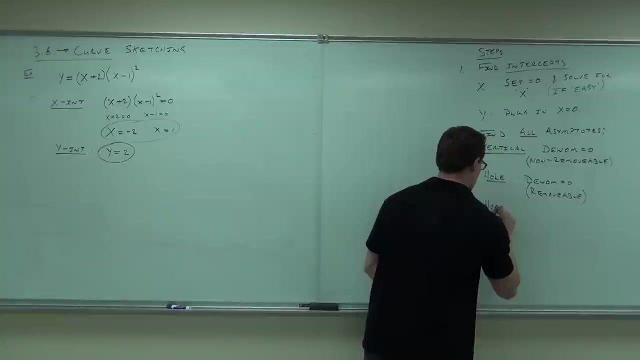 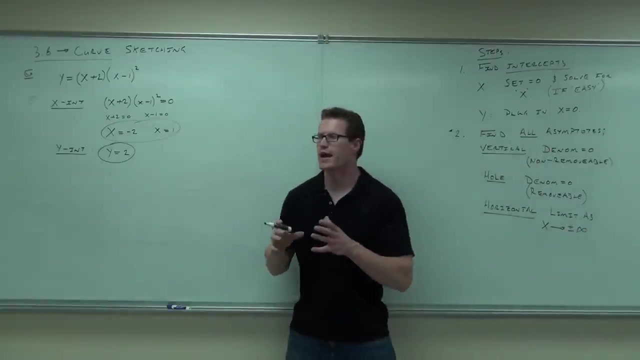 Vertical ascent tilt. Whole denominator equals zero, not removable. Whole denominator equals zero, removable. How do you find horizontal asymptotes? Good thing we covered that stuff. Horizontal asymptotes occur. That's what the whole last section was about. It said: can you find the asymptotes as we go to the right and as we go to the left? 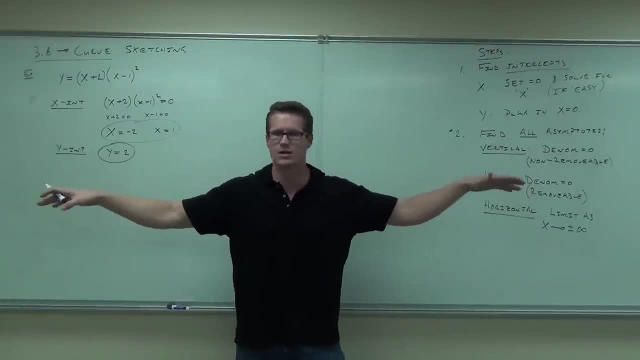 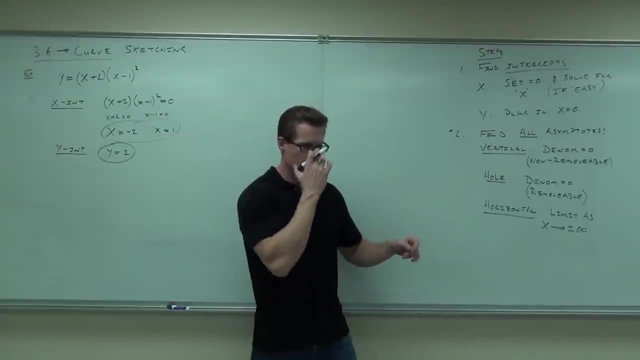 That's what we were finding. We were finding horizontal asymptotes at zeros or at ones. That's what that did, And so what we're going to do here for horizontal asymptotes is: you take the limit as we go: x approaches infinity or x approaches negative infinity. 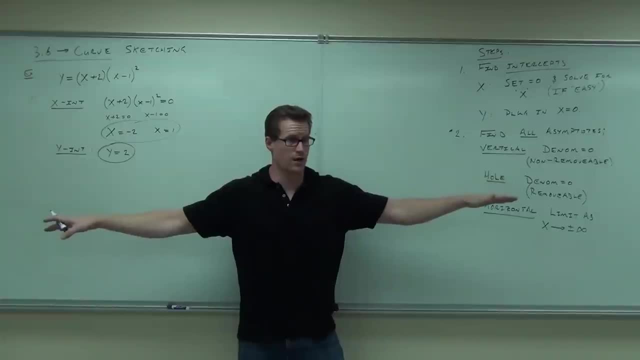 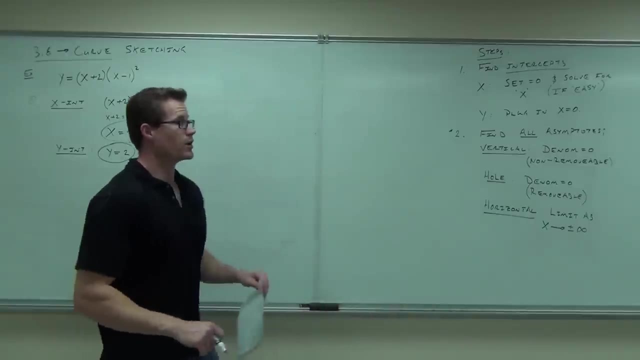 You have to do both of them because you know the limit could change. Remember that one third right It could change, So you've got to be careful on that. Take the limit, So do we need to do step number two for that problem? 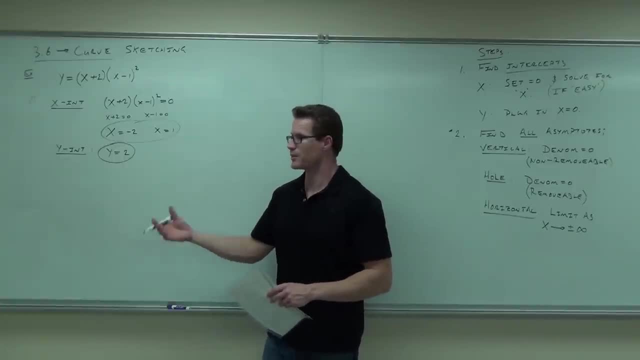 Is it rational? So if it doesn't have a denominator, we're not going to be able to do that. If it had a fraction and you had a denominator with a variable down there, then of course we would be doing that. But right here we don't. 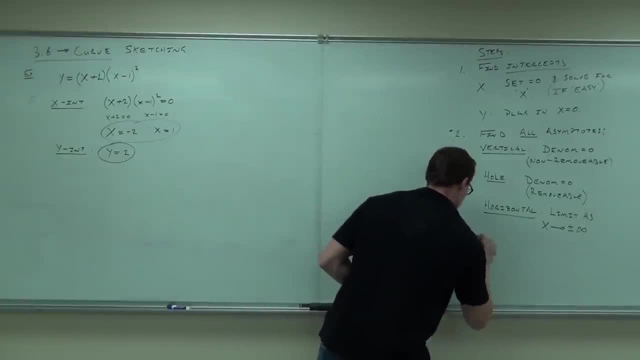 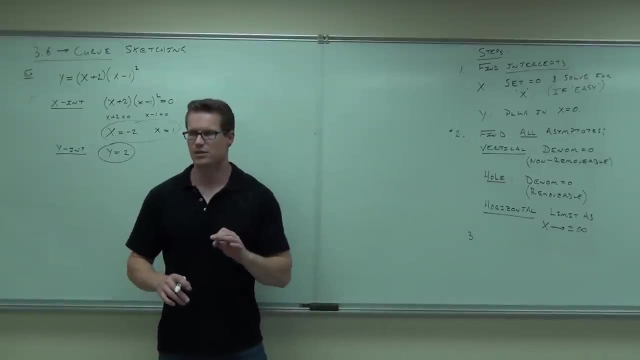 So now we're going to go on to step number three. Step number three is you finally get to do some calculus. You're going to do the first derivative test. You remember the first derivative test? You had a whole homework section on that right. 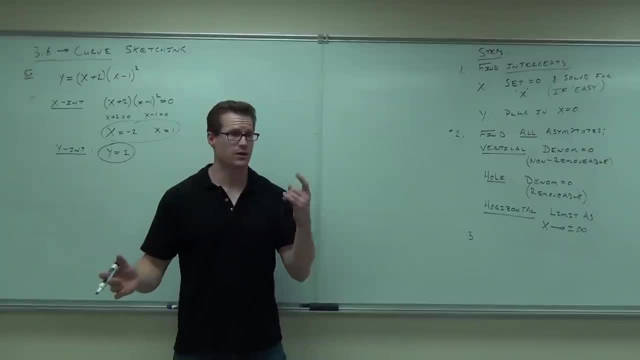 First derivative test. you said: equal to zero. It will give you two things: Critical numbers and increasing and decreasing. And that's what you care about, right, You care about where are my maxes, my mins, how am I going up, how am I going down? 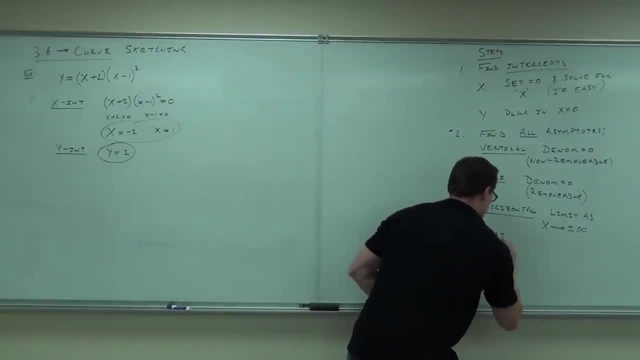 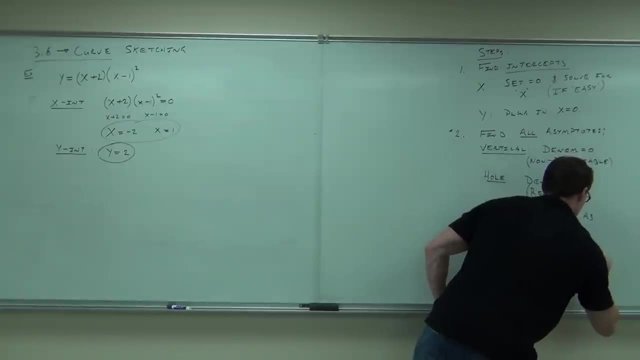 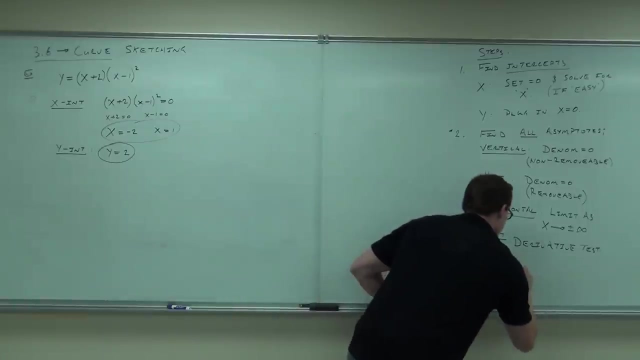 That's what you care about. First derivative test Why? Because it's going to give you critical numbers and increasing and decreasing, Okay, Okay. So you can keep doing it until you figure out where your podría be Okay Or areas where the graph will increase or decrease. 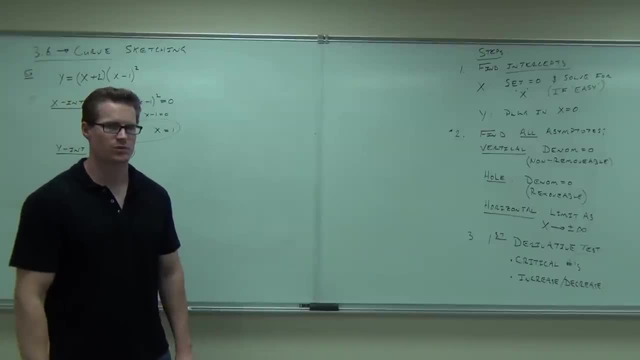 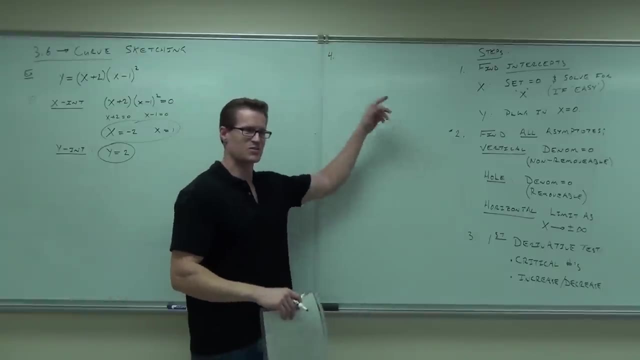 Let's try that now. You know what, Maybe I'll give you all the steps and then we'll go through it. Step number four: Sorry, I'm kind of backwards. One, two, three, One, two, three, reading a book backwards or something. 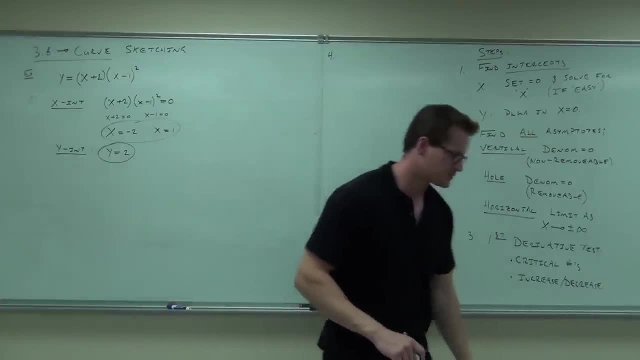 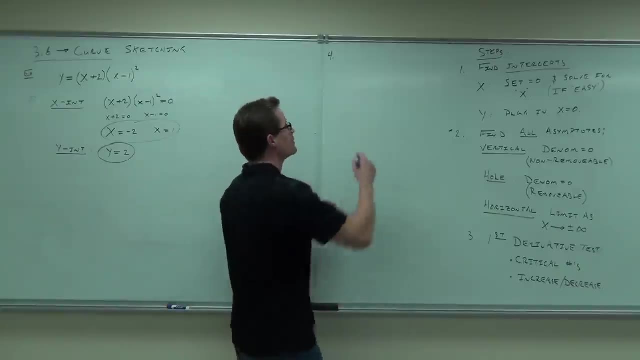 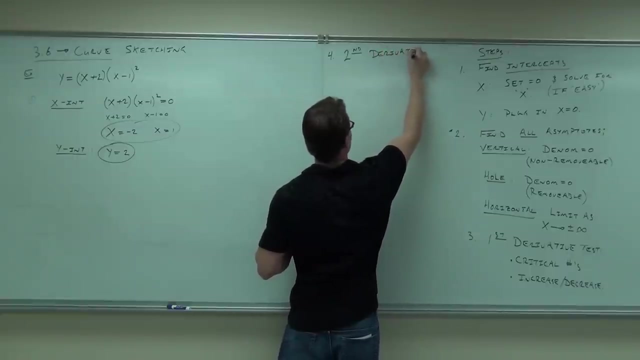 Step number four: After you do the first derivative test, what do you think you're gonna do next? Geniuses, The second derivative test. What does the second derivative test give you? Concavity, Yep, the reason why you do it. 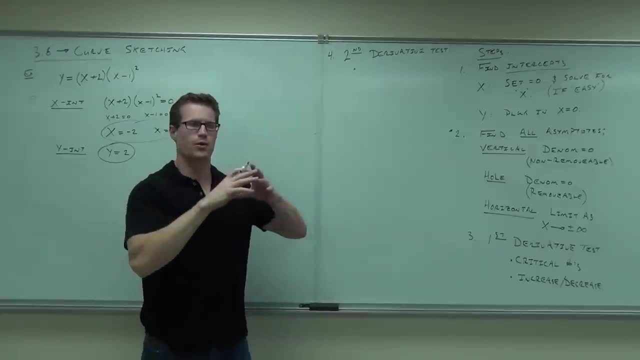 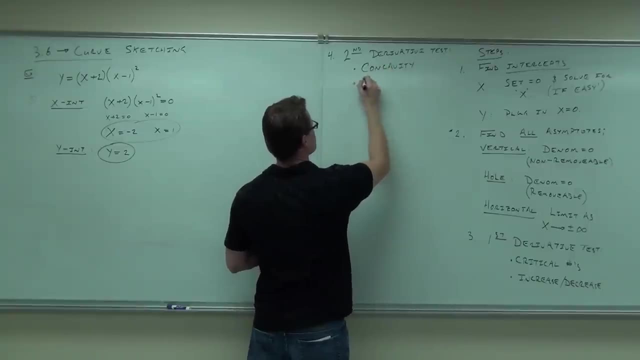 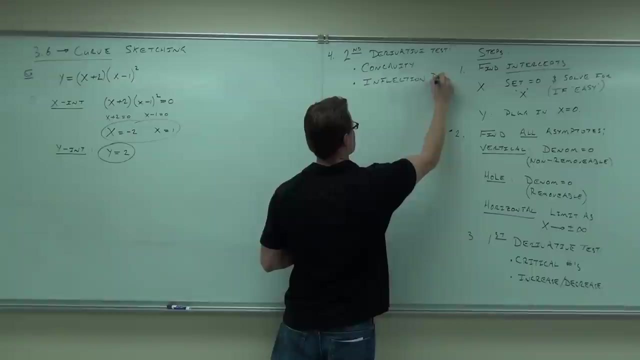 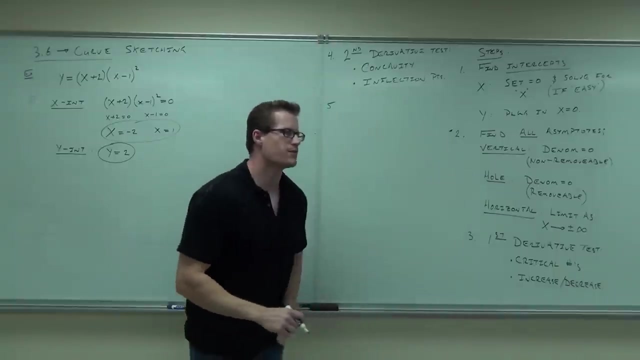 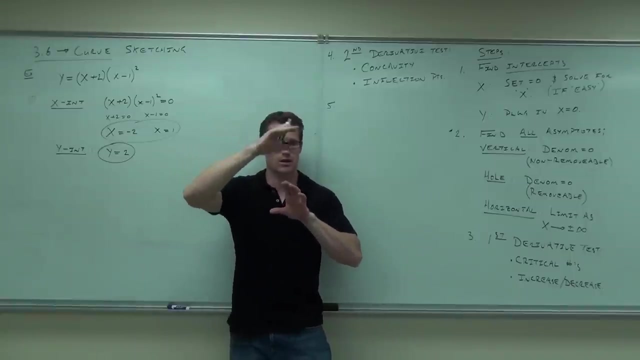 just like Scott said you're gonna do for concavity and for inflection points. Step number five: The table ahead you make that has the first derivative on the top, second derivative on the bottom. It tells you increasing, decreasing, increasing. 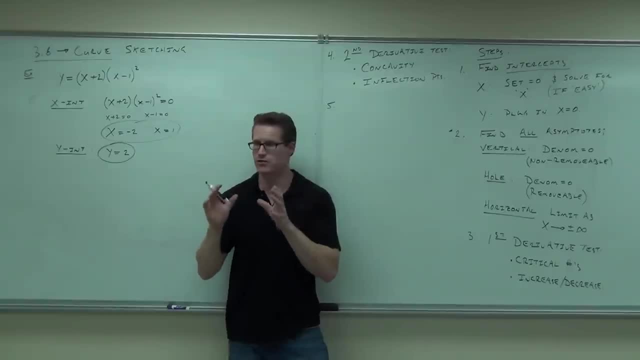 all that stuff and it tells you concavity. So basically it gives you a picture of your graph right there. That's what you're gonna make. So make the table. You know they're very long problems, Especially- oh my gosh, especially- with rational. 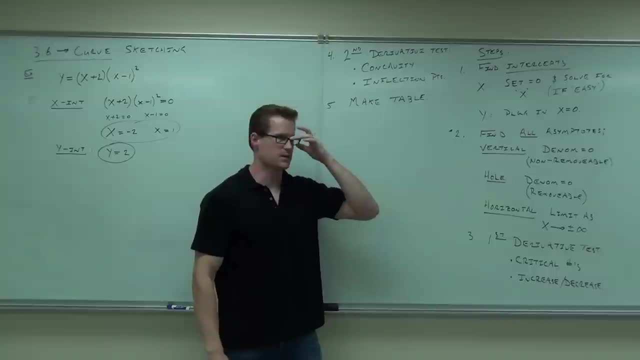 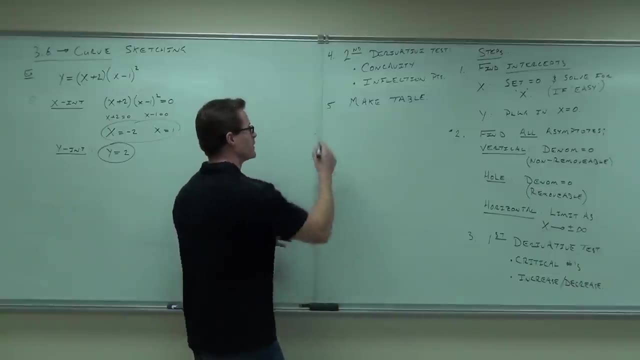 they take a long time, a very long time. They're not easy. Well, actually they're not hard. They're very time-consuming. So they're gonna take a long time. Not gonna lie, Number six, At this point you're gonna have everything you need. 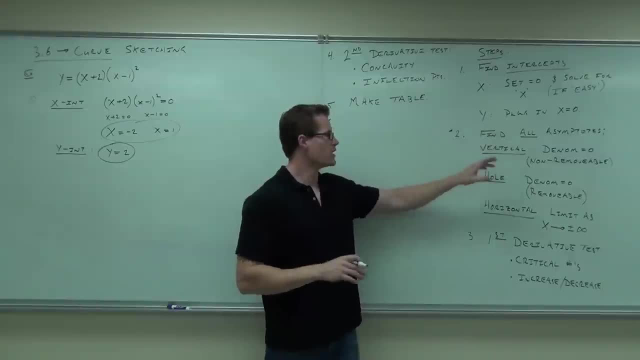 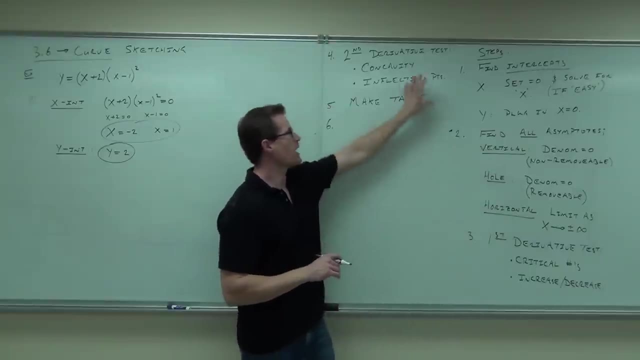 All right, You're gonna have your intercept: Intercepts- That's huge. You're gonna have any asymptotes: You'll put those on your graph. You're gonna have any holes? You put those on your graph. You'll have your critical numbers. 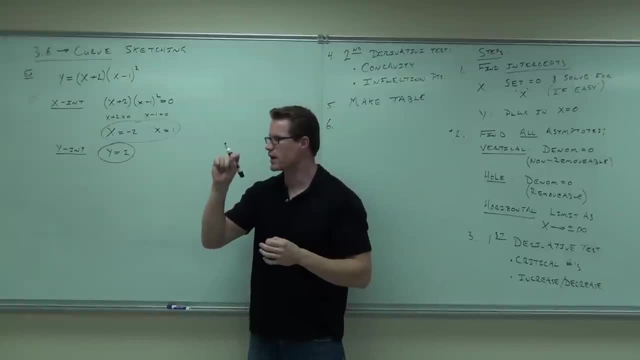 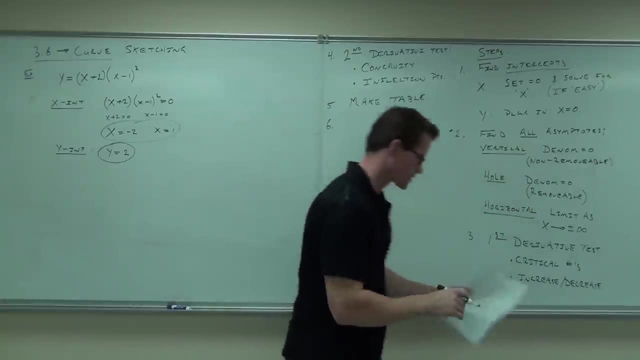 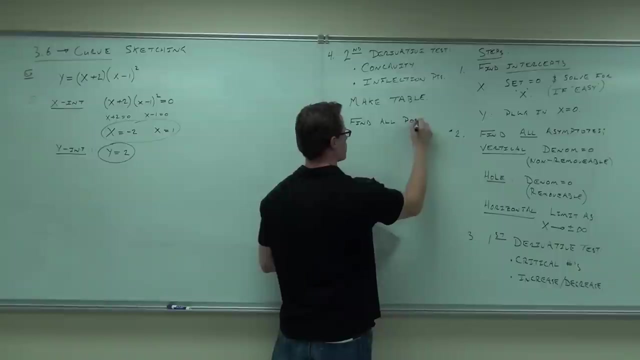 and your inflection points. What you won't have is the actual points. right, You'll have the critical numbers. Plug them in. Find all possible points relative to those means and inflection. Find your points from the original function. The last, if you get the points. 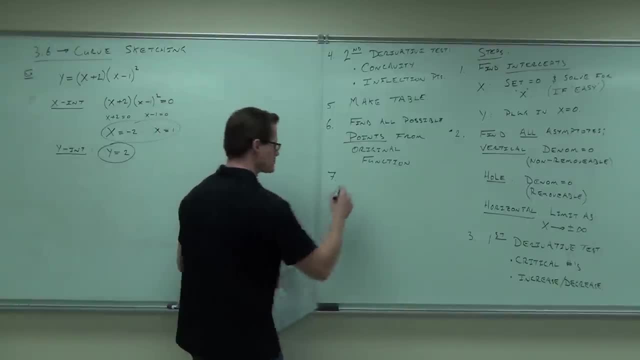 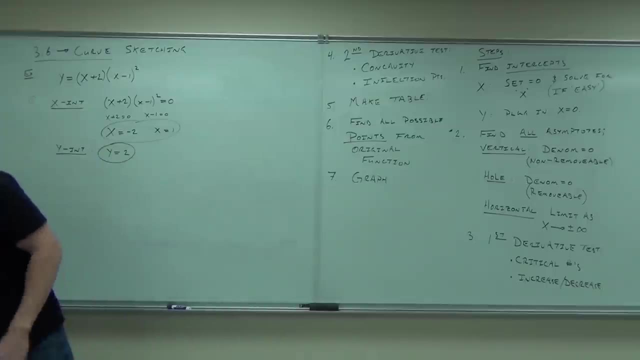 you got all the areas of increase and decrease in concavity. grab it. Okay, we're gonna get at least the first two tests done on this thing. We already have the intercepts, We got X and Y, We don't need to do step number two. 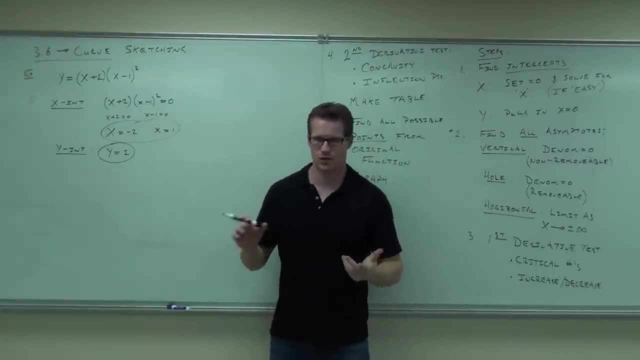 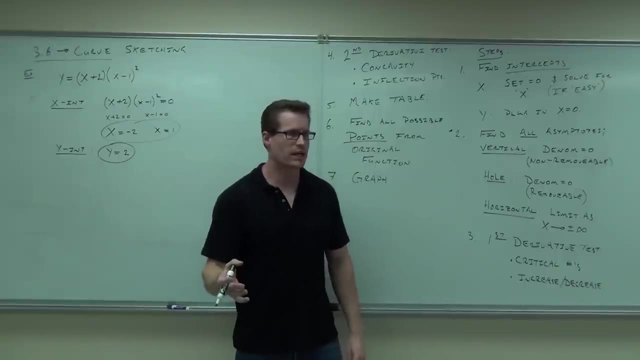 because they're not rational. We're gonna do the first derivative test. Now, don't fool yourself here. Yes, that looks pretty nasty That you say, oh my gosh, that's a product rule with a chain rule or a general power rule in it. 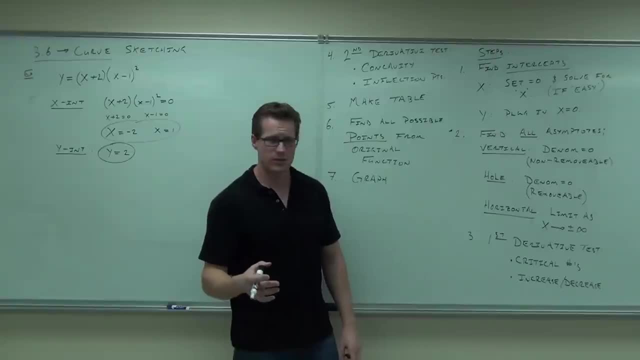 That could get pretty hairy and then I have to set it equal to zero, Or maybe be a little bit smarter about that. Probably easier to distribute that right. Maybe distribute some of those easier ones first. that way you don't have to do all those rules. 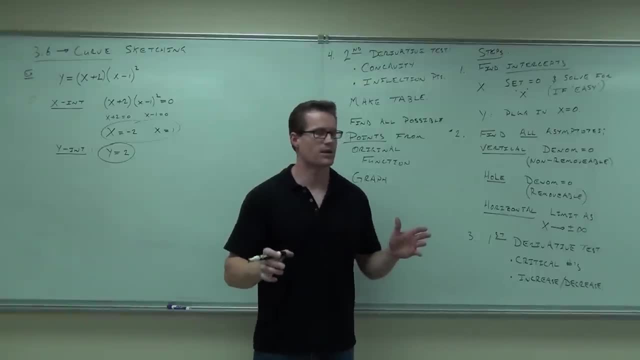 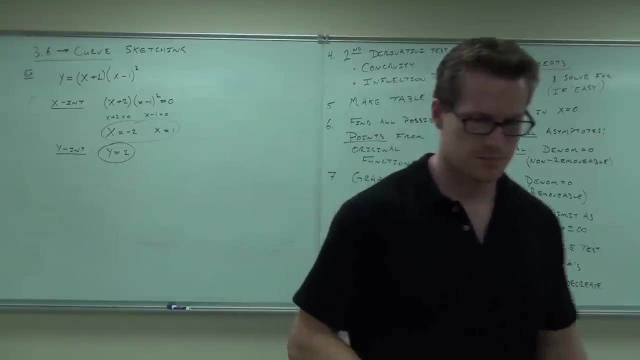 Now if it was two to the sixth power or something, firstly that'd be insane, But secondly you wouldn't want to do that, So just go ahead and maybe distribute that. So why don't you try that right now? 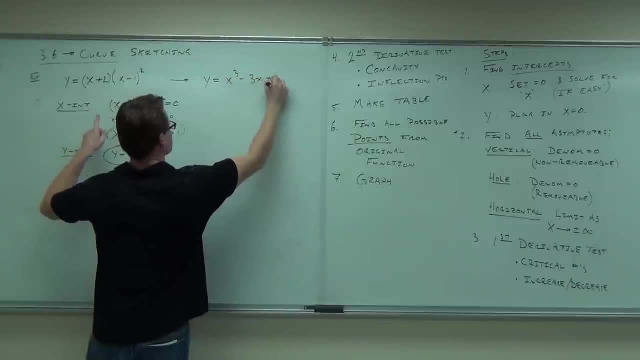 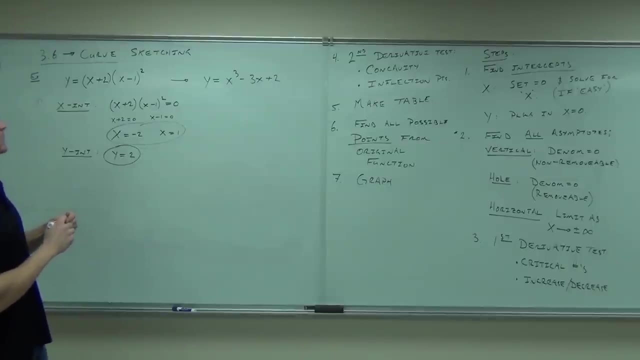 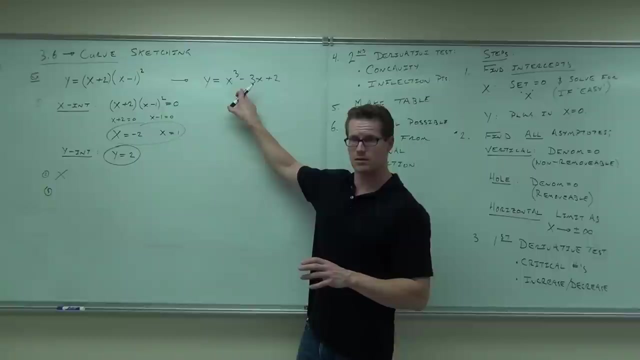 Hopefully you got that. Did you get that? Okay, keep working. Step number one: we got Step number two. we don't need it. Step number three: First thing: were you able to get that? Bless your heavy word? were able to get that? 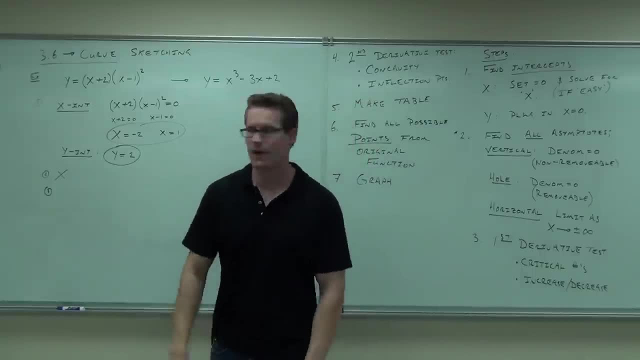 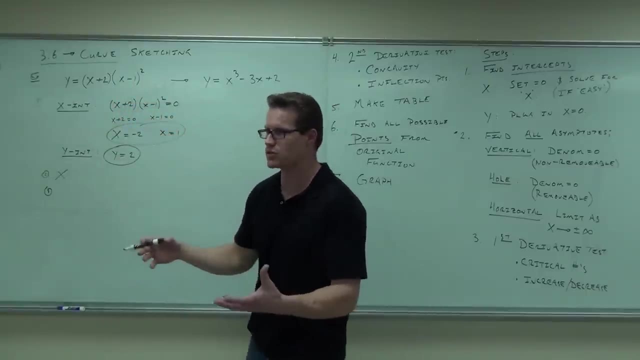 Yeah, Take the first derivative. do the first derivative test. go for it. By the way, that is a whole lot easier to take the derivative of than that right, Try that on some of those graphing ones. All right, that's usually gonna be something doable for you. 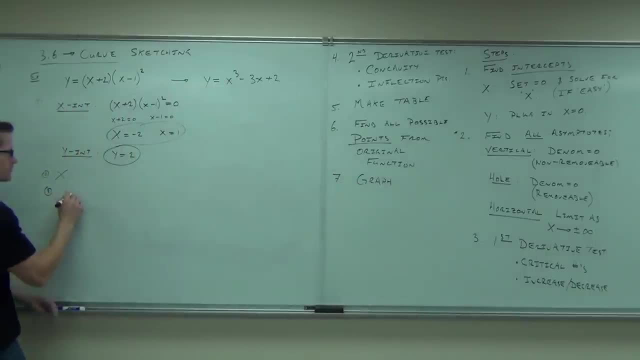 At least doable. So try some of that. So take the first derivative, Let's do that together, Everybody. what is the first derivative when I, when I do that, What was it? What do I do first? 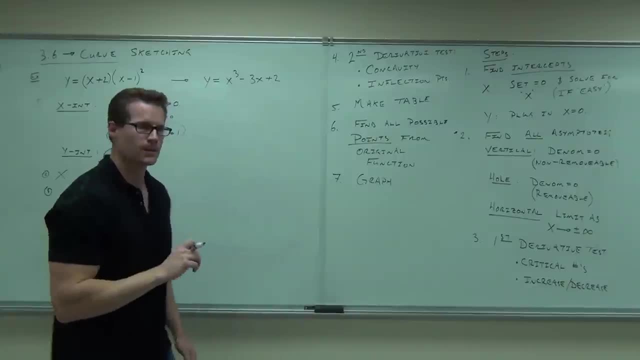 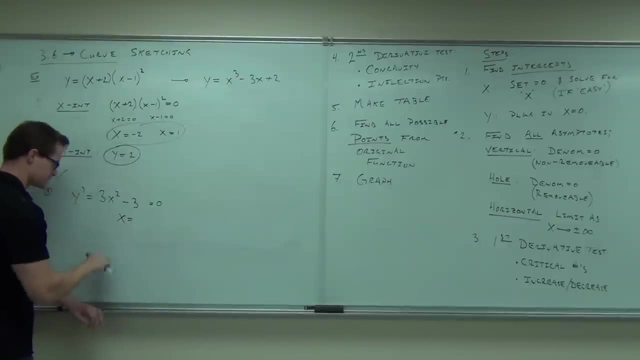 What do I do? What are we gonna do for our first derivative test? If I set that equal to zero, I'm gonna get x equals. well, I'll show the work on that, if you really want me to. This'll be: three x squared equals three. 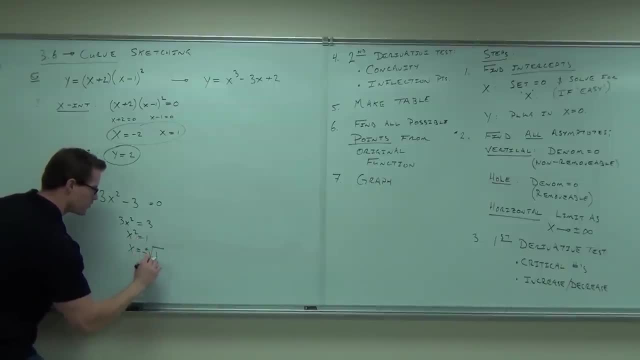 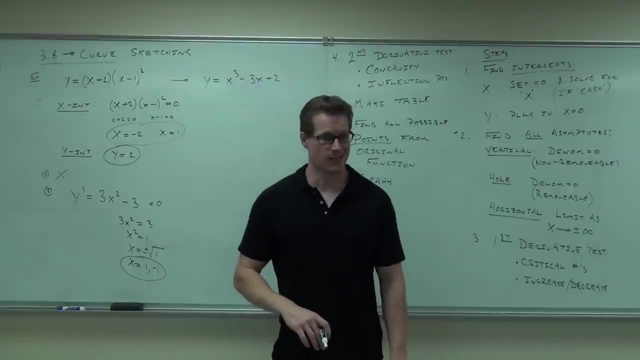 x squared equals one. x equals plus or minus the square root of one. X equals one and negative one. Okay, you okay with that so far? Okay, hey, that's the first derivative test. That's not too bad, Let's do step number four. 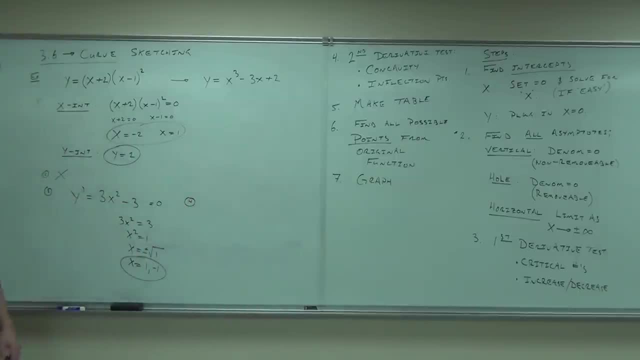 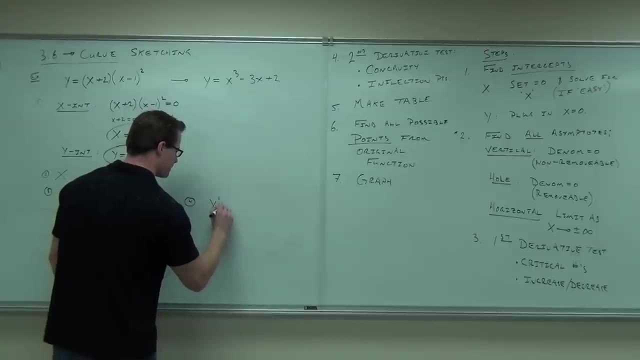 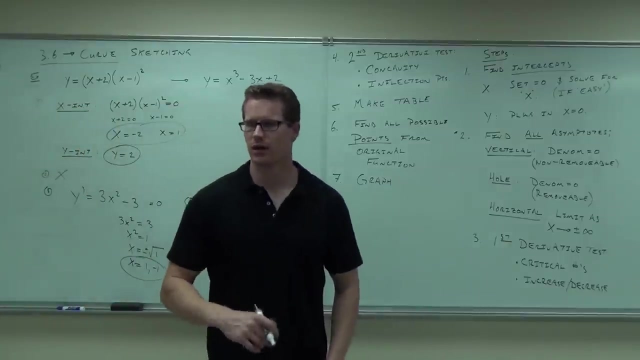 Step number four is: can you do the second derivative test? Second derivative test says: well, take the second derivative. Go ahead and do that now. Take the second derivative. How much is the second derivative? Six times six, Oh, that's beautiful. 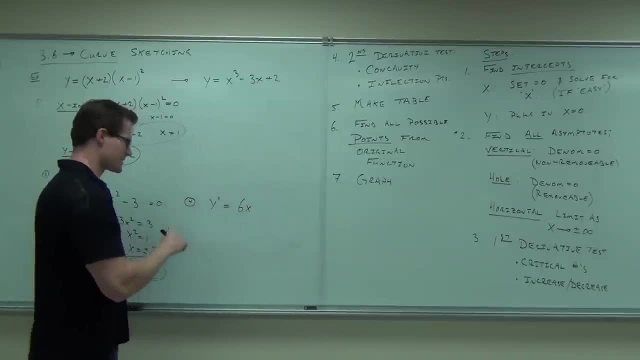 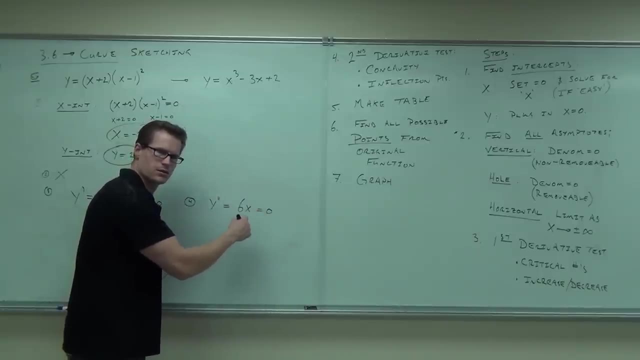 What do you do with that? What do you do with that? six x Set it equal to zero here, When you solve for zero, what are you finding here? Inflection points, You're trying to find possible inflection points. So when you divide by six, x equals zero. 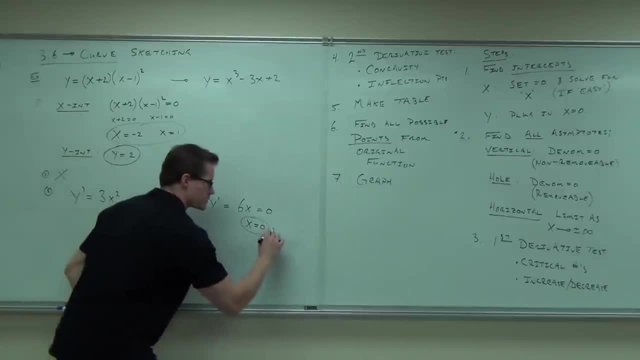 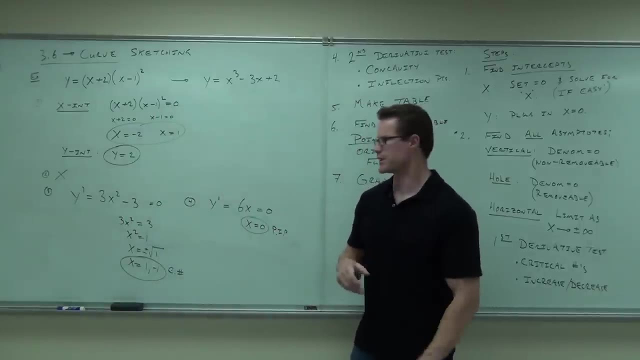 These right here are your critical numbers. This right here is a possible inflection point. Let's recap for just a second before I start making the table for you, and then we'll do the table next time. How many people feel okay on finding x and the y-intercept? 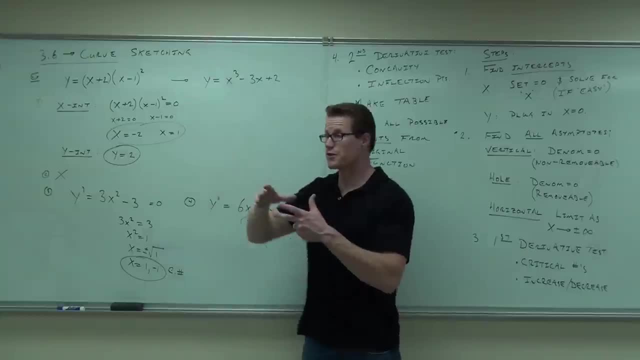 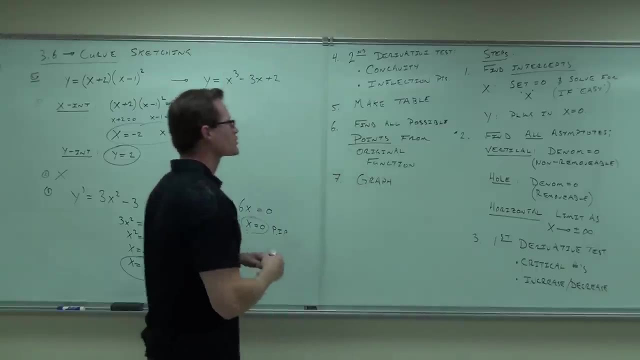 Feel alright with that. Good, that's our basic algebra. Do you feel okay with our first derivative test and our second derivative test? Raise your hand if you feel alright with that. Now step number five. This is where all your work happens, okay? 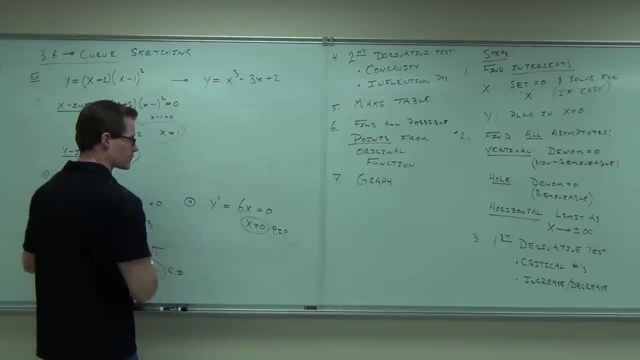 All your work happens right here, in step five. You're going to have. you're going to have what you got from your first derivative, you're going to have what you got from your second derivative and you're going to put it all of it. 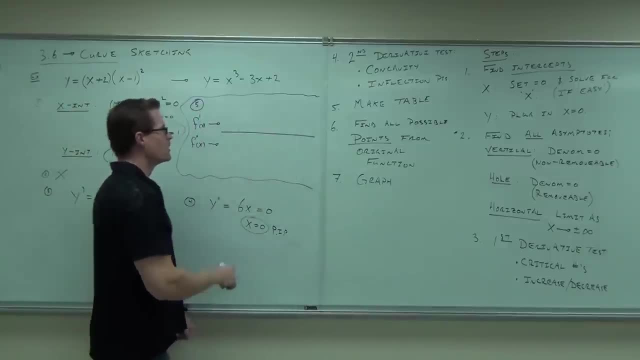 on something that looks almost like a graph. It's a number line. What were our critical numbers? that we needed For our critical numbers? So negative one, positive one, Zero goes on the bottom. Why does zero go on the bottom? 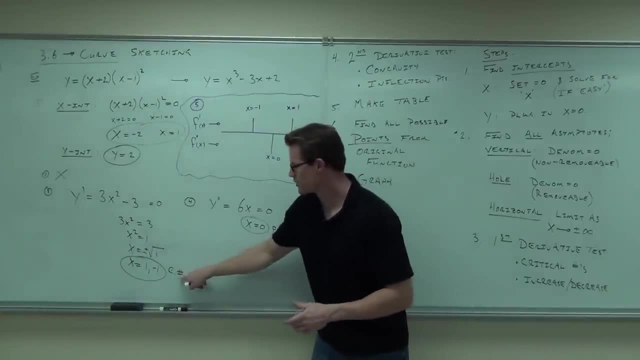 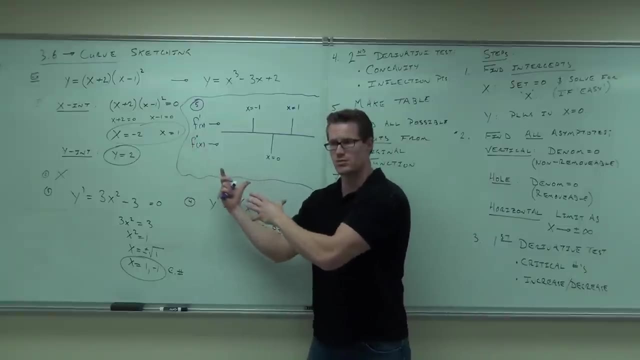 Because of your second derivative. Okay, so critical numbers: critical numbers When on the top. that was our first derivative. That's what we got right. Possible inflection points: that's from our second derivative that goes on the bottom of our table. 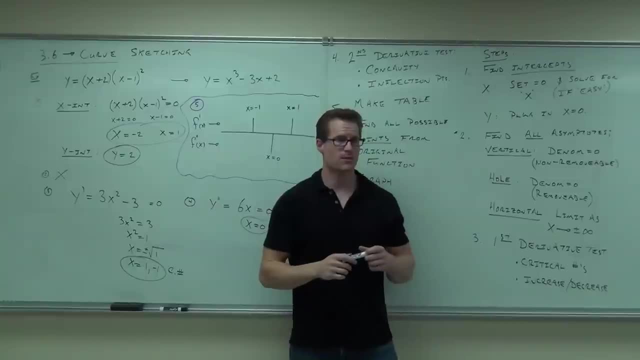 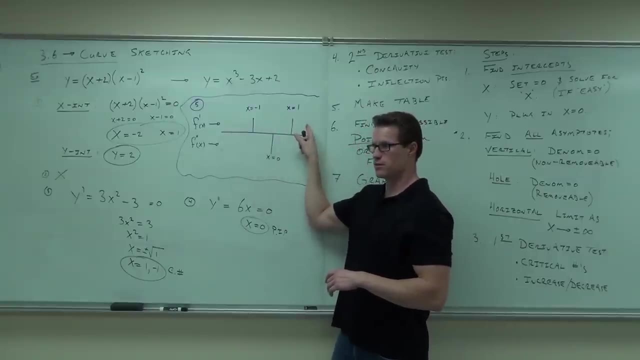 It has to be in order: negative one, zero one. Do you feel okay with that so far? What do you do now? So every single interval here you follow. What number are you going to check here And where are you going to check it? 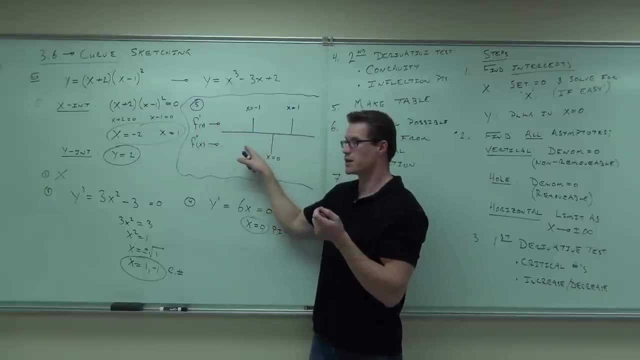 In the first derivative. What are you going to check here? What was it? Negative one? Negative one would work right. It doesn't matter. Negative one, you're going to check it in the Second derivative. Okay, Why don't you go ahead and do that? 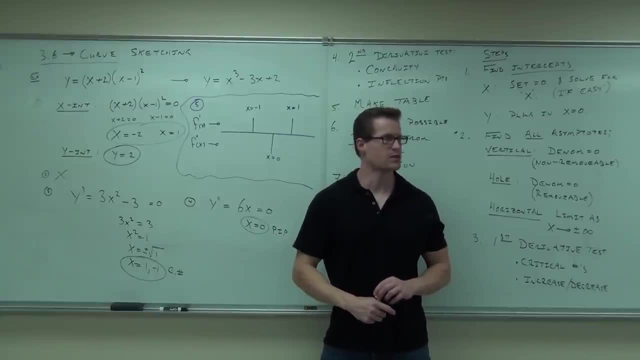 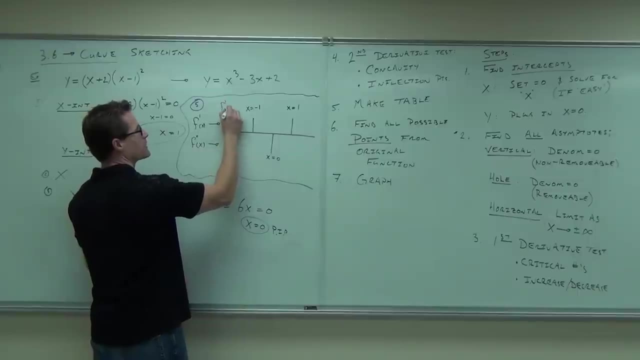 Fill that table out for next time, because that's where I'm going to start next time. If you want to hang out for a second, I'll do it right now. okay For this one, if I plug in f prime of negative two. 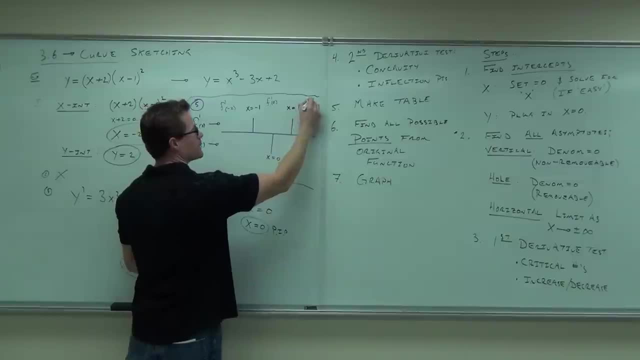 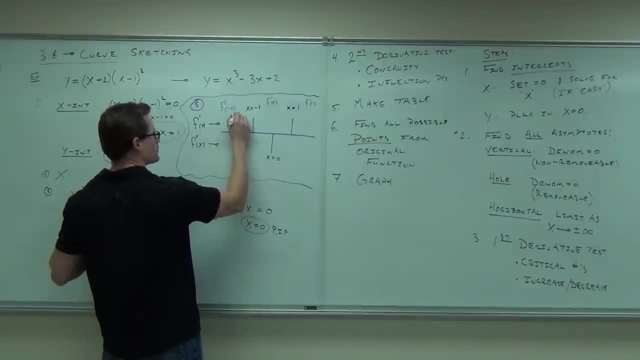 if I plug in f prime of zero, I can do that And f prime of one, I'm doing my first derivative. I'm going to get positive, I'm going to get negative and I'm going to get positive. That means increasing, decreasing, increasing. 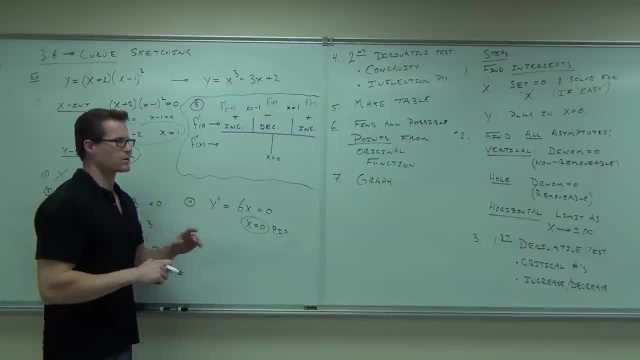 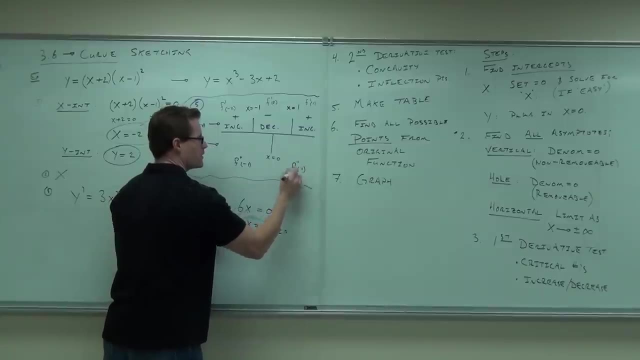 You follow me on that, Yes or no? Yeah, Okay. Second derivative: I'd try f double prime of negative one. I'd try f double prime of positive one. Remember, it's just this interval, It doesn't mean you can't plug those in for your second derivative. 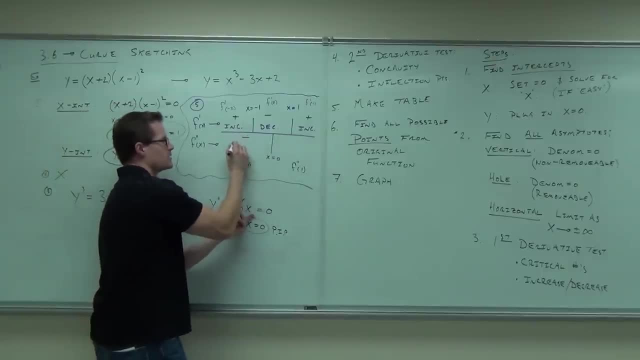 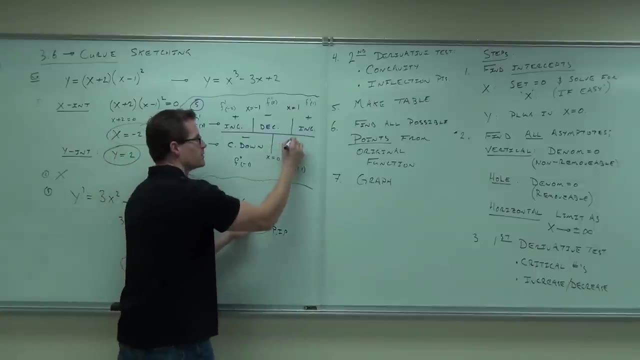 That's okay. Negative one gives you negative. Concave down. Positive one gives you six, That's positive. Concave up: Show of hands, if you feel okay with our concave down, concave up, That right. there is a picture of our graph. 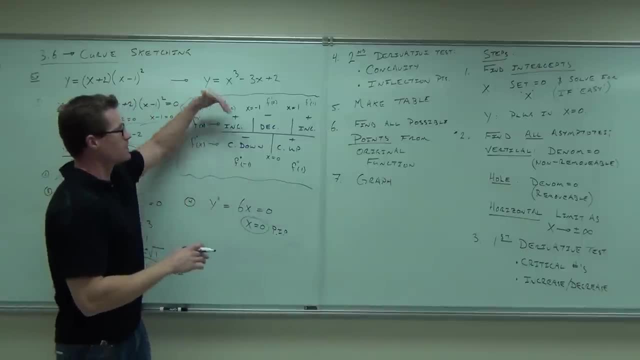 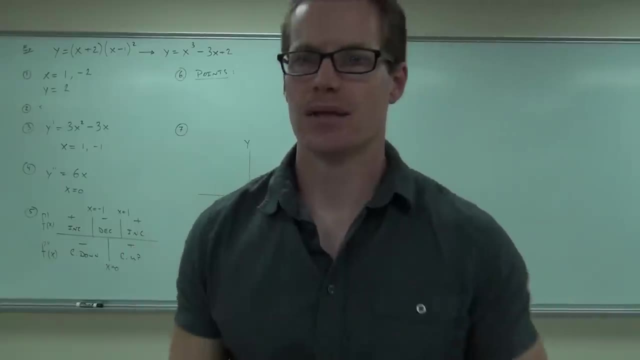 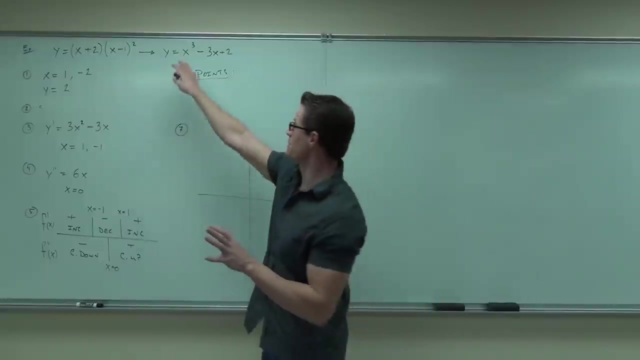 We're done with step five. This basically tells you up, down, up. We just have to find some points and we'll graph that next time. Let's finish that problem. We're dealing with basically just a polynomial. We know that we can take a first derivative pretty easily if we distribute. 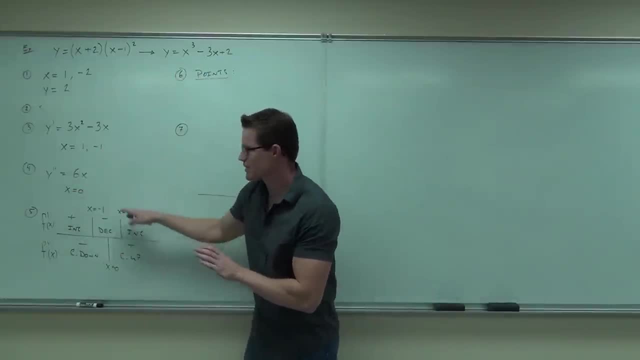 We've already done that, Let's do it. We've already done that, We're going to take that round. First derivative test. second derivative test: we have our intervals of increasing, decreasing intervals of concavity up and down. We also have our relative. 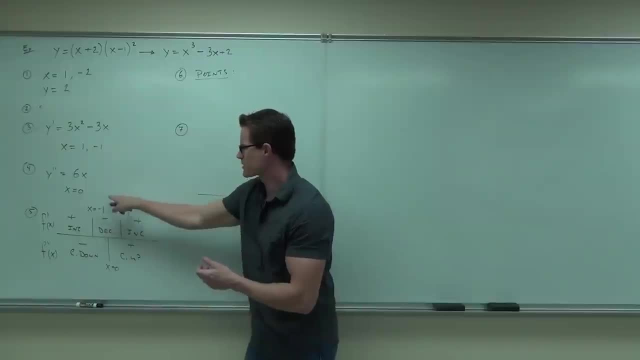 Which one is this, max or min? Relative max, relative min And Good Reflection point. What we don't have is actual points. We need the points now, The steps that we haven't done after you've done your first and second derivative test. 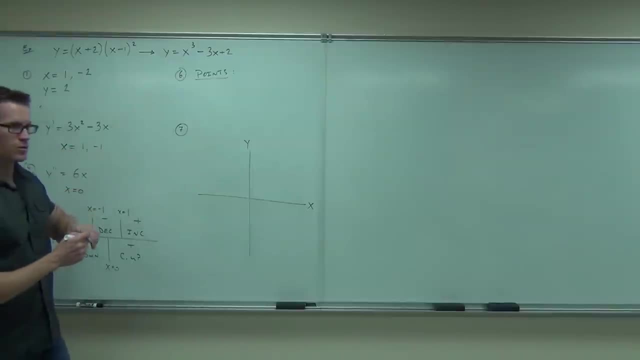 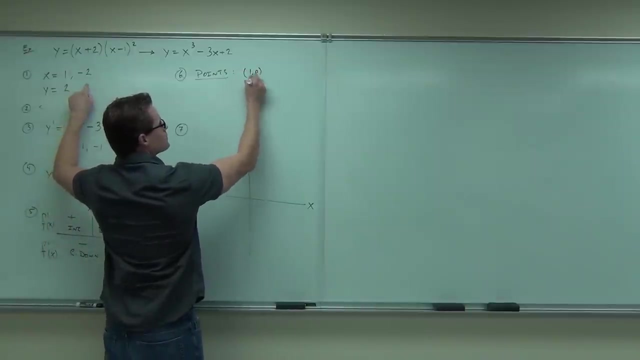 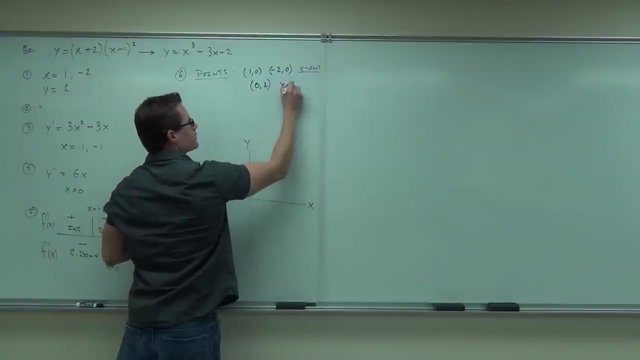 you've made me the table. What I want to see is your points. Go ahead, points. now I know the x-intercepts automatically give us some points. basically one zero, negative, two, zero. those are my x-intercepts. my y-intercept will give me another one zero, two. so x-intercept, y-intercept, but then all of 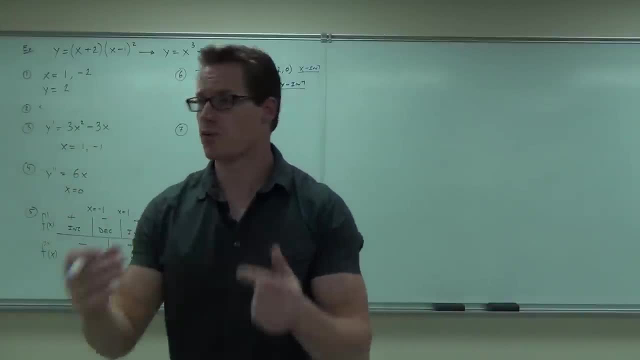 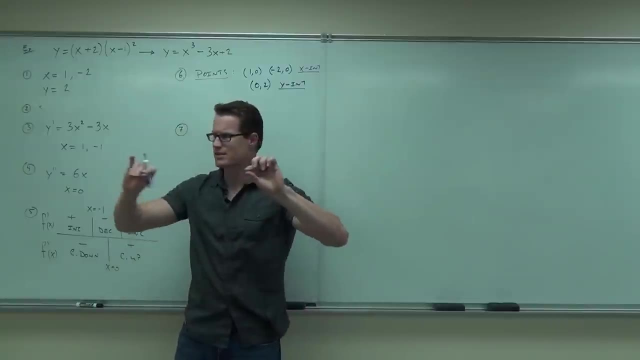 my critical numbers, my critical points like my relative max and min, that's more points. my inflection point, that's another point. so you need to also give me. are you okay on the one zero and the negative two zero. it's my x-intercepts. my y-intercept is at zero two. that's what we got those from. we did that last. 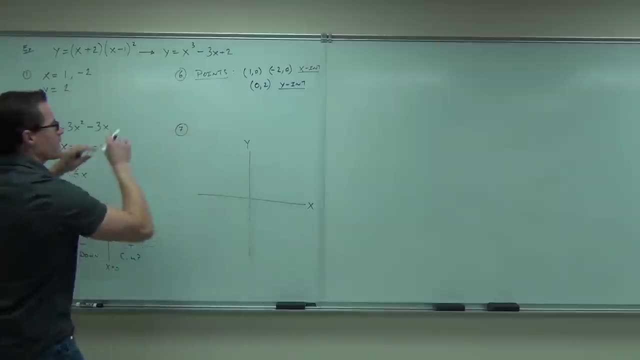 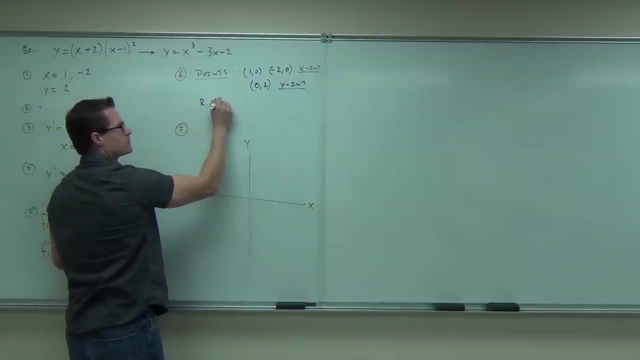 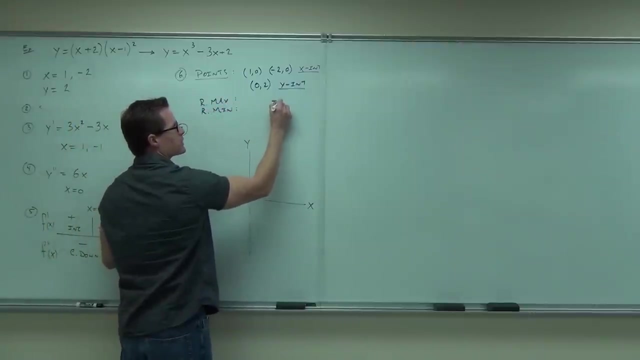 time, right? if you don't remember that, look back at your notes or look at the video. we did that last time. now those were x-intercepts, y-intercepts. we also have relative max, we have relative min and we're going to have an inflection point. 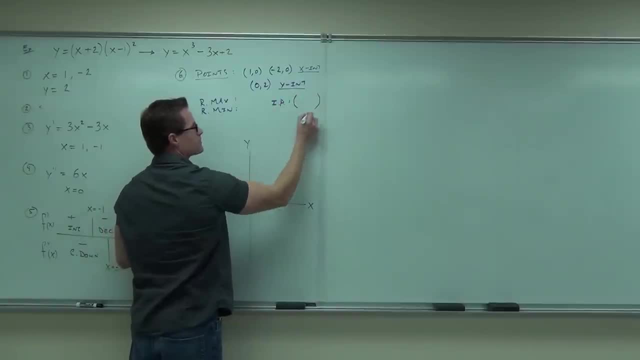 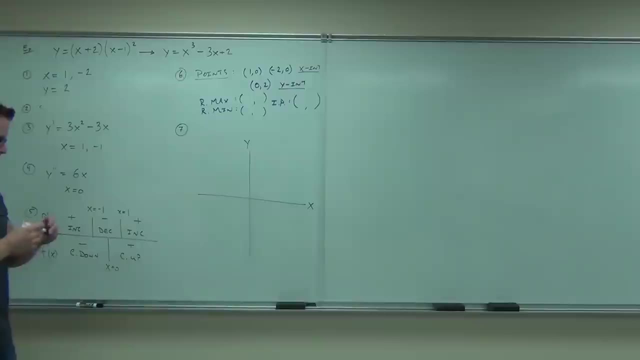 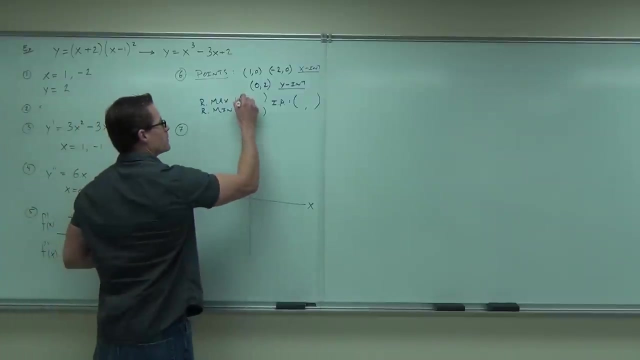 just one of those. can you please tell me what's the x-coordinate for my relative max? the x-coordinate- my relative max negative one to be the x-coordinate of the next you follow. how did you get the zero? good, the original one is what gives you points. so 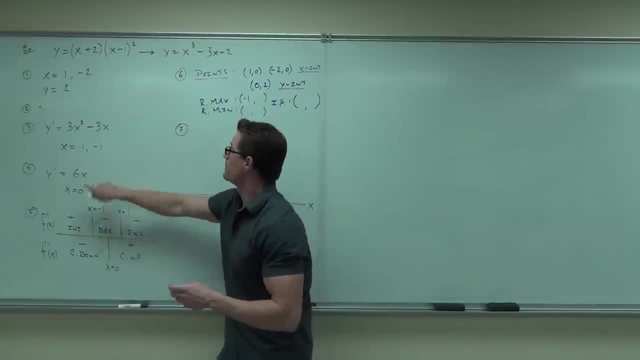 the To find our points out. you take the negative one, plug it back up into here, or this one would probably be a little bit easier, and that will give you out the y value. You follow me. That gives you your points. 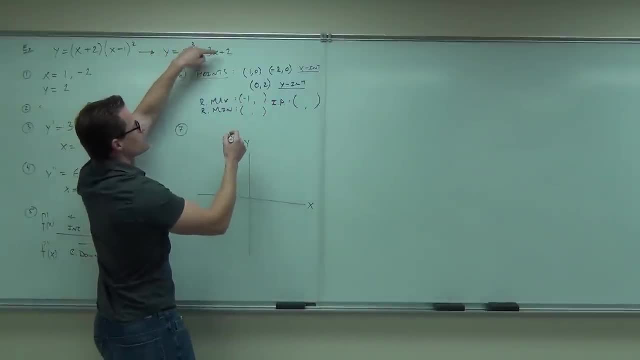 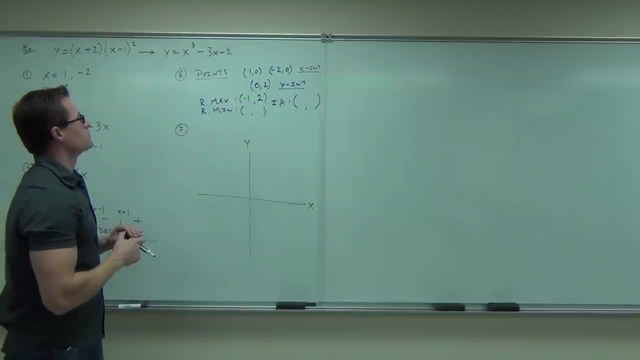 So this is gonna be negative one, let's see. negative one plus three, Two, Two, I think. so I don't know. Let's see. Can you plug it in to this: four Over Over. Ish happens right. 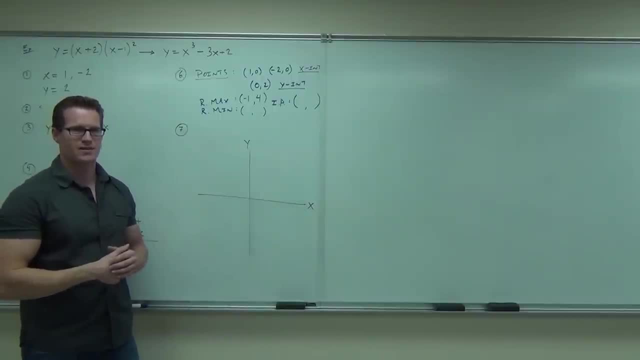 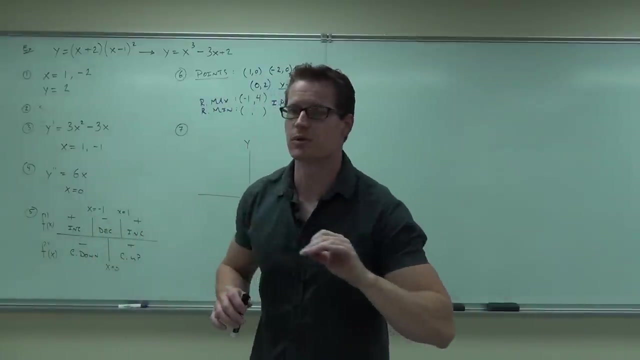 It's all good. What's a little point between friends? huh, A moot point. Right, right, Okay, negative. one plus three plus two, four: Find your relative min. What's the x value for your relative min, please? 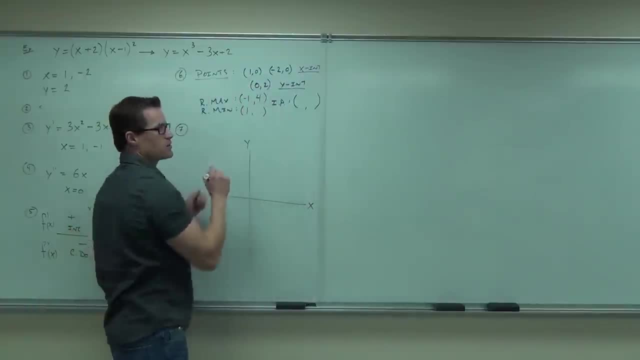 What is that One? So I'm gonna put a one here. How do I find the one? What's the y value? Ah, look at it, That one's gonna be Zero. That one's zero Inflection point. 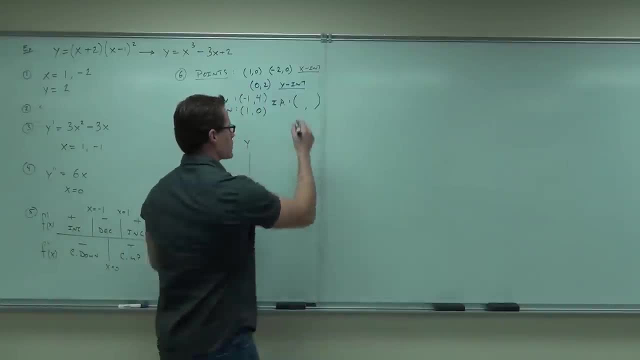 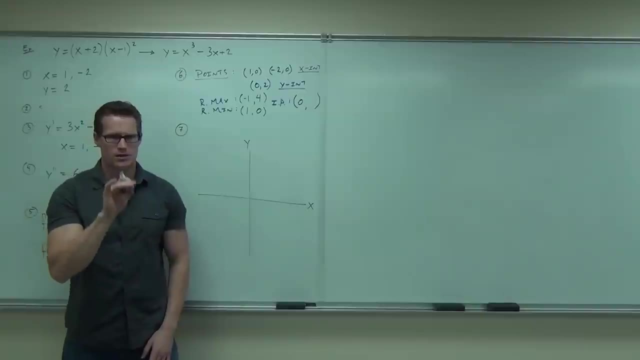 Can you please tell me my x coordinate for my inflection point? Zero, Zero, Zero, comma Two. That's an interesting point, isn't it? Not only is it the y intercept, it's also the inflection point. So we have that point twice, not a big deal. 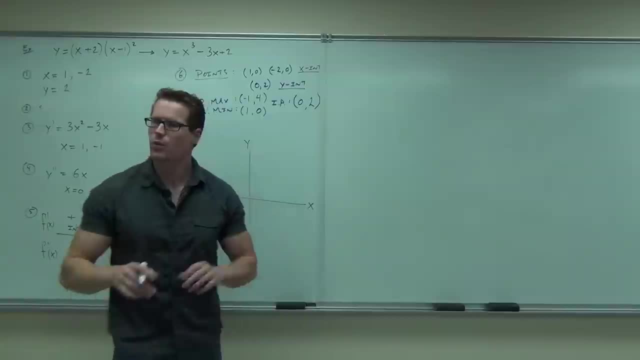 You feel okay with the points, Here's how to label them on your graph. First, you're gonna just work your way down, just like we did with the process. Start with your x intercepts. One zero, put a point. 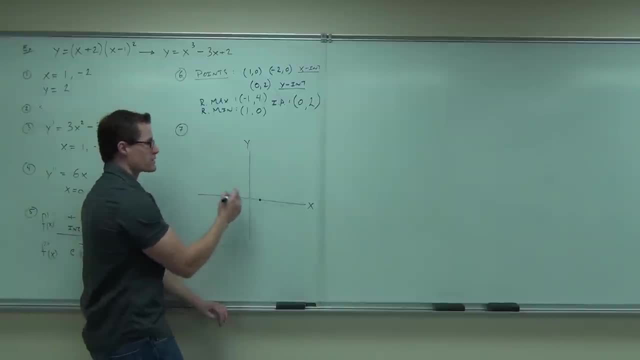 Negative. two. zero. put a point. Those are my x intercepts. My y intercept is zero. two. put a point Relative max happens at negative one. four. Put a point. relative min happens at one. zero. Put a point. that's already there. 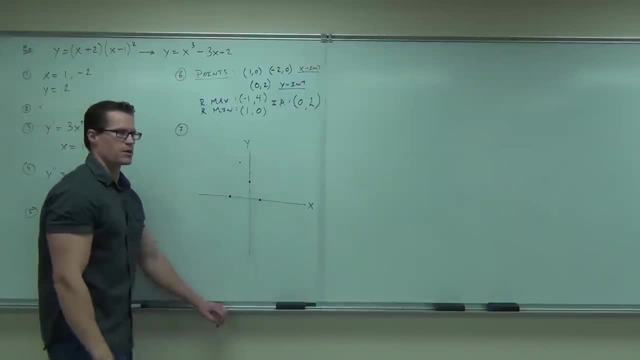 Now here's how I like to label these points. Are you okay on, firstly, the four points that we get? I mean, we have one, two, three, four. we have six of them listed, but we have two pairs of points. 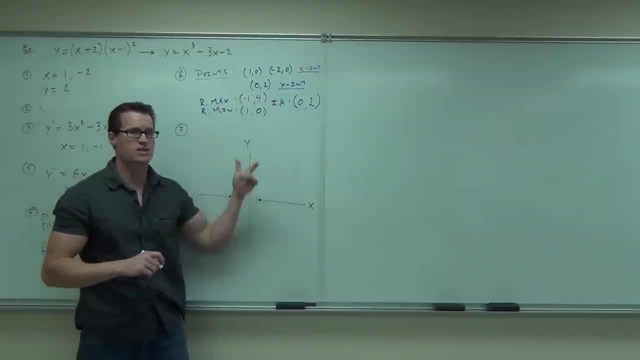 Here's also what I like to do: When you have the inflection point, you need to label it inflection point. That way you see the change in concavity. So which one of these is an inflection point? One, two, three, four, five. 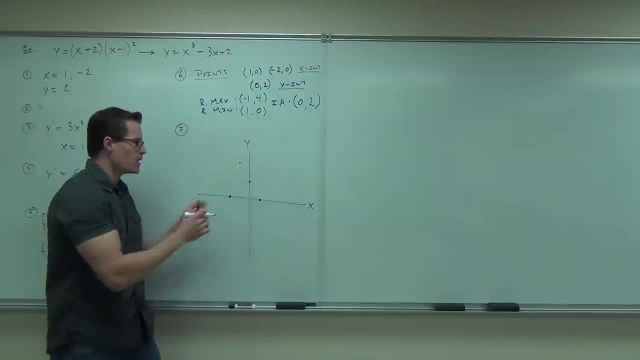 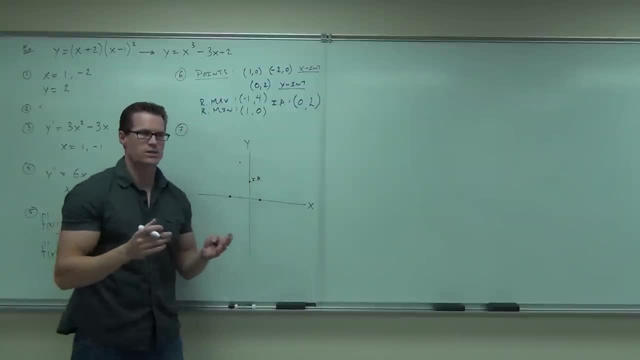 So I'm gonna label that inflection point just IP, just so you know it's IP For your relative extrema, your relative max and relative min. what I like to do, I like to draw a little dotted line. So for my relative max, which is at negative one. four: 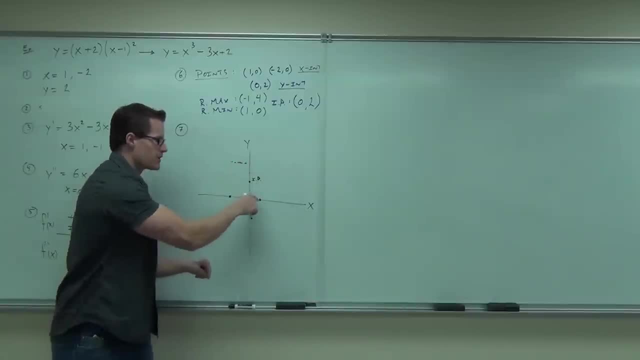 I like to do that. That says I can't go above that For this one, this one, zero. I know that was a relative min, right, I'm gonna do this. I can't go below that. I know that my graph is gonna bounce off of those dashed lines. 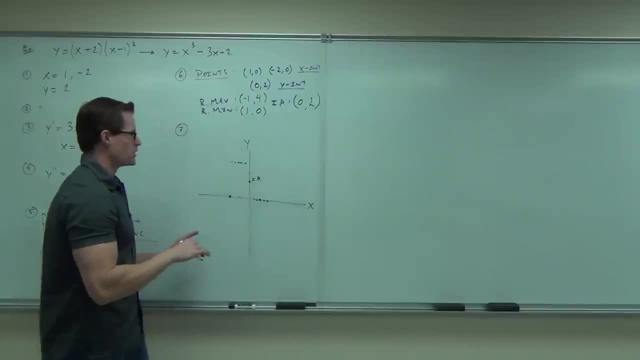 Do you follow me on that? That's what's gonna happen here. It's gonna. we'll follow in our graph: Go up, bounce off, hit an inflection point, bounce off and then keep going forever. Does that make sense to you? 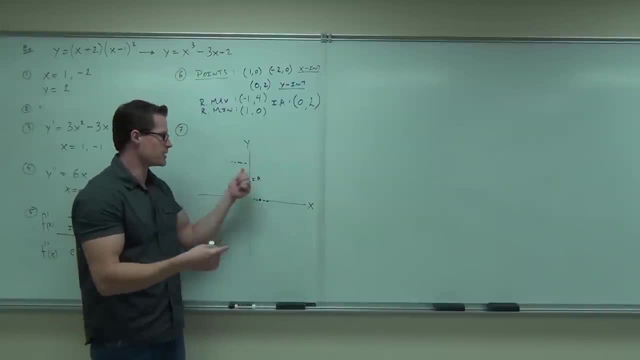 So label those things with something like that: Do the inflection point, change the concavity, Do your relative max, relative min, do little dashed lines, That way you know you're not gonna go past that. You're gonna be changing those values. 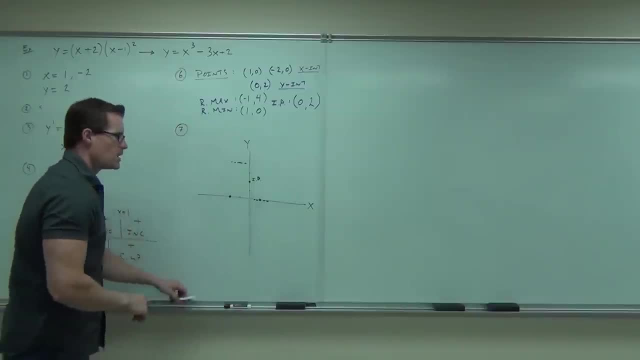 So let's see if we can graph our graph. If we follow this table and associate them with these points, we should have a pretty good looking graph. It says: you're gonna start out, you're gonna be increasing. Which way is increasing? 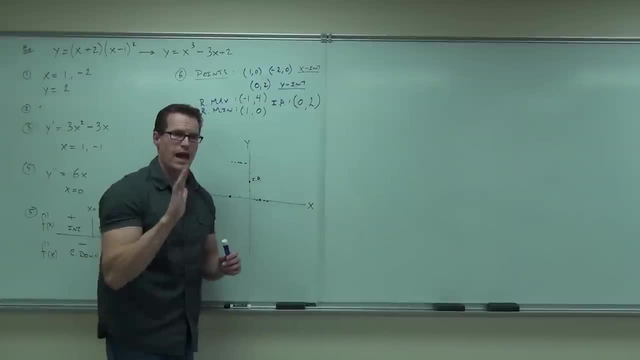 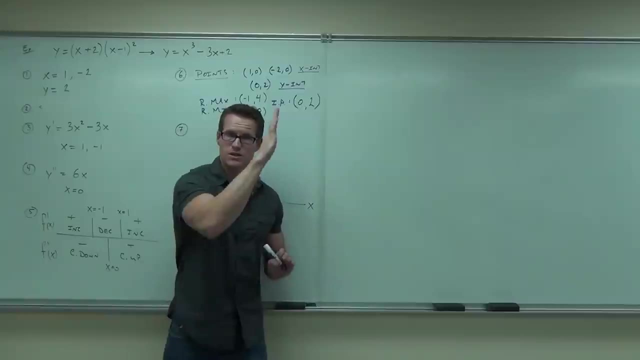 This way or this way. This way, So we're increasing. How are we increasing Concave down? Concave down. So increasing concave down, Increasing: this is concave up, this is concave down. You follow. 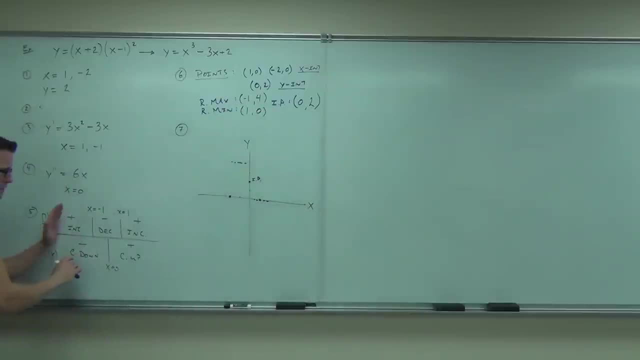 We're increasing concave down. It says: increasing concave down. We're gonna go through that point, So increasing concave down. It's gonna be hard to draw that way. I tried to do it: Increasing concave down. 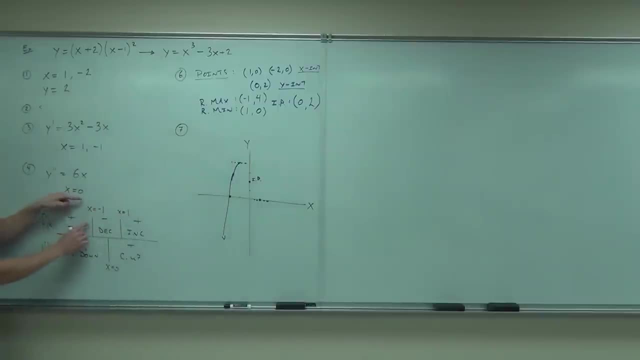 Are you following me on this? I'm gonna hit that what it says: a relative max Increasing concave down relative max. Then I start decreasing. How am I decreasing? Look at the board here real quick. How am I decreasing for this interval? 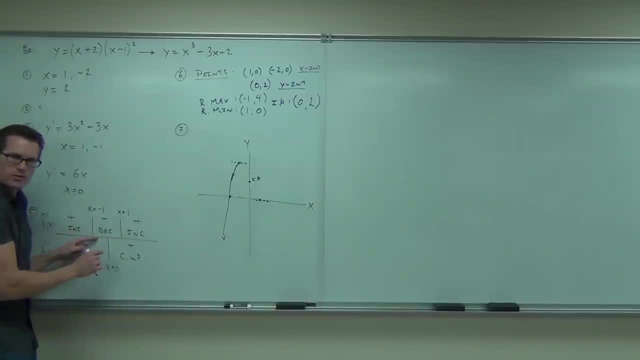 It says: you're decreasing, but you're doing it concave down, You follow me. So for this little interval right there, it says x equals zero, right? It says: from negative infinity to negative one on the x-axis, you're increasing, concave down. 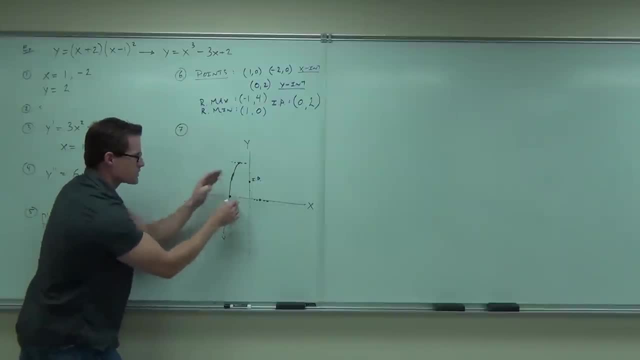 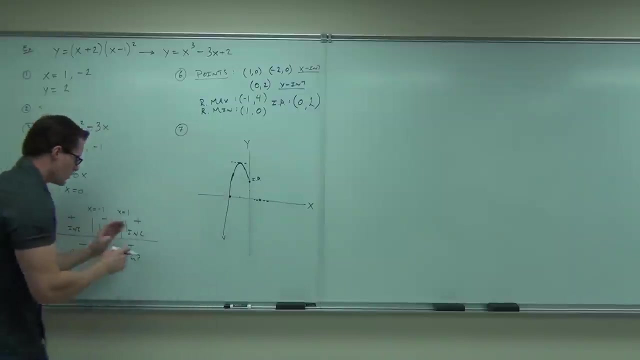 From negative one to zero, you're decreasing concave down. That's this way, Decreasing concave down. You still okay with that? Yes, though, Yes, After zero. After zero, it says I'm still decreasing. 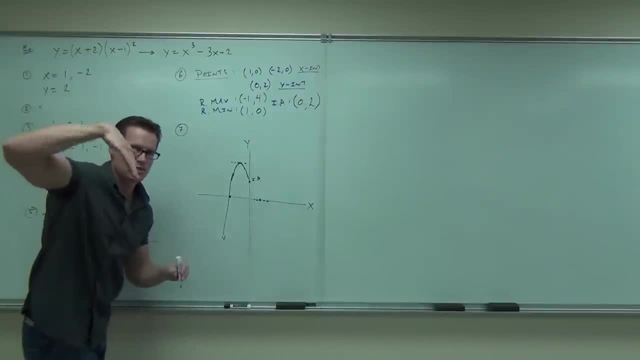 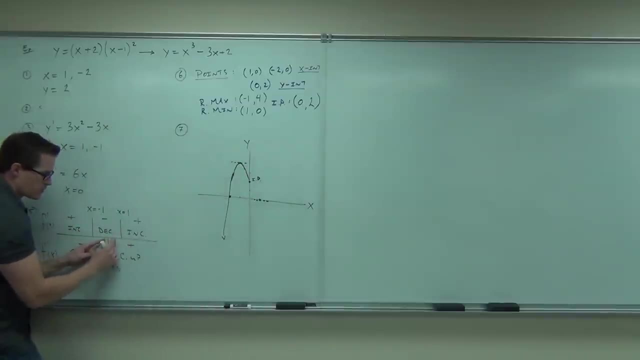 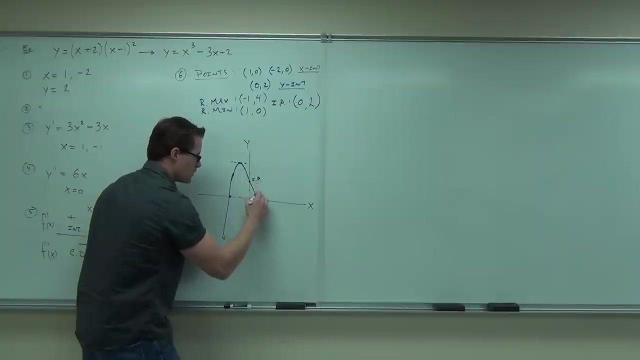 I'm still decreasing, but now I'm concave up. That's like this: Decreasing concave up. So that was my switch in concavity: I'm still decreasing from zero to one, From zero to one. I'm still decreasing but I'm concave up. 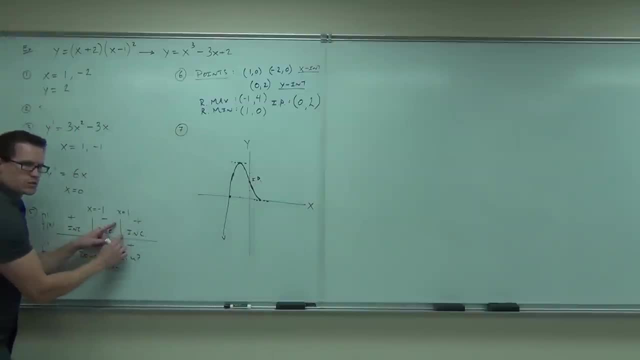 As best you can. After x equals one. That's why I made the point earlier in the class that you have to follow the x-axis, Right? So you go. okay, after x equals one. I'm increasing again and I'm concave up. 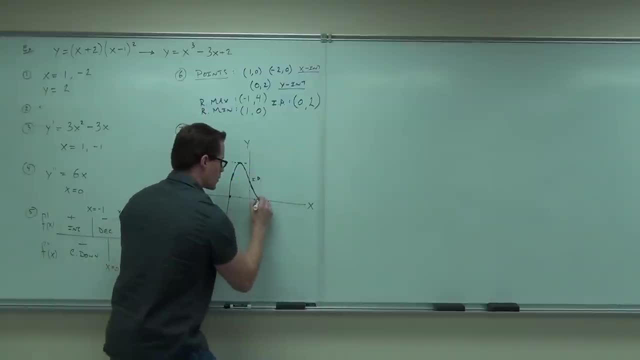 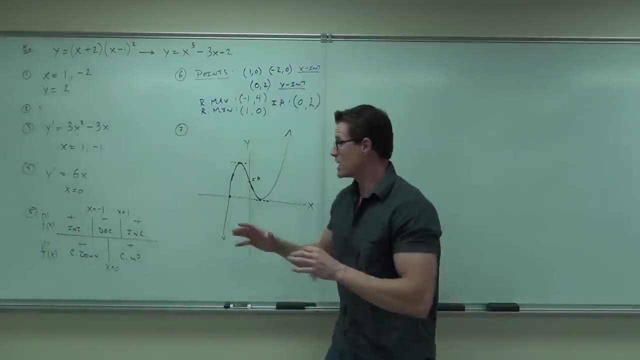 Increasing concave up looks like that. That probably should be a little more narrow. So that's the idea. Can you get this graph from this picture of the graph? How many of you would be okay with that? So follow along the x-axis. 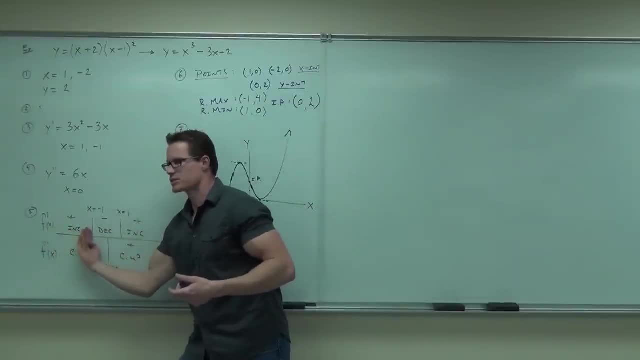 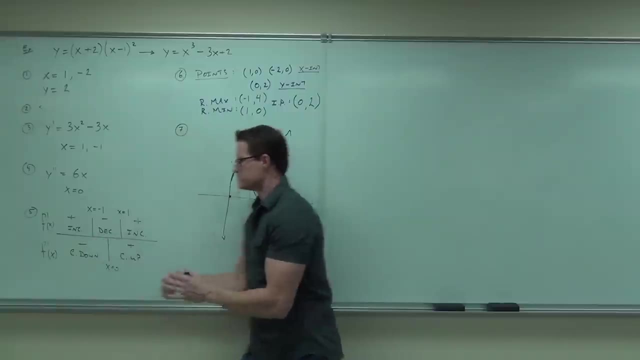 Start from the left, work your way right, Increasing concave down until x equals negative one. Right there, What's the point for that? For that little interval decreasing concave down, Right there. For this next interval, decreasing concave up. 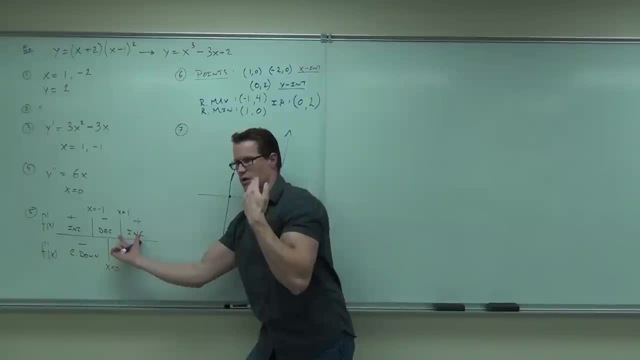 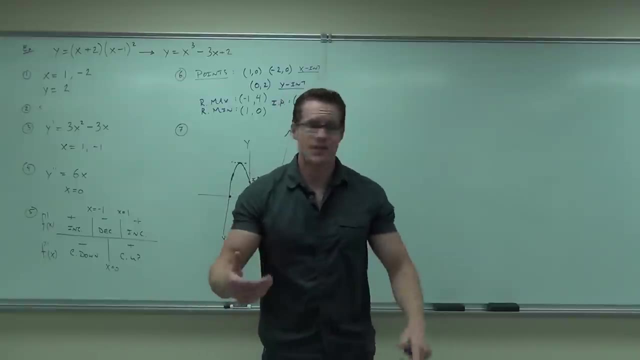 Right there, Last interval. one from x equals one on Increasing concave up And we have our picture Now. of course it's just an x cubed, So we kind of have a picture of that anyway, But the double root's interesting, right. 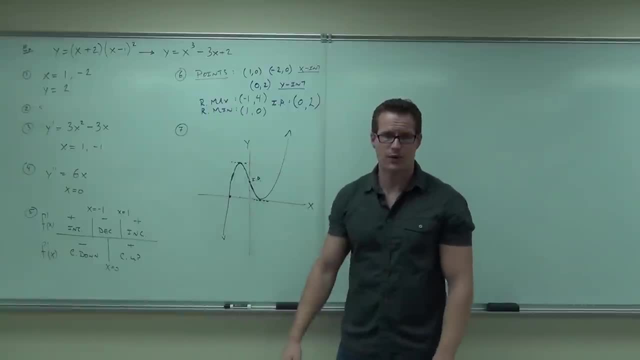 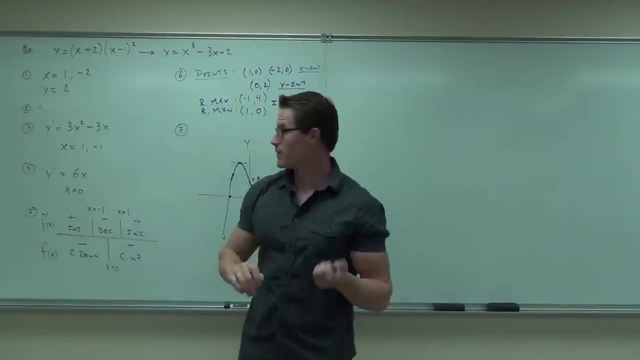 We were able to find that, We were able to find all these points. That's a pretty accurate graph, Fairly accurate. How many of you feel? just fine with it All? right, Now I'm going to erase this because it takes a long time. 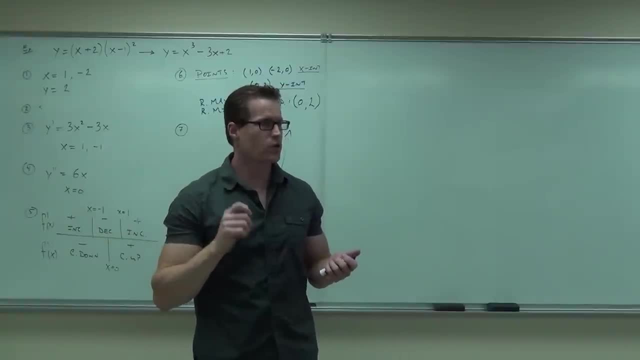 A lot of board space to do these problems. We're going to graph some rational equations You ready for. rational Rational are harder, First because the derivatives are harder And second because you have asymptotes. That's what makes them harder. 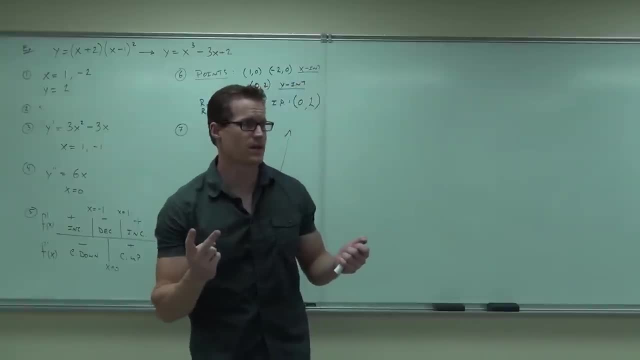 So I'm going to try to get through two. today. We have about 40 minutes, 30 minutes or so 35 minutes right now, So they take a long time. We're going to try to get through two, All right. 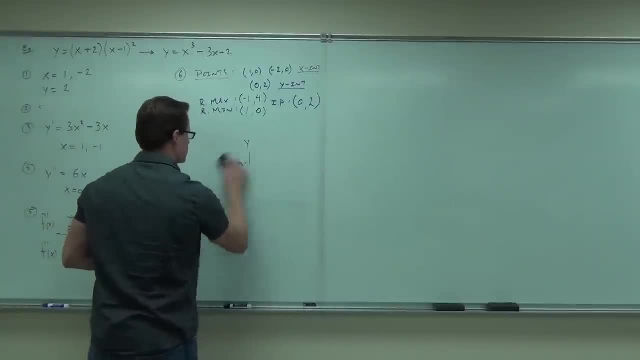 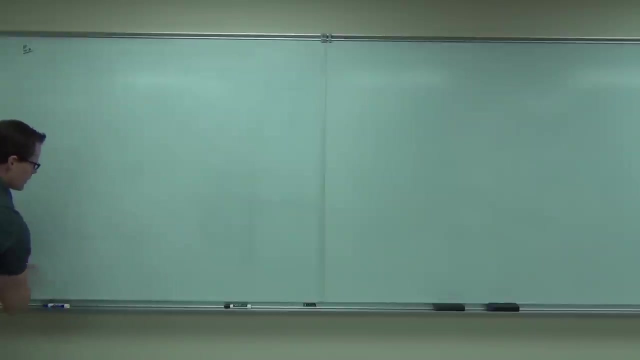 Let's see. Oh yeah, Were there any questions on that? Now the question is: do I do that on purpose? I think you'll never know. I'm not going to rewrite the steps because I gave them to you last time. 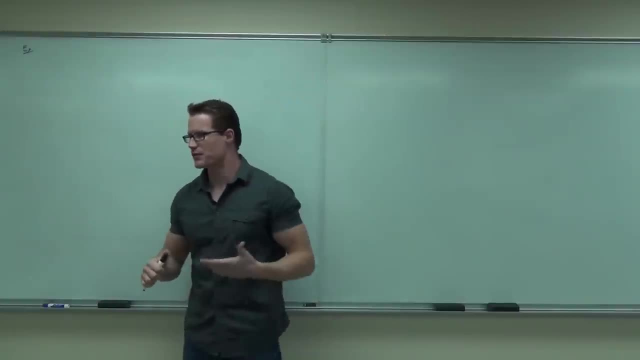 They're on the video if you need to check those out again. The steps were: one through seven. Number one: x and y intercept. Number two: asymptotes, if it's rational. That's why we didn't have a number two up here. 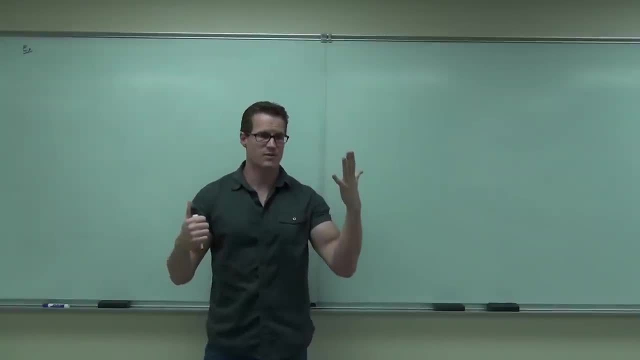 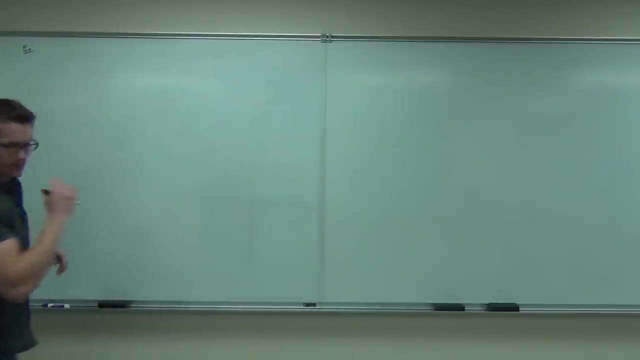 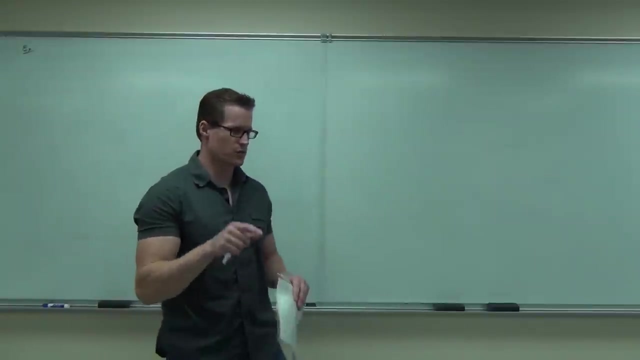 Three first derivative tests, Four second derivative tests. Five is make the table up, Six is make the points And seven is graph it. So we're going to follow the same seven step process the whole way through. By the way, we are going to be dealing with some roots on this, so if you take your calculator, 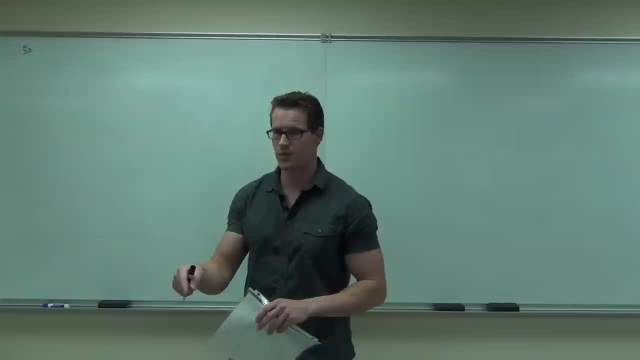 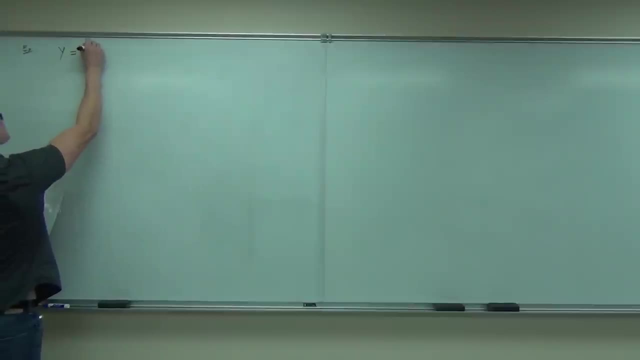 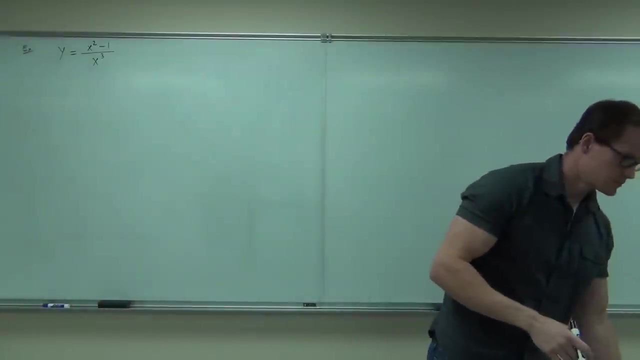 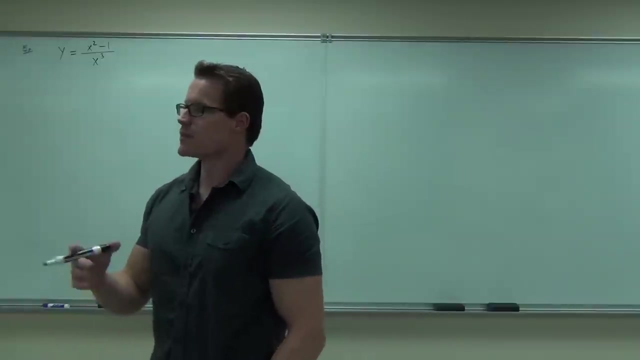 out. I'm going to need some calculator work from you on this, All right, So let's get started. Okay, So x squared minus one over x cubed. Step number one- hopefully the algebra type stuff you find your x and your y intercept. 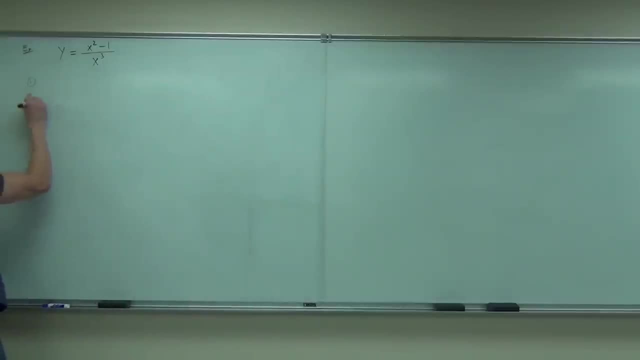 So we're going to do every step together here. X intercept would happen where you set your function equal to zero. Yeah, You follow me. Set your function equal to zero and then you solve it. Well, if you set your function equal to zero, basically, that's just where the numerator 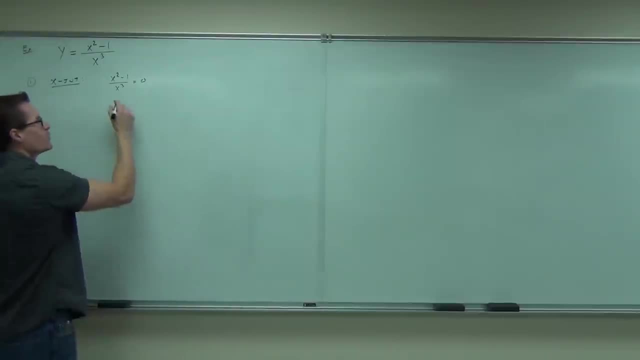 equals zero. The denominator if it equals zero is undefined. So we really just say okay. even if you want to think about it this way, multiply both sides by x cubed. you still get x squared minus one equals zero. What are my x intercepts? 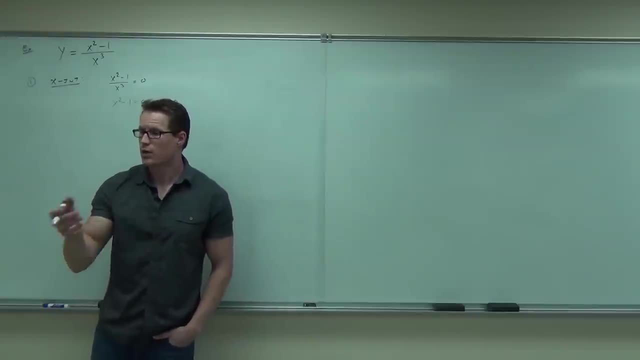 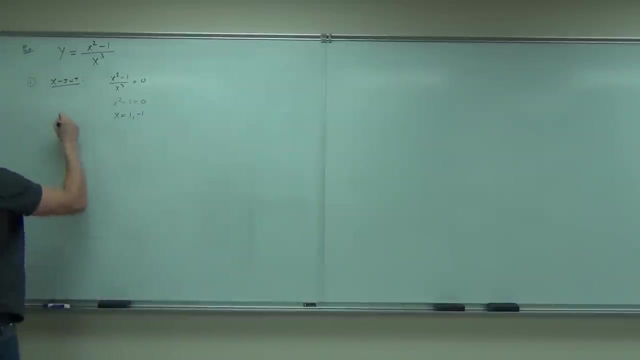 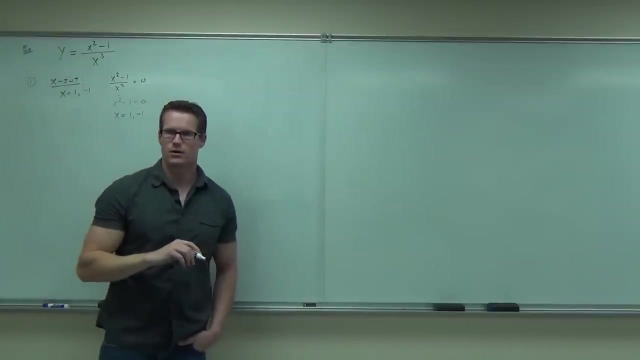 One and negative one. Say what One and negative one. One and negative one? Very good, Add one. take a square root Or factor. Either way you're getting x equals one negative one. Are you okay with that so far? 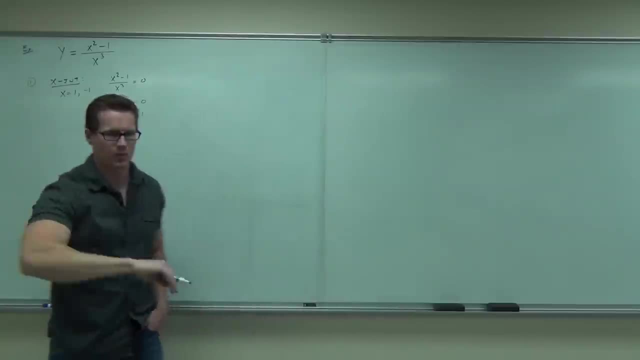 You sure? So if the numerator equals zero, no problem. That's how you find your x intercepts. for any rational function, Numerator equals zero. You got it Now y intercept. Y intercept says you plug in x equals zero and you find out an answer. 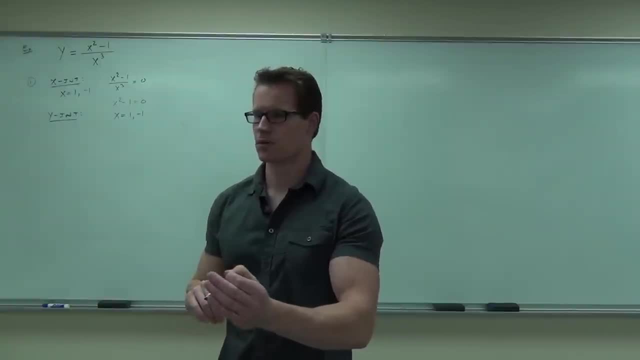 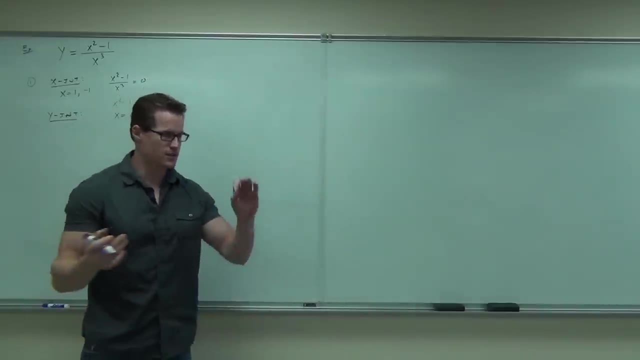 What do you get when you plug in: x equals zero, Negative, one over zero, Negative, one over zero. That's a problem. That means there is no y intercept And we're going to find out y in step number two, but it does not exist. 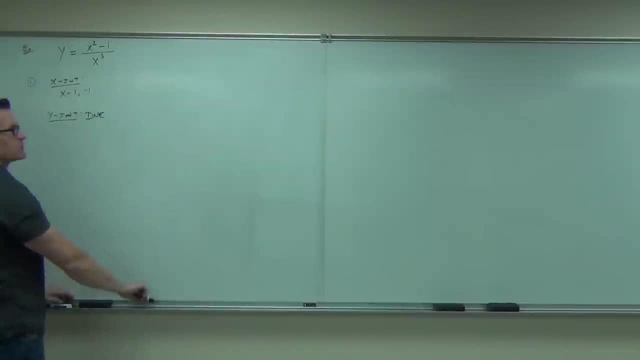 I'm going to erase little parts so we save space, But this is from: x squared minus one equals zero. That gives the one a negative one. Step number two: Oh, step number two is a good one. Step number two is a good one. 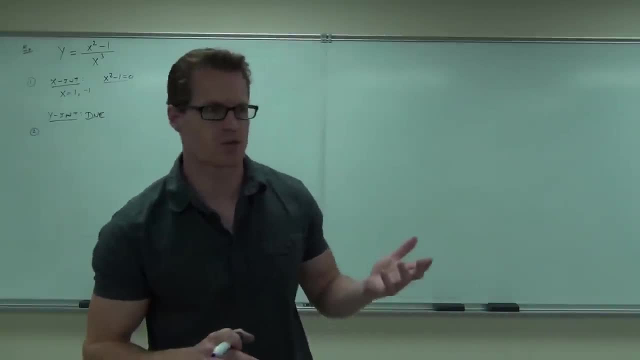 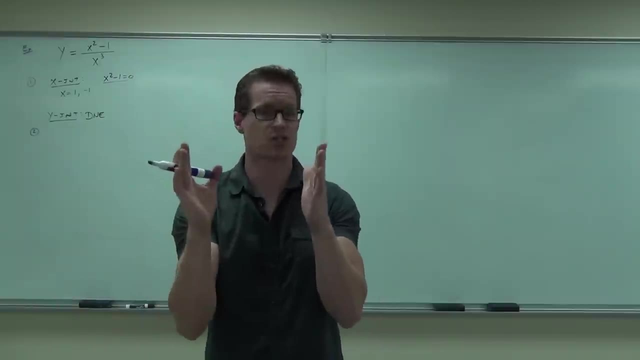 Step number two is where you find out all the asymptotes. Now you might be thinking: who cares about asymptotes, Don't we have increasing and decreasing? The asymptotes tell you most of what you need to know for your graph. They really say: here's your sections. 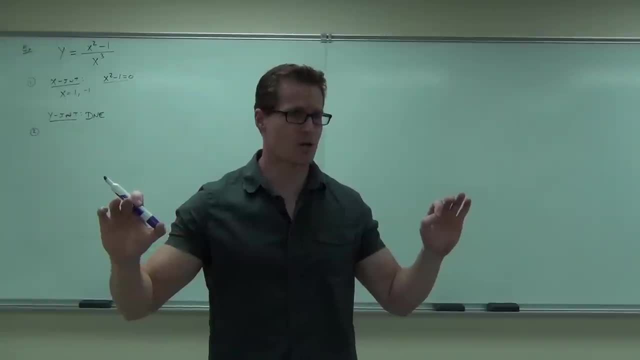 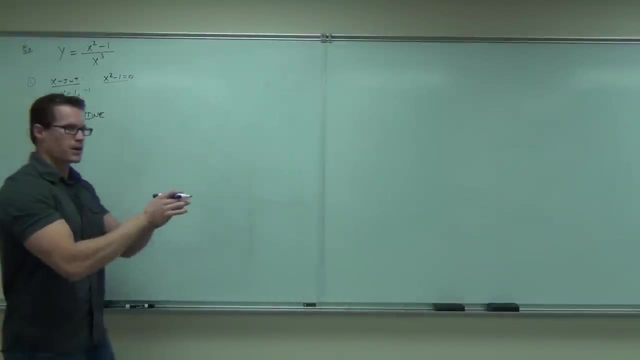 Here's what you're going to do in those sections. Basically, if you knew the asymptotes, you can almost guess what this graph is going to look like with just a couple numbers. So we're going to find our asymptotes, both vertical and horizontal. 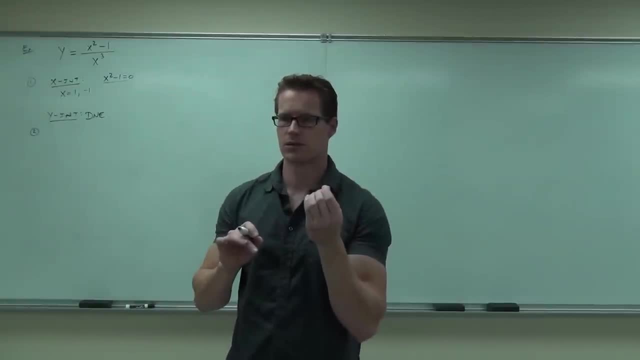 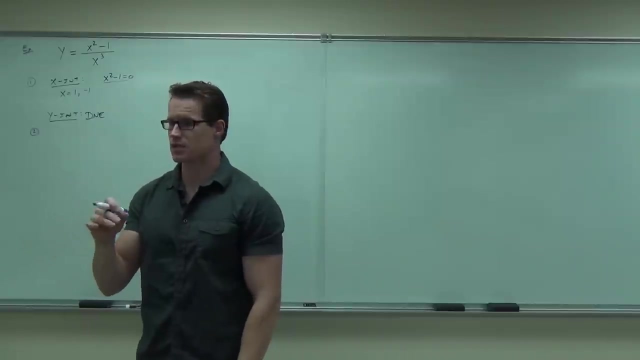 How do you find vertical asymptotes? No, not derivatives. We don't do calculus until step number three. by the way, Good, When the denominator equals zero, you're going to have discontinuities, right? Those discontinuities are equal. 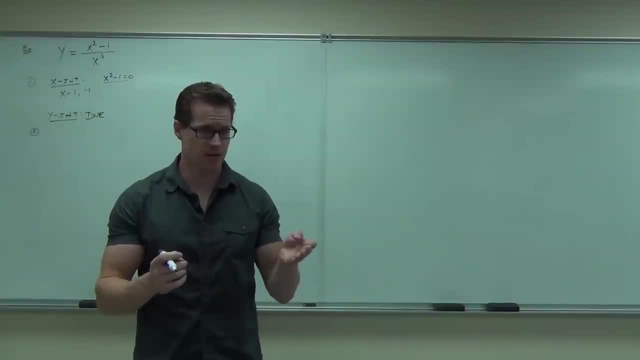 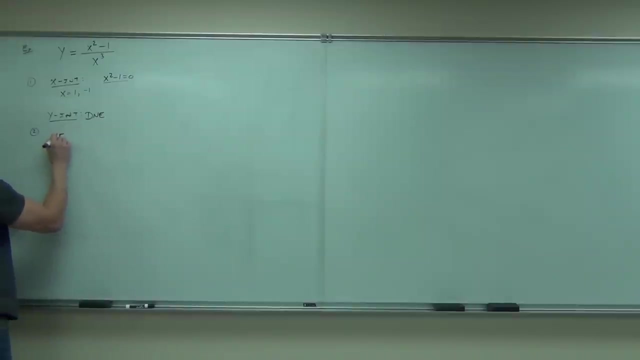 They're either wholes, if you can cross them out, or asymptotes, if you can't. So you'd say: x cubed equals zero and x has to equal zero. Can you cross out the x cubed with anything? So then what that says is there's a discontinuity. 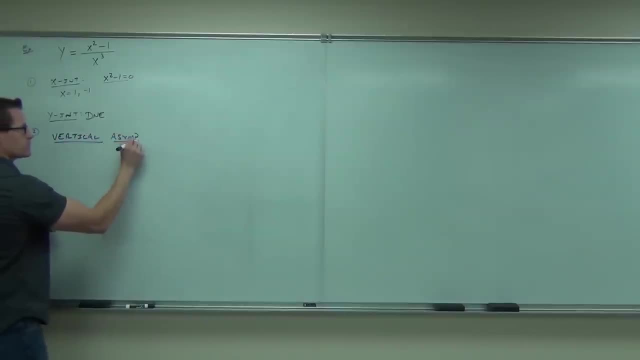 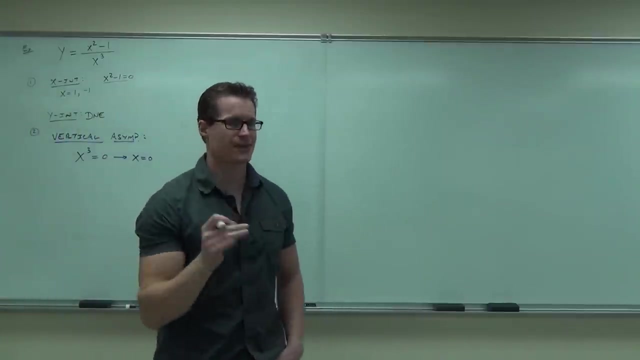 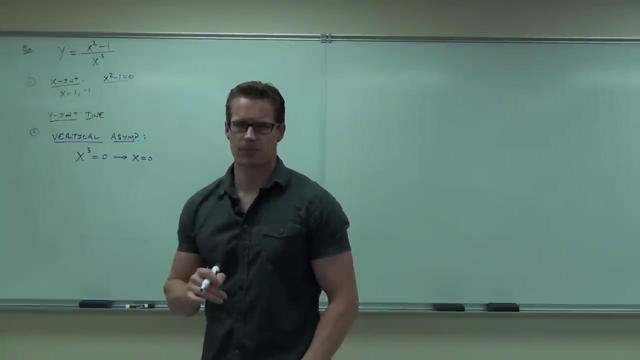 A vertical asymptote occurs where x cubed equals zero, or in other words, x equals zero. That's going to give us a vertical asymptote at x equals zero. Now, let's be careful. If you were able to cross it out, you would do that. 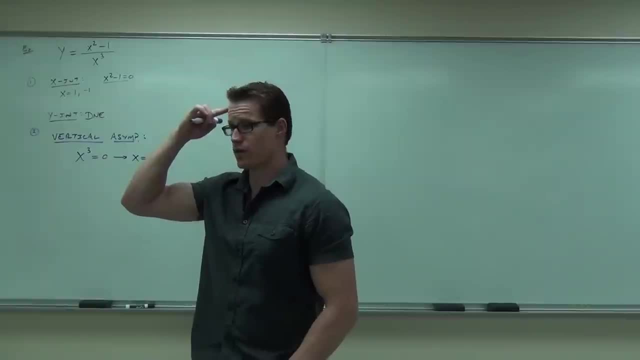 You'd cross out that discontinuity. You'd just keep in your mind that there's a hole there, all right, And you'd have to identify the hole. So it's a little bit easier than an asymptote. You'd cross out the problem. 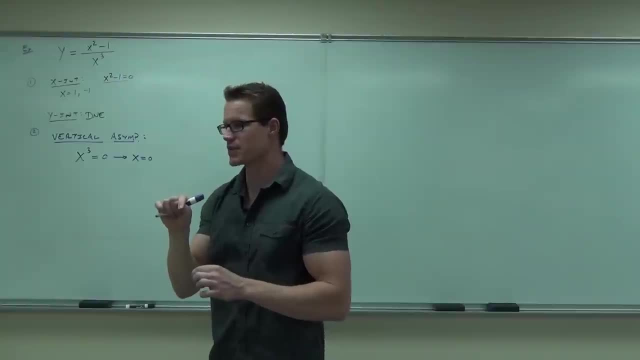 You'd say that a hole exists at this point and you'd put a hole in the ground. Does that make sense to you? That's what you would do. I think I've shown you how you do holes. I think I gave you x squared minus 4 over x plus 2.. 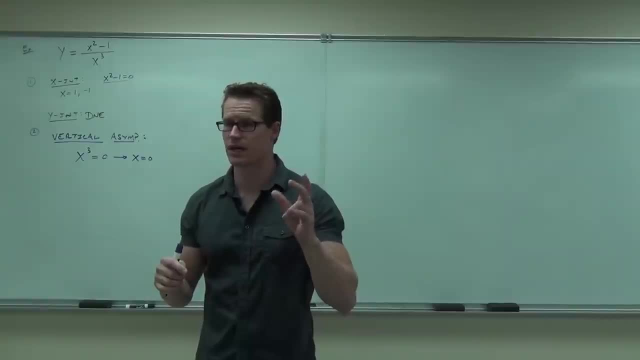 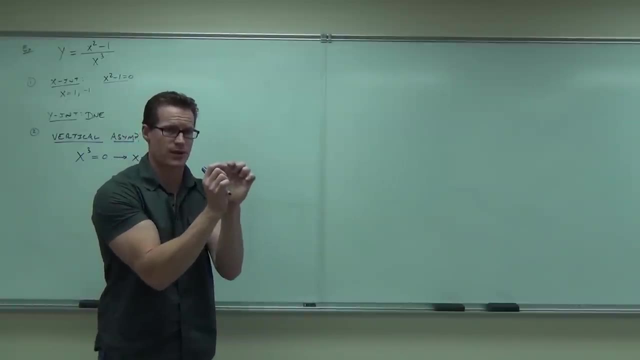 The hole would exist at 2.. And then you would find that value. You'd put a little circle there and it would just be an undefined little point. You follow me on that, Okay, so that's what you would do with holes. 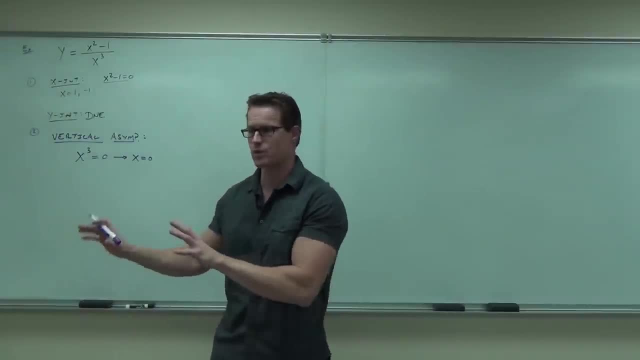 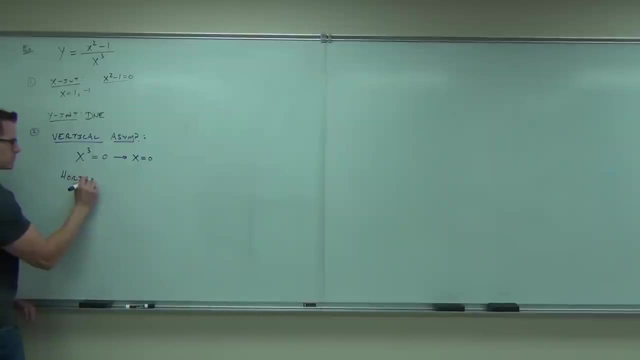 Most of the time, I'm going to give you asymptotes. Most of the time You will have some holes. Most of the time, asymptotes. How do you find horizontal- Yeah, you're right- A limit as what? So, really, there's two of them, right? 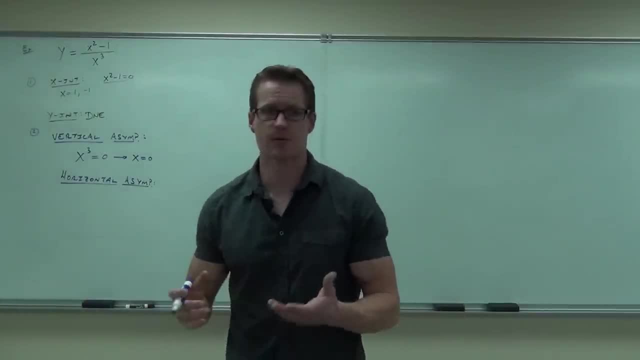 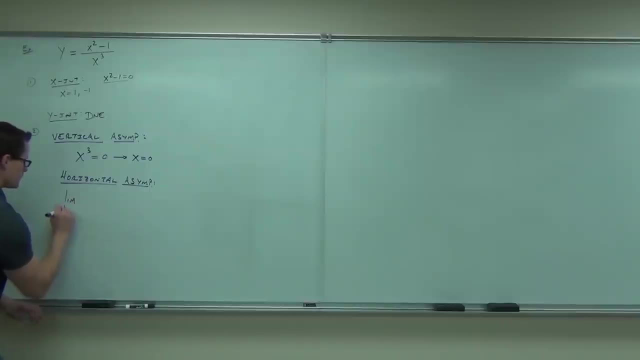 You've got to check both. Don't just assume that it's going to be the same. A lot of times it is, but we've seen cases where you have different horizontal asymptotes. Okay, So you're going to be able to take a limit. 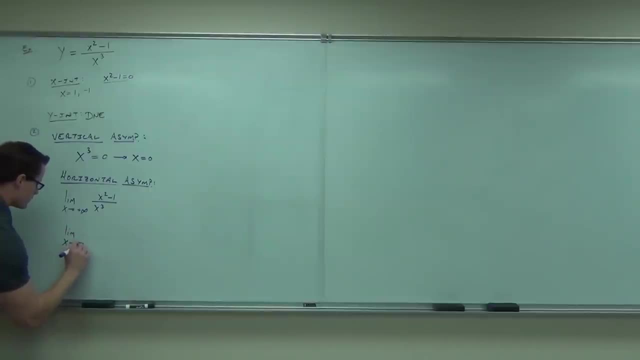 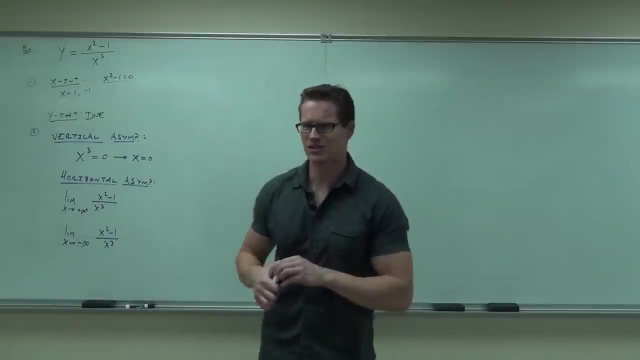 Do you know how to take limits of that stuff? I think that's what your homework is on, right. How do you take a limit as we approach positive infinity or negative infinity? Don't mumble it, Say it. Divide by the highest value in the box. 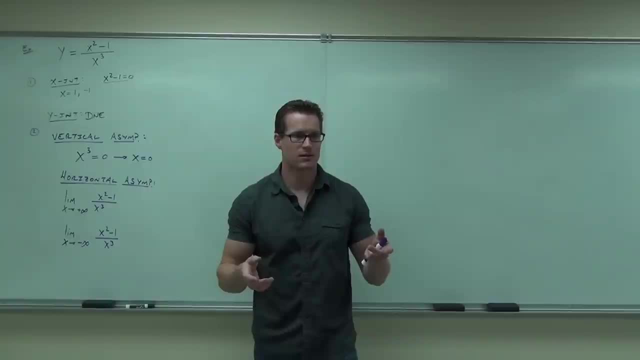 Okay, No, I'll do it. I'll do it Divided by the highest power of the denominator. Very good, In the key word Denominator, not numerator Denominator. So we would be divided by x cubed both here and here. 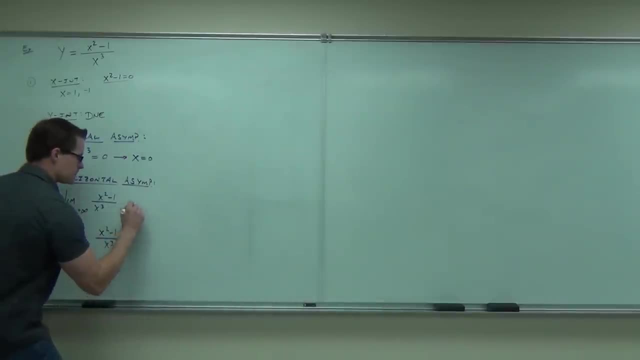 If we did that, it's going to look identical to this. You'll get x squared over x cubed, minus 1 over x cubed, all over x cubed over x cubed. Can you see that this is going to go to 0?? 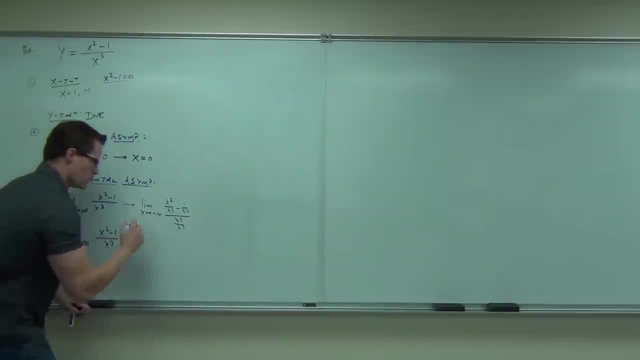 No, Yes, no, No. If you want the rest of it, here it is. I'm just going to do this one right here. You got 1 over x minus 1 over x, cubed all over 1. True. 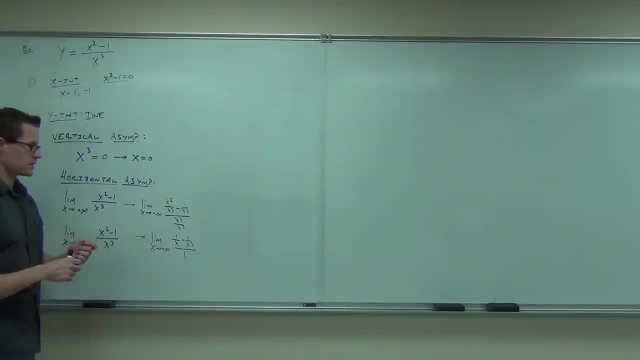 1 over x. 1 over x, cubed 1.. Tell me something, ladies and gentlemen. You need to know this: When x goes to infinity, what's this do? It goes to 0. What's this do? 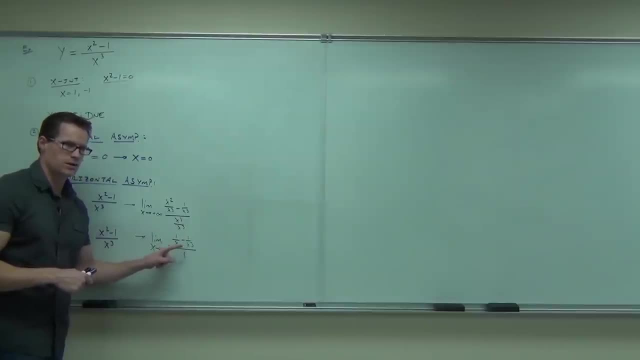 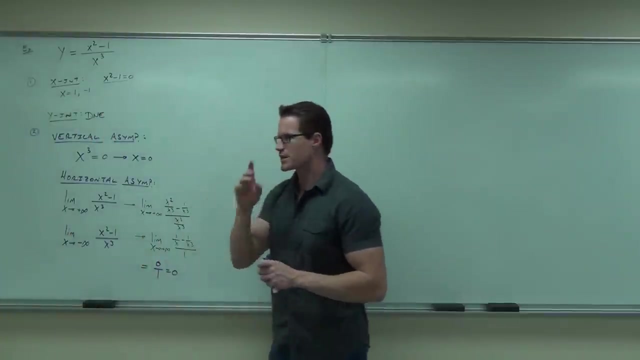 0.. What's this do? Stays at 1.. Stays at 1.. That's 0 over 1.. That's 0.. Now just think through it. think through it. Is there going to be a difference if we go to negative infinity? 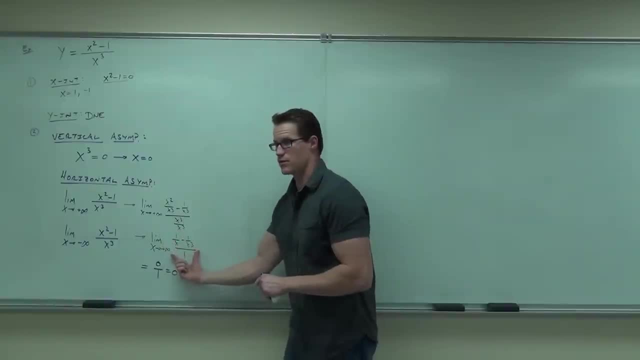 This would still work, right. You'd still do that. You'd still have exactly this thing. You follow me. Now take it to negative infinity. What's 1 over negative infinity? We'd be over here right now. What's 1 over negative infinity? 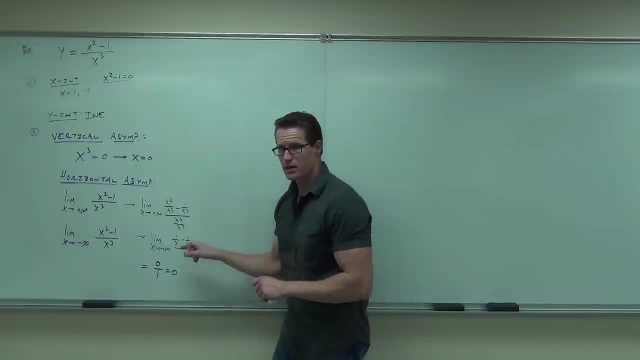 It's still 0.. What's 1 over negative infinity? It's still 0.. This would still be 0, and that's still a positive 1, because you're dividing x cubed by x cubed. No matter what it is that's going to be a positive number. 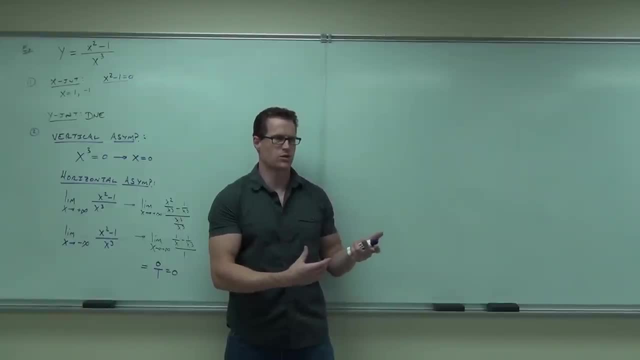 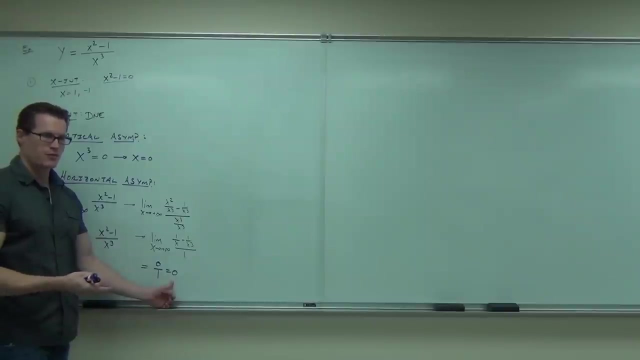 A positive 1.. You follow me on that, You sure? Yes, no, Yes, I see some nuts like questions. Are you okay that this is equal to 0?? Yeah, Okay, Now if it was going to negative infinity. so let me just change the problem here. 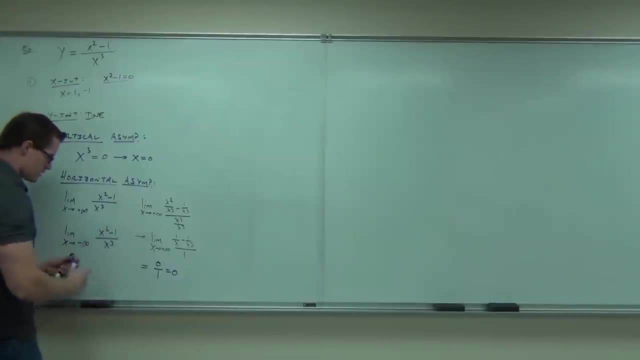 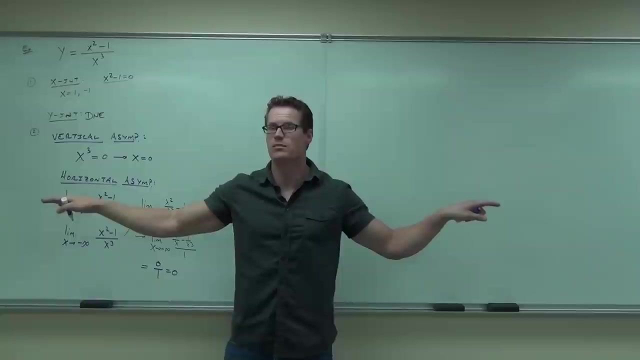 Now let's say ah, Ah-ha, ah-ha. does anything change? Is it still 0?? So where are our horizontal asymptotes? Zero, Zero, Both left and right, Both left and right. So horizontal asymptotes occur at y equals 0, both positive and negative infinity. 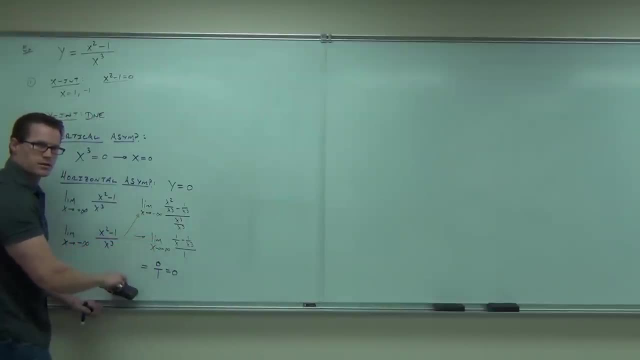 Would you mind if I erased this? Do you need it? So I can't see it. So I've taught you how to do the limits. You do the limits. Also, you're going to hate me for just telling you this. 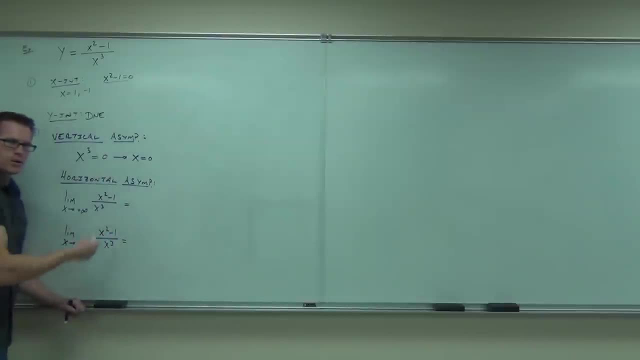 but you can see it just by looking at the limit. Where's the power bigger- top or bottom Bottom? That's something over infinity, right, That's going to be 0.. Where's the power bigger, top or bottom Bottom? 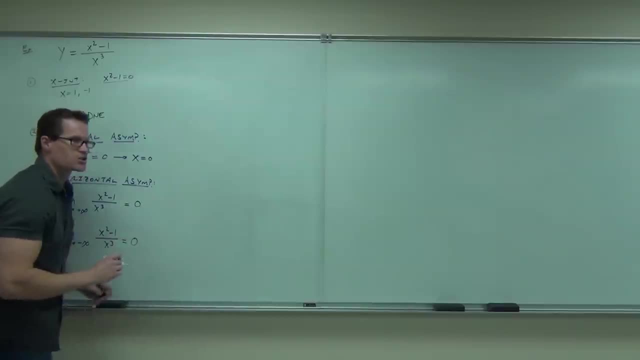 That's something over infinity. That's going to be 0.. However, you want to, if I want you to show it, Yeah, I want you to show it. yeah, But at least you can check your work really quick, right. 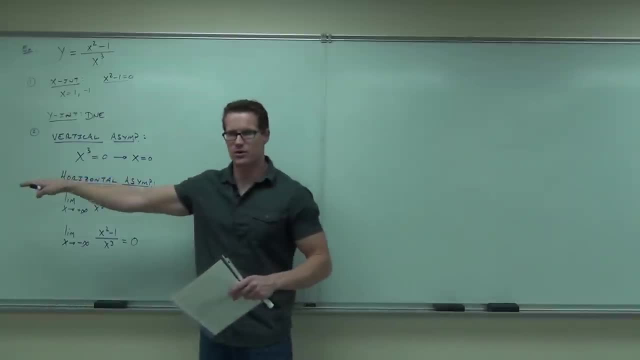 So this means, as we're going to the right, we're going to 0.. Let's go to the left, we're going to 0.. How many of you feel okay with what we've done so far? Any calculus, Not really just limits? 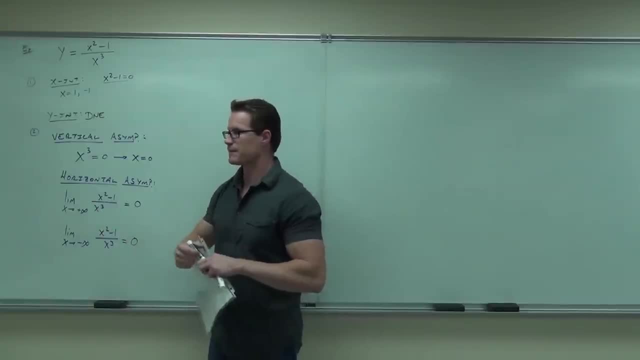 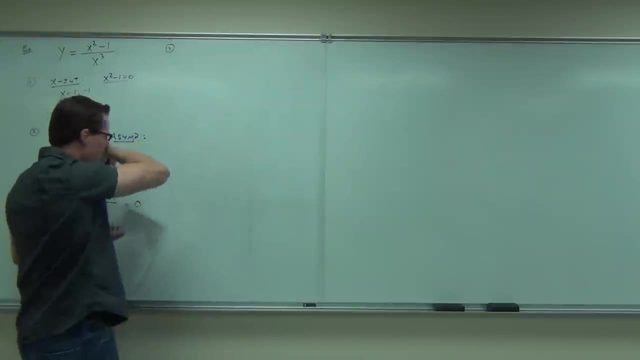 Let's start doing our step number 3.. What's step number 3?? Let's do our first derivative test Now. I know you all know how to take the first derivative, so I'm going to start doing these first derivatives a little bit quicker. 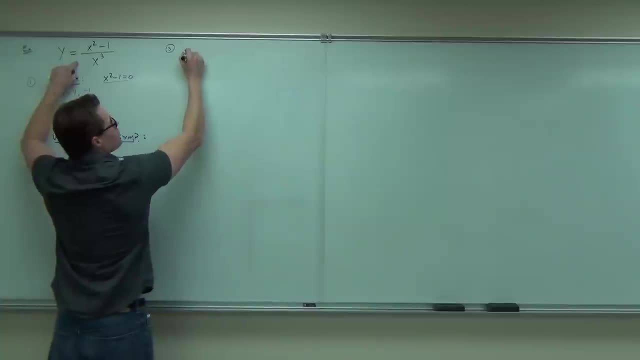 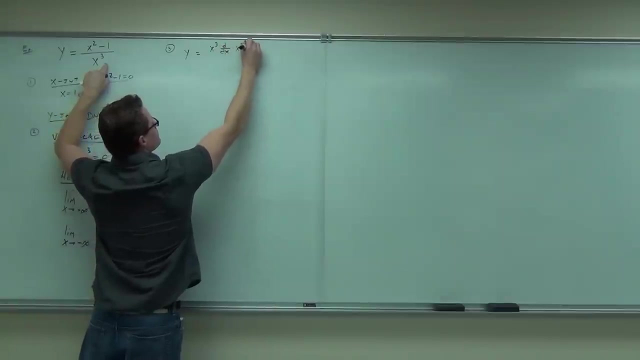 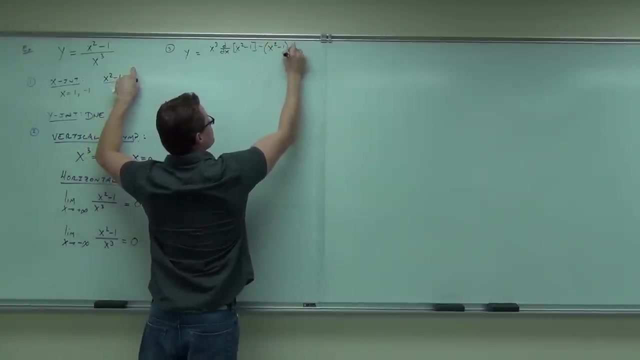 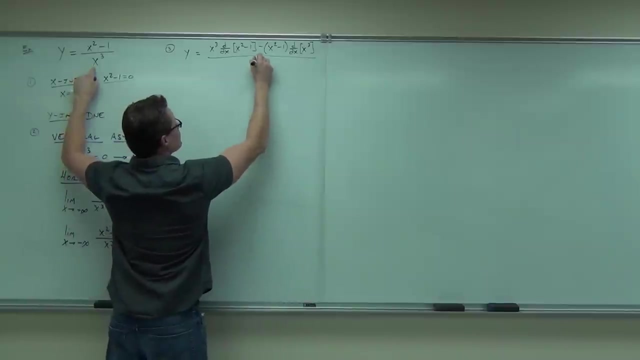 Just stick with me on these derivatives. What you would do. take your quotient rule and you're going to have this minus this. All over that squared Still okay so far. I guess you ought to show the work if you really want me to. 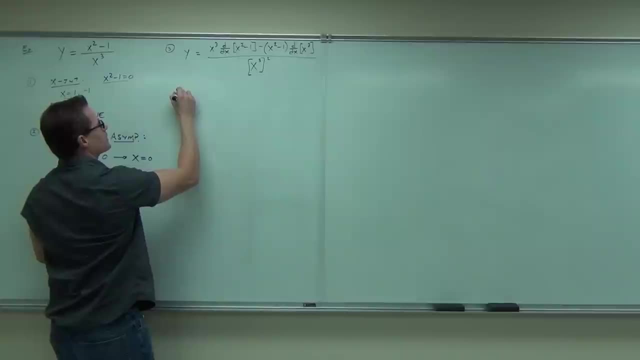 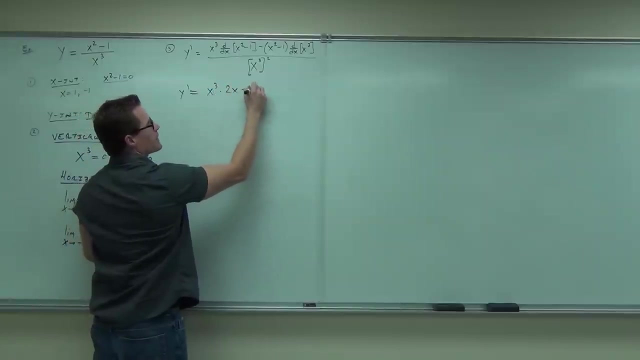 Low d high, minus high d low, square the bottom and we're okay to go X cubed times 2x minus x squared minus 1 times 3x, squared all over x to the sixth. Yes, no, Okay, so basic derivatives actually. 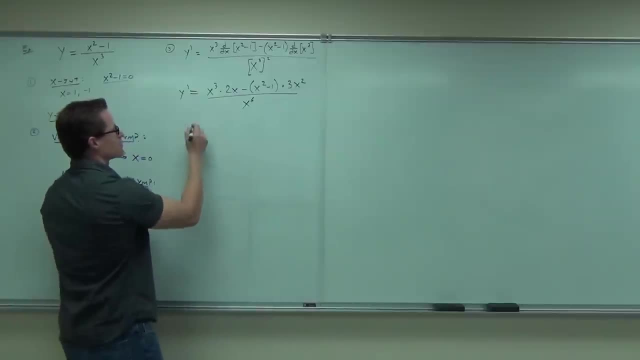 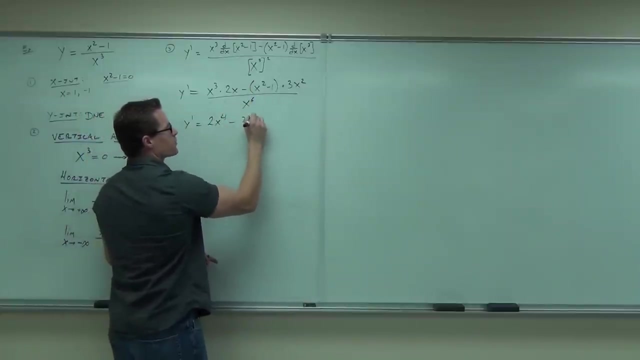 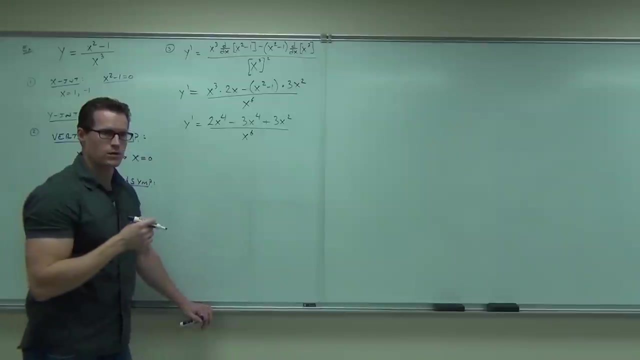 What you do with them later. kind of sucks. but basic derivatives. so far: Y prime equals 2x to the fourth, minus 3x to the fourth, plus 3x squared over x to the sixth. So far, so good. Distribute deal with those signs. 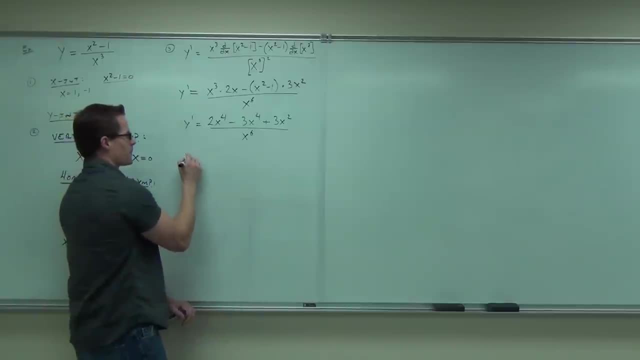 You see where the plus is coming from. I hope Y prime equals negative x to the fourth plus 3x squared all over x to the sixth. Can you keep going? Can you factor simplify? Yes, Factor out an x squared. 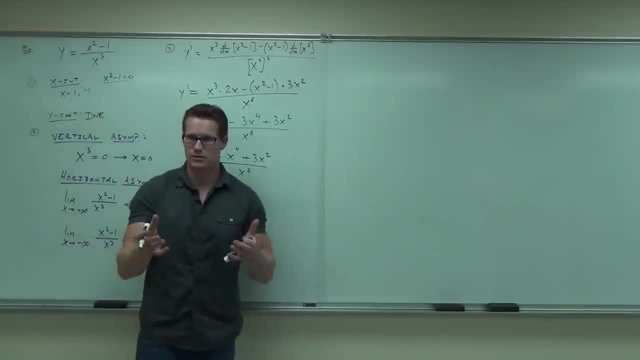 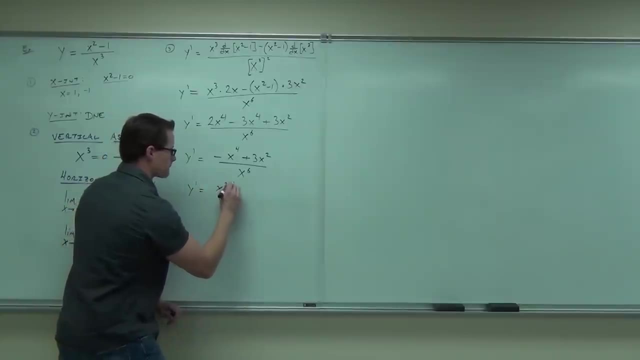 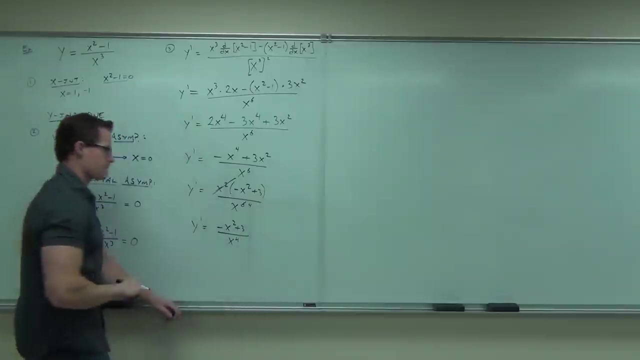 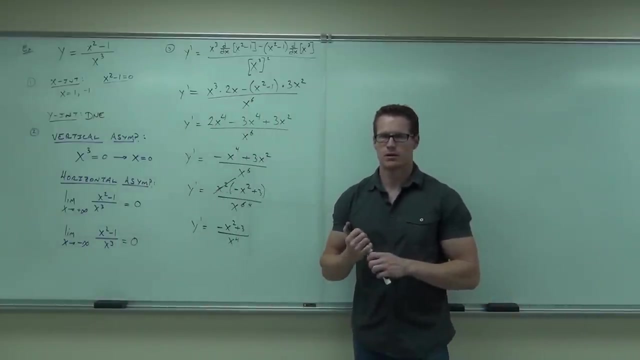 Yes, That is going to make your work later easier. Would you agree that that is your first derivative? Yes, Ladies and gentlemen, are you okay on your first derivative? I've gone kind of quickly through that, but I'm assuming that at this point, 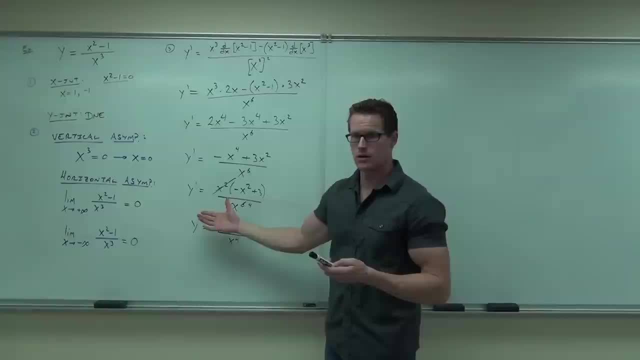 you can do a quotient rule and simplify it. You following me, Not sure if you're feeling okay with it so far. What is this? I know it's the first derivative. What is it? Increasing or decreasing? It's going to give us increasing or decreasing. 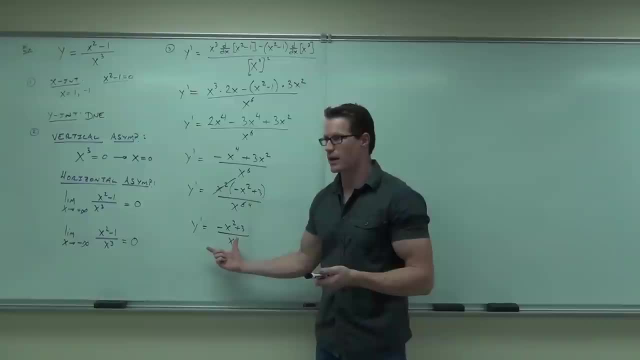 because this is a slope, And if slope is positive you're increasing. Slope is negative, you're decreasing. So if slope is zero, you have a potential relative maximum in You following me. So what we're going to do for the first derivative test? 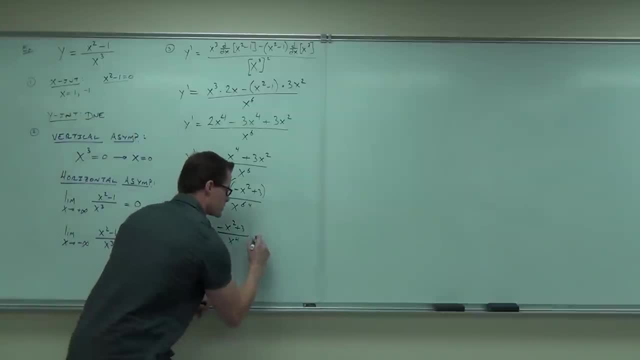 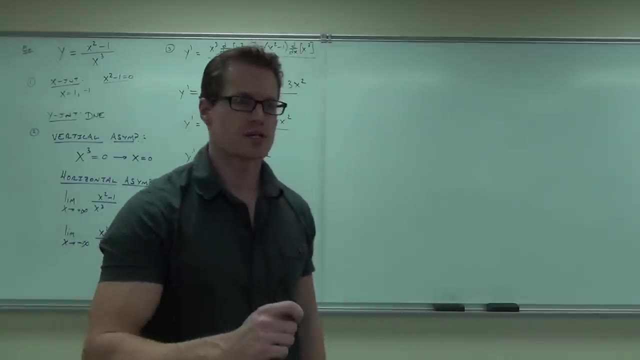 is you go? okay. now I want to set this equal to zero, And what we're going to do on this is pick out all the points that are undefined and all the points that have a zero. So can you please tell me for my critical numbers? 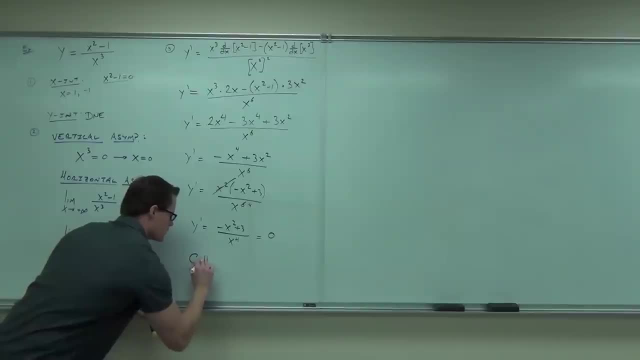 that's what we're talking about here. for critical numbers, critical numbers. the first one I see is x equals zero. Where am I getting the x equals zero, ladies and gentlemen? That tells you that right. That says x equals zero is an undefined point. 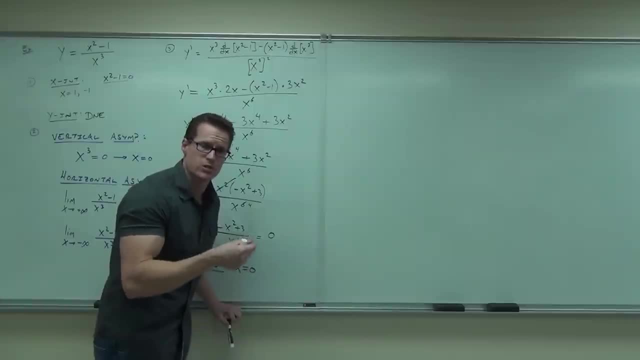 for your slope. That could mean that you're changing between increasing and decreasing. Does it have to? No, but it could. It could mean that. Do you follow that? So you have to have that x equals zero. Make sure you have where the denominator equals zero. 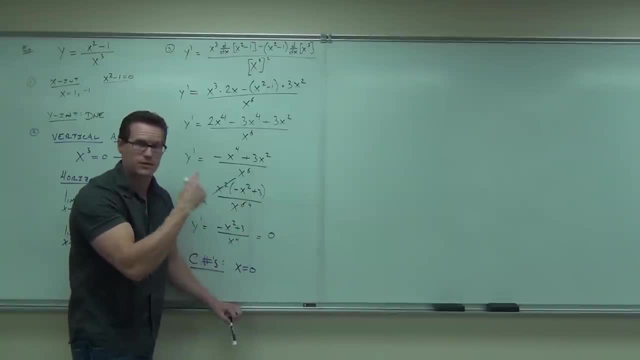 on your critical numbers and for your inflection points later. You've got to have that. Secondly, you're going to set the numerator equal to zero. That's the same idea as over here. That's the same idea as over there. It's very much like finding roots. 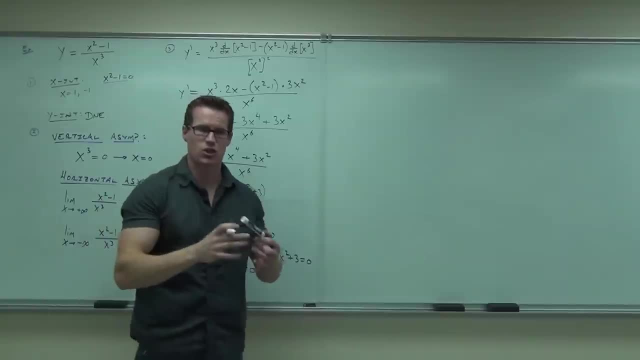 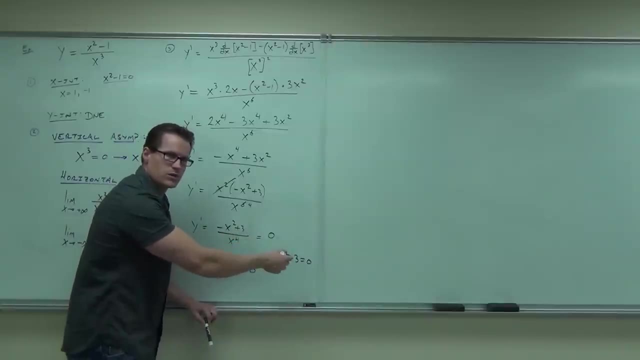 Numerator equals zero is going to give you the actual numbers. that makes your slope equal to zero. You follow me on that one. So if you want to multiply by x to the fourth, you would see the same thing, wouldn't you, Wouldn't you? 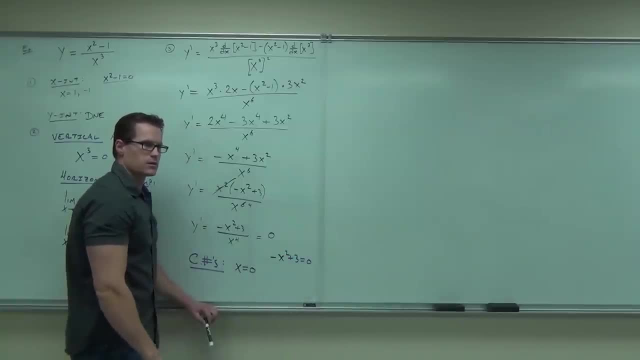 How do you solve that? Subtract x squared and then divide by the root. I would probably add x squared and then take a square root. You could subtract three, divide by negative one, take a square root. It's just more work, But you're going to get. 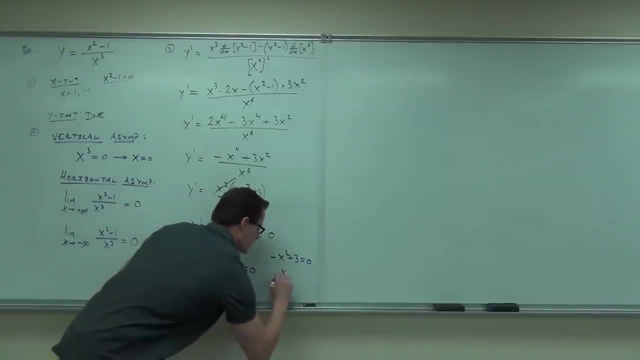 somehow you're going to get x squared equals three, True? Well, that means that more critical numbers occur at plus or minus square root of three. So I have x equals zero, x equals root three, which is why I had you take your calculators out. 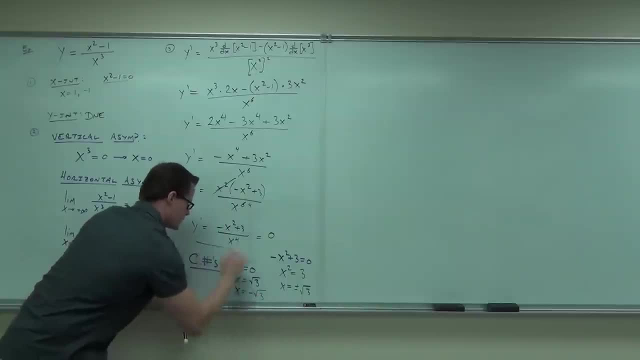 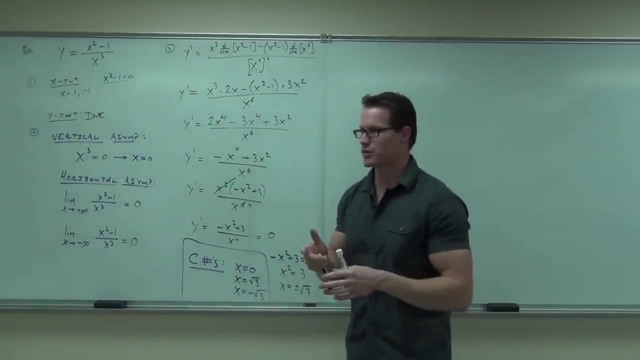 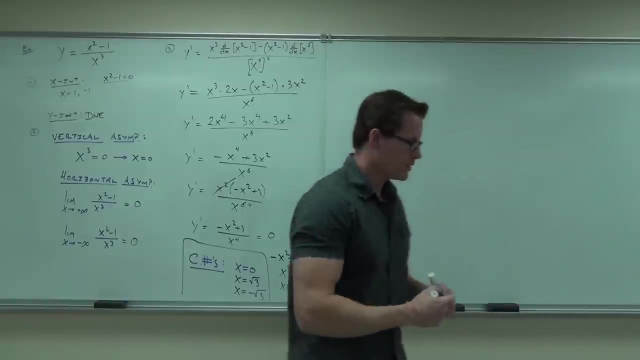 because I can't do that- and negative root three. Those are my critical numbers. What do you give to critical numbers, Yes or no? You take a square root of three, you have three, and root three 1.7 or something. 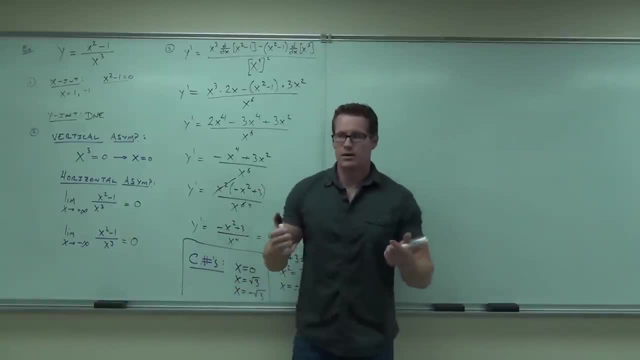 What's next Now? the reason why we simplified this as much as possible is for our second derivative. Let's go ahead. I'm going to do the second derivative. Why don't you try on your paper as well? see if we can match up with the right answers. 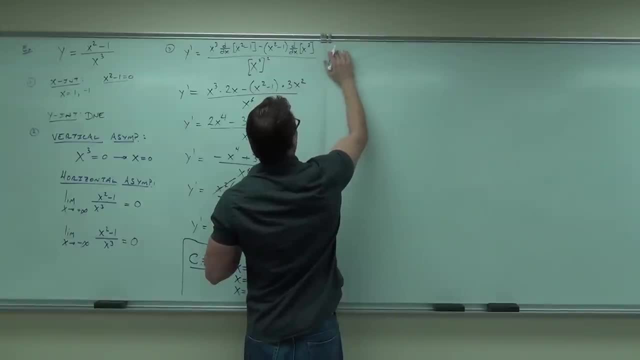 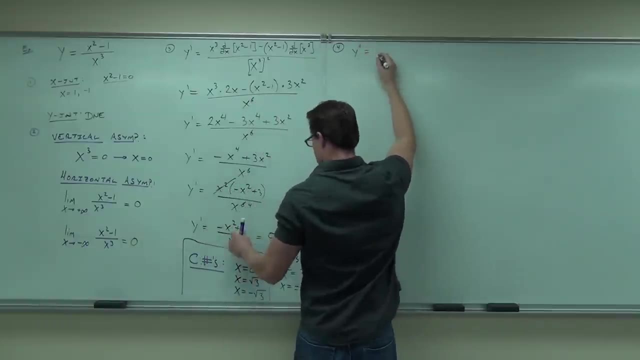 So set number three- sorry, set number four- is our second derivative. So you have two things. So this is: uh, you have to multiply the zero with one, So there's your zero plus one squared, which is negative. But what you have to do is: 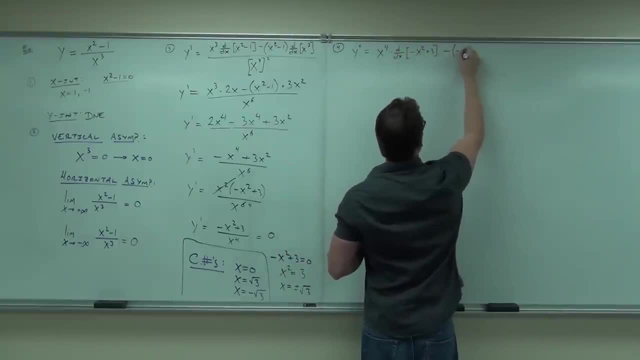 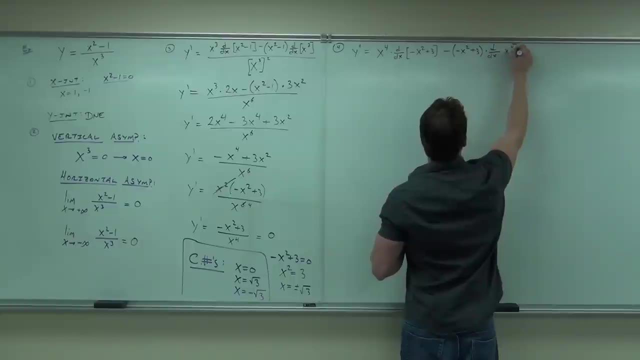 go to your reading that little bar over there, put that there and set any polar. I'll be just saying 이랑 같ig games that read 0, let's say 0, 0, 0, 0,. let's try writing another function. 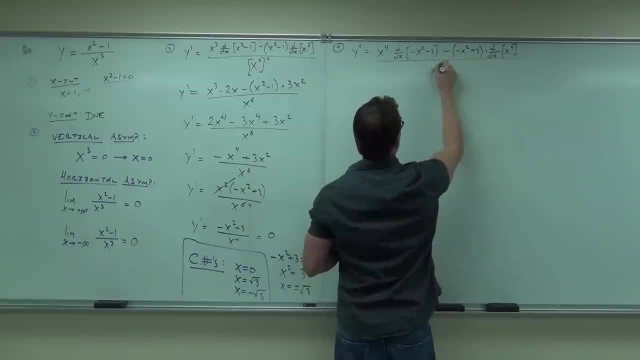 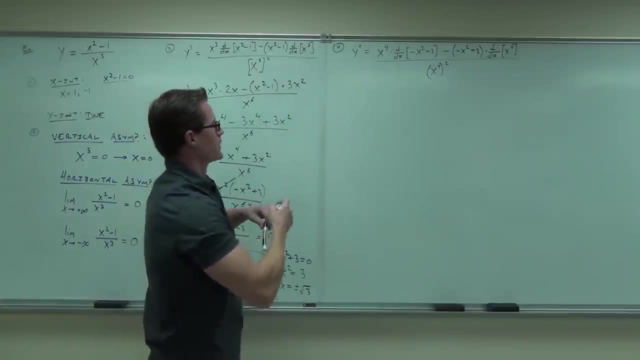 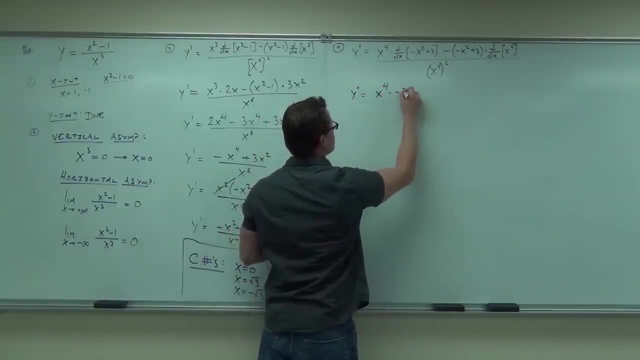 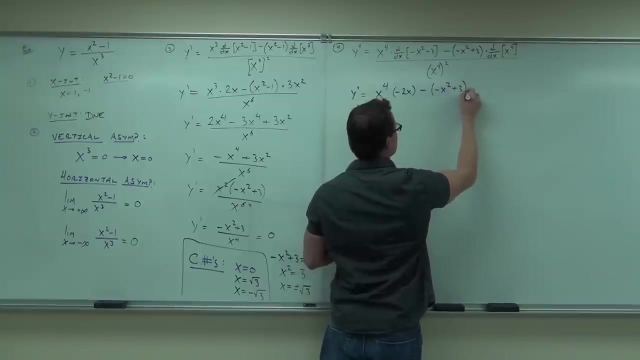 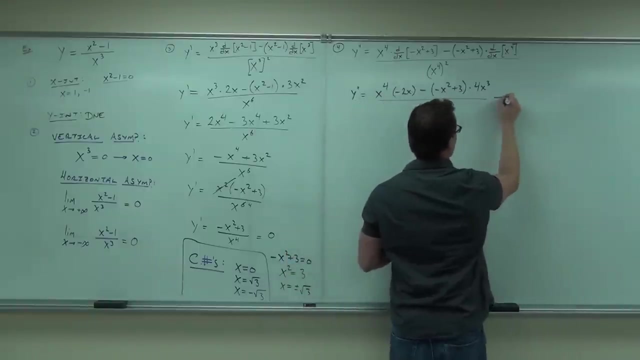 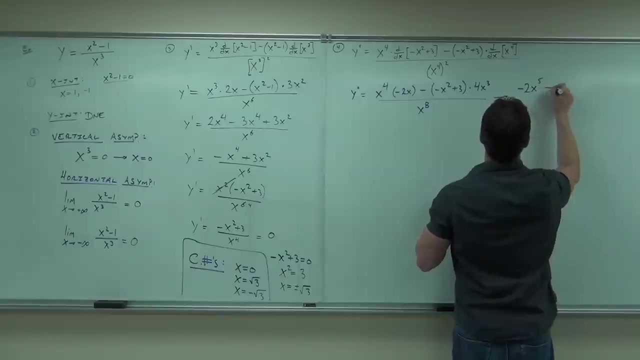 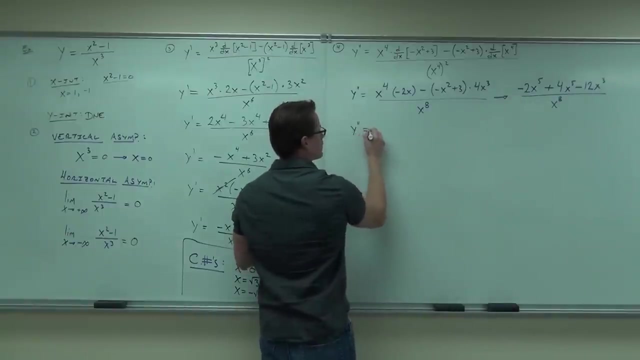 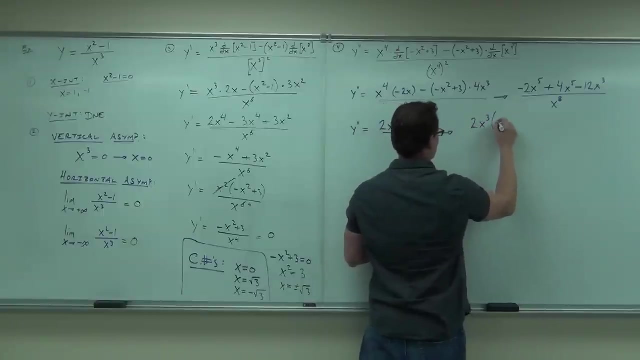 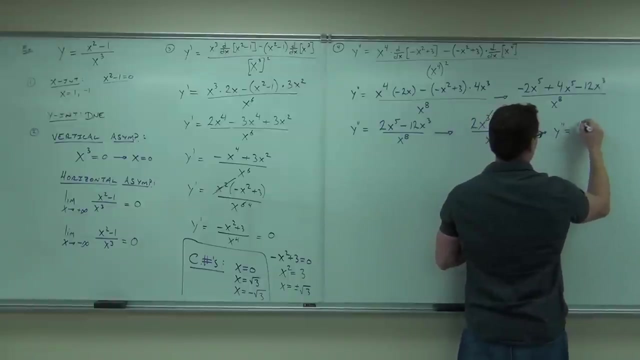 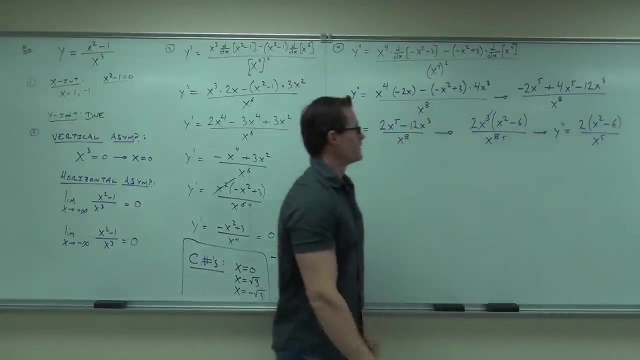 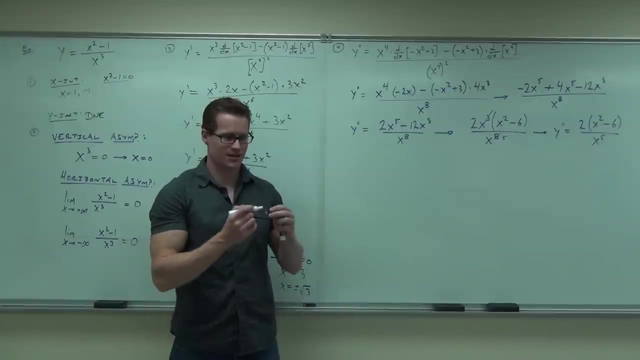 so that Y equals 5,. oh, because that's a very small LOL, Okay, Okay. Oh, that's not as bad as you thought. huh, Hopefully not as bad as you thought. Did you get that one? If you're still going, still go. 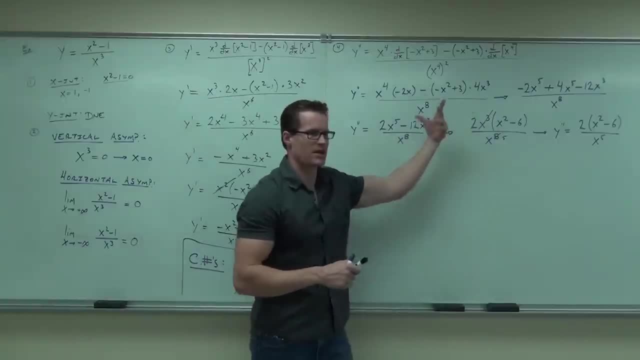 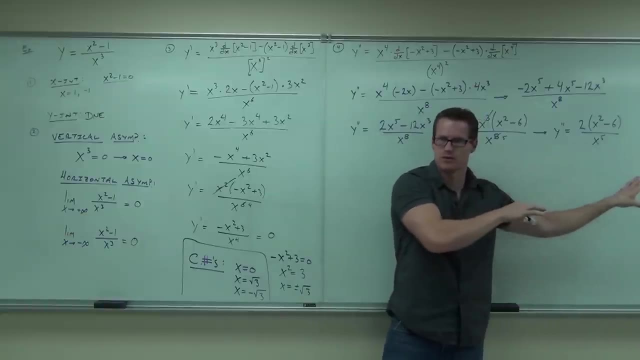 That's fine. Distribute, combine like terms, factor, simplify. You're going to get down to that point. Let's all make it down to this point. Are you okay that that is your second derivative? You know how to do the second derivative already. 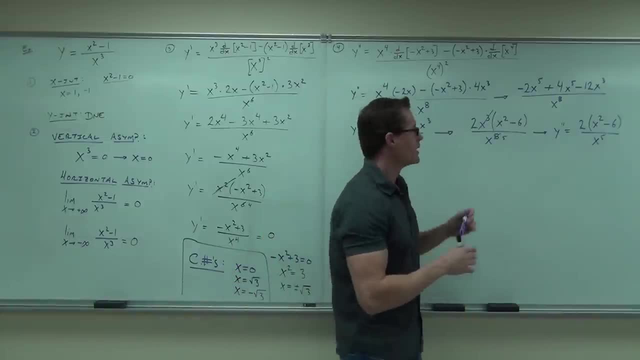 That's not the issue with this problem. okay, I know you know how to do that. Your point now is: let's find our possible inflection points or the numbers where we are going to change concavity. Can you tell me from here the numbers where I'm going to change concavity? 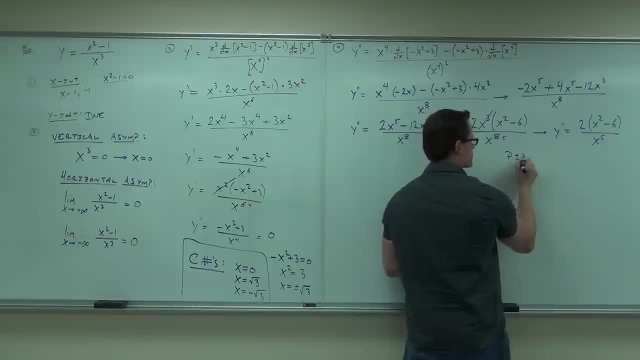 Okay, I'll tell you one of them. So possible inflection points. I'll tell you one of them. One of them is x equals 0.. How am I getting x equals 0?? Yeah, In fact, you know what? 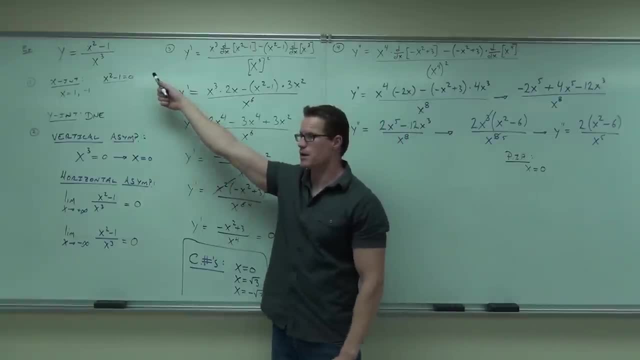 That's kind of a key point for us. That was an undefined point from the very beginning, right? If you take a quotient rule, look at that- It's going to come back again because you're just squaring it. Take a second quotient rule. 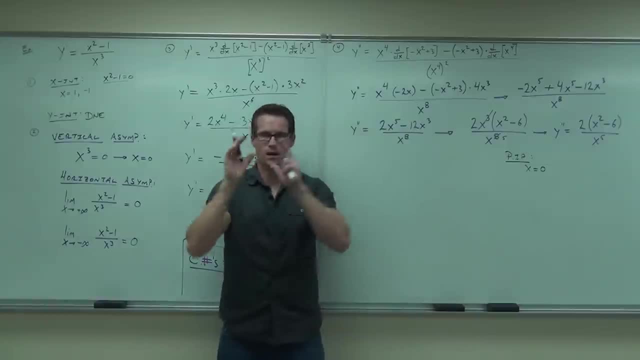 It's going to come back again because you're just squaring it. So that's going to be undefined. It's going to be a critical number. It's also going to be a possible inflection point where we change concavity. It shows up. 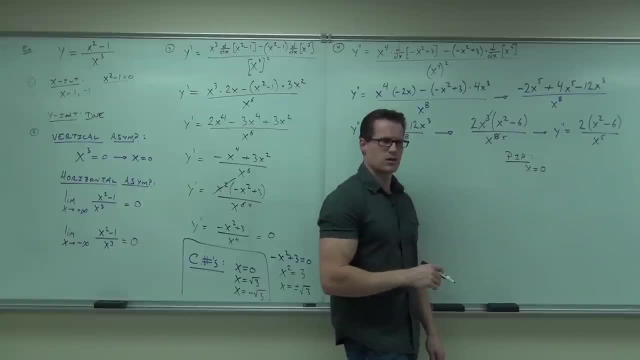 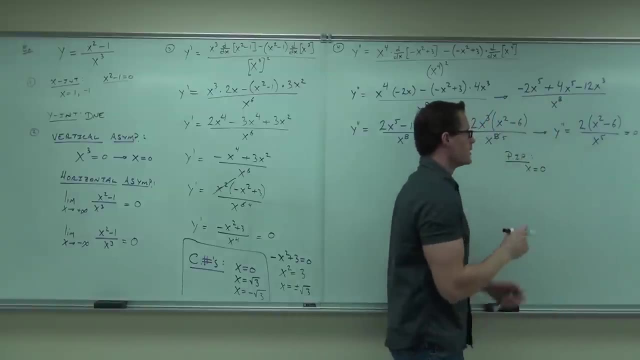 It shows up a lot in our problem. You okay with x equals 0?? Now the factoring is nice for us because it says: if you set this equal to 0,, which is what you're supposed to do- you can clear out the denominator. 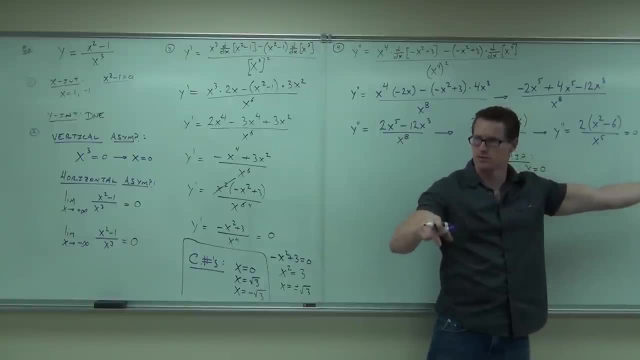 We had to include that point because it did make an undefined second derivative, so we do have to include it. the x equals 0.. But now you can say: ah, 2 times x, squared minus 6, equals 0. You set the numerator equal to 0.. 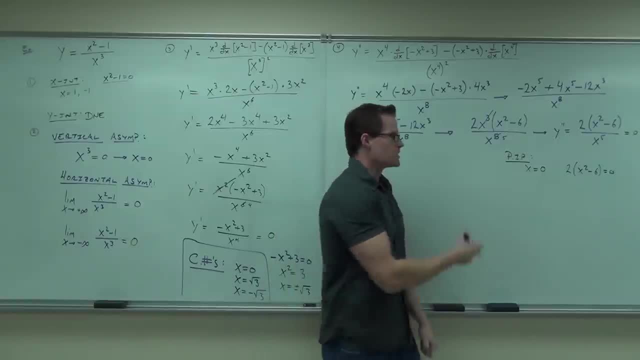 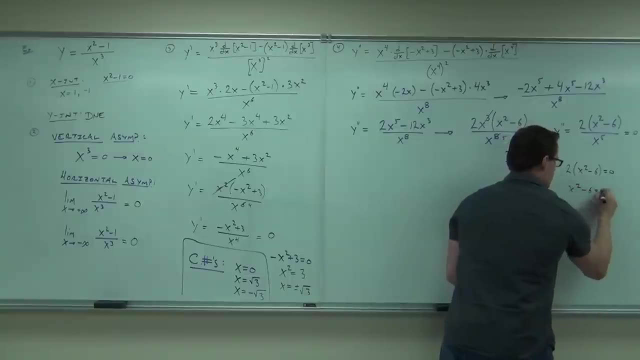 Are you with me on that one? Yes, no, Yes, Okay, But the 2,? does the 2 do anything for you? So if you divide by 2,, basically you're going to get: x squared minus 6 equals 0.. 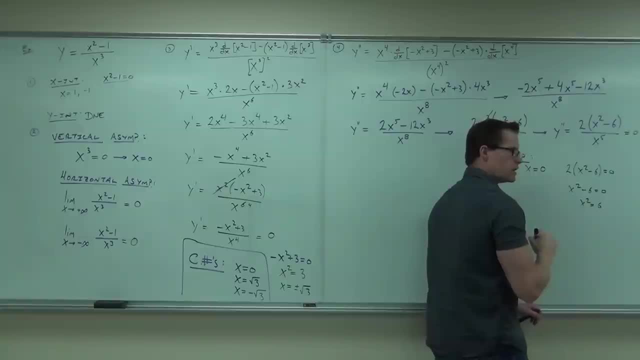 You're going to get x squared equals 6, and you're going to get Plus 1 squared, minus 6 squared. Okay, yeah, I understand Not very nice numbers. I get it, But can you find them Yeah? 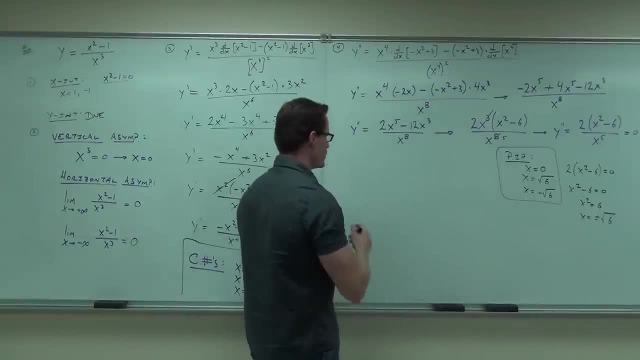 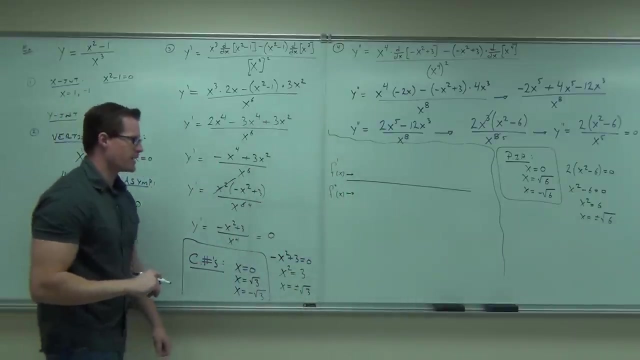 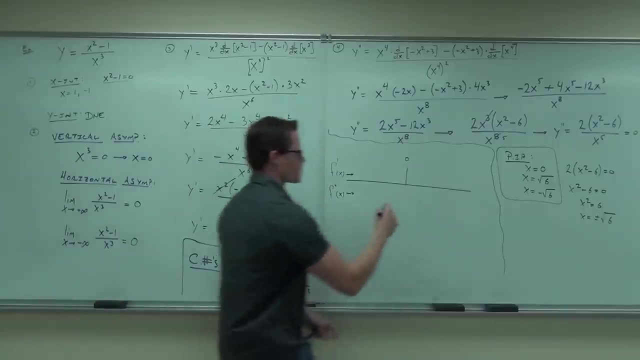 Now the point is, as soon as we do our first and our second derivative, we're going to make our table up. From our first derivative it said: you're going to have something special happening at 0.. You're also going to have something special happen at the square root of 3,. 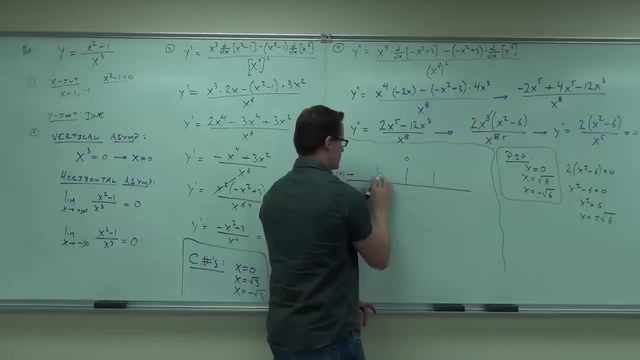 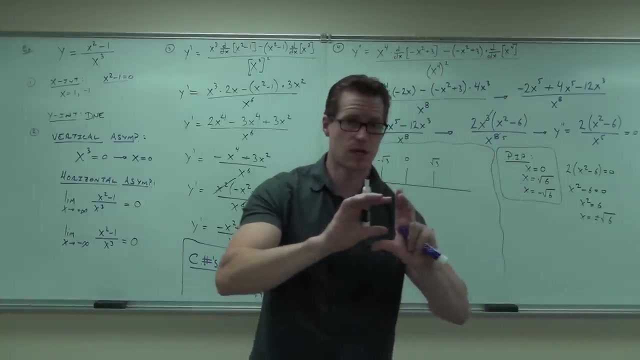 and the negative square root of 3.. Are you okay with the points that we got from the first derivative everybody? Are you all right with that Negative root 3,, 0,, 0 especially and the root 3.. Okay with that one. 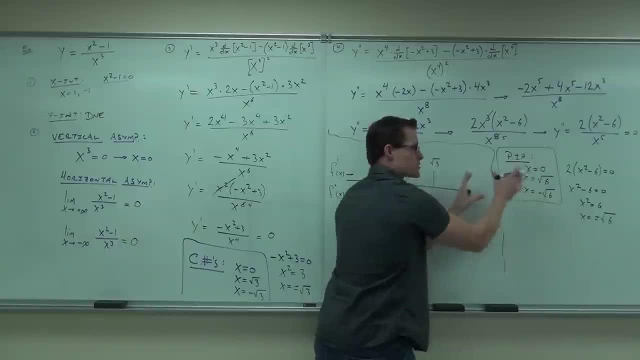 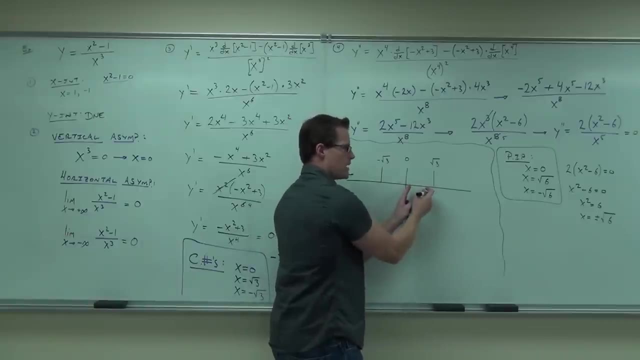 Now the next one says: okay, you still have from our posse inflection points Zero. Then you have root six, Root six to the left or to the right of root three, Three. It's actually pretty important to put this. 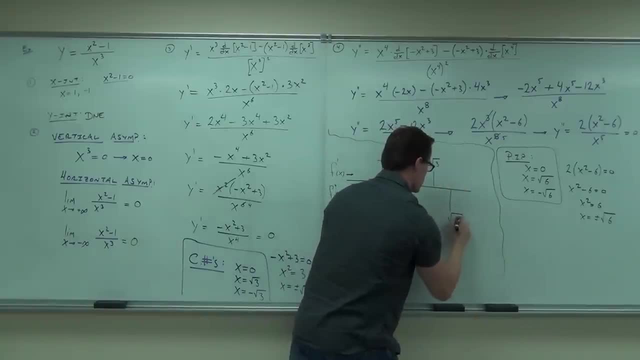 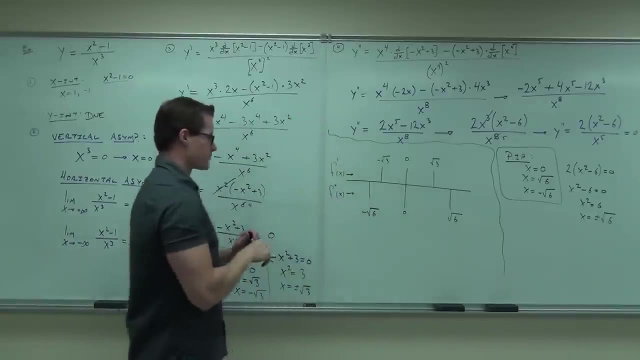 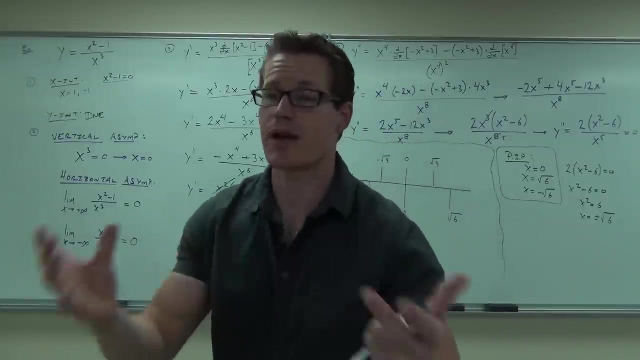 in the proper order, right? So you have to have root six over here somewhere And negative root six. Now we're gonna do what with this After you find those numbers. Are they hard to find? Not, really, not really. What do you do now? 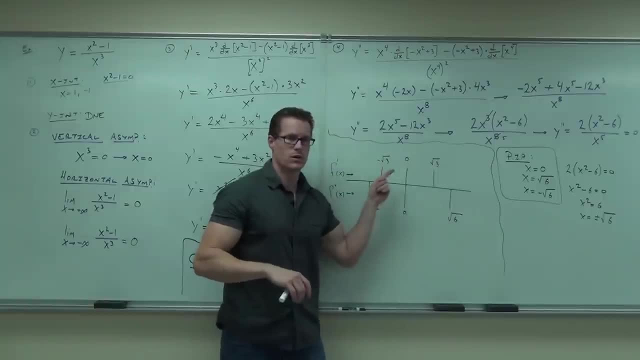 After you have the negative three, zero, root three- what do you do? Plug them into the derivatives. What wait, plug that in, That's gonna give you zero. Test them in the original function, If I plug that into the original function. 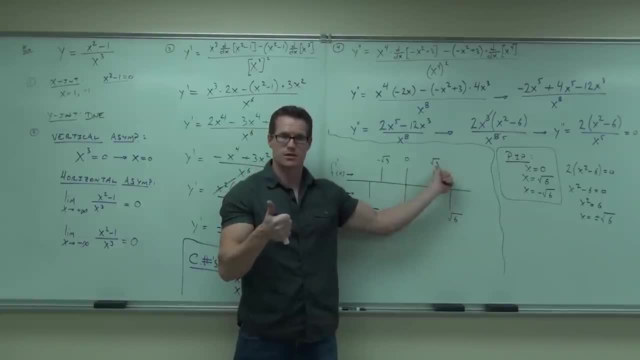 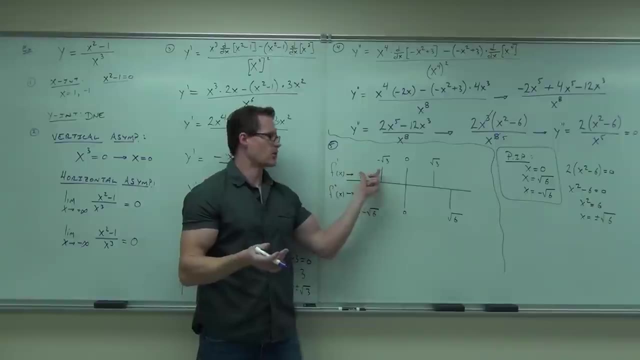 that will give me points which I'm gonna have to do in step. number six: Numbers between general intervals, Test each interval. You need to know what happens here. You need to know what happens here, here, here, here, here, here, here. 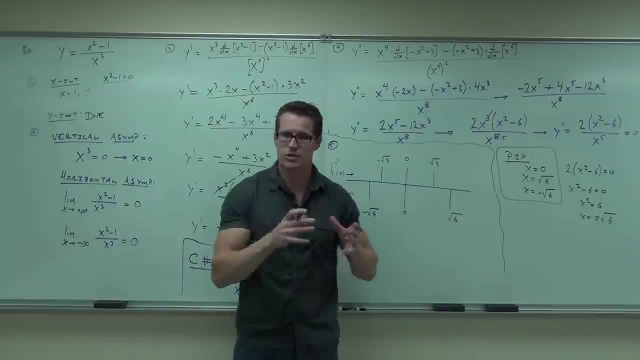 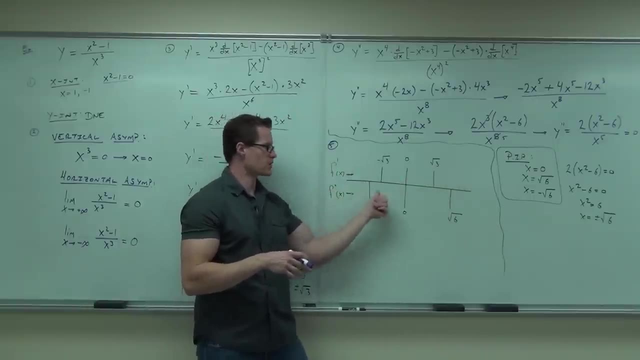 All those little intervals. right, Gotta know which area to plug them in. Negative two: Where am I gonna plug in points from all these four? Into the first derivative. That's why we have that first derivative And these are gonna go into the second derivative. 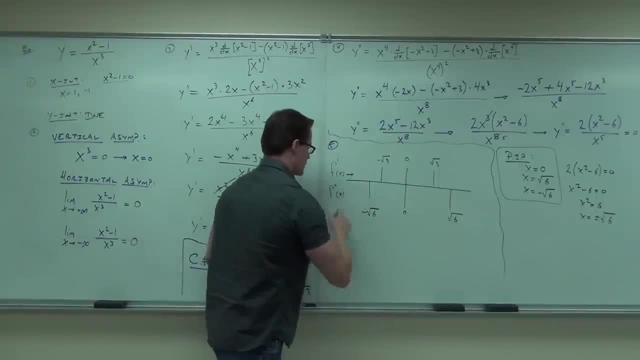 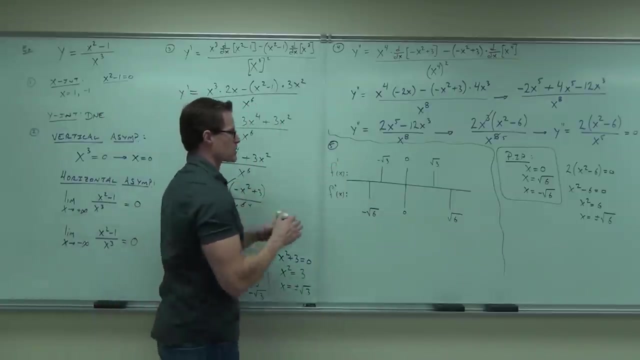 So let's go ahead and try that For this one. I'd plug in negative two. I'd plug in negative one one and positive two. We do it in the first derivative. So if I plug in negative two here, so 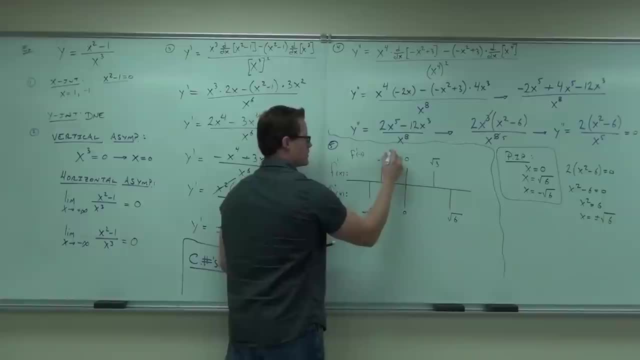 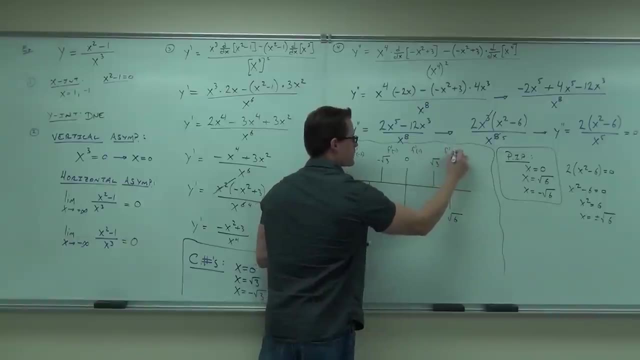 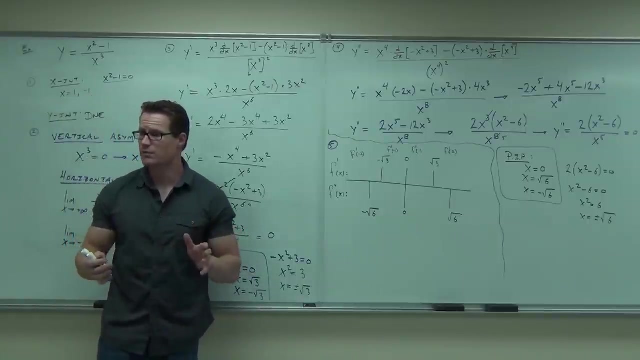 F prime of negative two. F prime of negative one. F prime of one. F prime of probably positive two. I don't really care about the actual value. all right, I really don't. I care about the sign, positive or negative. 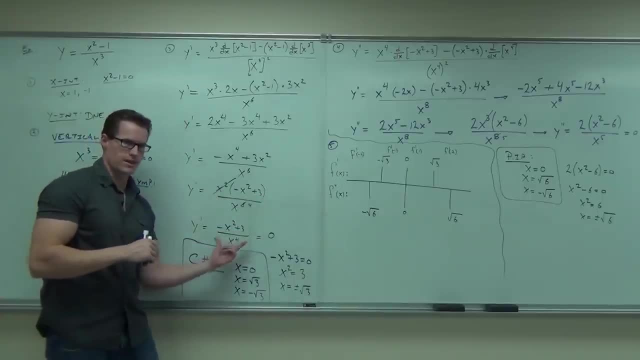 So we're gonna take negative two. Plug it into the easiest one to work with, That's this one. If I take negative two, I know I'm gonna have negative four plus three. That's a negative number over a positive number. 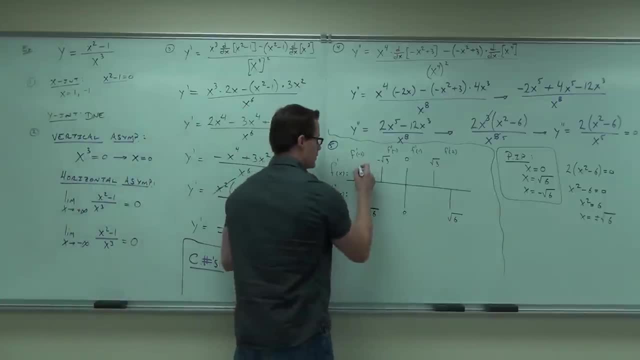 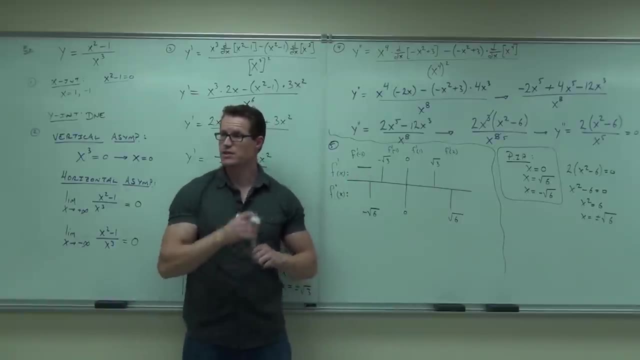 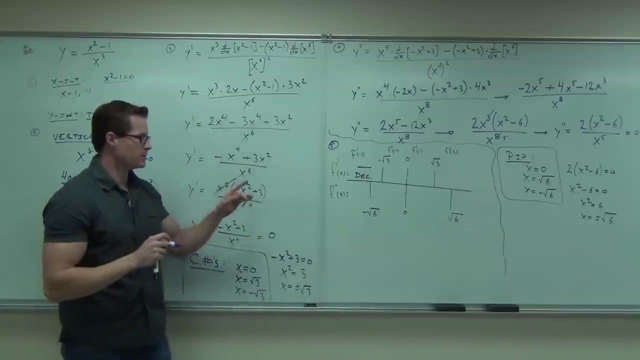 Did you get a negative as well? Yes, Negative, Hey, hey, What's negative mean in relation to this Decreasing? Decreasing very good, Because it's a slope. Negative slope means decreasing. Plug in negative one. If I do negative one, I get. 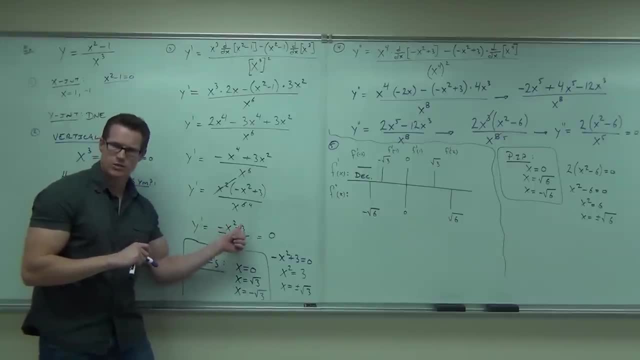 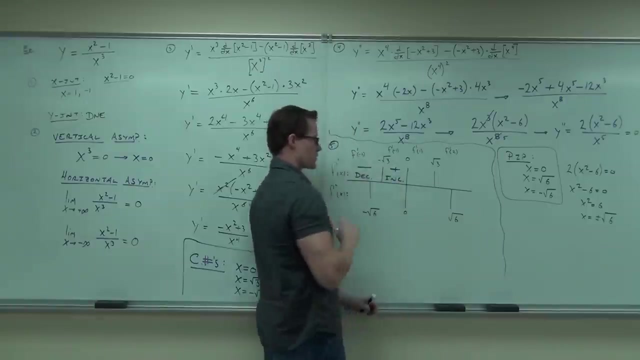 remember that you don't square this negative right. That says negative x squared, So this'll be negative. one Plus three, That's two over positive one. It's positive. What's positive mean Increasing, Increasing, Increasing, Don't just say up. 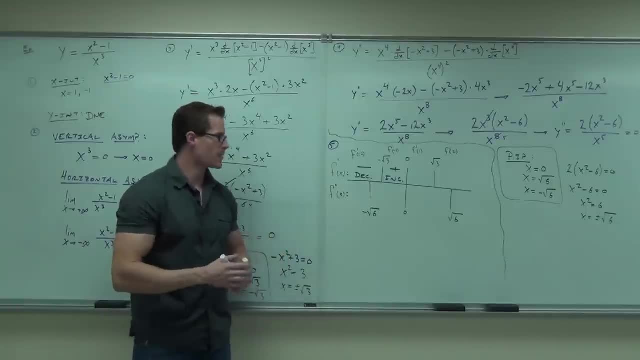 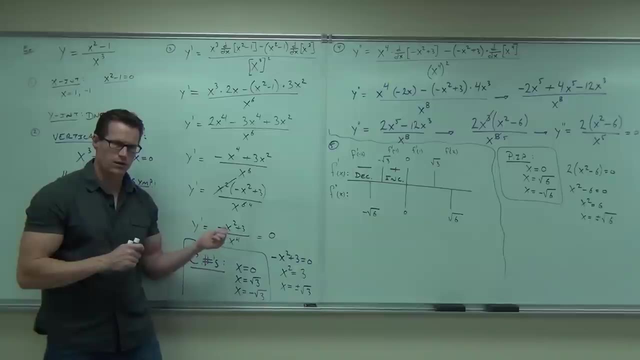 because that could be misconstrued as concave up. I wanna say increasing or decreasing. How about one? Let's try one. If I try one, do you see I'm gonna get the same exact thing as negative one, Because that says negative one plus two. 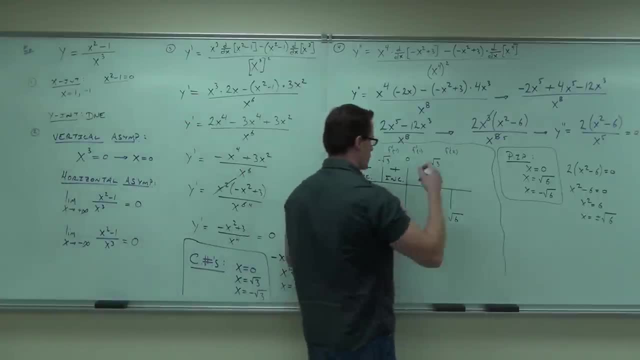 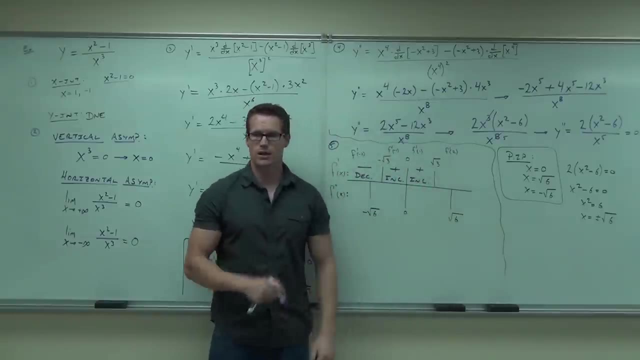 That's positive, over that's positive. So is that a relative extreme? No, This one, No, That zero actually didn't change right. We're increasing and increasing again. That's interesting. How about that? The two? 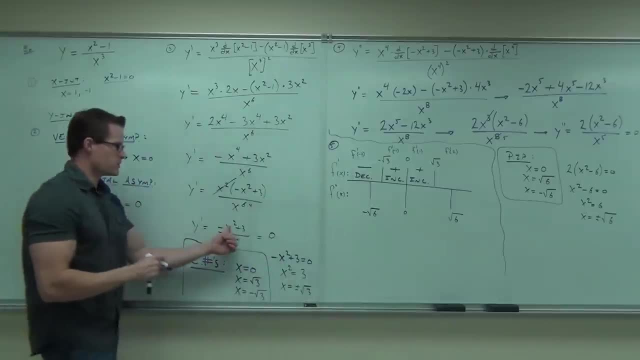 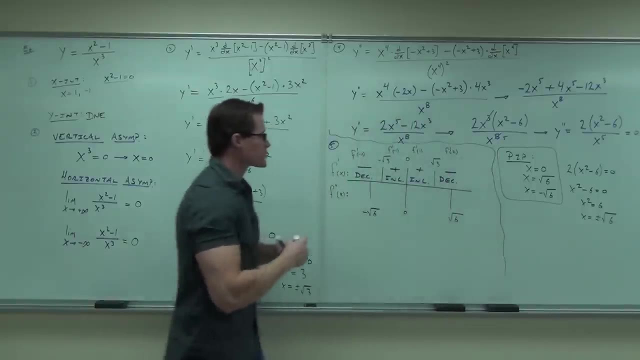 Negative, It's gonna be negative, Yeah for sure. You plug in the two, you get negative over positive. That's a negative. Now let's try our, our second derivative. If we do, for those of you who really have a hang of this, 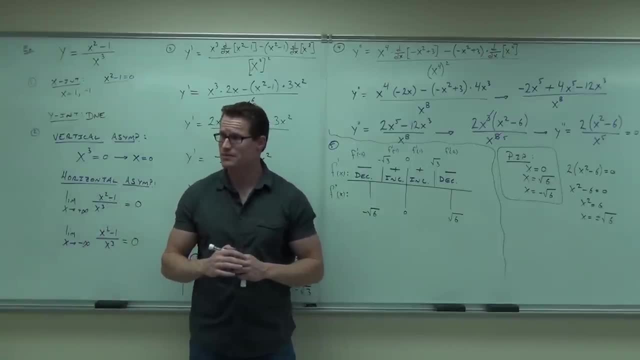 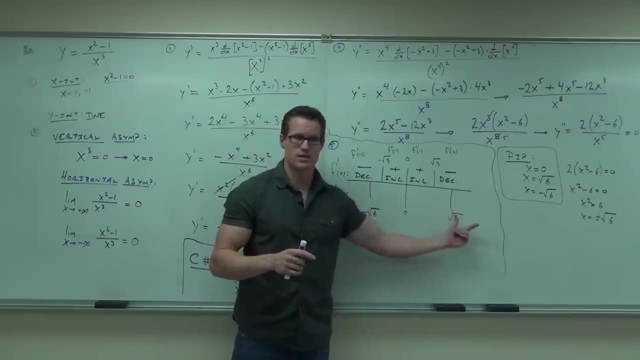 can you do me a favor right now? Can you start finding me points? I think I can pretty much take care of the zero, but I'm gonna have a hard time plugging in the square root of negative three, root three, negative root six and root six. 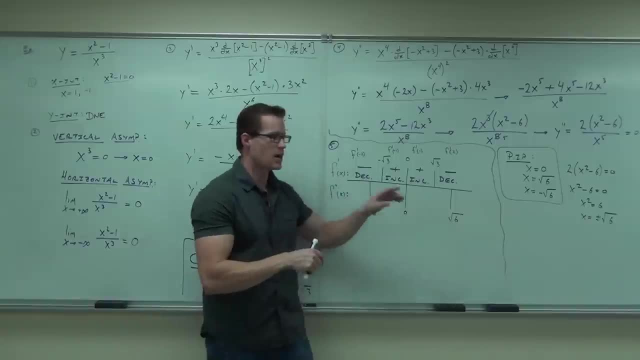 So if you wanna try this, as I'm going through the second part, if you really get to grasp this left side of the room, my left side, you guys try the root three and three, root three. You guys try the negative, root six and root six. 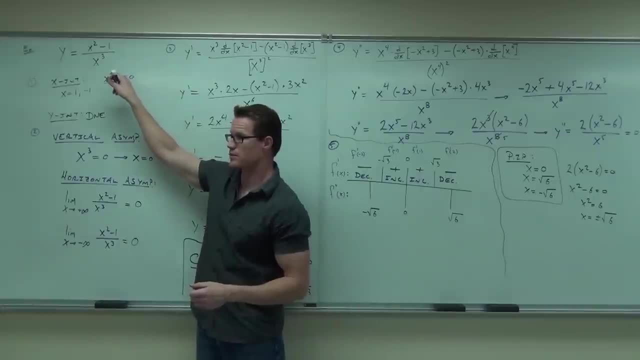 in the original original. Okay, Can you do that for me? Give me two like the first. I don't even care. the first derivative is five, 2.5 or whatever. Now for our second derivative. we're also gonna try some values in these intervals. 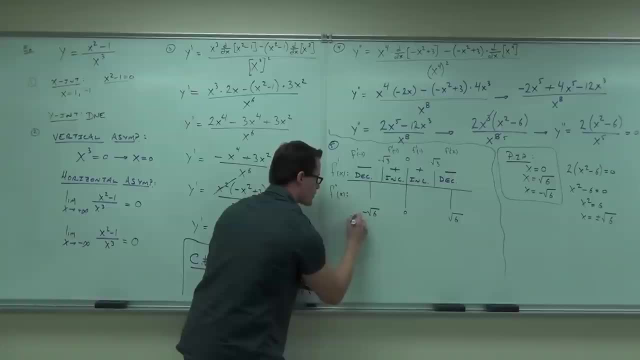 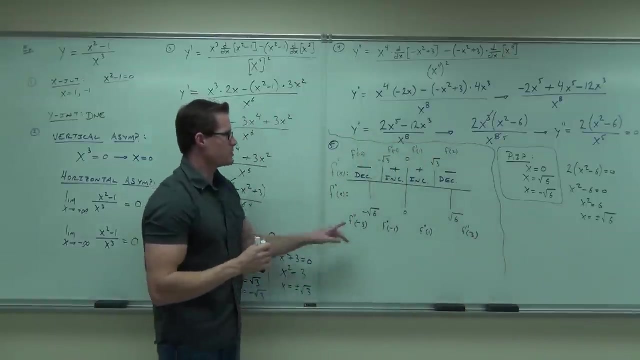 but you're gonna plug them into the second derivative. So f double prime of, that's gonna be like negative three, Double prime of negative one. Double prime of one. Double prime positive three. If I do that, if I do that, 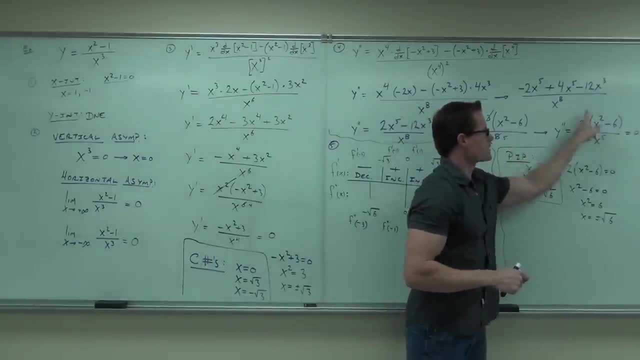 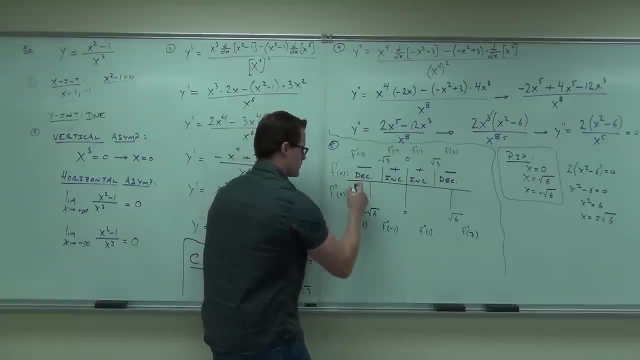 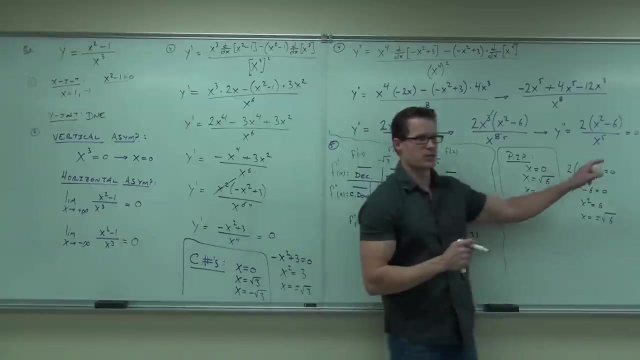 if I take the negative three over here, that's gonna be a positive over a negative. I have a negative. What's negative mean, by the way, when I'm talking about second derivative, Concave down, Concave down. If I plug in negative one, notice what we do. 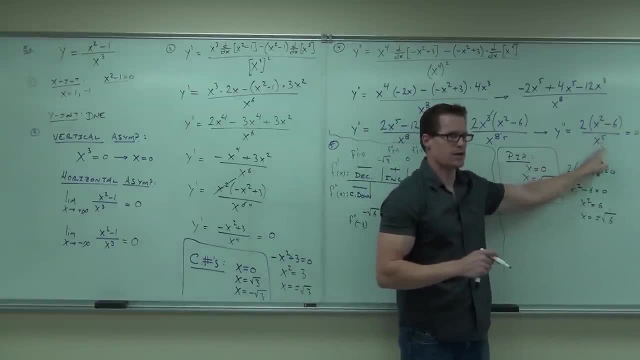 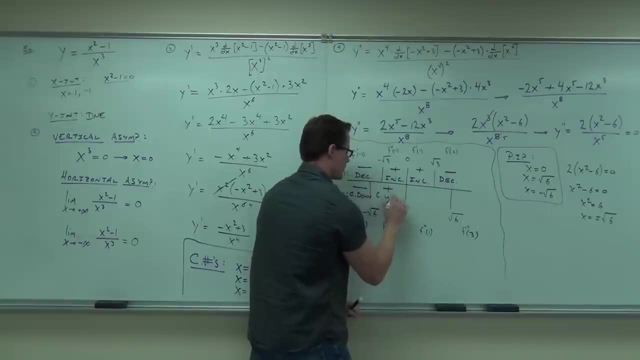 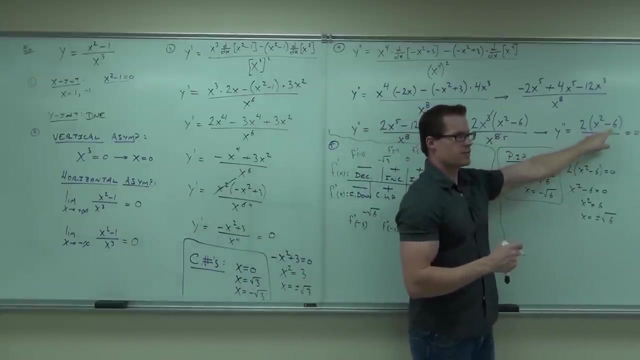 We've got one minus six. that's negative. five over a negative: That's gonna be a. that's a positive. Concave up. If I try positive one here, I'm gonna get a negative over a positive. that's gonna give me a negative. 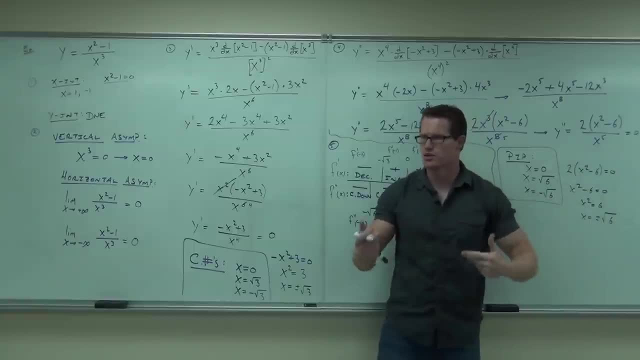 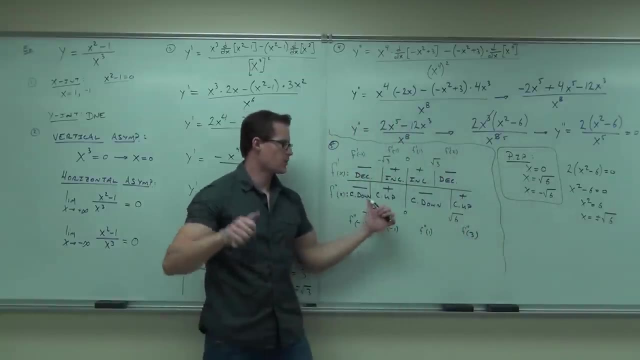 And if I try three, I have a positive over a positive. that's gonna give me a positive By a show of hands. how many people feel okay with our concavity at this point? Right row, are you guys okay with this? 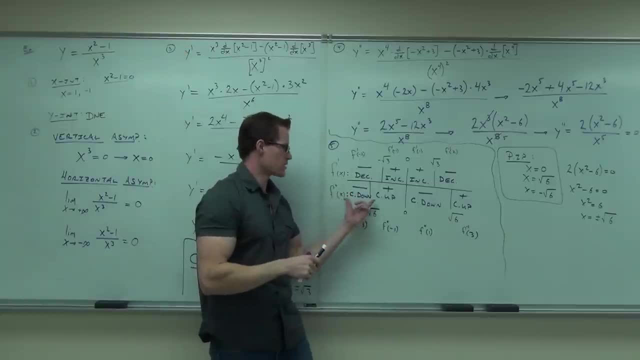 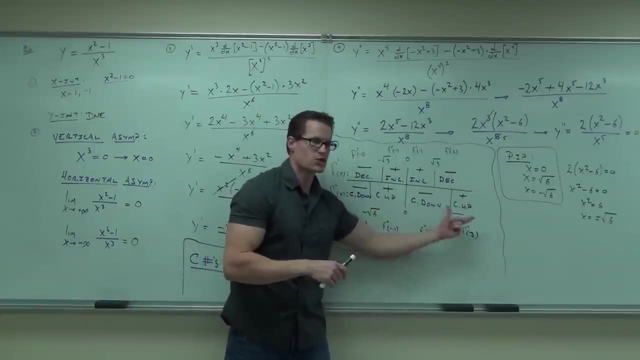 You guys over here? yes, no, So we've checked this. in the second derivative We got, this was a negative interval, positive interval. negative interval, positive interval. concave, down, up, down, up Were these inflection values. 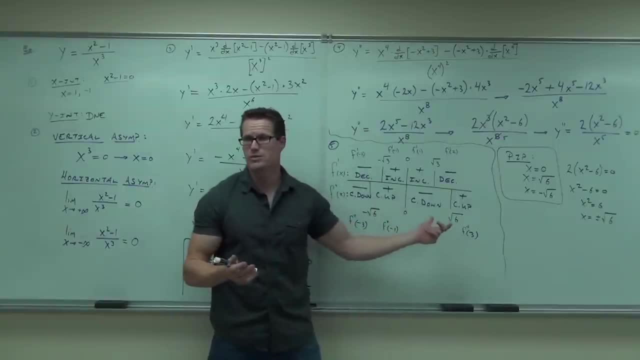 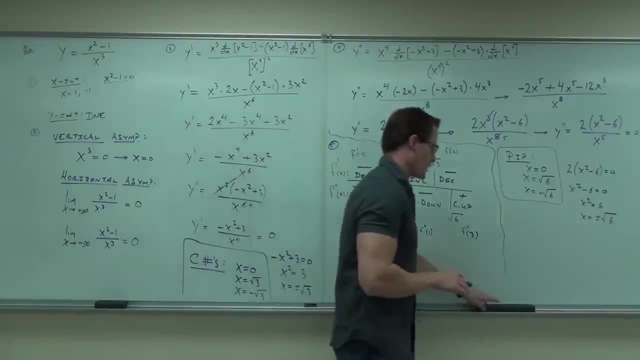 Does concavity change? here and here And all of them actually, we had different concavities. Step number six is you have to find all of them, Find all of your points. So right down here I'm gonna write my points. 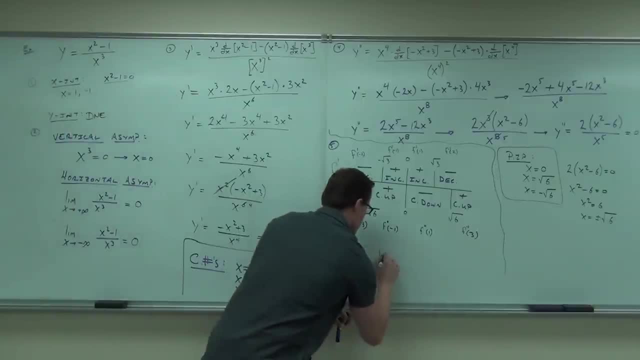 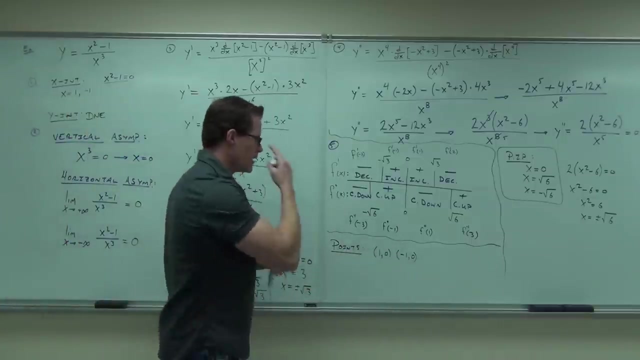 I know for my x-intercepts I'm gonna be at one zero and negative. one zero My y-intercept. I didn't have any, so that just came from my x-intercepts. Now I also have all of this junk over here. 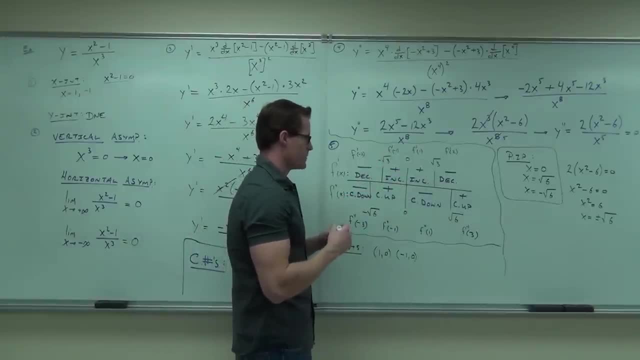 So my relative max and relative min. Can you tell me which one of these is going to give me my relative maximum? My relative maximum, Is it gonna be the negative root three or the positive root three, Positive, Positive- This one's gonna be a relative minimum. 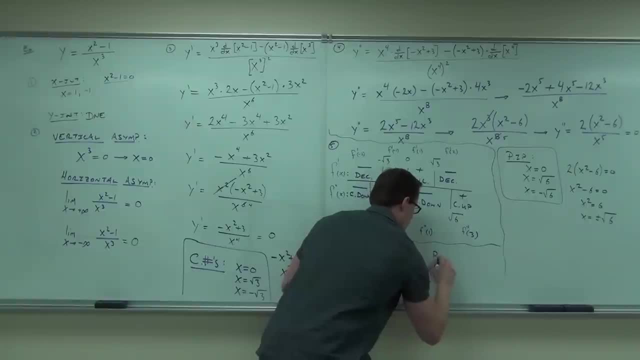 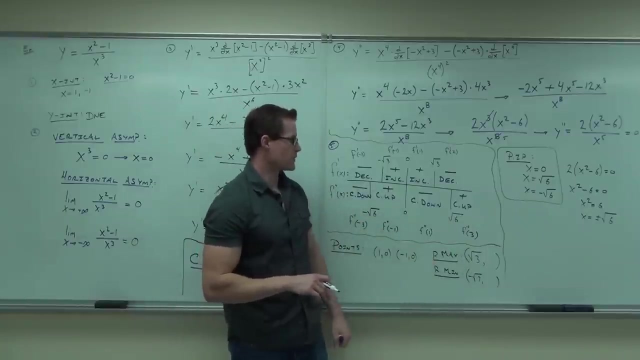 So relative max. The relative max will be at square root of three comma, something. I don't know what. it is Negative square root of three comma, something Somebody plugged in the square root of three. About how much did you get? 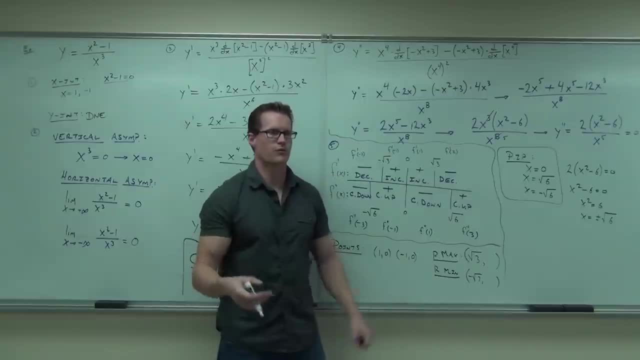 .38? .38? Yeah, Okay, so let's say .4.. Is that negative .4? Negative: .38.. Okay, Are you okay in getting those numbers? Do you remember where I'm getting these numbers from? Where do I plug in the root threes? 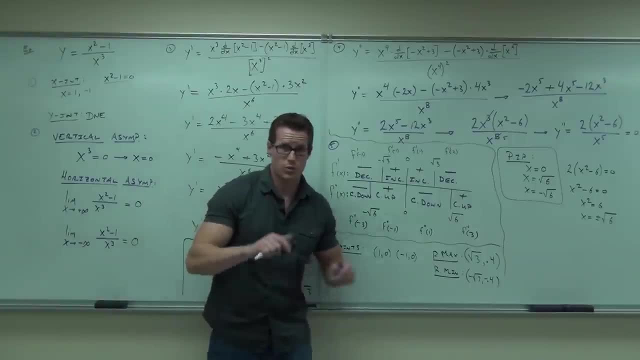 Not the first derivative, not the second, but the original function's gonna give you points, Are you okay on that? so far, Are you sure? We're almost done, Almost done. Now let's do the root sixes. The root sixes are my inflection points. 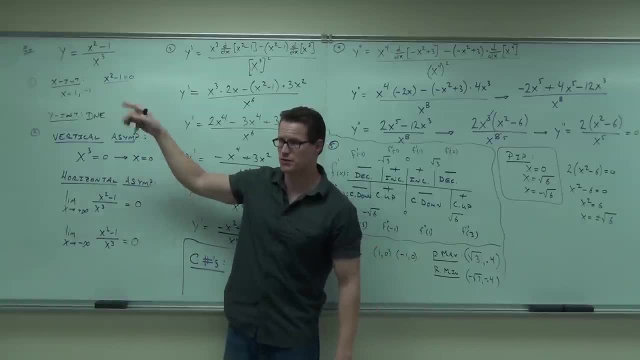 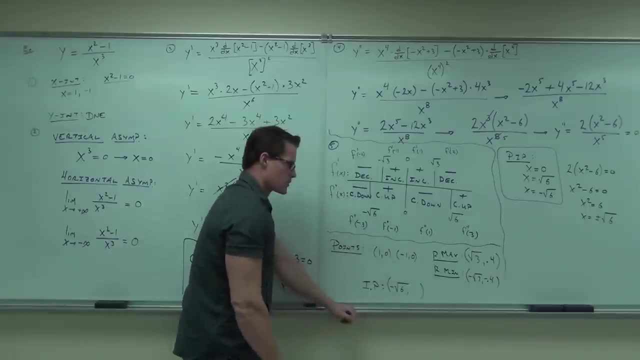 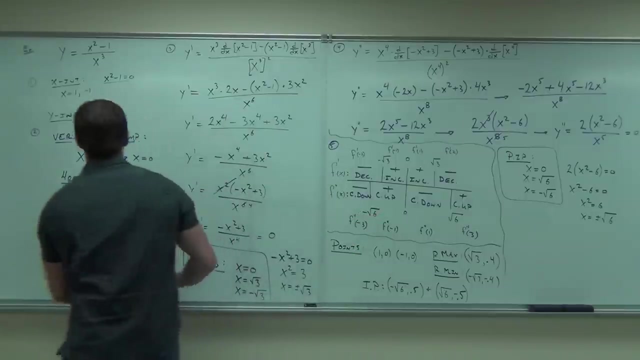 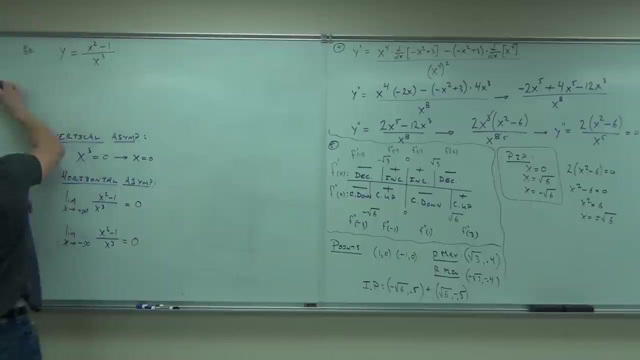 I'm going to leave the asymptotes, because I need those. 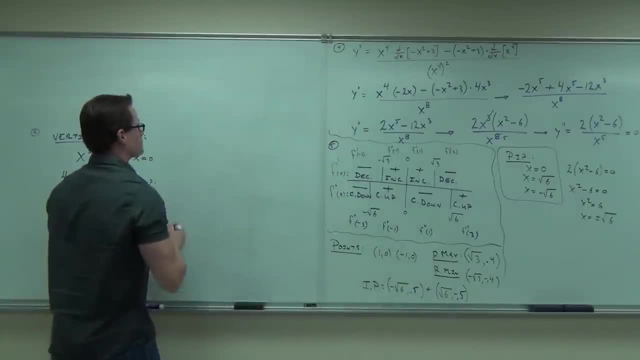 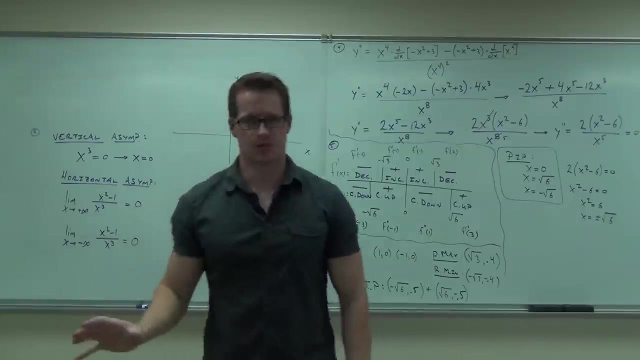 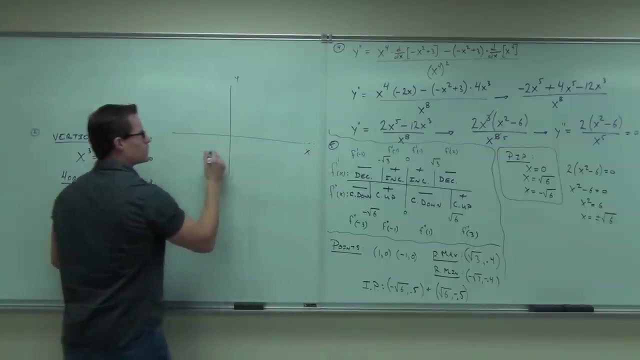 That's going to be important. You're going to kind of see what I want from you on this. The first thing that you should do: put out your asymptotes wherever those things are. So my asymptotes are at: x equals zero, x equals zero horizontally, both right and left, and 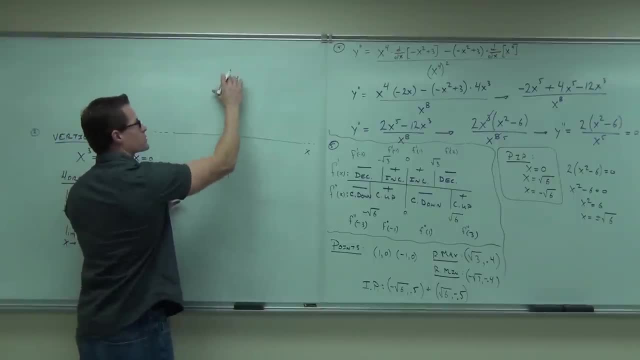 I'm sorry. y equals zero both right and left, and x equals zero for our vertical. So we know we have some asymptotes. Next thing you do put down your points. Your x intercept is at one zero and negative one zero. 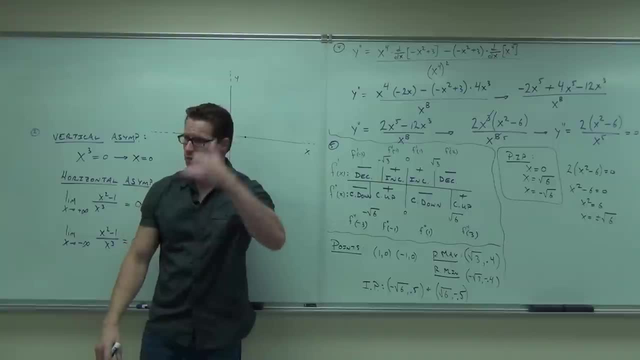 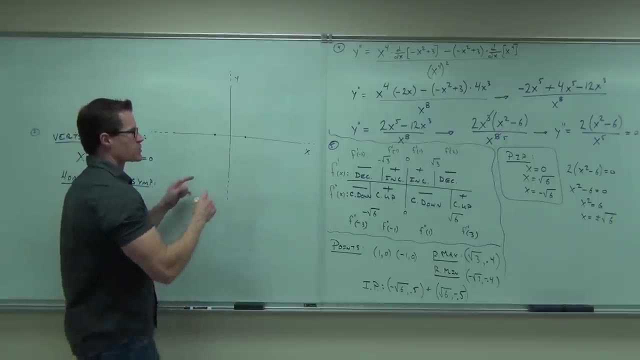 Okay, Your y intercept. ah, you don't have one because you have an asymptote there. you don't have that. Your relative max and relative min square root of three. the square root of three is about 1.7, somewhere around there. 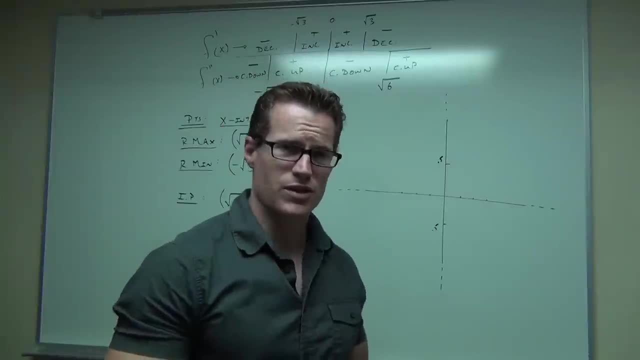 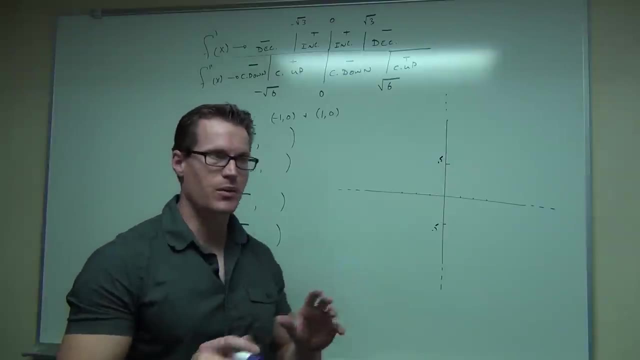 So the relative max occurs at okay. so there's a slight error in the class. The numbers that some of the students gave are a little bit off. Here's the correct numbers. It's a couple times so of course, if you watch the video you're like whoa, what's? 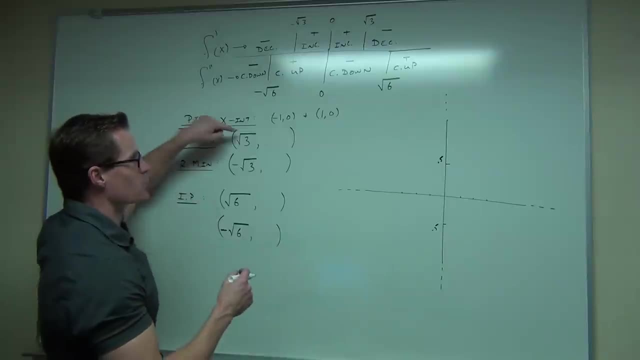 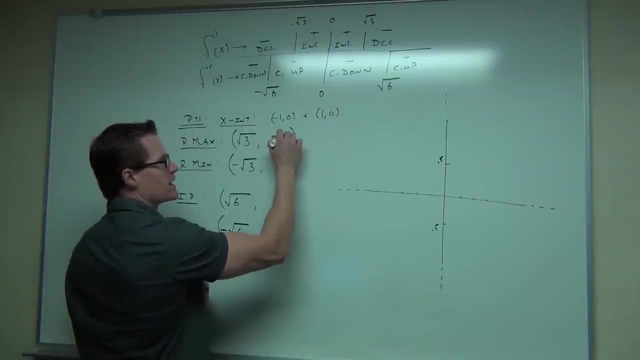 going on here. Why are these numbers changing? Here's why the number's changing. When you take the root three and you plug it into the original equation which gives you points, what you actually end up getting is .38.. If you take negative square root of three, plug it into that original equation. you're. 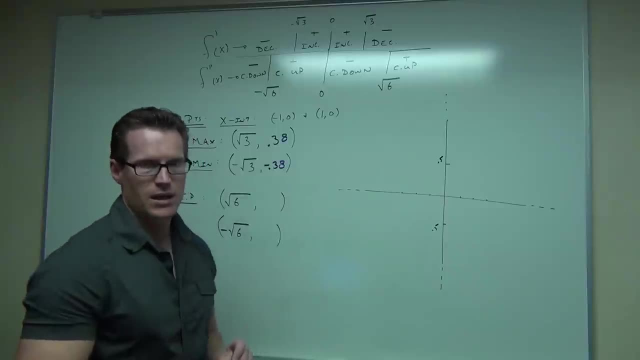 going to get negative .38.. Now, when you take the square root of six, you plug it into the original function, what you're going to get is .34.. Okay, Negative .34 and negative .34.. They're very close points. 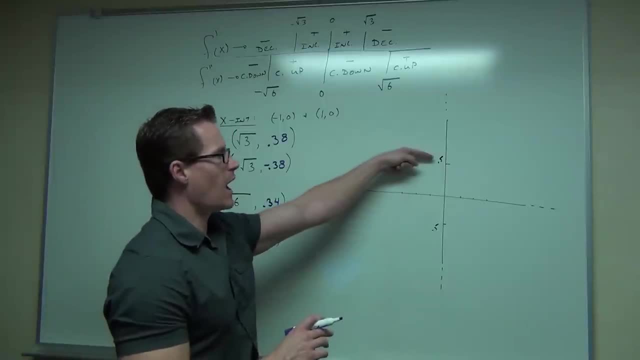 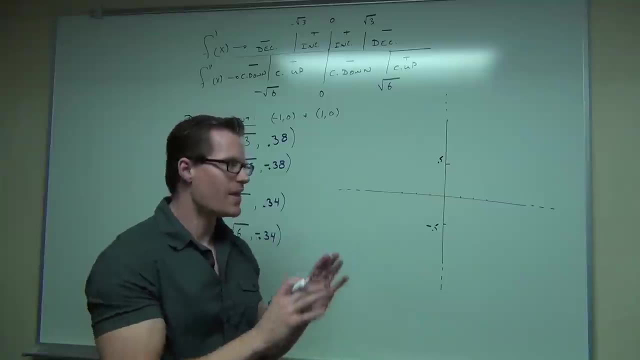 Now the graph's going to look somewhat similar, but you'll notice that on the video I have that as one and negative one If you just change that to .5 and negative .5 and just extend the graph even further. this is about what it looks like. 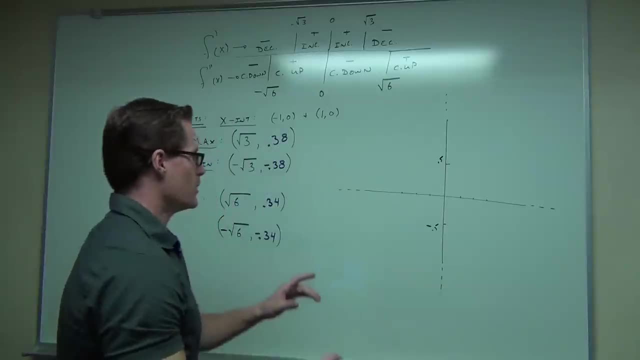 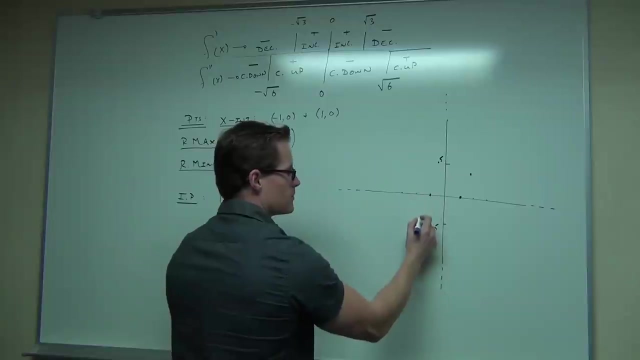 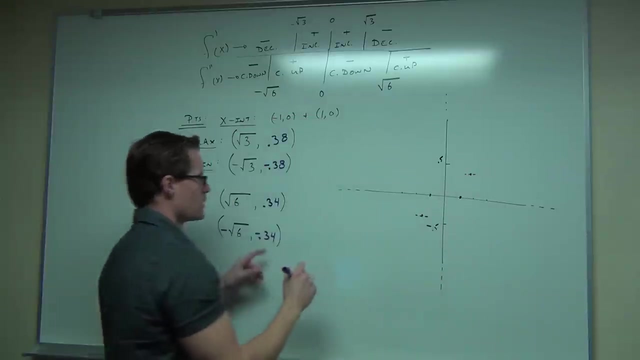 The picture of the graph on the video is just fine. So here's what you would end up doing: You would still have your same x intercepts, You would have your relative min, You would have your max and your relative min. You would have your inflection points. 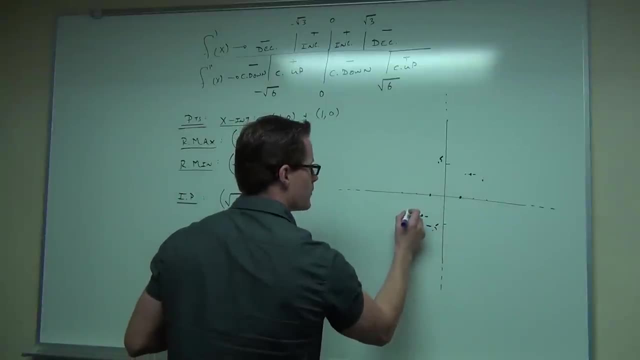 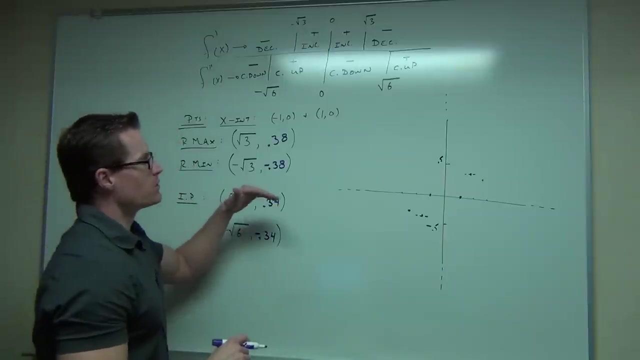 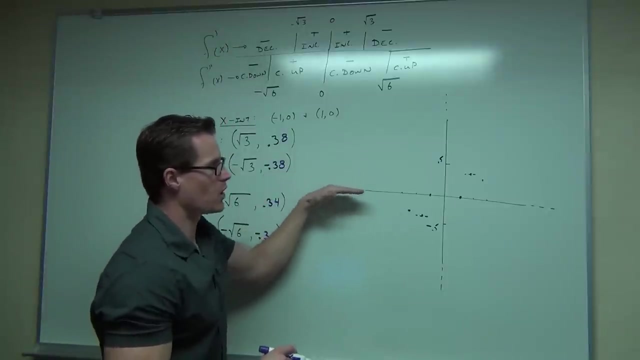 They're just really close together. So our graph, as you can see, we're still decreasing. That's what this is, That's what this means right here, decreasing concave down. So we're dropping and we're concave down. 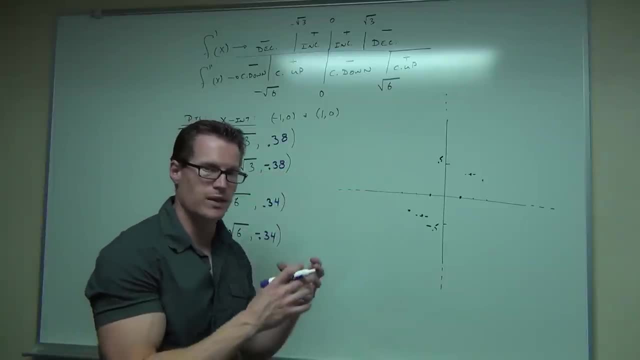 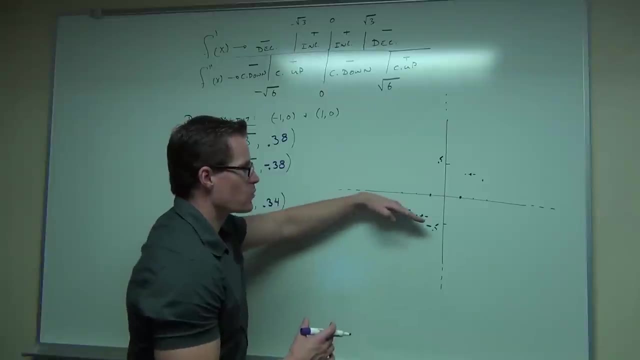 That's this way. Also, we have this horizontal asymptote. That's what that was so important for was to tell us that our function's not going to be going way up like this, not going to be going way down like this. It's going to be riding along this x axis. 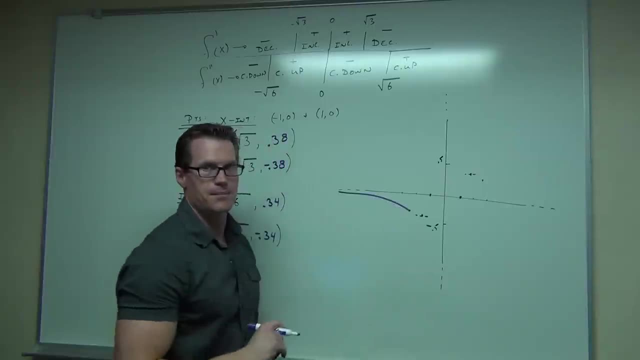 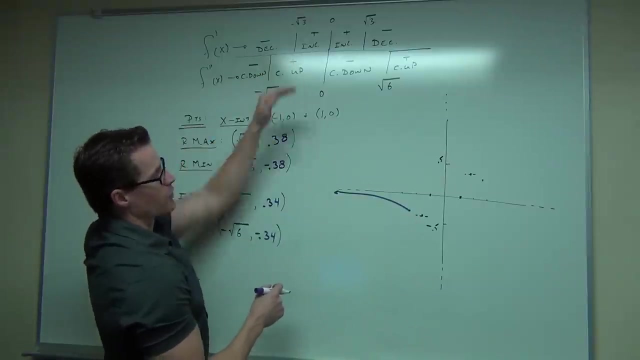 So it must look about like that- Not exactly like that, but pretty close to that. Then, from this point to this point, It's this little interval. It says you're still decreasing, but you're concave up, Your slope is starting to increase. 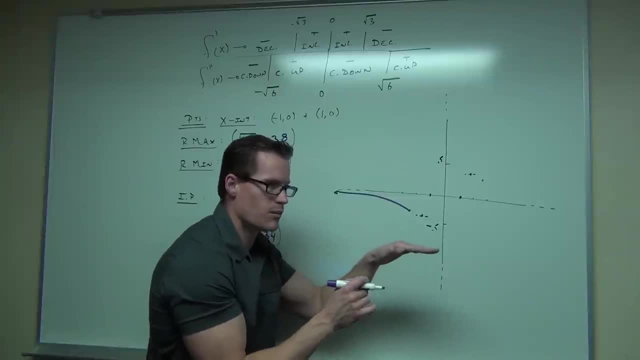 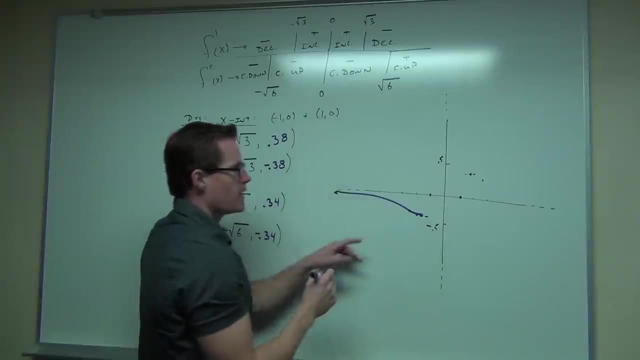 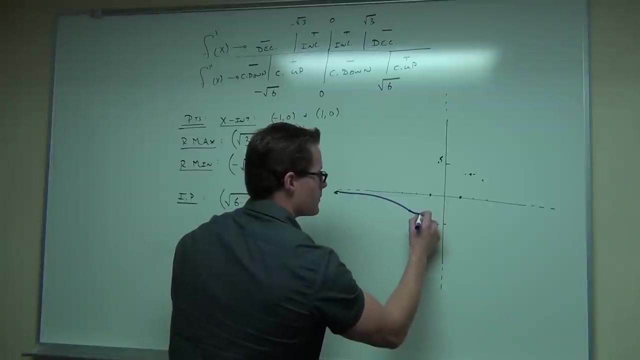 Your function's still decreasing, but your slope is getting larger and larger. So we're going to decrease, concave up. And then, right after that point, right here, it says you're still concave up, but now you're starting to increase. 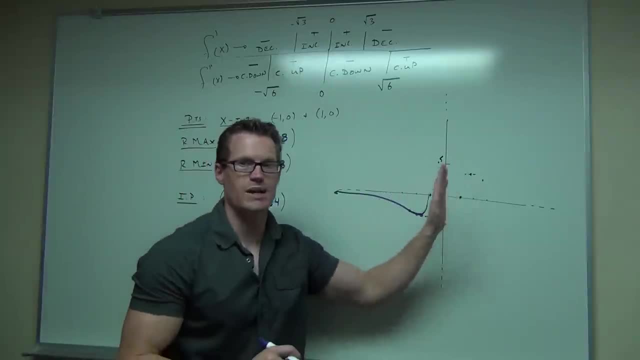 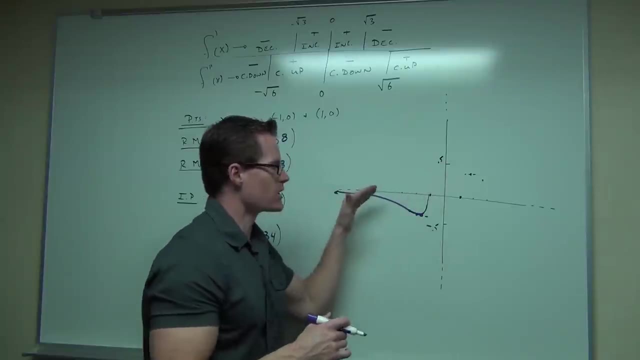 And what that does is increases all the way up until you get to zero. Now, at x equals zero, you have a vertical asymptote, which means that you're never going to reach this y axis. All that's going to happen is if you're still increasing as you get closer and closer you're. 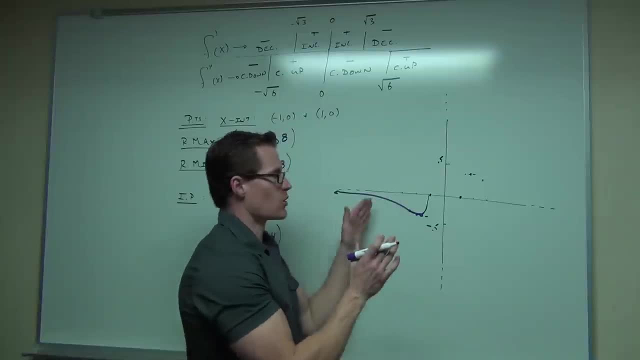 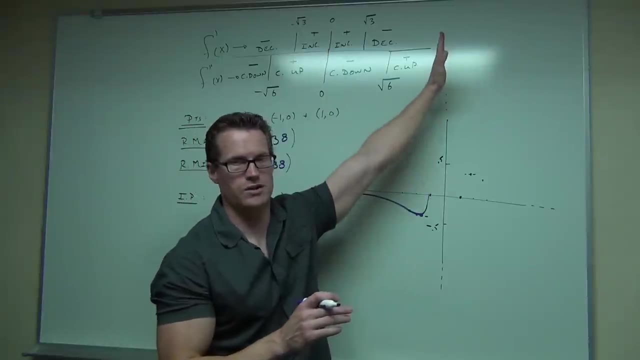 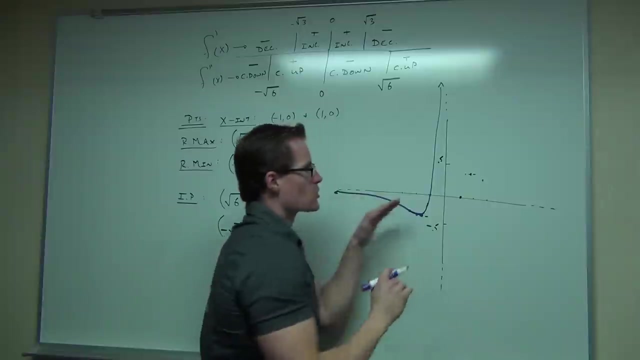 going to shoot up to positive infinity. So that's what the horizontal asymptote said. It says you are increasing, You can't be decreasing. You're increasing all the way up until x equals zero. That says horizontal asymptote. And you're concave up the whole way. 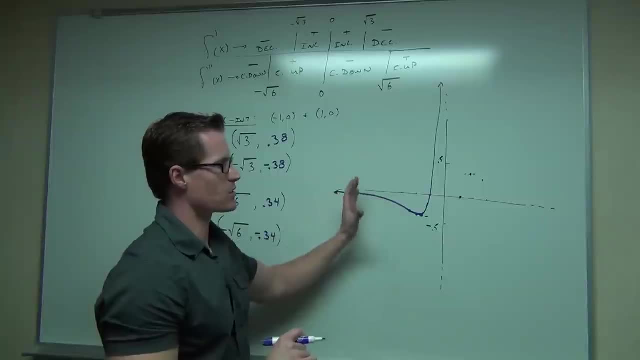 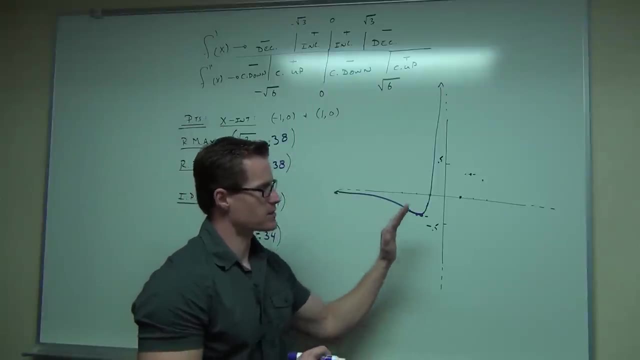 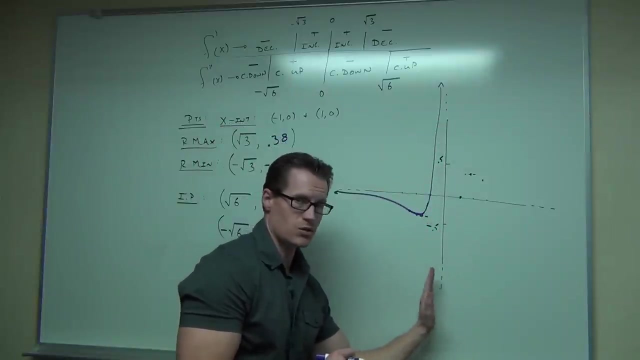 Now the other picture. it's going to look very similar to this, only kind of rotated a little bit, Starting from zero. you're increasing and you're concave down. That's this way, increasing concave down Now, because again you have this vertical asymptote, the only way you can be increasing. 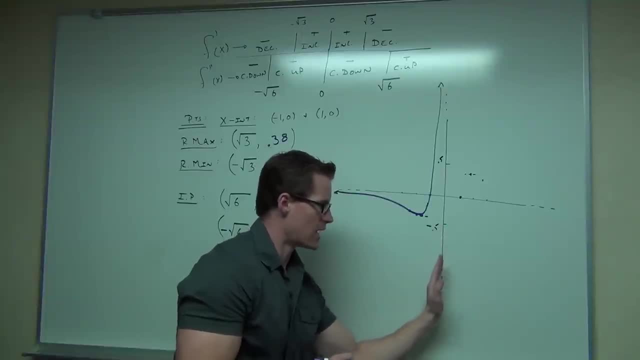 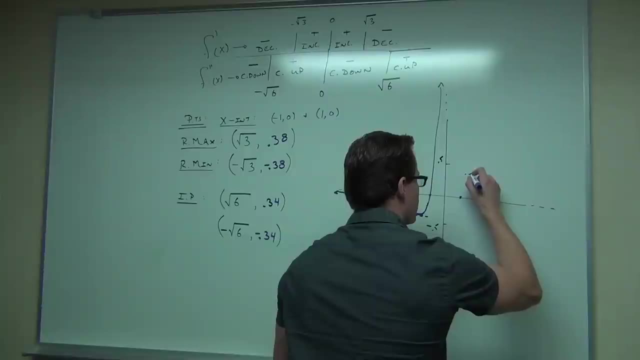 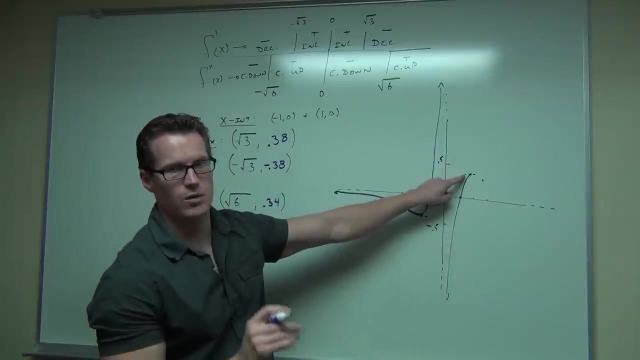 and concave down and have this vertical asymptote is by shooting up just like this. You can't come down, That would be decreasing, So you're coming up like that, Coming up just like that. Now we've reached this point and that is our relative maximum. 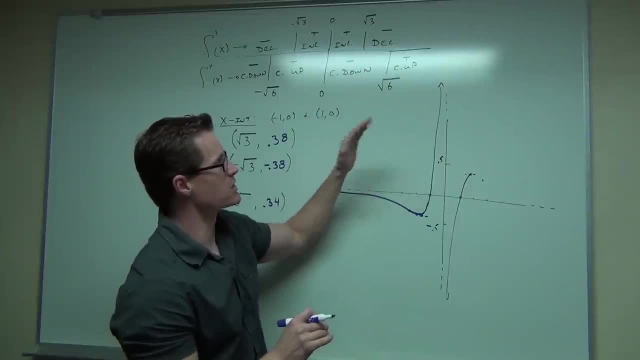 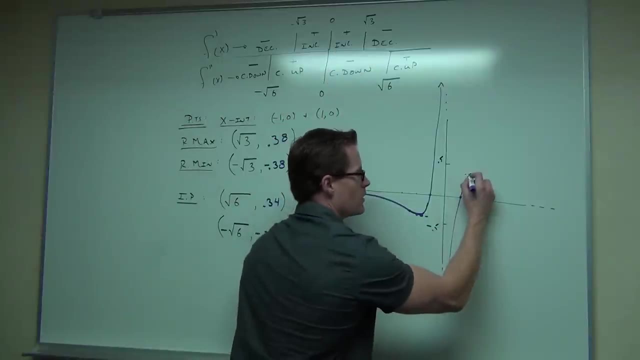 It says: at your relative max you switch from increasing to decreasing but you're still concave down for that whole interval. So increasing to decreasing but concave down. That's that little point right there. After that point it says you're decreasing for the rest of your graph. 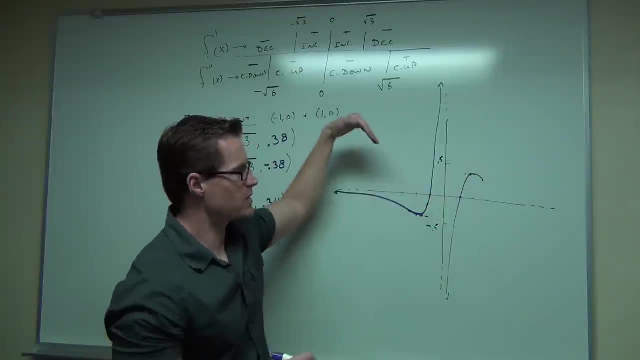 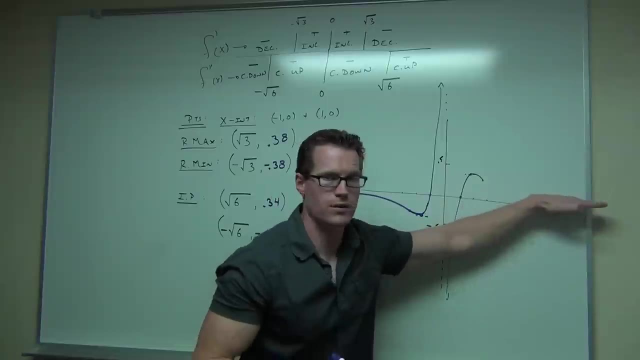 You're decreasing the whole way, but now you're concave up. The only way we can decrease the rest of the way and be concave up and associate this whole horizontal asymptote is by putting it right along the x axis, just riding that thing. 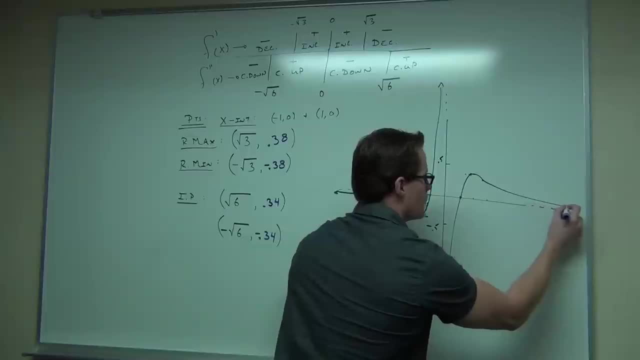 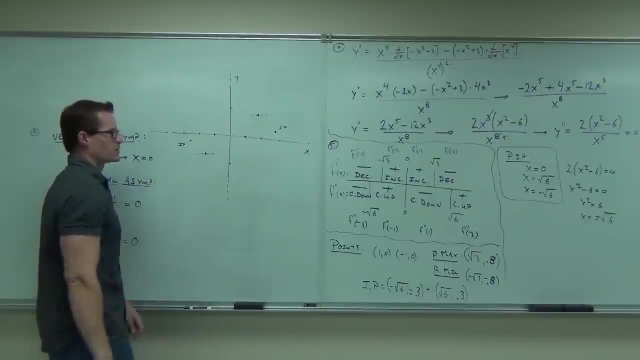 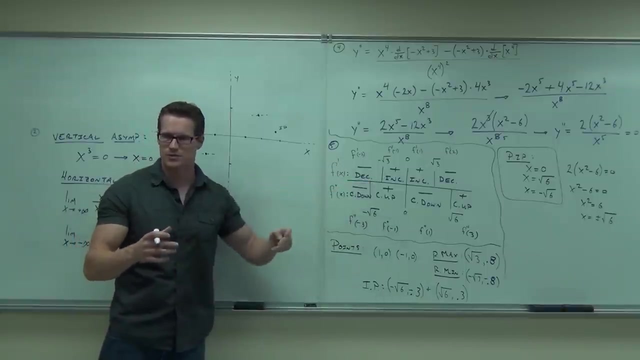 all the way out, And that's the same picture that you have on your graph. That's an inflection point. Now, how in the world does this graph look? That's the way I have the table. This is pretty interesting because we're going to associate all this stuff with our asymptotes. 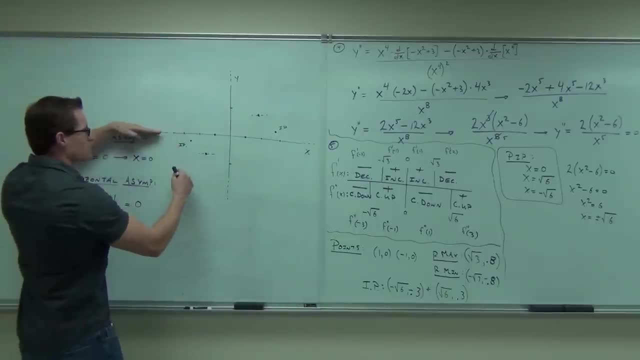 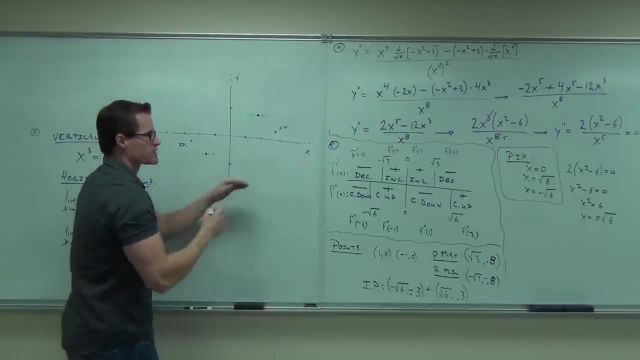 Now check it out. You know that this has to go close to this one. This has to go close to this one. It has to go here, somewhere and there somewhere right Now. here's what it says. It says you're going to be decreasing. 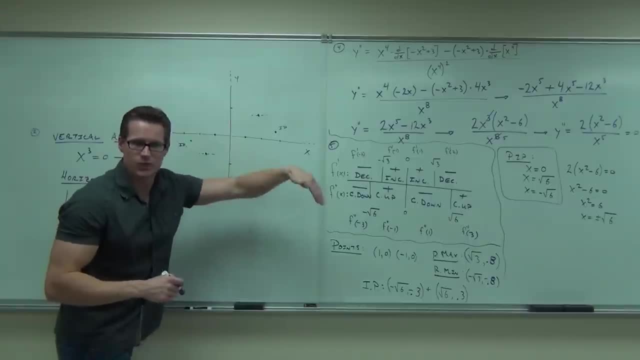 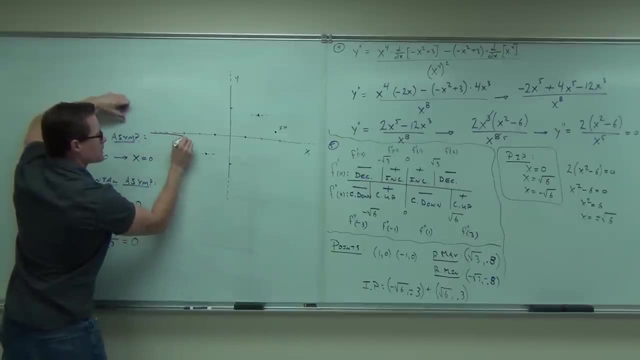 Decreasing is like this and you're going to be concave down. That's this way. Does that make sense? All the way until you get to this point, that negative root six. That looks like this: Decreasing, concave down. 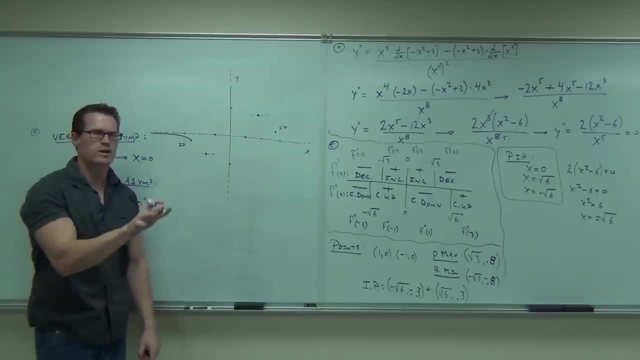 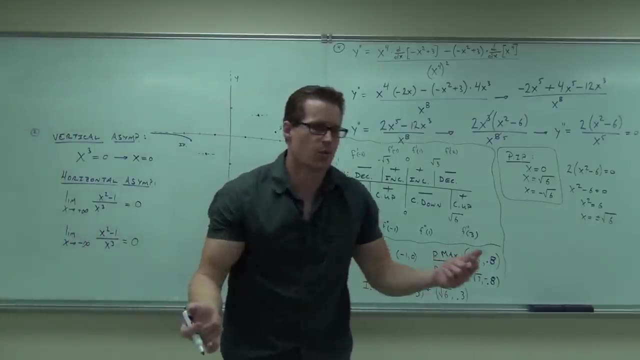 Do you follow me? That's the only way you can have it. If you're decreasing concave down up here, you fail the asymptote. You have to be with the asymptote. so asymptotes are important. It says you're going to be at that asymptote, right there. 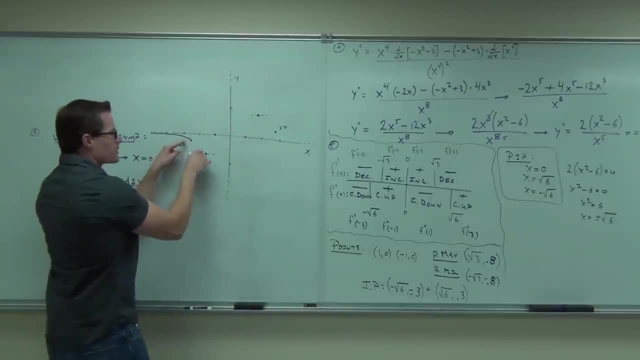 You see what I'm talking about. From here to here, this little interval says you're decreasing, but you're concave up This part decreasing down, This little part decreasing up. That's the inflection point coming back at us. 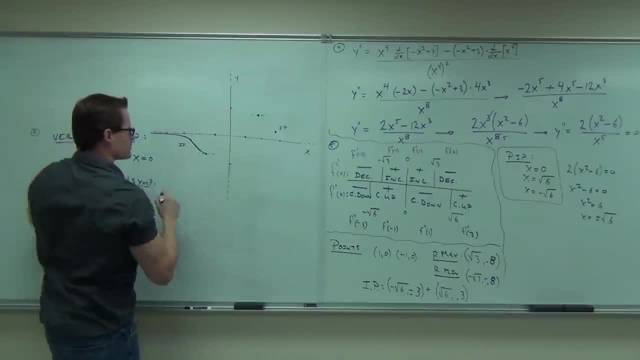 That's this. That's concave up. You see the decreasing concave up. Then this part says increasing concave up. That's this way, And you actually do that all the way to zero. Now how do we go all the way to zero? 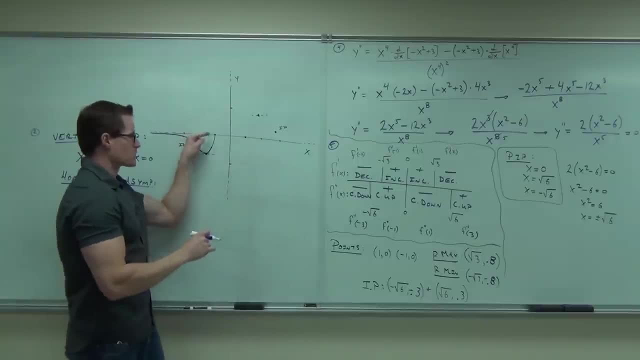 Where do you think this is going? If it's increasing and there's an asymptote, does it magically go back down here? Otherwise we'd have another relative max, wouldn't we? It's going to go all the way to infinity. There's an asymptote, folks an asymptote. 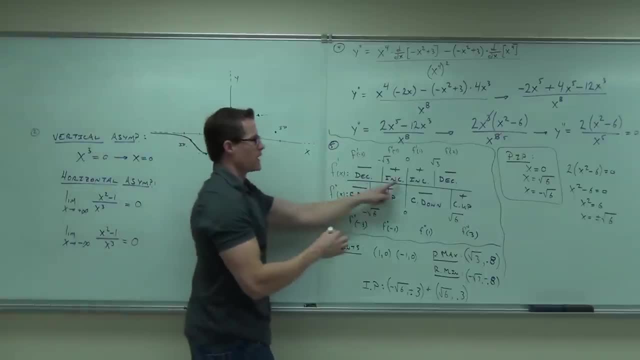 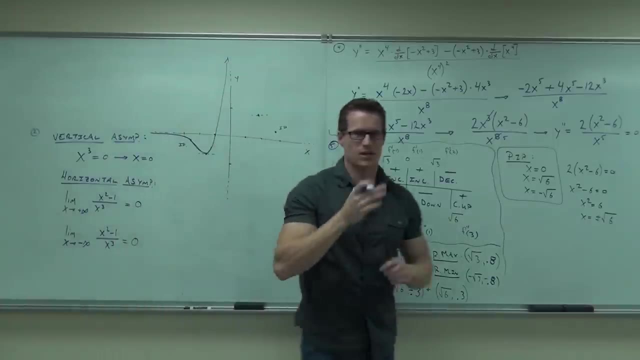 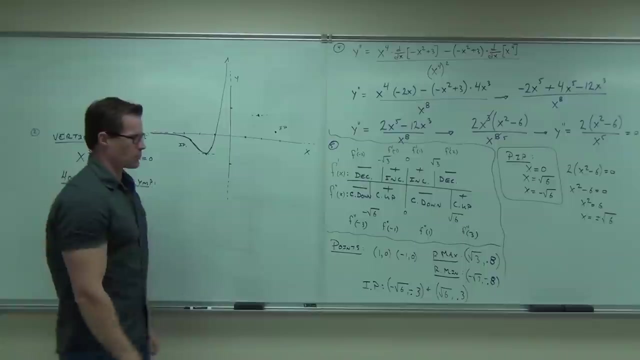 It has to go to the asymptote. So if it says increasing concave up to zero, it's going like this Forever. Is there any other way that it could be and still have the asymptote? Nope, Now the rest of it, the other side of the graph. 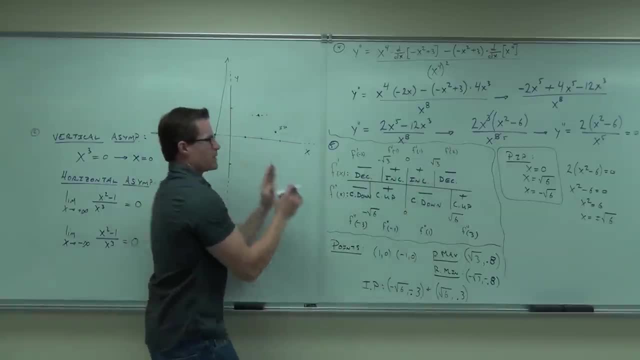 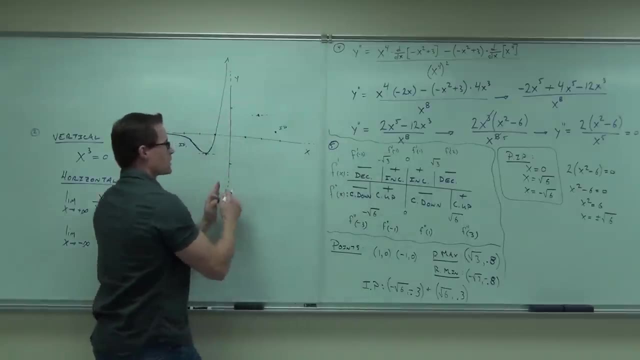 The other side of the graph says: for this interval up to root three, you're increasing, you're concave down. That's this way. You follow Increasing concave, but you also have an asymptote, so you have to meet the asymptote. 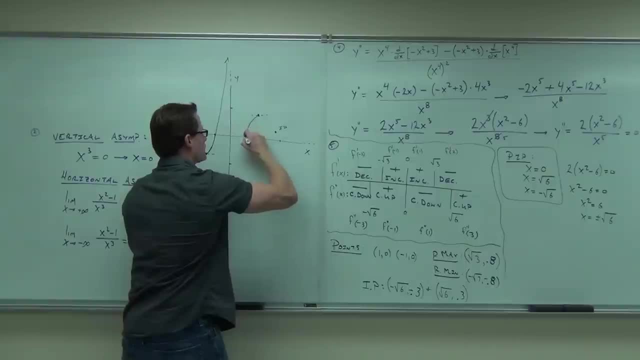 Increasing Concave down. That's increasing concave down Until you reach a relative max. You know that's a relative max. Then it says: for this little interval, you're decreasing, you're decreasing and you're concave down. 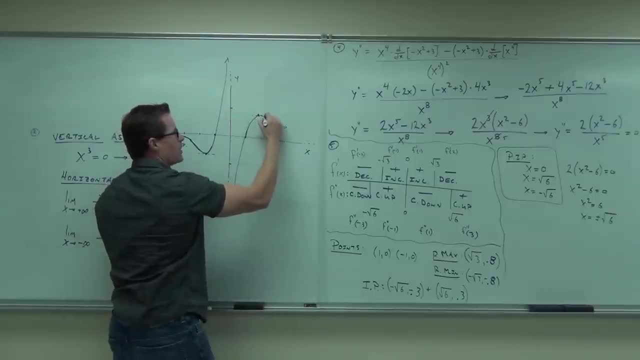 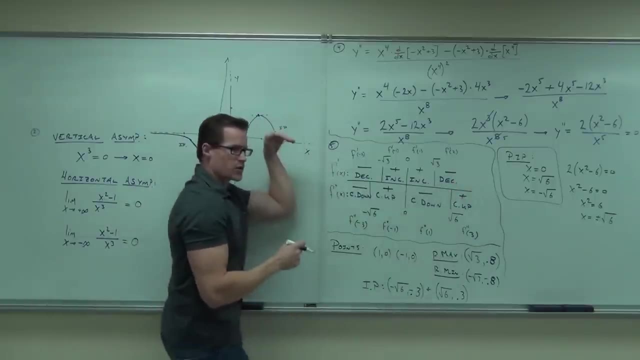 Decreasing and concave down. That's this way. So for here, you're going to go oh down And then, from here on out, after that root six- remember that's our root six- you're going to be decreasing but you're concave up. 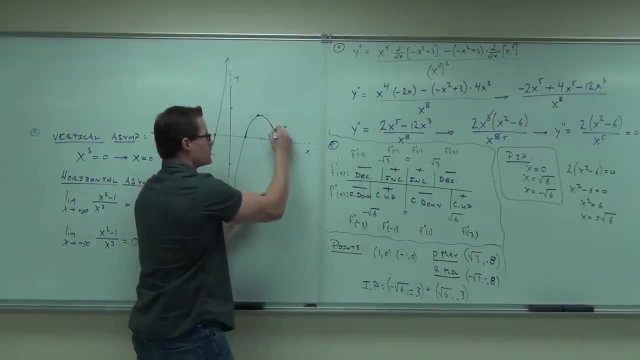 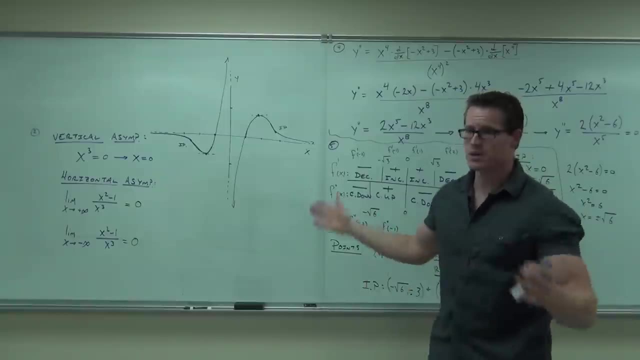 That's this way And you have to meet that asymptote. Okay, That's there. That's good as we can do, But that's a pretty darn good graph. for just having some for no graphic calculator, That's pretty good. 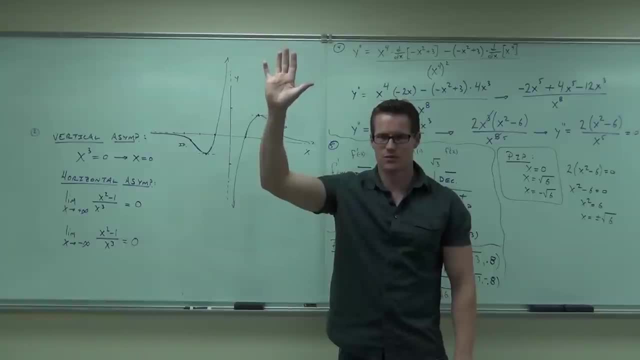 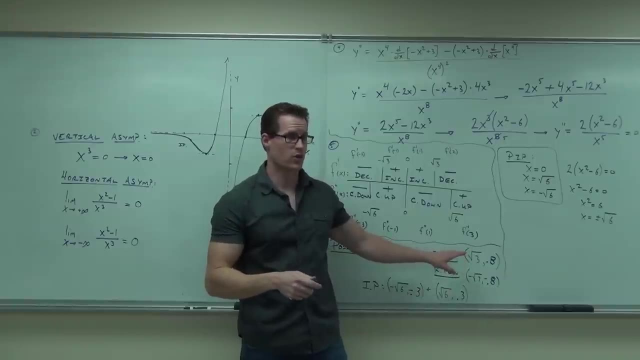 How many people are able to follow that? Now you've got to be careful. Be careful with these numbers. You messed me up, but that's okay. Be careful with your numbers on your own Now. we only got through one example. 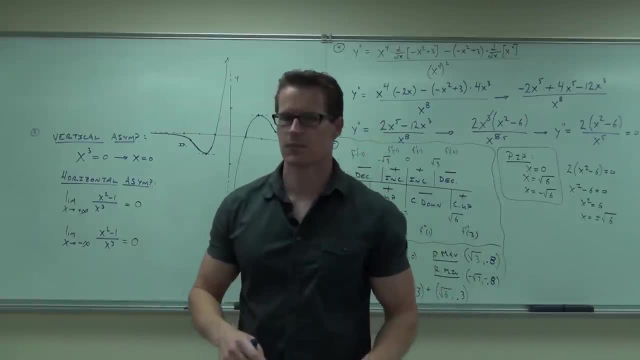 If you want to hang out just a little bit, I'm going to try to do one more. Okay, All right, We're going to do one more example: How to graph some rational functions. I'm going to try to go all the way through it, but I'm going to be erasing things as 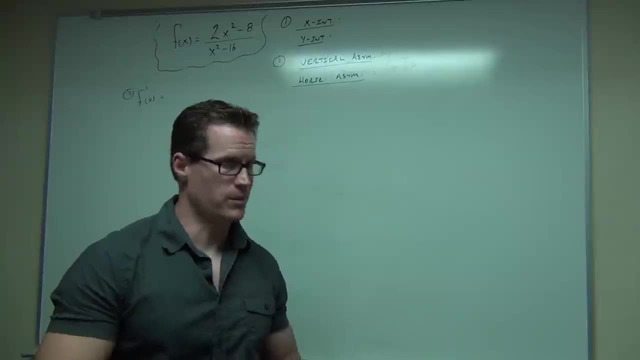 we go. So it might help you to write this down as we're going through it. That way when I erase it you're not like totally lost. So I'm going to save some space. I only have a limited board to work with. 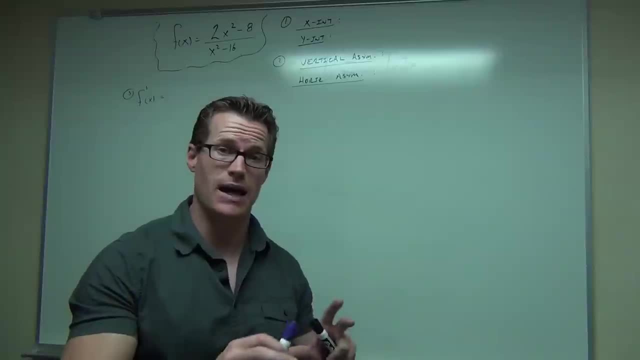 So let's start with our x and y intercepts. That's always step number one. X intercept says: where is the numerator equal to zero? That's the only places where this function can actually be used. So let's start with our x and y intercepts. 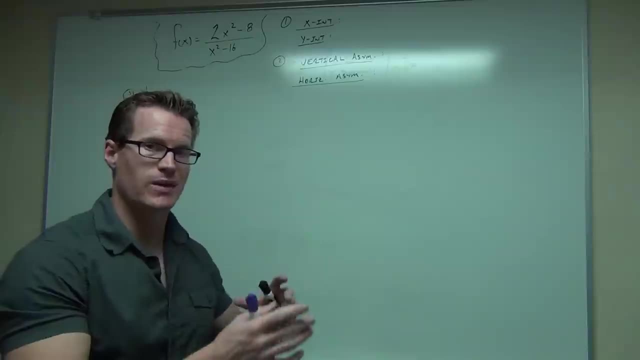 That's always step number one. X intercepts says: where is the numerator equal to zero? That's the only places where this function can actually be used. So let's start with our x and y intercepts. That's always step number one. 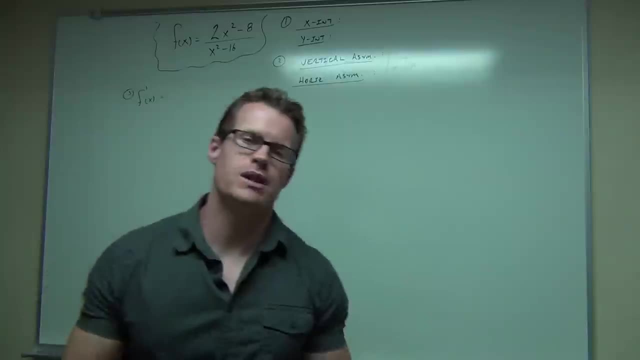 X intercepts says: where is the numerator equal to zero. That's the only places where this function can actually be used. If the denominator equals zero, then we're undefined. We have either the wholes or asymptotes. So in our case, x intercepts are at eight divided by two. take a square root plus two. 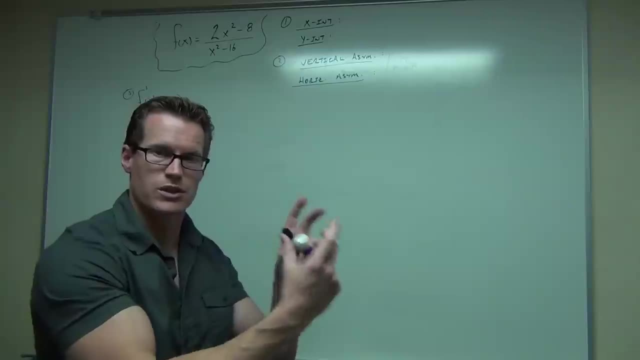 minus four times eight minus 4.. So in our case, x intercepts are at eight divided by two. take a square root plus two times eight, minus four times eight, minus four times eight, minus four times eight plus four times eight. 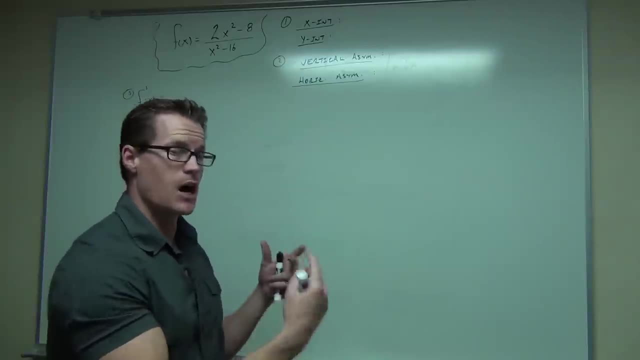 So that's this keinenheit of the numerator and the above denominator. So let's use this as an example. So these are the equations for all the ways you can actually compute them. If the denominator equals 0, then we're undefined. We have either the wholes or asymptotes. 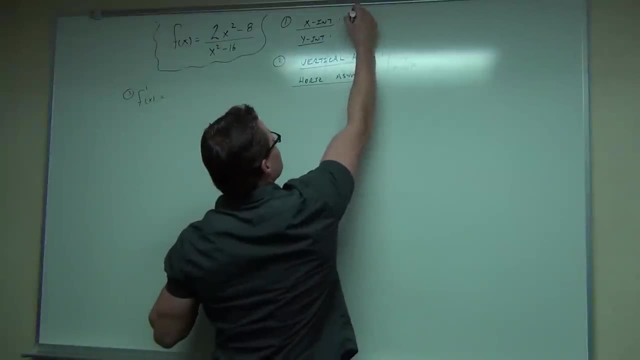 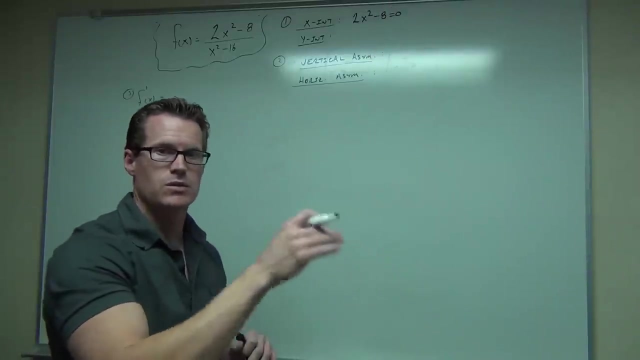 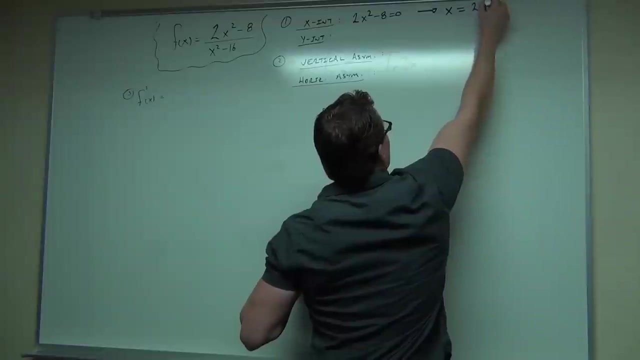 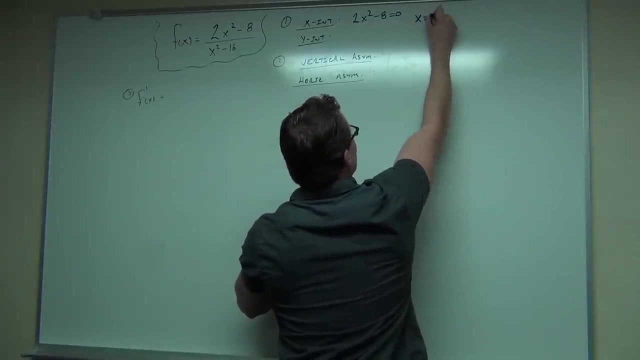 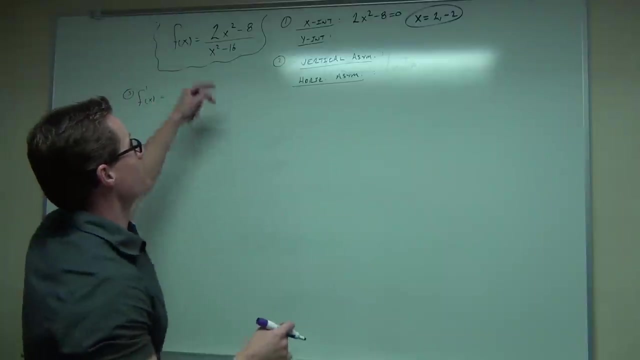 So in our case, x-intercepts are: add 8, divide by 2, take a square root, plus and minus 2.. I'm going to write that a little bit lower. Okay, y-intercepts you plug in: x equals 0, what you have is 0 minus 8,, 0 minus 16,. 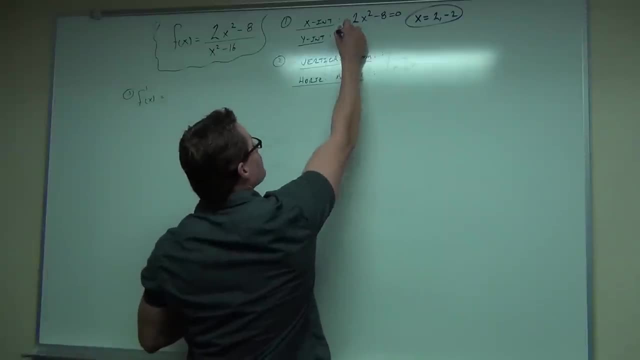 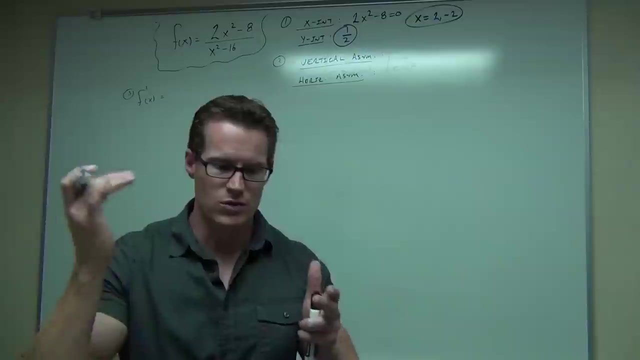 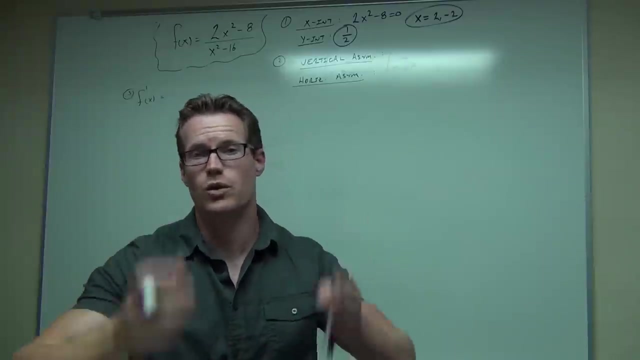 negative 8 over negative 16 is positive: 1 half Vertical asymptotes: those occur where your denominator equals 0 and you can't cross it out. You can't simplify. If you were able to simplify it, it would be a whole, but if you're not able to simplify it, that's a vertical asymptote. 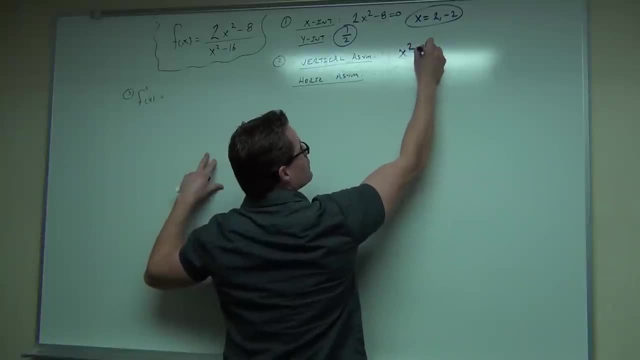 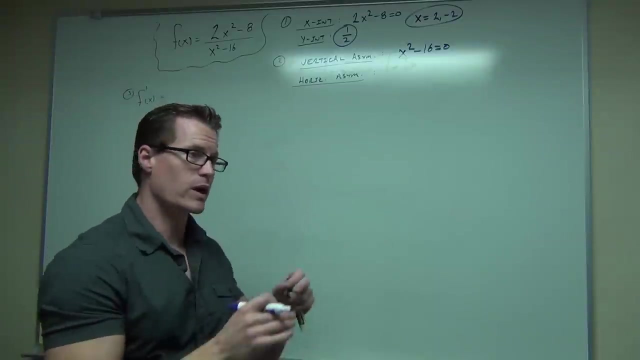 So when we have this denominator equal to 0, again, well, it's a difference of squares. You can factor it, You can add 16, take a square root. Either way, you're going to get x equals 4 and negative 4.. 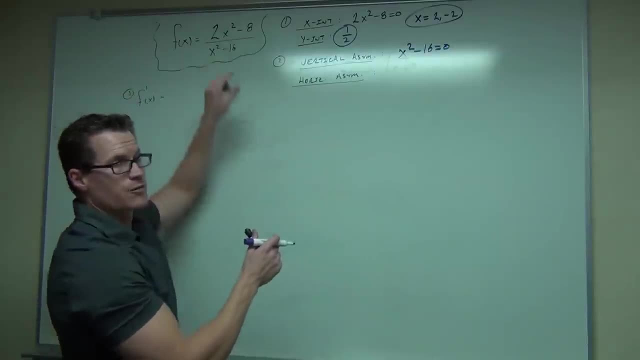 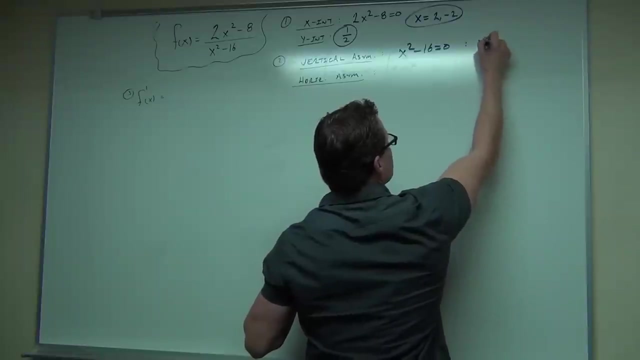 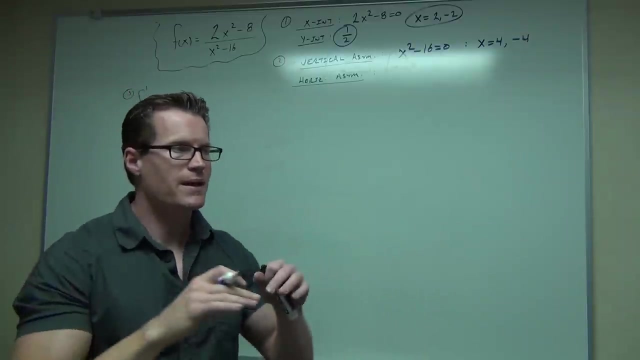 Now x plus 4 and x minus 4, they do not simplify with our numerator. That means they're not wholes. They are in fact asymptotes. All right now as far as our horizontal asymptotes go. that says what happens when we take x to infinity and negative infinity. 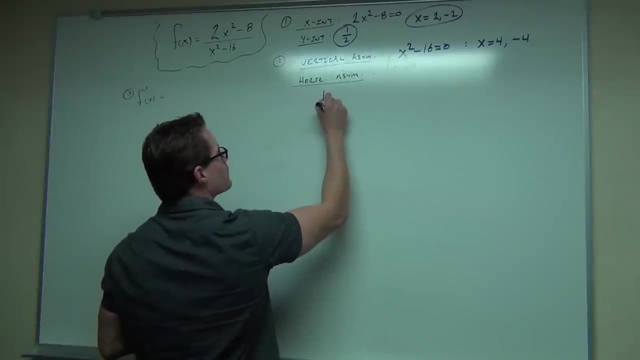 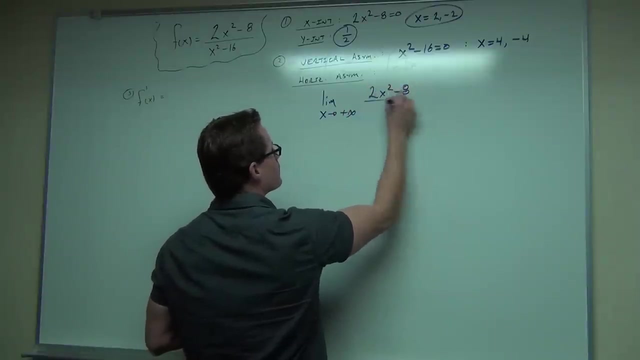 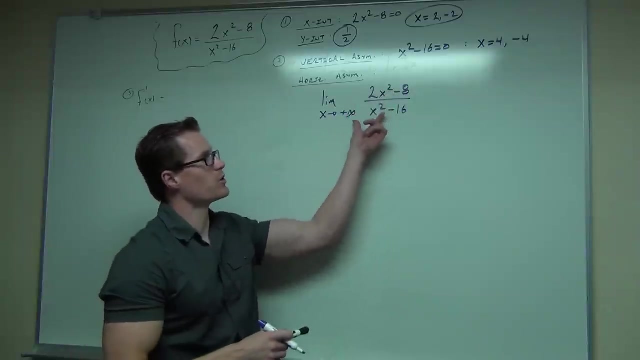 And that's the limit. If you notice that we have our leading terms: polynomial here, polynomial here, the powers are the same. So when you do that whole divide by the largest power in the denominator thing, you're going to divide by x squared. 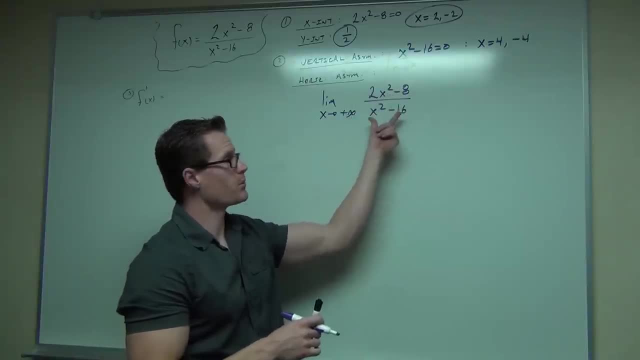 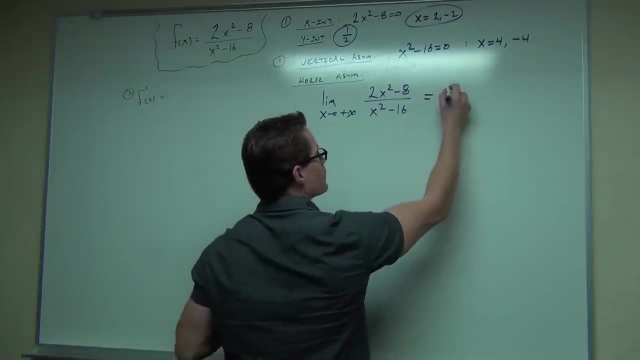 What that's going to give you is 2, 0, 1, 0.. So basically, you have 2 over 1.. That's going to be 2.. Also notice that it doesn't matter if I have negative infinity either. 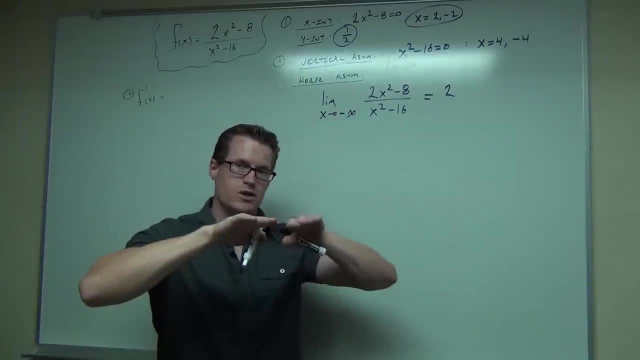 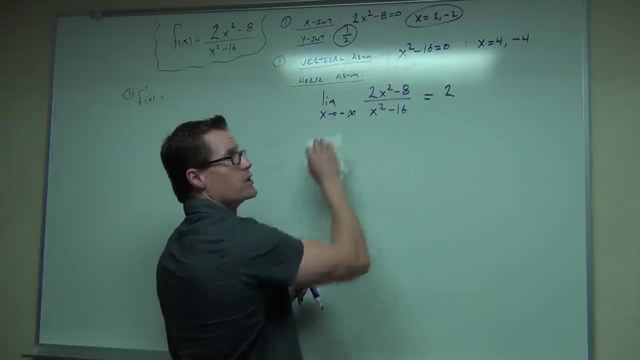 You get the same exact thing. What that means is we have a horizontal asymptote at 2 to the right and 2 to the left, So I'm going to erase this now. We know our horizontal asymptotes are at 2 either way. 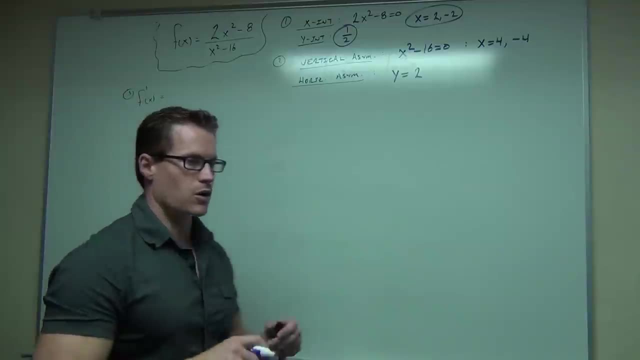 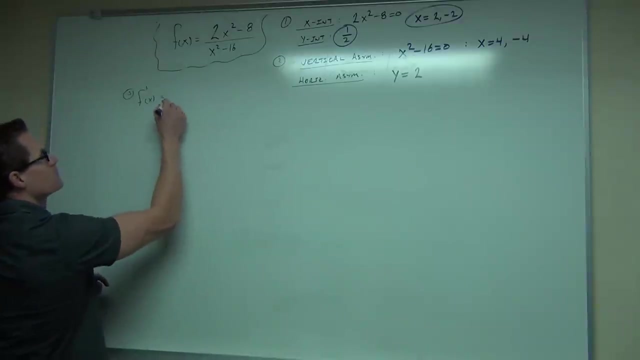 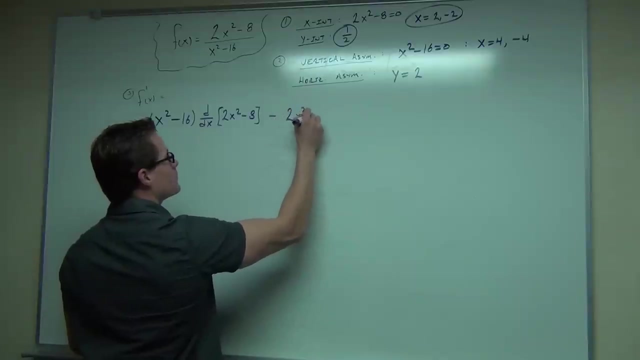 y equals 2.. Now, as far as our first derivative test and second derivative test here goes, our derivatives Try to follow along Again. I'm going to erase this when I'm done. y equals 2 aims to be 1 and 0. 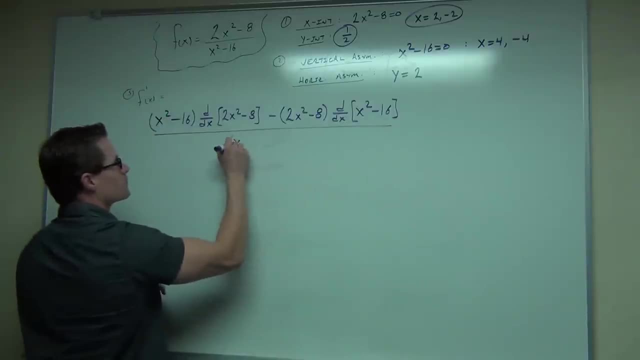 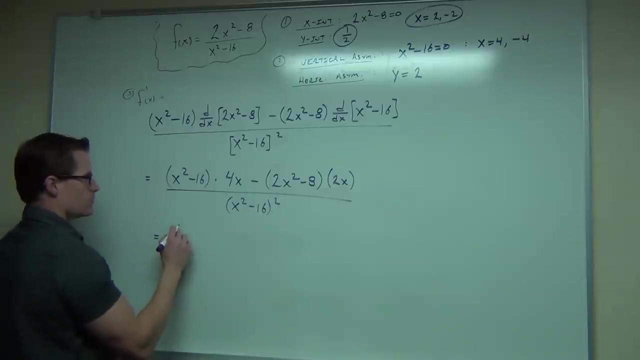 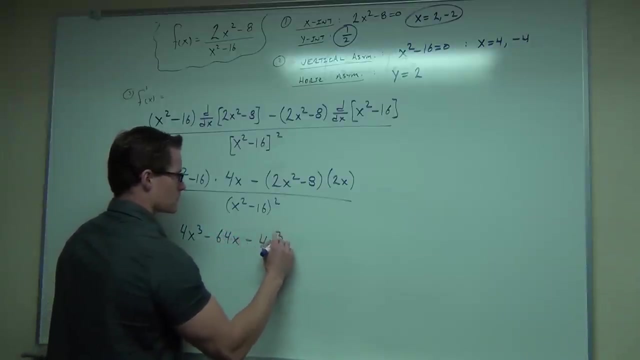 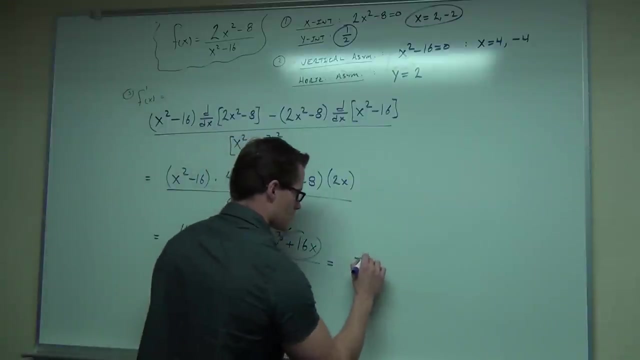 Now, honestly, if you knew Vm Jupiter, you would have gotten it right. You would have gotten it right. You would have gotten it right. Thank you. That's our first derivative. Now, what the first derivative says is slope. 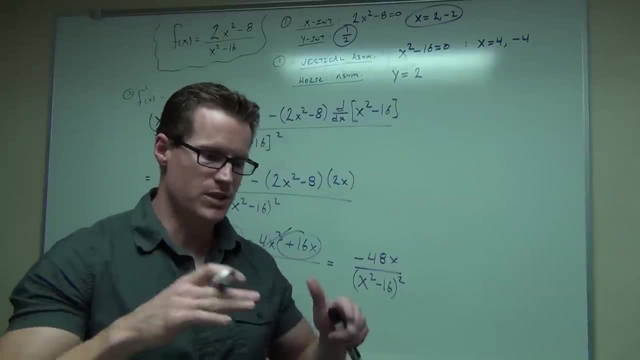 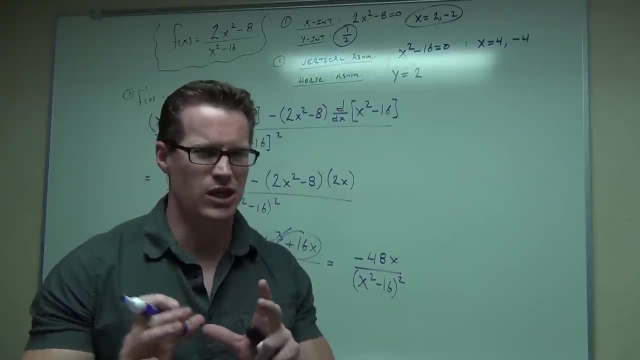 Where slope is positive, you're increasing. Where slope is negative, you're decreasing. Where slope is zero, you have the potential for a relative max, relative min Or something interesting, Maybe around an asymptote or something: Change from increasing to decreasing. 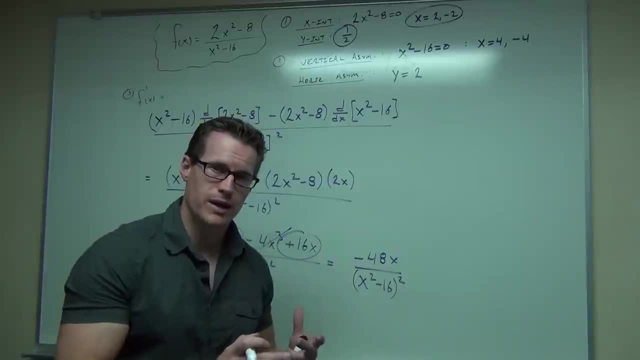 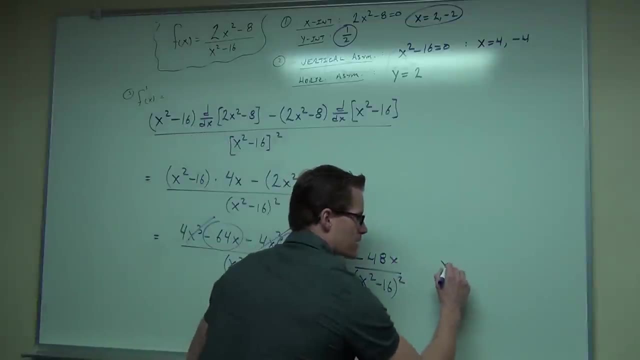 We've seen that before. So the ideas are: find all the places where the numerator and the denominator equals zero. So in our case the numerator equals zero. When negative 48x is equal to zero, that says x equals zero. 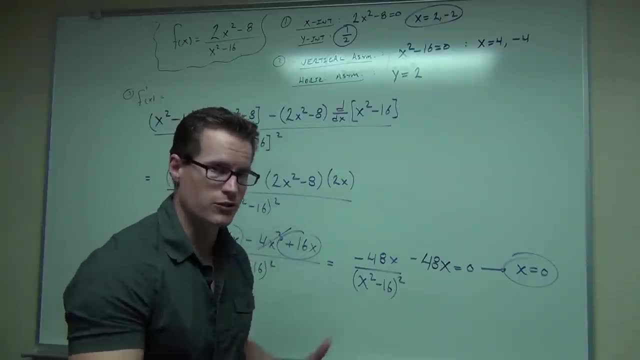 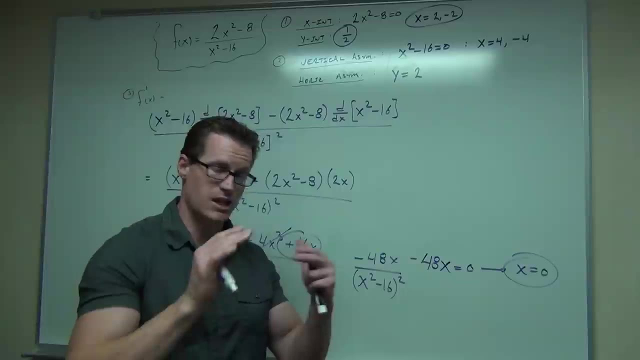 That's going to be one critical number. That possibly is a relative max, relative min. Now, where the slope is undefined, it's not necessarily a critical point, But it could change. It could change from whether the graph is increasing to decreasing or vice versa. 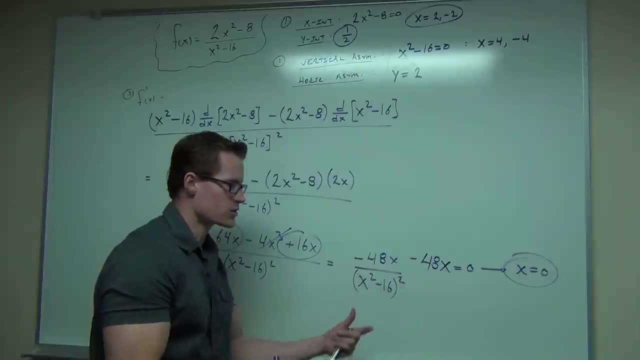 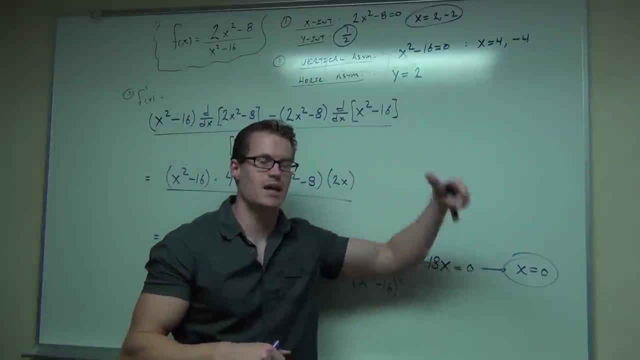 So in our case here- hopefully you can see this- Denominator equals zero when x is four and negative four. It's not coincidental that that's our vertical asymptotes. Those points can come up again, especially with the quotient rule. 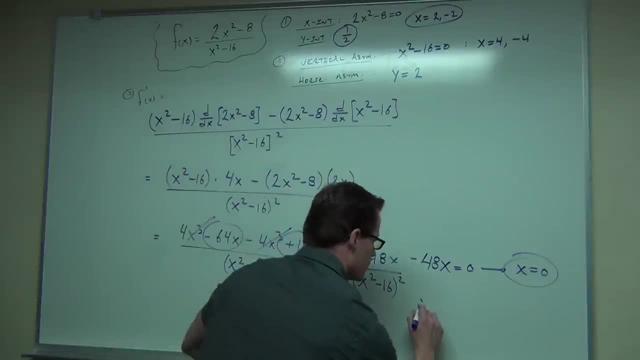 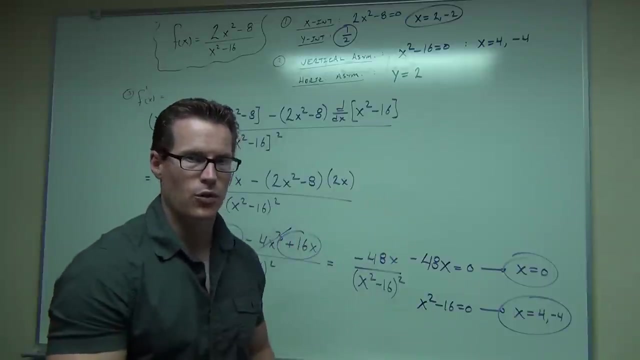 when you notice you're just squaring the denominator. So three critical values that we're going to be putting on our first derivative. We've got our zero, our four and our negative four. Take a look at this. Hopefully you've written this down. 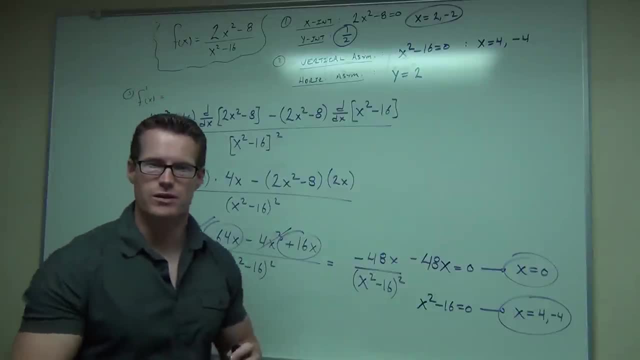 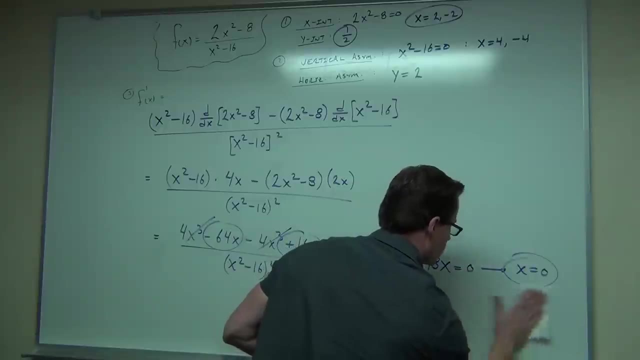 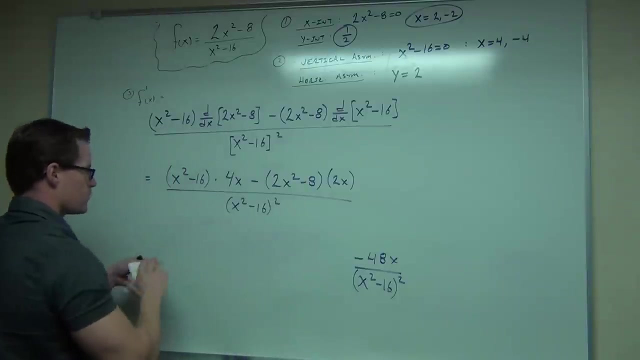 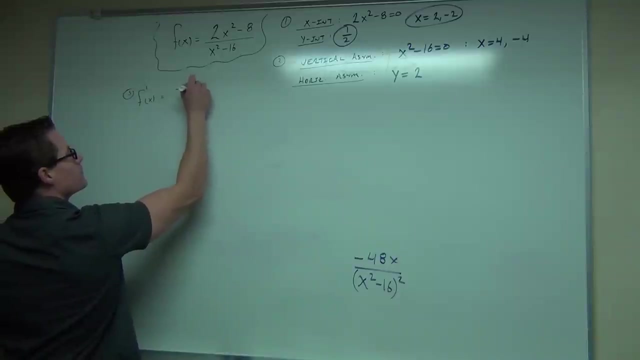 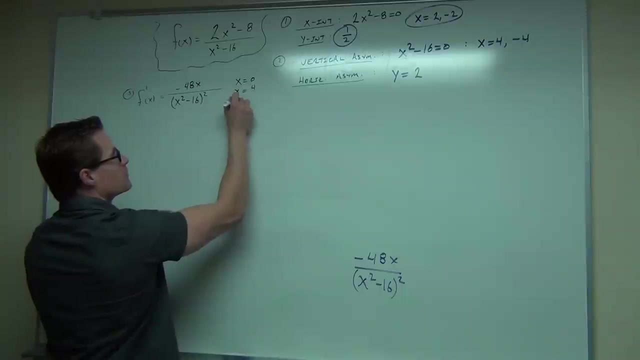 I'm going to erase this right now and write it right up here, That way I can work on my second derivative. So we have the number zero, the four and our negative four. What we got out of that again was zero four, negative four. All right, We're going to add up those points, Then we're going to add our four and our negative four. So one cubed one minus four. What we got out of that again was zero four negative four. 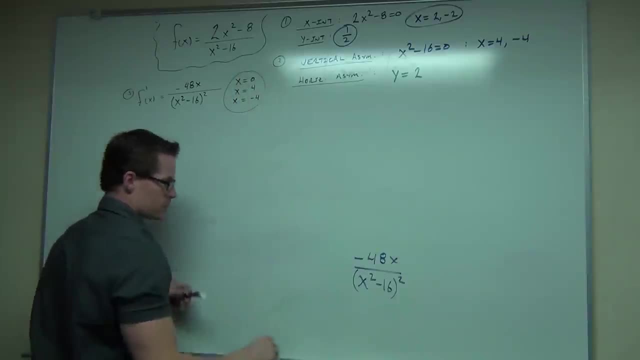 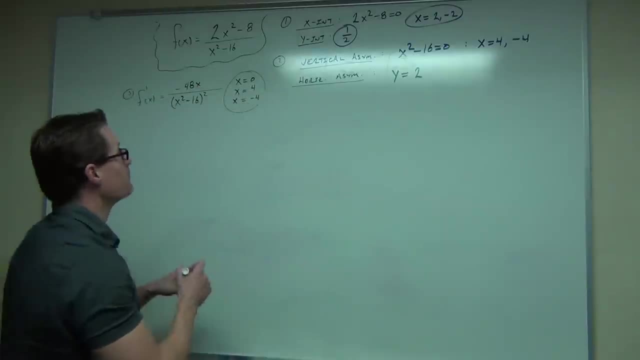 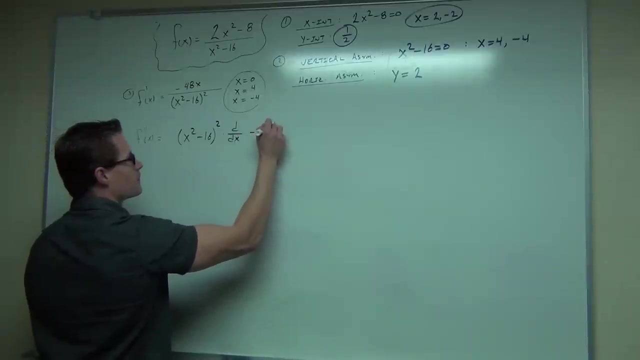 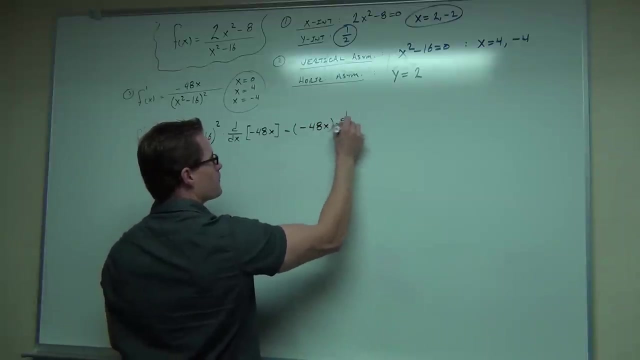 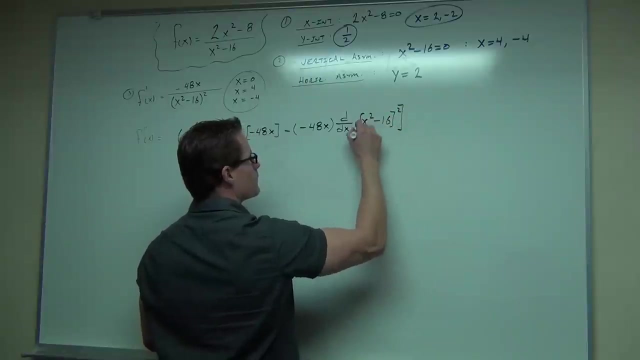 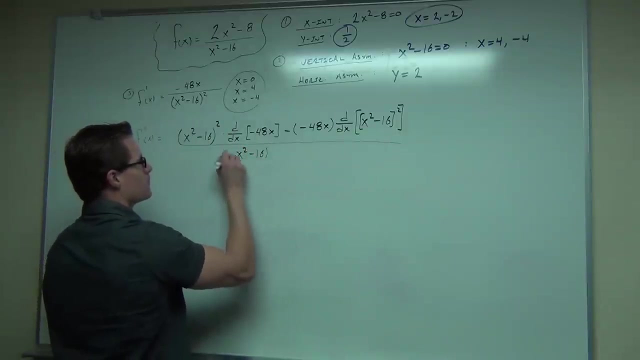 So let's take the second derivative and see what we get. Again, write this down and erase it when I'm done. Let's take the third derivative and erase it when I'm done. Again, write this down and erase it when I'm done. 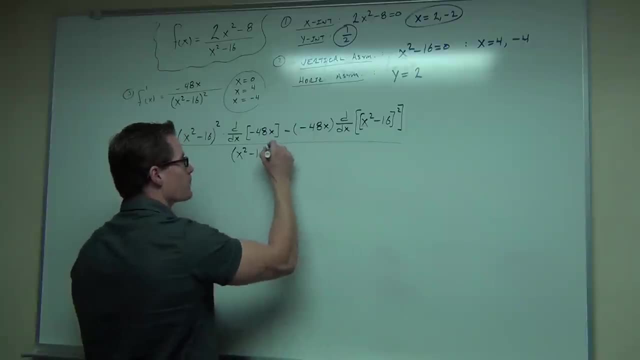 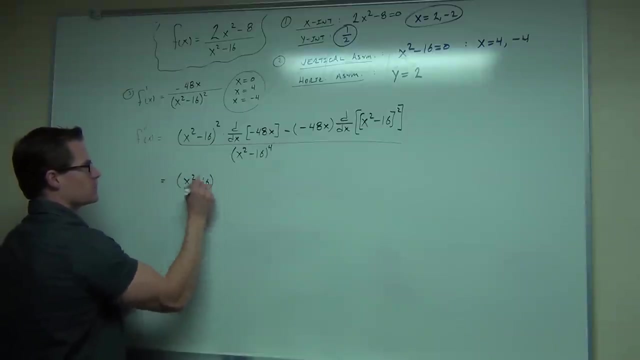 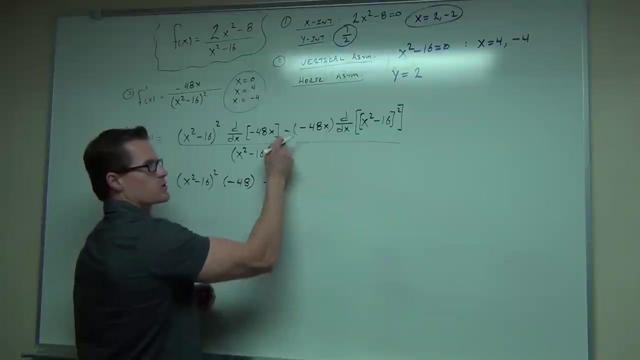 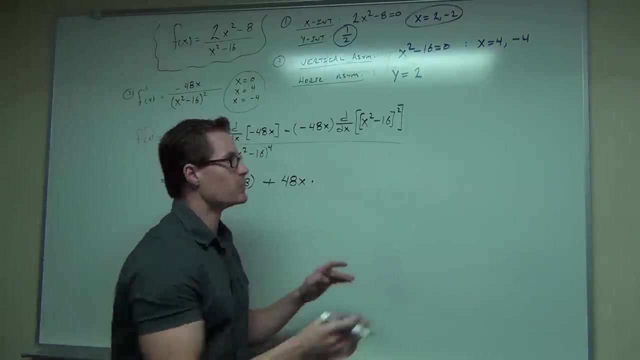 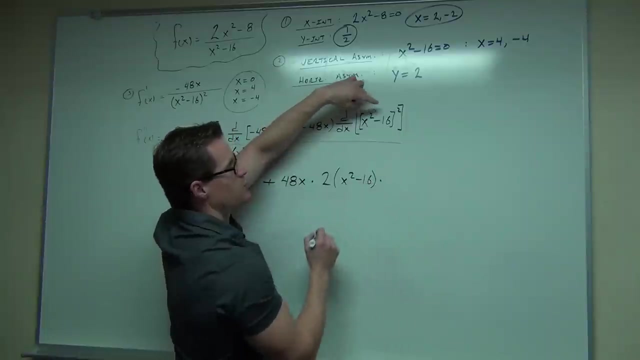 This is going to be the fourth power. since we're squaring that square, Notice the plus. I'll change that right now. I'll just make a negative negative into a plus. Also, I'm going to take a shortcut here. I know I tell you not to do this, but we're going to take a general power. rule times: the. 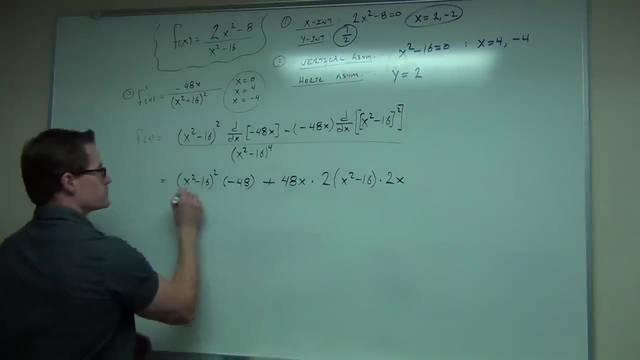 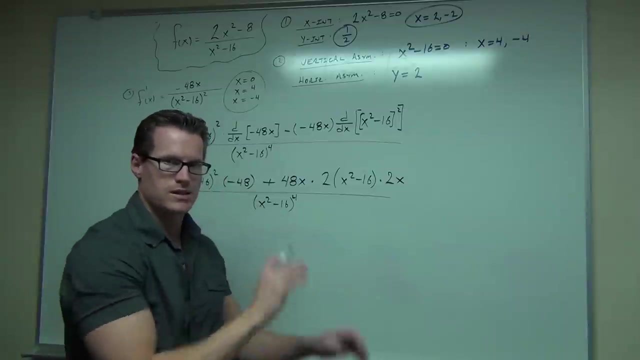 derivative of the inside, and that should be our derivative. Now we're going to do a little fancy math here. We're going to simplify a couple pieces, but I'm going to leave a couple pieces alone because I want to factor it. I want you to see the factorization. 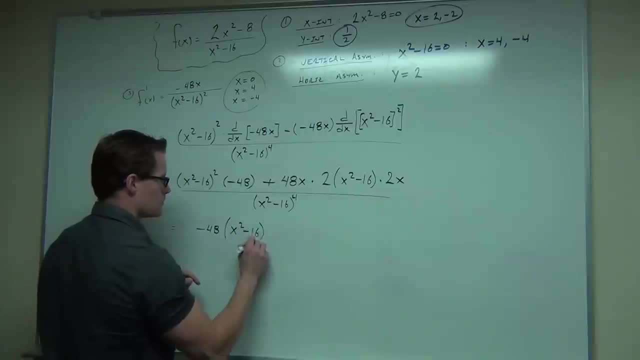 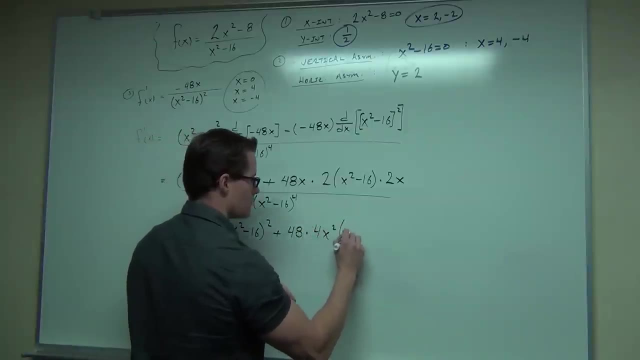 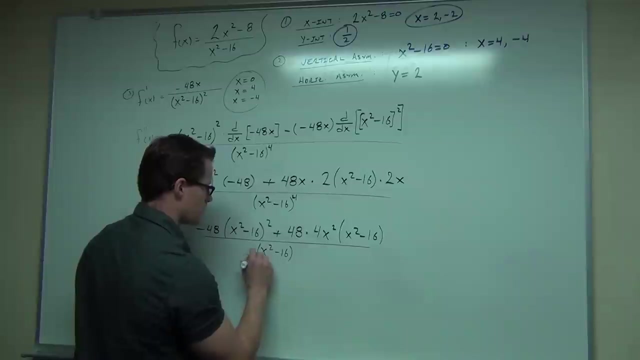 So hopefully you've seen what I've done. I've multiplied the 2x times the 2 and this x to make it 4x squared. I've leaving the 48 alone because I want you to see that factorization. It just makes things a little bit easier. 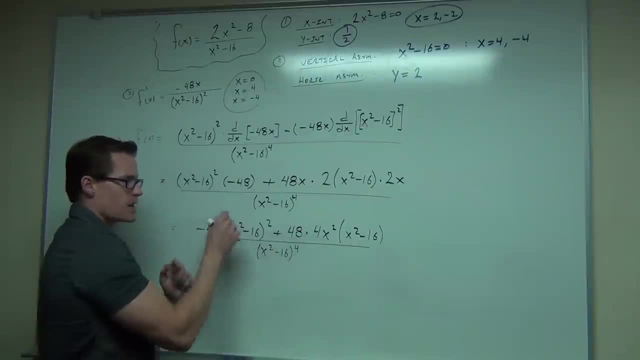 easier for us. so I'll be factoring out my 48 from right here. Also, I'll be factoring out x squared minus 16 from here, and one of them from right here. So what that's going to leave us with? be careful on your signs. check this out. 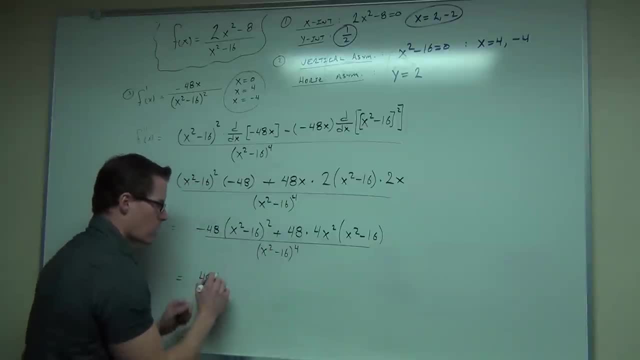 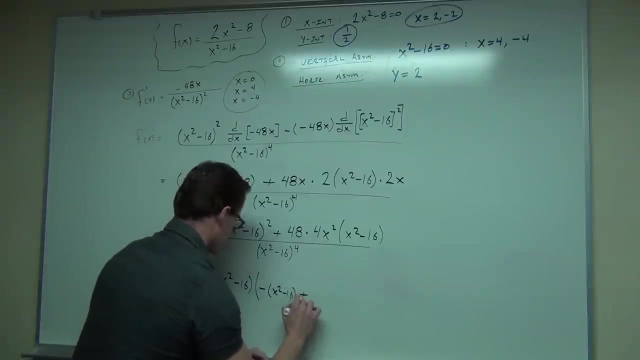 Factor out your 48.. Factor out one of your x squared minus 16s. What you're left with is negative: x squared minus 16.. Negative and one of those is remaining, Plus the 48 is gone. We have 4x squared. the x squared minus 16 is gone. 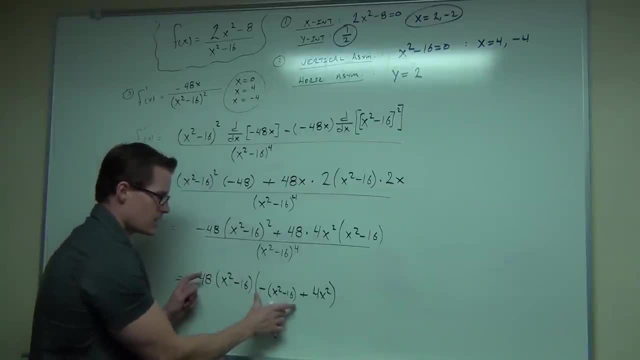 Check it with distribution if you really want to. but if you distribute this in, that's negative: 48x squared minus 16 squared plus 48 times 4x squared and then x squared minus 16.. So that's the correct factorization. 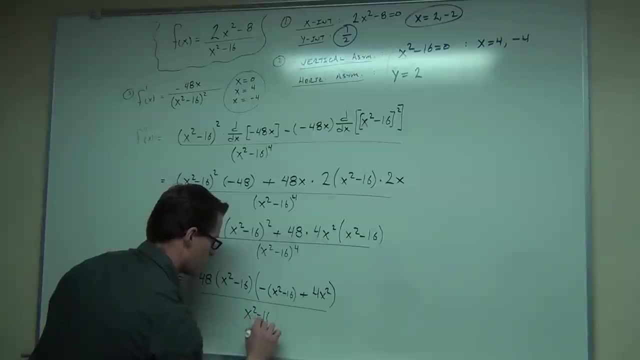 Almost done. One last little step. What we're going to do is simplify this a little bit. If you look at that, that's negative x squared plus 16 plus 4x squared, That's 3x squared plus 16.. 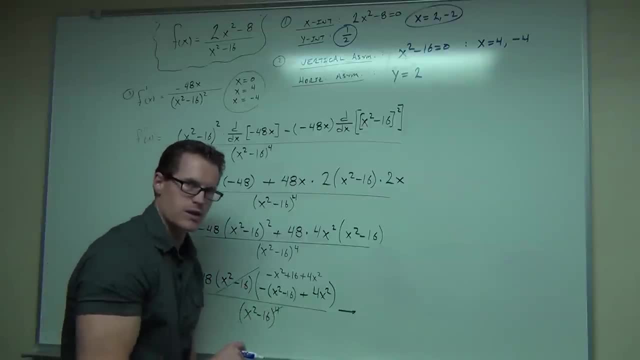 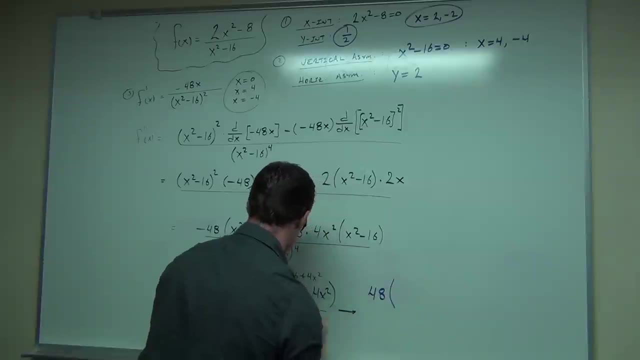 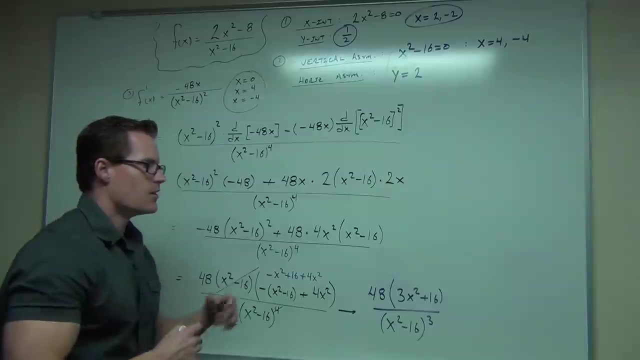 Also, we're going to simplify out One factor of x squared minus 16. So gone. part of that's gone. That's our second derivative. that's about as good as we can make it. Now. what the second derivative is? again, it's concavity. 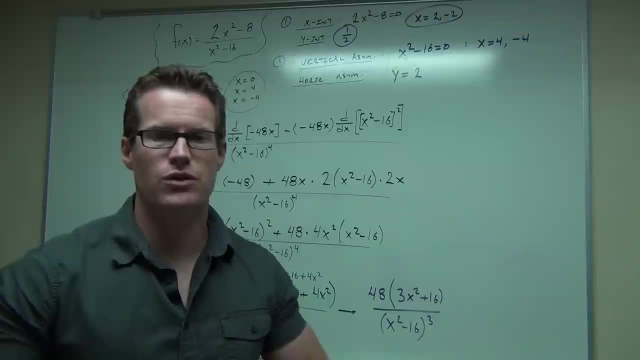 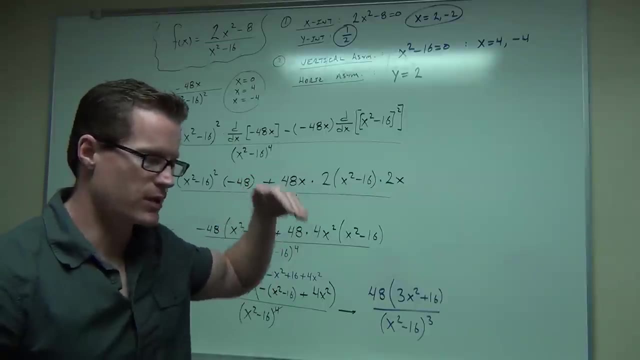 It's how your slope is changing, or in other words, the curvature of your graph, if you will. So, whether it's increasing or decreasing, we can have two different types of that. We can have increasing concave up, increasing concave down. 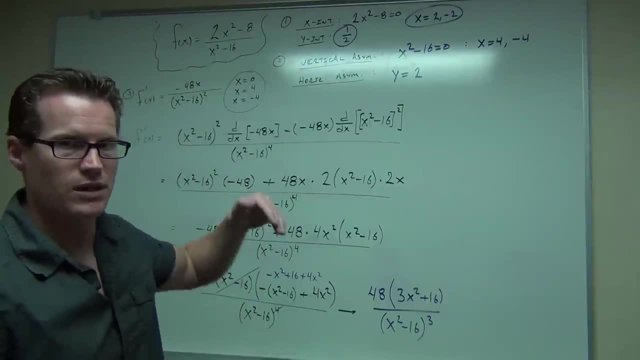 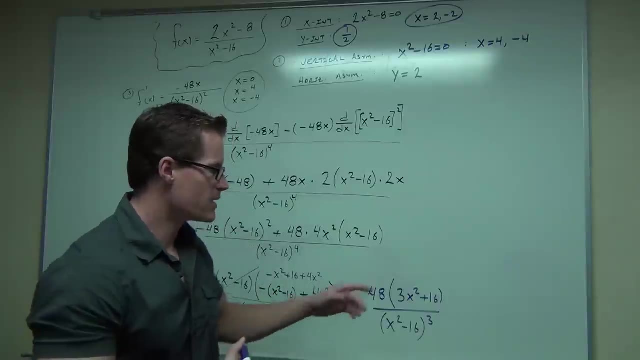 We can have decreasing concave up, We can have decreasing concave down, Just like that. So what this says is to find those points where you change, where you possibly can change concavity: Set your numerator equal to zero and your denominator equal to zero. 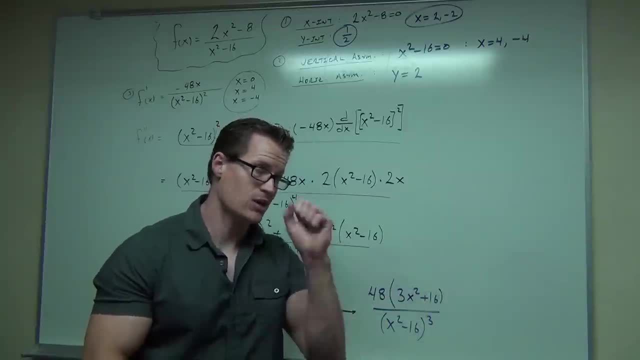 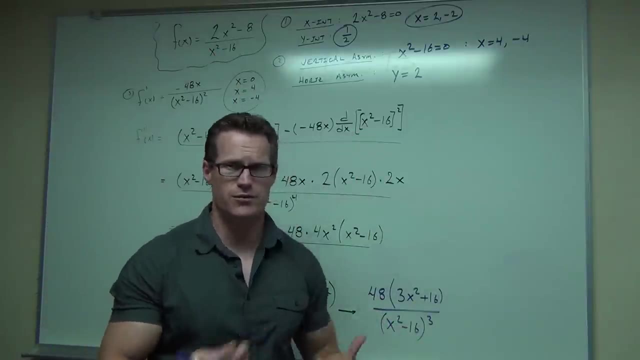 The numerator gives you the possible inflation, The denominator gives you the possible inflation. So either you plug in the reflection points like the actual numbers, the values, where you can plug them into the actual function and get a point The denominator says where the second derivative's undefined. 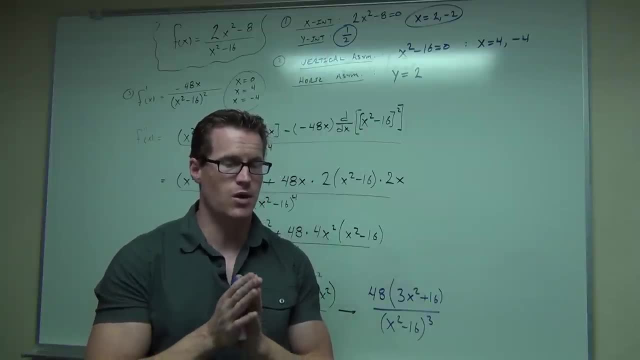 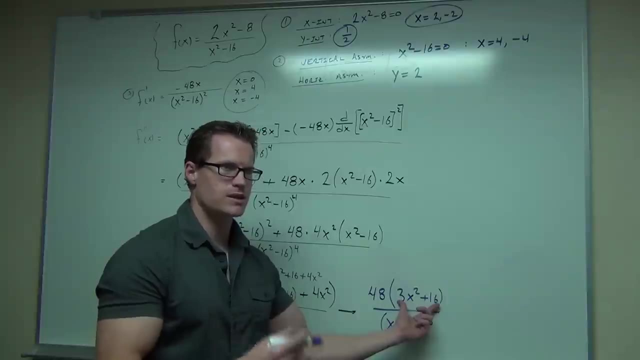 Well, it could still change concavity at those places, but you probably won't find a point because it's most likely an asymptote. So here, if you try this well, notice that 3x squared plus 16, is that ever going to be? is that ever going to work for you? 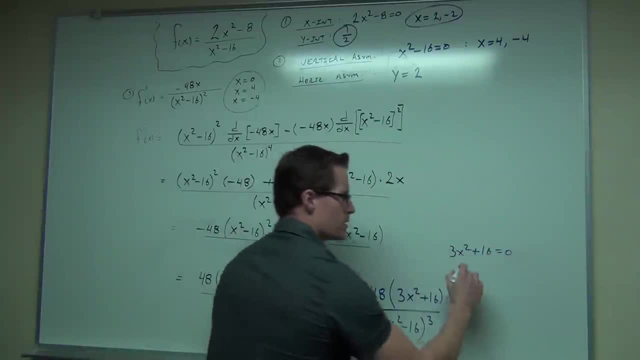 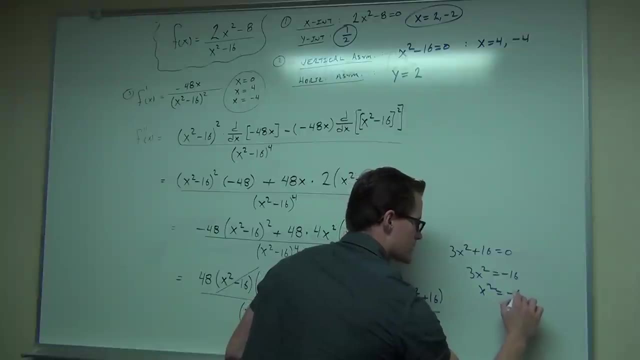 3x squared plus 16 equals zero. Well, 3x squared equals zero equals negative 16, x squared equals negative 16 over 3.. Can you have x squared equals negative? The answer is no, not in the real number system. 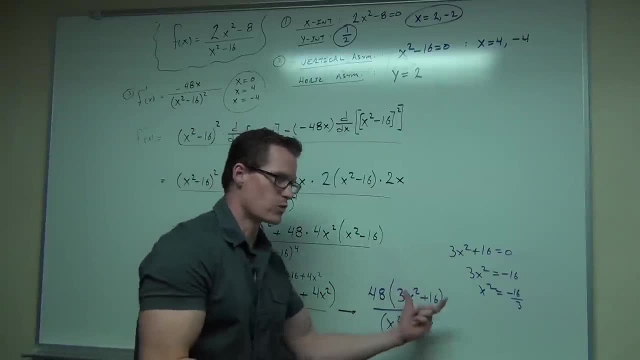 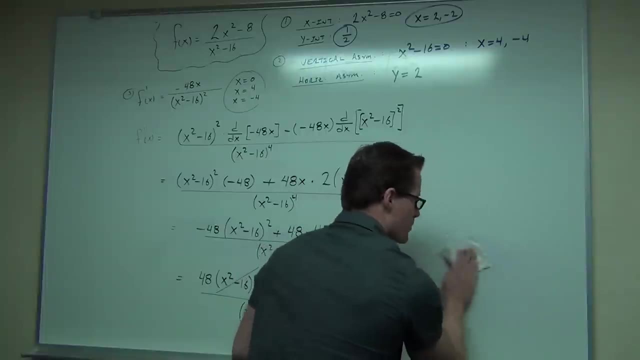 So here that's not going to give us any possible inflection points. So the numerator pretty much doesn't give us anything. The denominator you're going to see again. those same points keep popping up, Even from the beginning of our function. 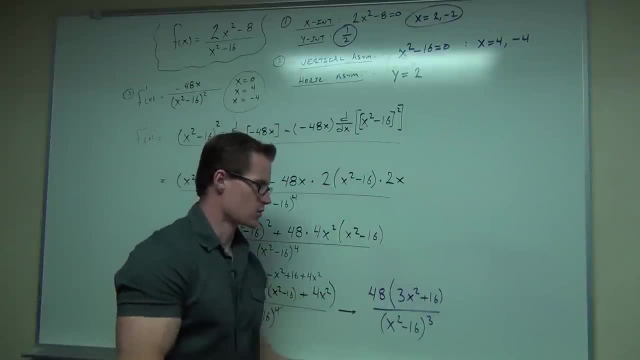 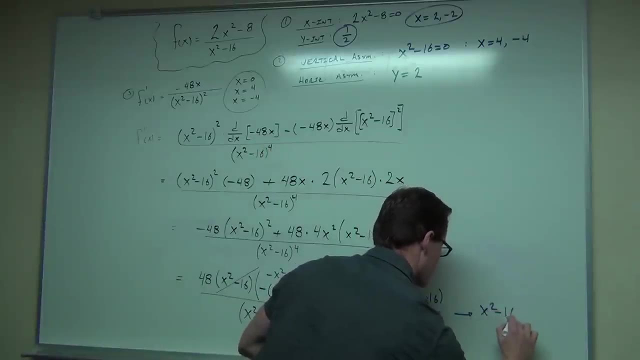 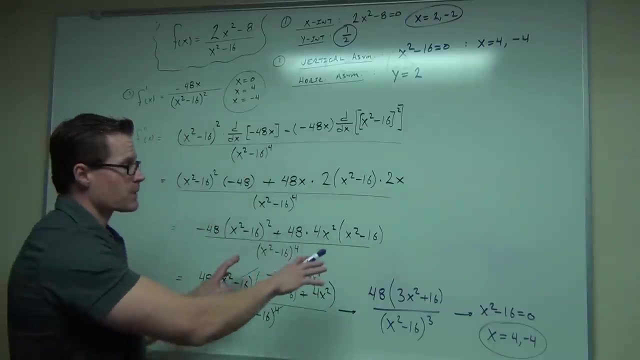 we had 4 and negative 4 as being undefined. That happens here as well. So again, we're going to have the points 4 and negative 4.. OK, again take a close look. That's our second derivative. all worked out for you. 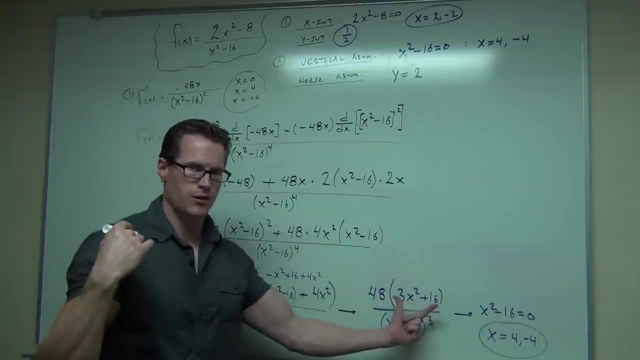 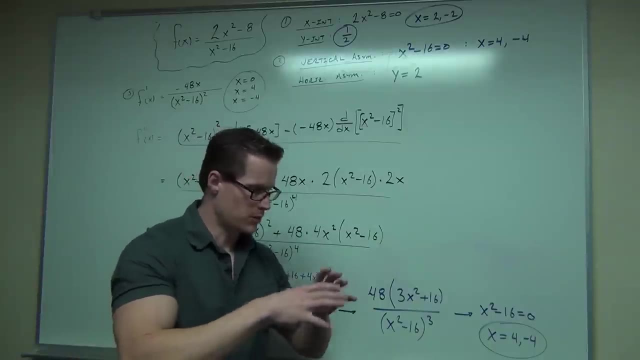 nice and pretty. Set equal to 0, numerator: nothing. Denominator: same points we've gotten before. I'm going to erase it and then we're going to talk about step number 5.. We'll plug all this stuff in. 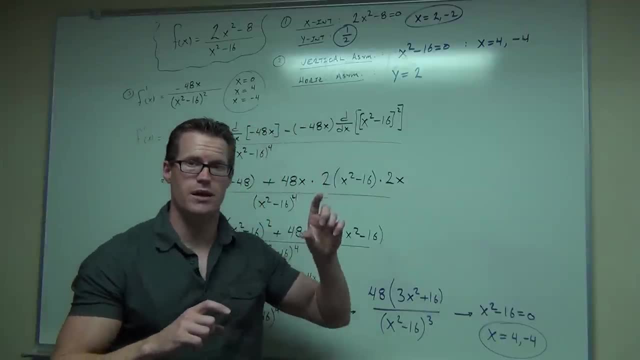 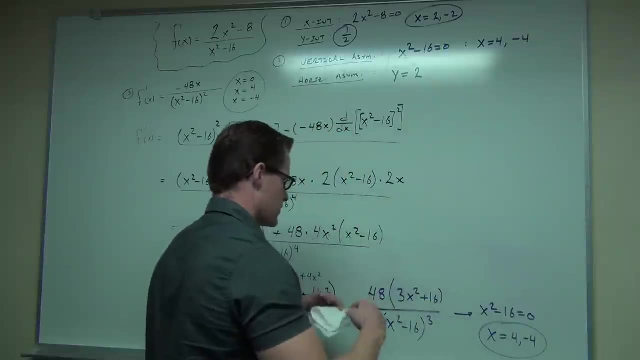 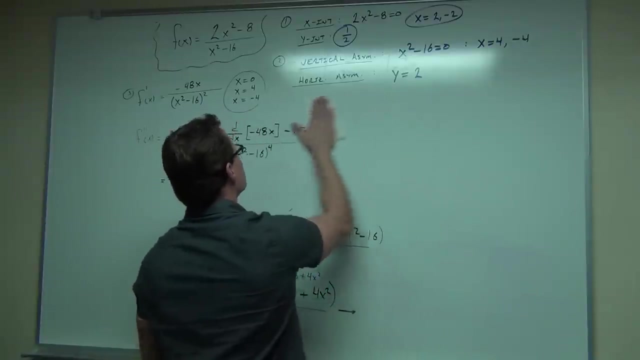 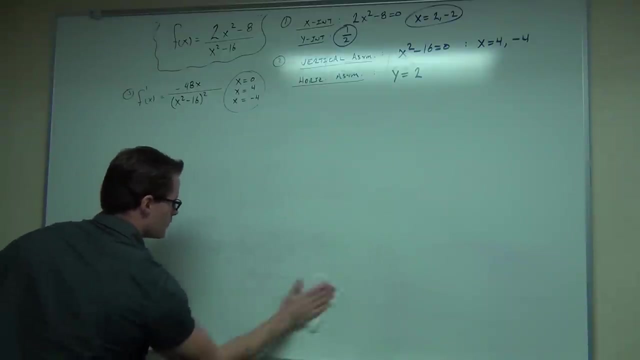 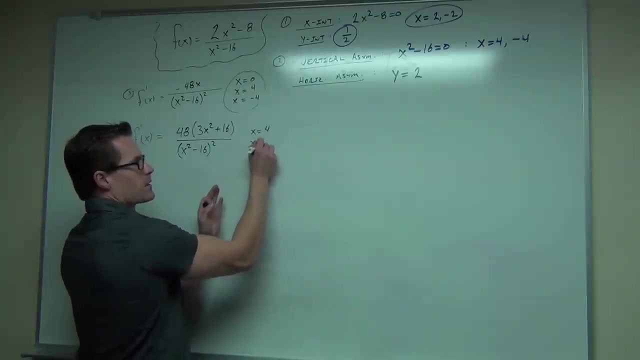 We'll make a nice table. We'll have the points from our original function in step number 6, and then I'll graph it, And what this gave us was 4 and negative 4 again. Now when we make the table. hopefully you remember this. 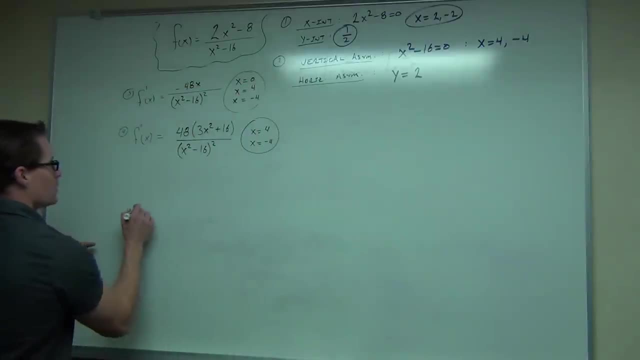 from class or from previous videos. if you're watching this on video, OK, So we're going to make a table. We're going to make a table, We're going to put our first derivative up top, second derivative on the bottom and basically gives us: 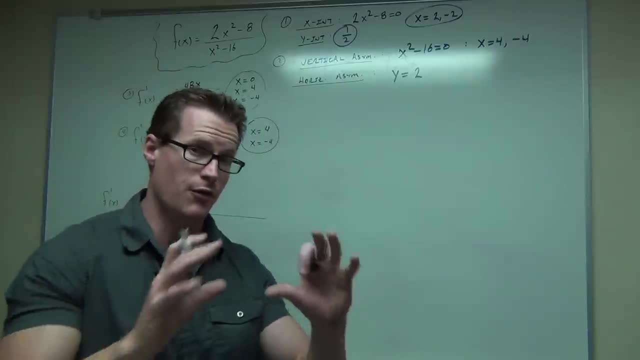 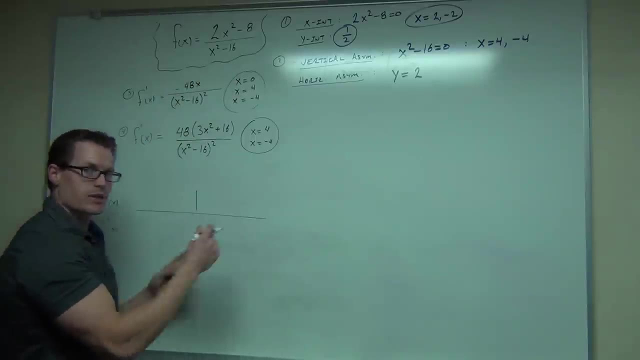 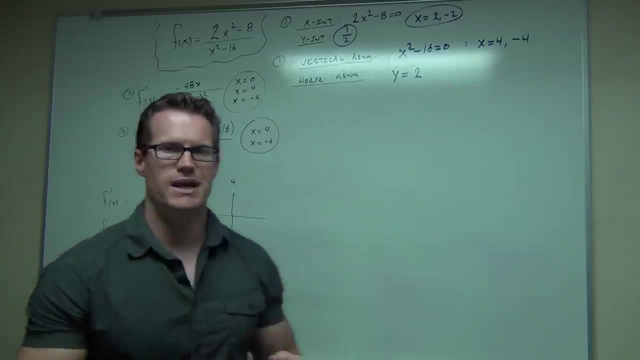 a kind of a concise version of our graph, of our function on a graph. So we're going to put all of these points on the top- got to be in order- and these points on the bottom, And what we do is we test specific points in each interval. 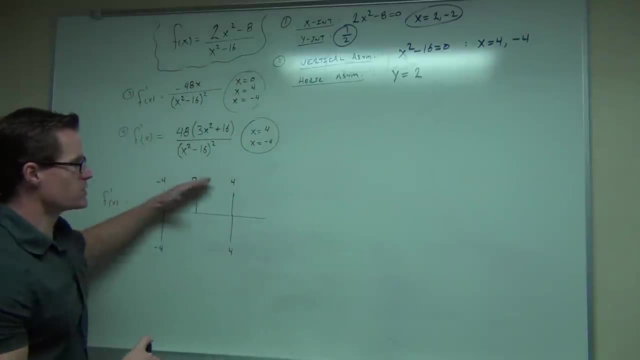 And what that's going to tell us is where our graph is increasing or decreasing from the top. That's our first derivative, or concavity for our second derivative. So I would test the points like negative 5, negative 1, 1,. 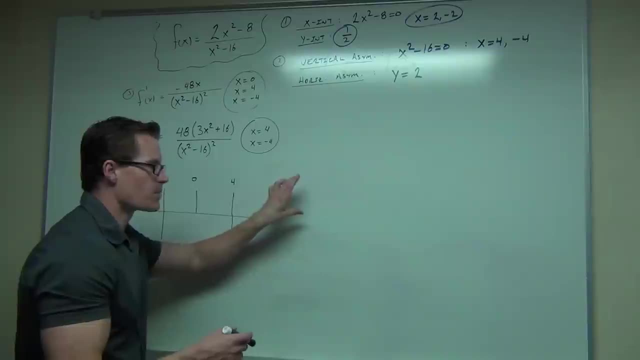 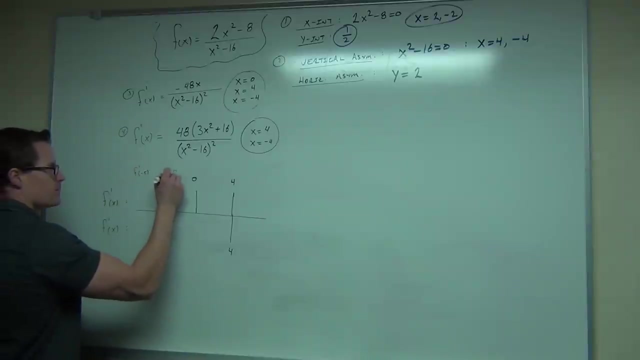 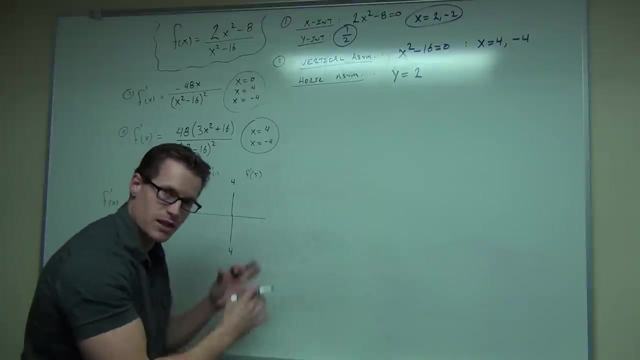 and 5.. And we're testing them in their respective derivatives. So here we'll be using the first derivative. On the bottom we're taking second derivative, so concavity, And we'll test some similar points, But make sure you put them in the second derivative. 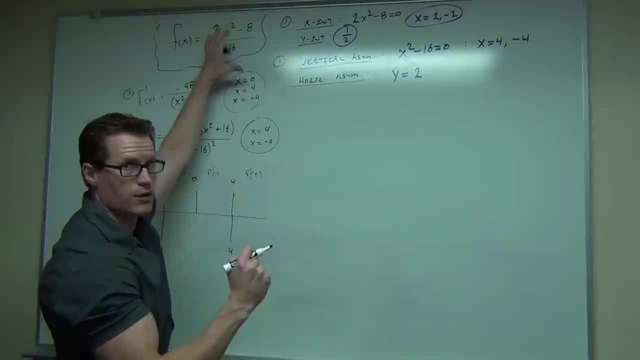 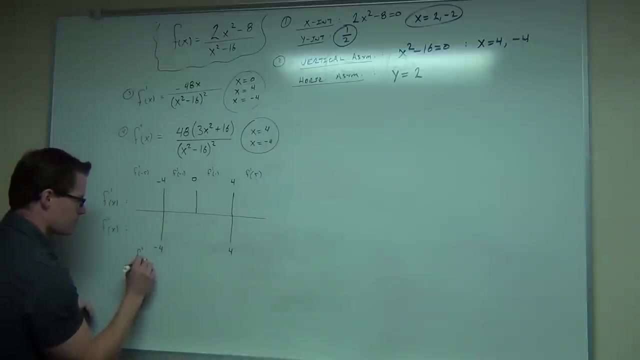 not the first, not the original. Original function gives you points on a graph. First derivative gives you increasing or decreasing. Second derivative gives you concavity. So let's try this. If you want to try it at home, plug in your own points. 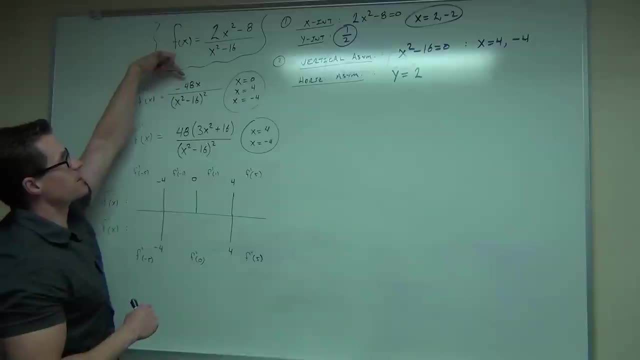 But we're going to try f prime of negative 5. That's a negative times a negative. This is our first derivative. Again, remember first derivative Negative times negative is a positive. That's a positive because it's squared. That means that this is positive. 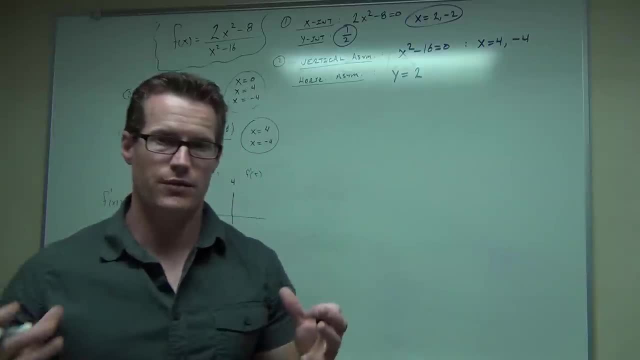 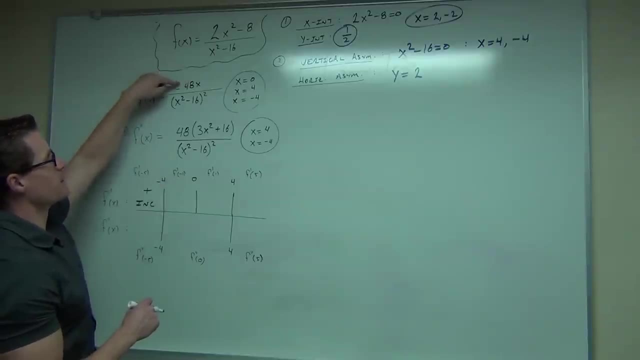 You don't exactly care about the whole value of it. You care whether it's positive or negative, Increasing Negative 1. Well, that says negative times. negative is a positive over a positive. Again, that is positive, Increasing. Next up we have 1.. 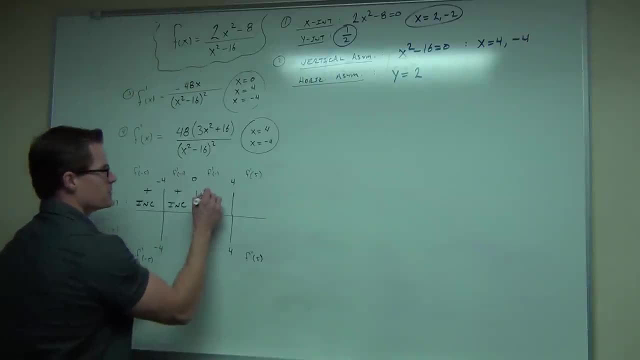 Negative times a positive is a negative over a positive. That's going to be a negative Decreasing. 5.. Negative times a positive is a negative over a positive. It's still a negative Decreasing. Second derivative is going to tell us some more things. 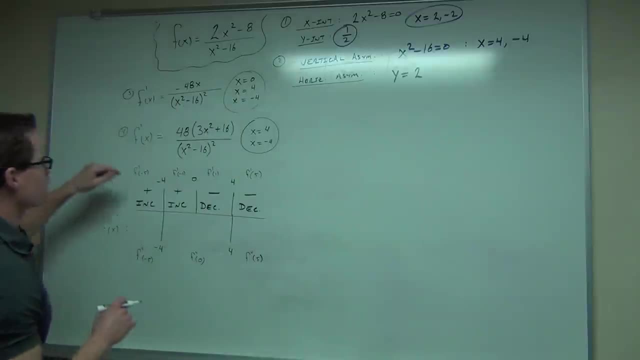 It'll say: plug in negative 5, but now do it to the second derivative. Second derivative is right here. This is well, let's see Negative 5 squared. well, that's going to be positive plus positive. Positive- oh, that's positive. 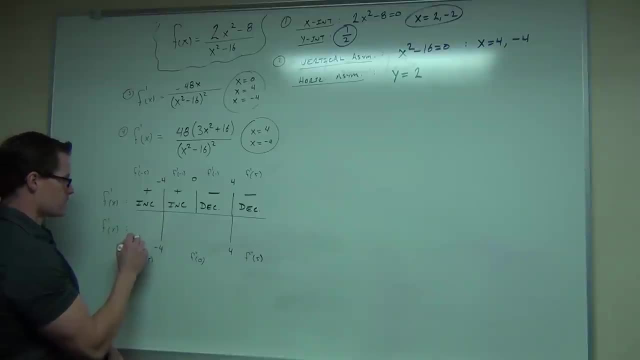 Negative 5. where is it? Negative? 2. Minus, 2. Positive sign of negative. 7. Positive sign of negative in the first. Negative sign of negative in the second. Negative sign of negative 7. Oh, you know what I made a mistake? I think I drew that wrong. 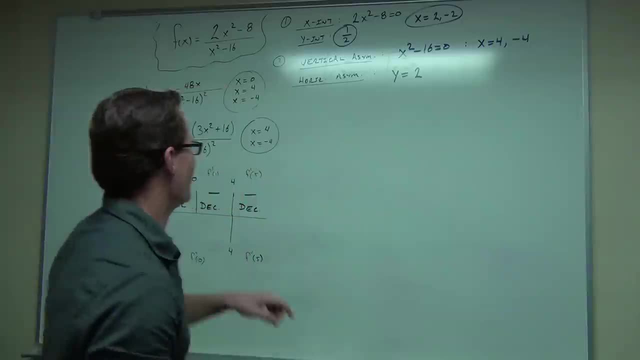 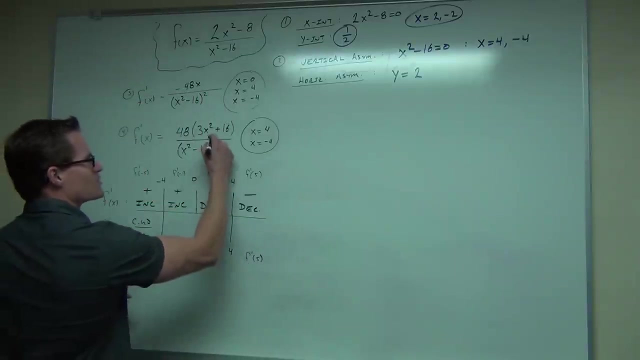 If you were watching at home, you might have noticed that. What's Mr Leonard thinking? That should be a power 3.. I was kind of thinking through that, thinking: wait a second, that doesn't make too much sense, So let me change it to a positive 3, and then we're going to check this point again. 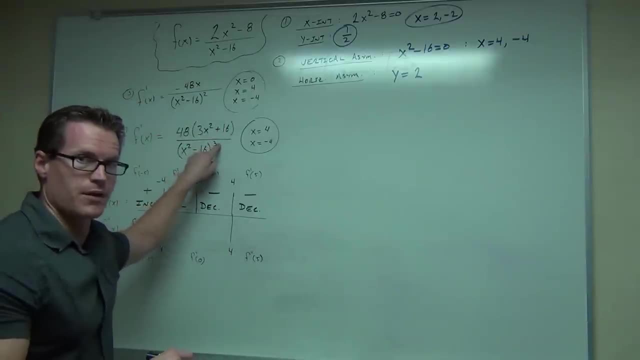 I think that one's going to work out for us, but make sure you have a 3 right there, because that would be a big mistake. I forgot to erase it before I copied it down, so bad mistake on my part. Let's check it one more time. 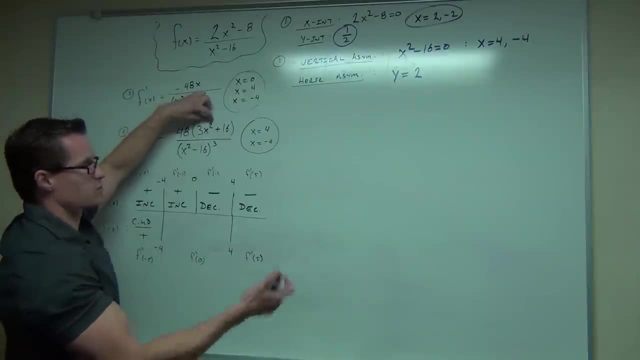 Let's check the negative 5.. So negative 5 squared: well, that's positive Times. the 3 is positive. Plus 16 is still positive Times 48, that's positive. Now let's check it down here. We have negative 5 squared, that's 25.. 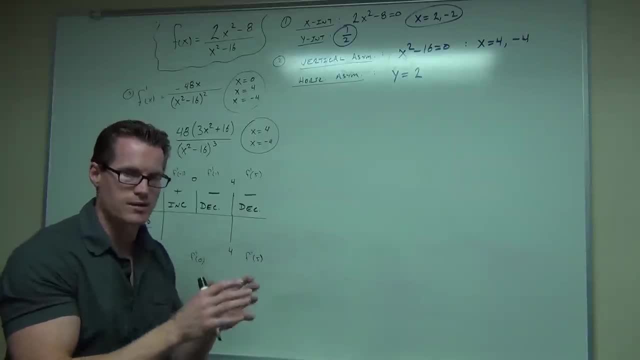 Minus 16,. well, that's still positive. and when you cube it it'll still be positive. So we're okay on the concave up, It's still going to be concave up. This is the one that's going to be changing for us. 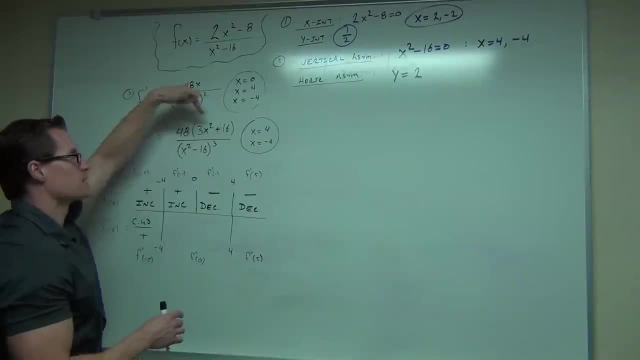 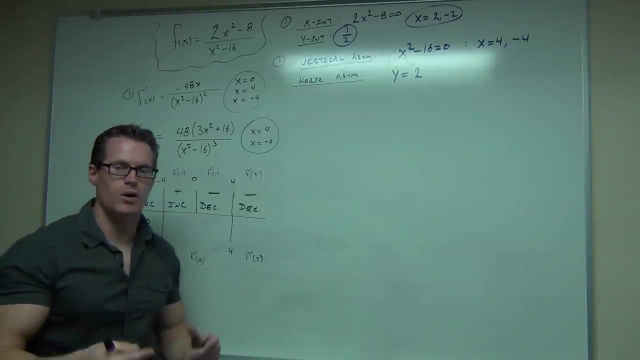 If we plug in 0, well, that's 16 times a positive number. It's still positive. but look what happens down here: 0 squared is 0.. Minus 16, well, that's a negative. What happens when you cube a negative? 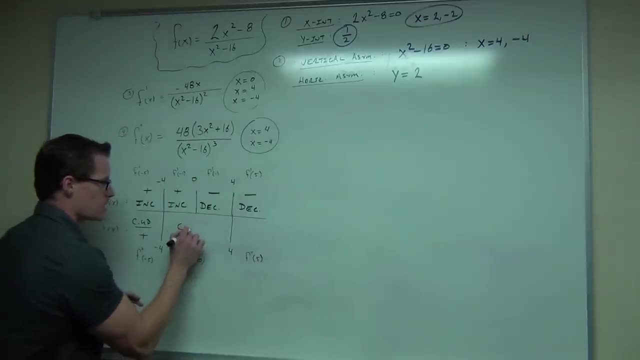 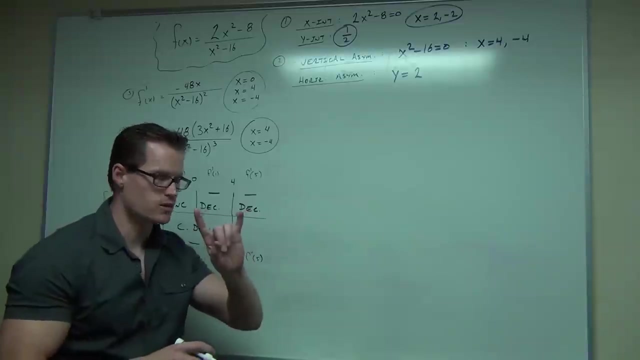 Well, it's still a negative. So this is going to be concave down And it's concave down for its entirety. Notice how we didn't get that 0 in our second derivative, so that's not going to be a place where we're changing concavity. 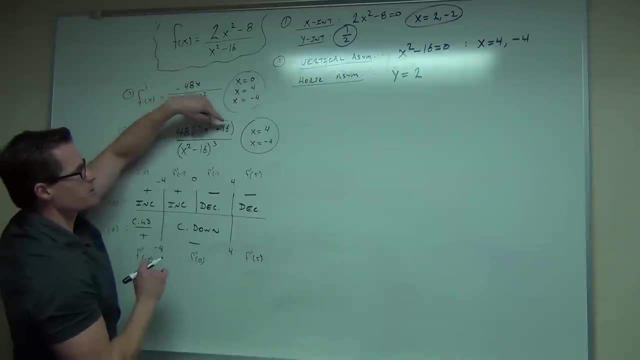 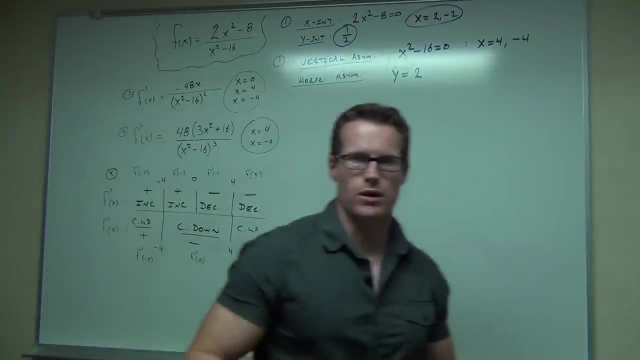 5, same thing's going to happen as negative 5.. We're going to have a positive up here. We're going to have a positive down there. That's concave up. Well, that takes care of step number 5 for us. 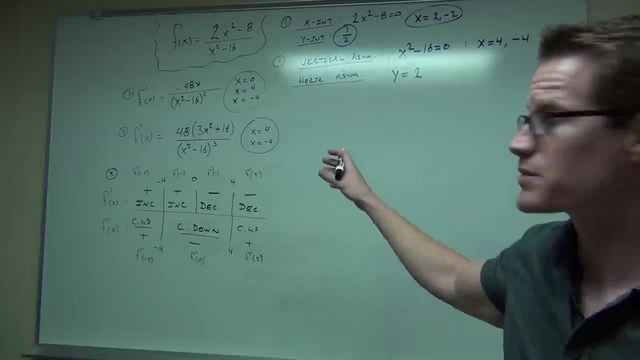 So so far, we've found our x-intercepts, our y-intercepts, We've gone ahead and done our first derivative and our second derivative. We've made up our table. We have all of our intervals of increasing, We have decreasing. 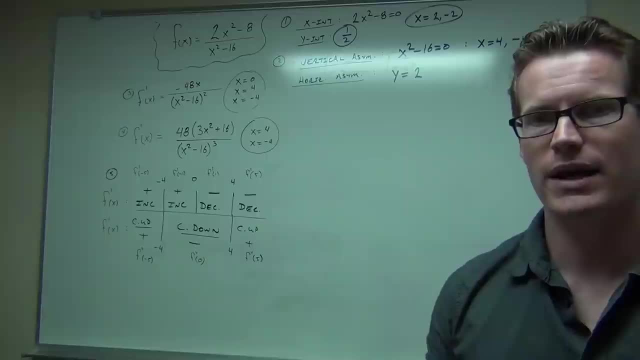 We've got concavity up there. We're almost done. What we need to do right now is find out some points, what our points are, plot them on our graph and look at how this is going to be graphed for us. 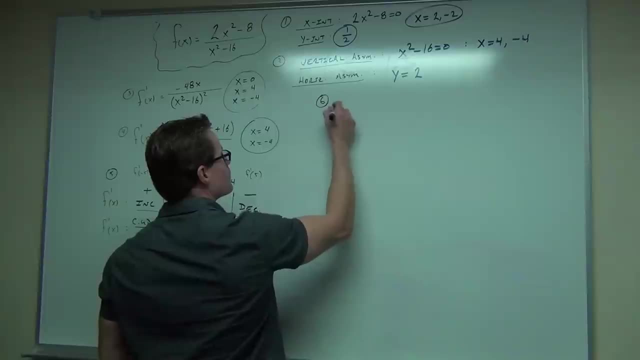 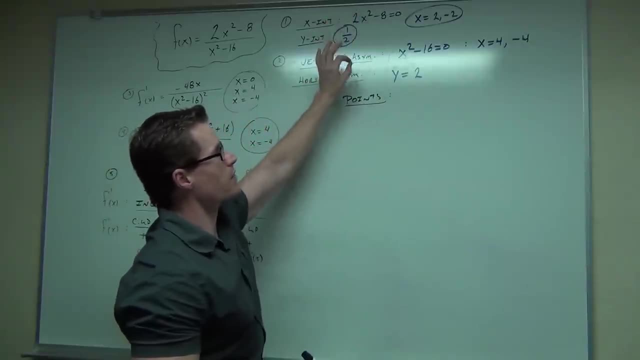 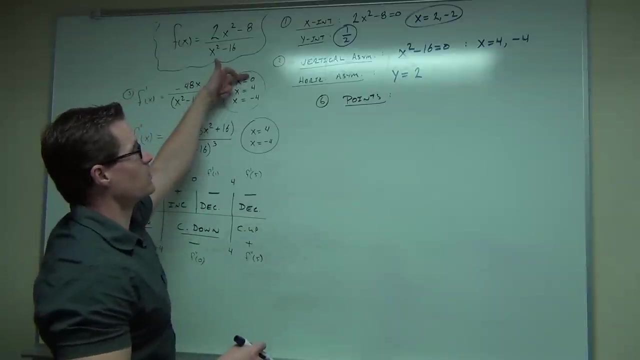 Well, our points are already on the board. We have our x-intercepts, we have our y-intercepts and we have our asymptotes. You're going to notice that all those points come back again at us. We have 0.. 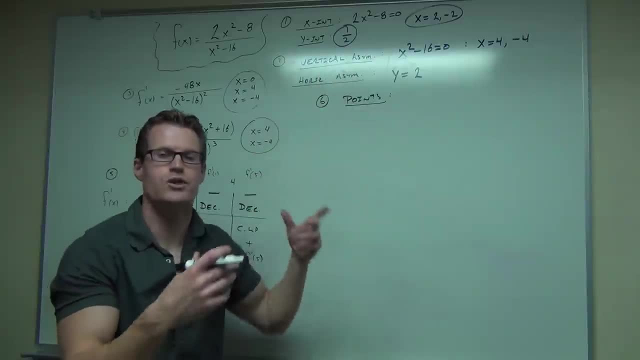 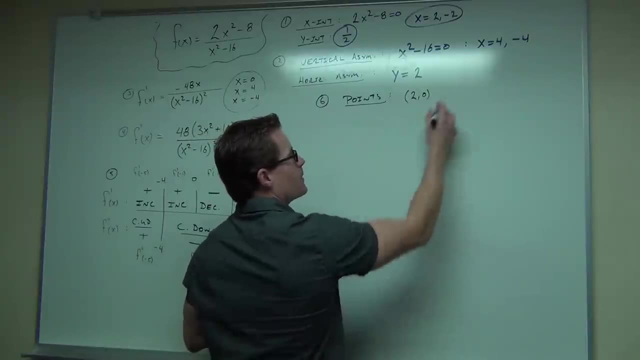 Well, if we plug in 0, you get 1 half. That was our y-intercept. So all of our points are basically listed. We've got 2, 0.. Negative 2, 0.. Those are our x-intercepts. 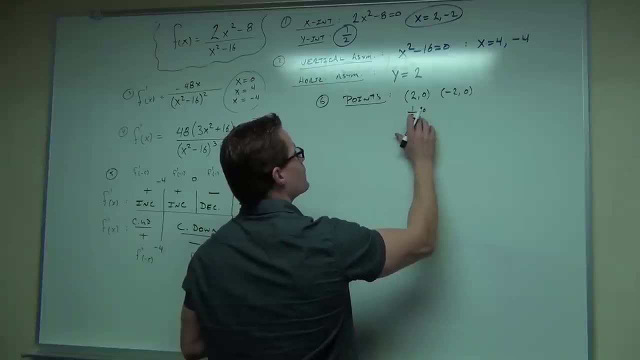 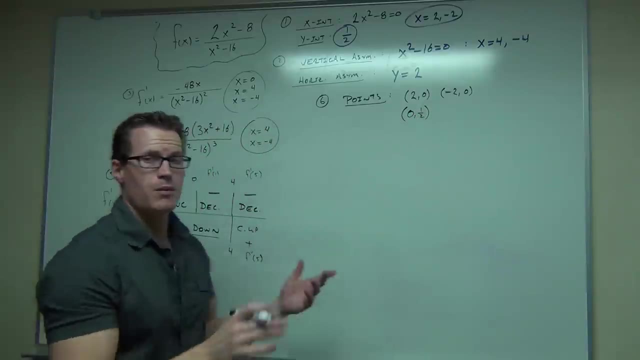 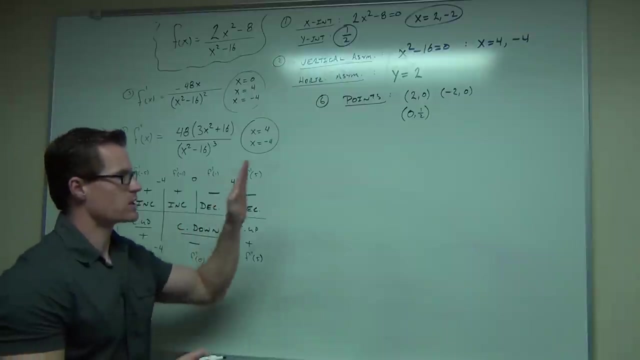 We've got 0, 1 half. Keep in mind what that is, though. That's our y-intercept, and it's also, if you look at it, it's also this which is increasing to decreasing, increasing to decreasing. 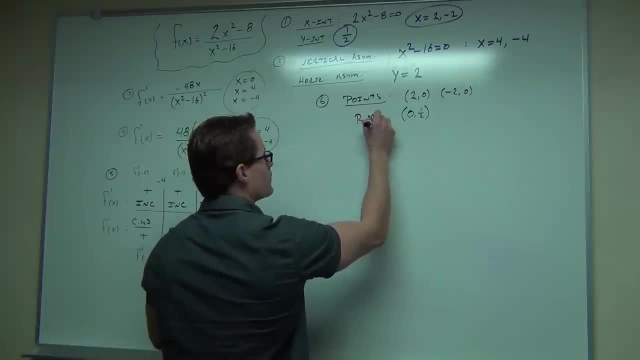 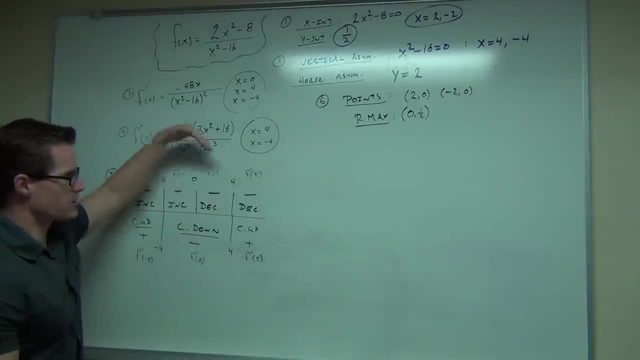 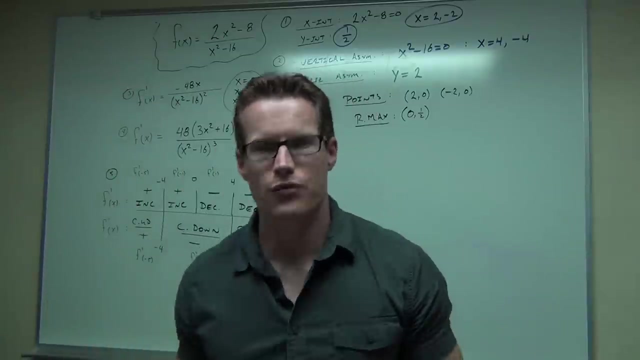 Is there a relative min? No, This says increasing, increasing, decreasing, decreasing. There's no way we're having a relative min here. It doesn't happen. Also, inflection points. We could try for inflection points. We could try for some of these points, but you'll see. 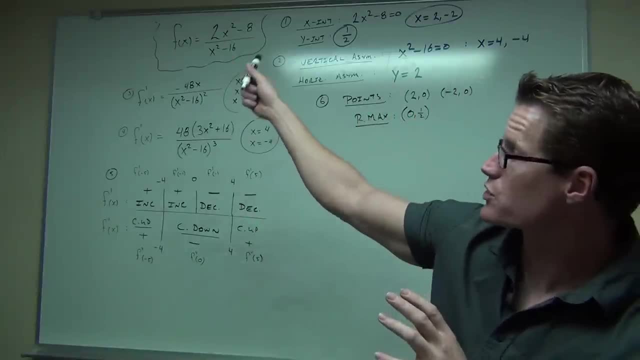 when you plug them in, plug them into your original function. you've got 4 squared minus 16.. You've got negative 4 squared minus 16.. That's undefined. That's how we got those asymptotes in the first place. 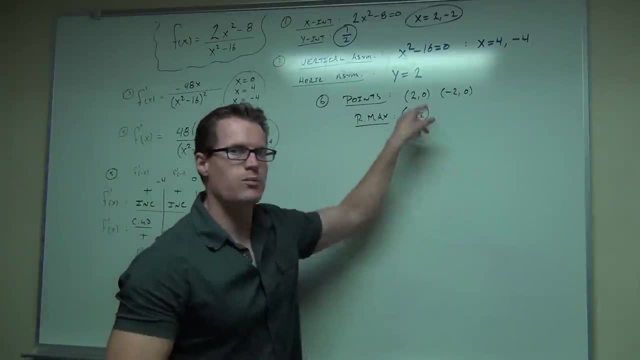 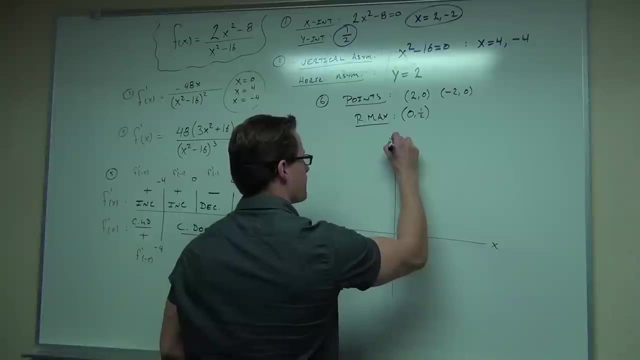 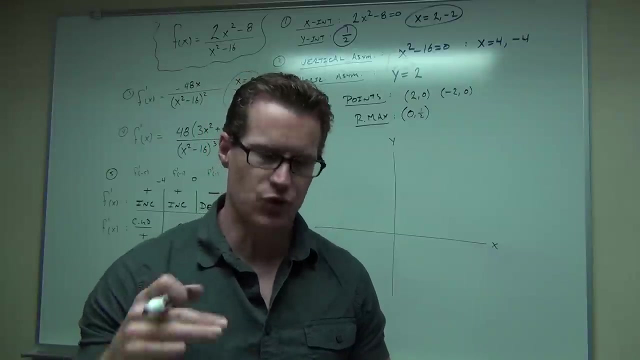 So these things are all asymptotes. What it means is we only have 3 points to graph Now. I told you in class around the video that a lot of times you can actually graph these graphs just by looking at the asymptotes and increasing, decreasing. 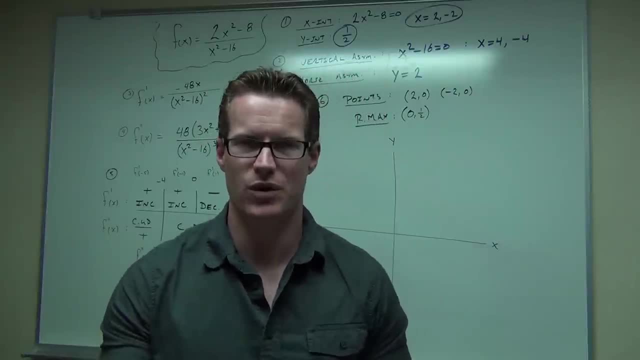 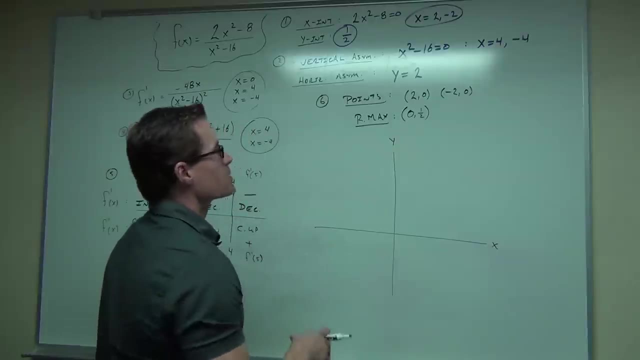 I'm going to try to show you that right here so that you can kind of visualize what it's going to be, even without the second derivative sometimes. So if that's what you're looking for, this is the part that you want. So, number 1, do your asymptotes. 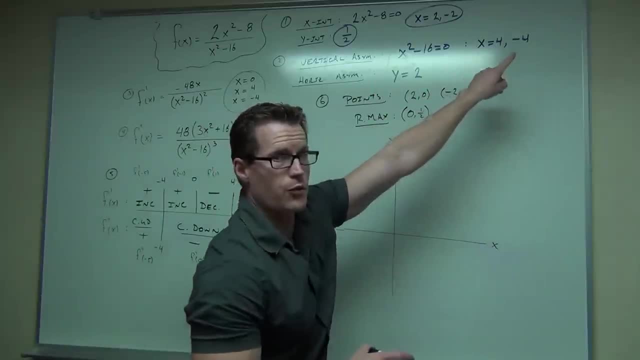 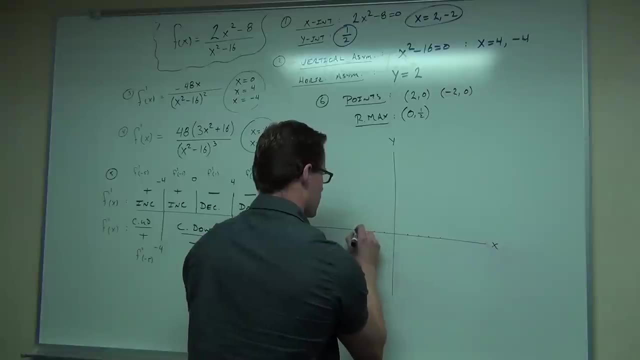 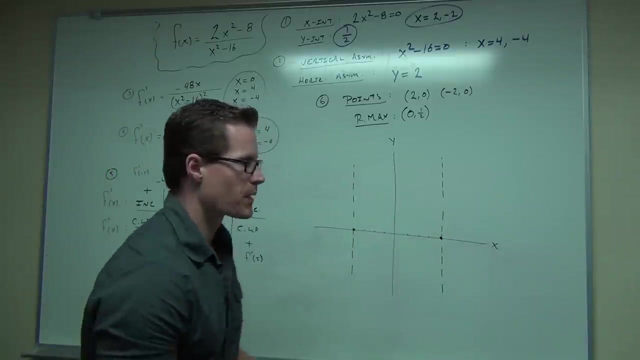 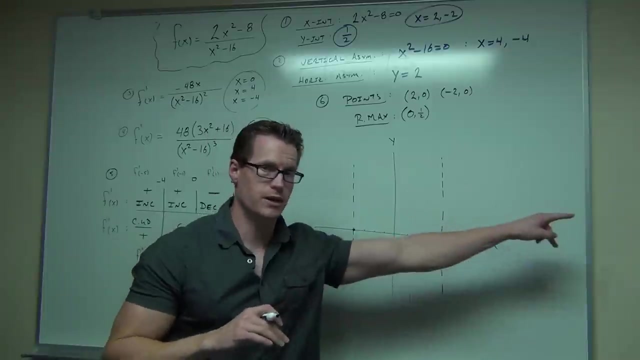 Asymptotes are vertical, 4, negative, 4. Hopefully you're okay with our asymptotes. Horizontal says 2. In each direction. Now keep in mind: horizontal asymptotes only work as you're going to infinities. 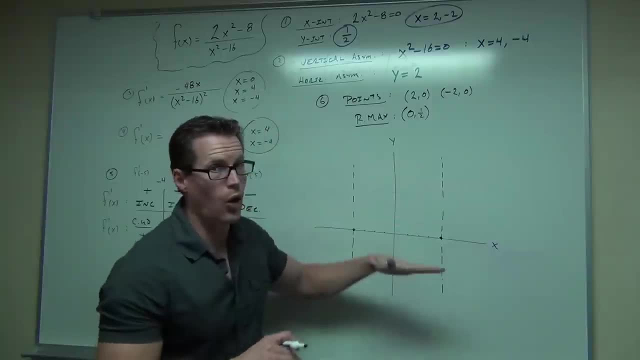 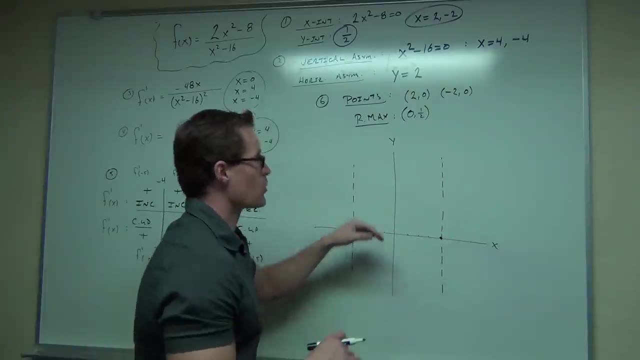 So could you cross it here? You could. It doesn't mean it's like a wall for you. Well, it's a wall for the y, yeah, for our vertical, But a horizontal not necessarily. So horizontal says 2 in both directions. 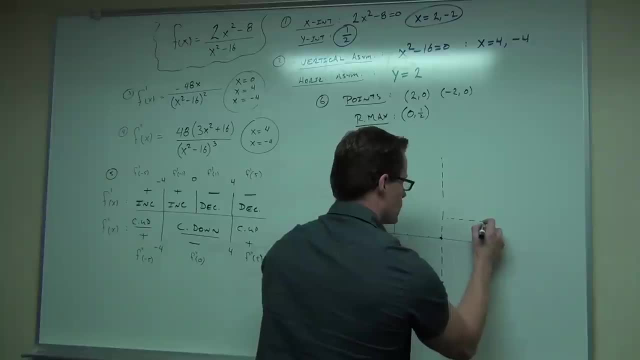 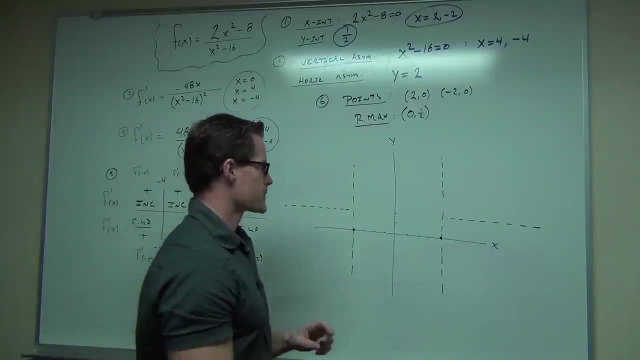 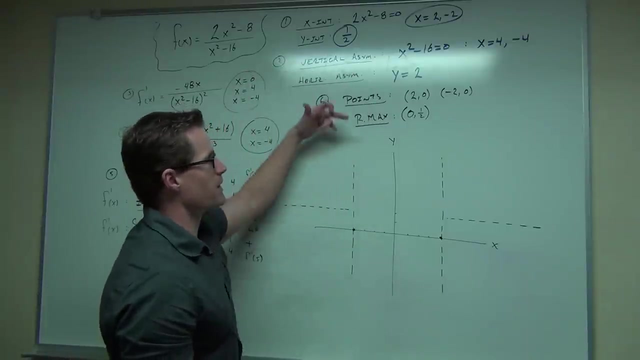 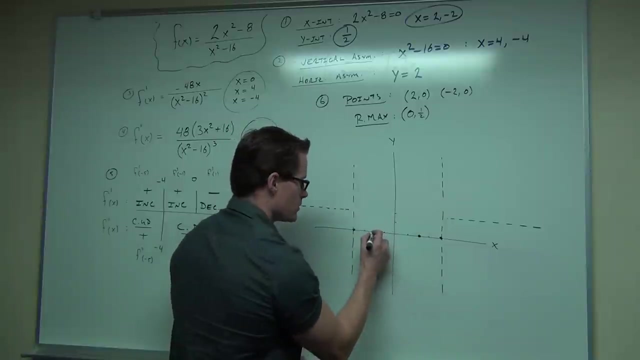 But it only starts out here. The next thing you do, after you take care of your asymptotes in your graph, you're going to plot all of your intercepts. So our intercept says 2, 0, negative, 2, 0, and 0, 1, half. 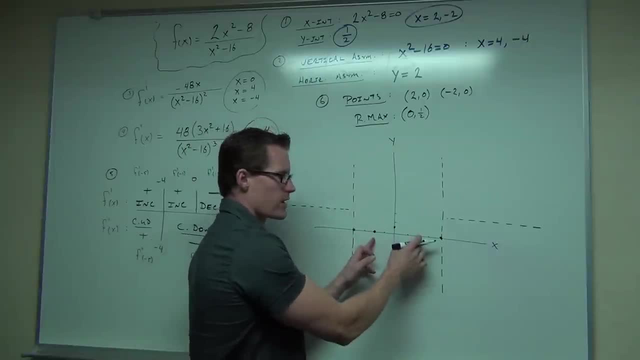 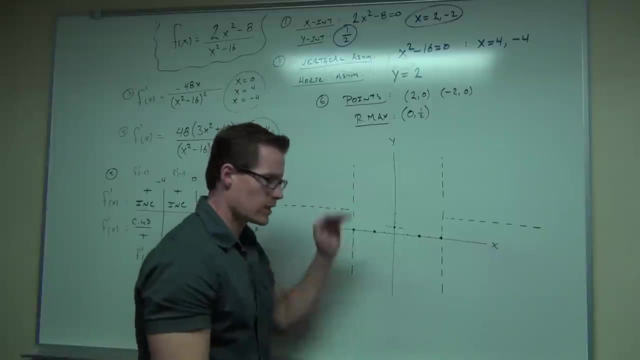 We're going to label what they are too. I've showed you that when you label these points well, they're intercepts. Those don't do much for us. besides, say, you cross the x-axis here, But that said, you have to be a relative. 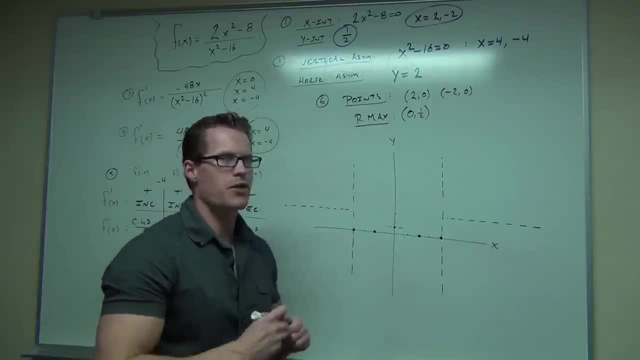 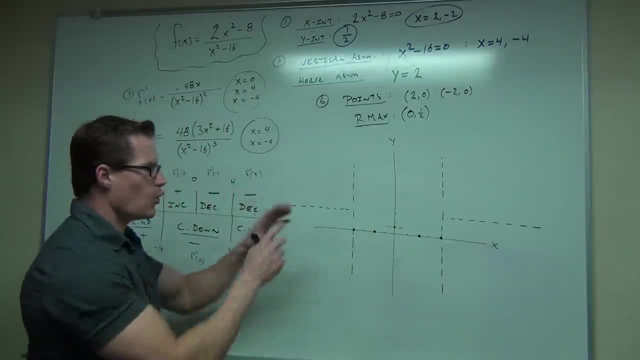 that's what that said. we listed it as Now. just think about it, Even if you don't have the second derivative. so let's just pretend I didn't even do the second derivative. What's the only way we could fit this information on this graph. 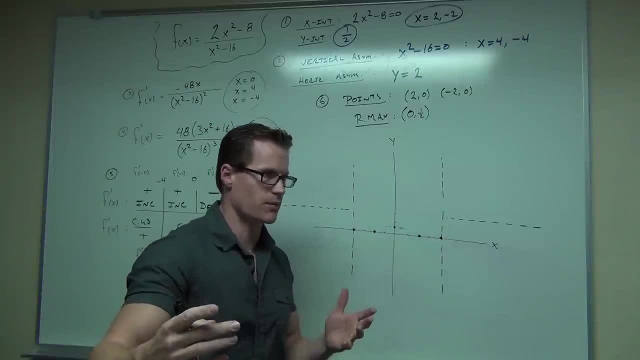 with just the first derivative. So hint hint on that test. if you're looking at how do I do the graph with just the first derivative, Sometimes you can do it. This is one of those cases. Sometimes you can't, You need the second derivative. 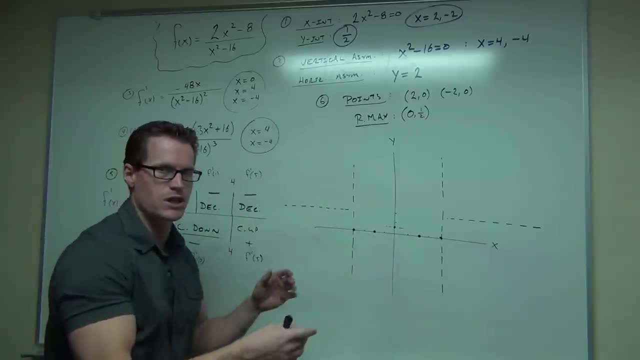 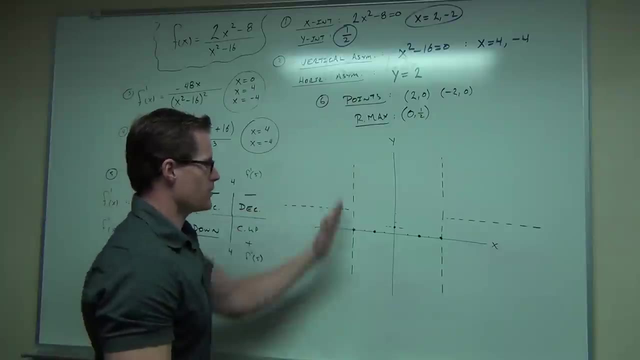 But a lot of times, if you have asymptotes, and you have increasing and decreasing, you can picture what this graph looks like. Here's what I mean. This is what I'm expecting from you If you know that your asymptote goes this way and this way. 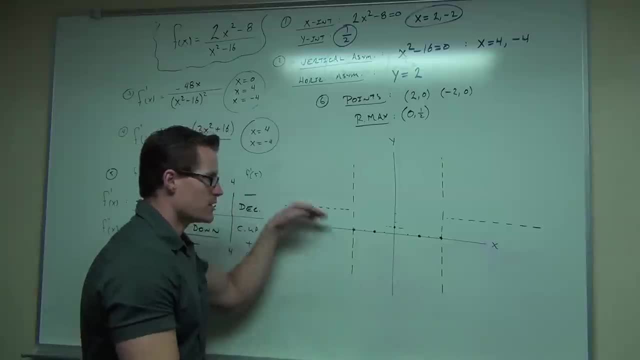 there's only two scenarios. You're either going and you don't have any relative max or min. notice you don't have any of those in this interval. You don't have any of those in this interval. You do have one in this interval. 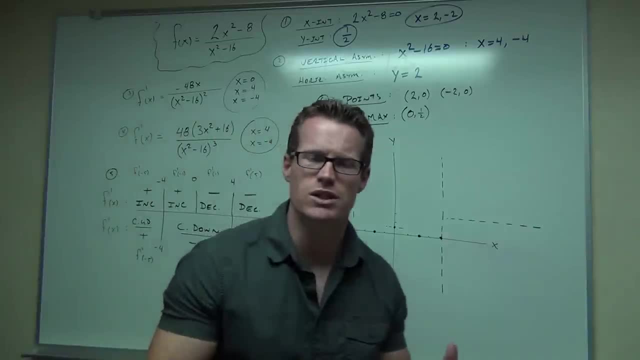 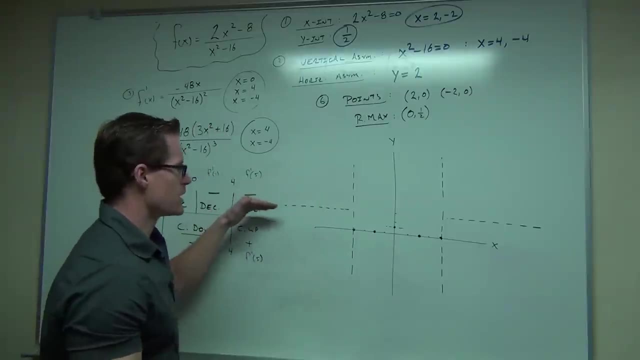 But other than that, there's no change in increasing, There's no change in decreasing. So, unlike the previous example, we can't do things like this, Otherwise we'd have relative max. We can't do things like this, Otherwise we'd have a relative min. 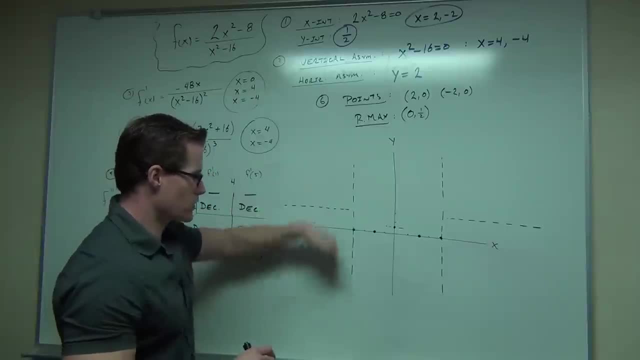 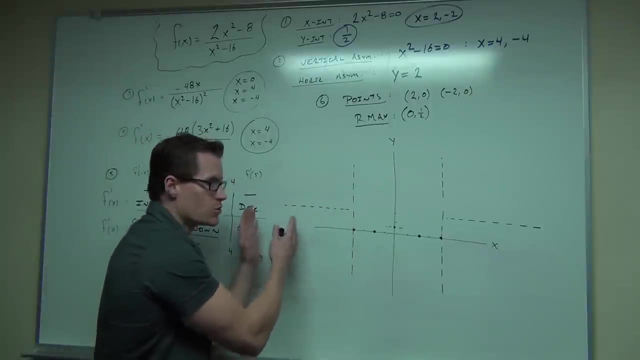 It's either going to be up or down, That's it. It's the only thing we can have. So when you look at it, if there's no relative maxes or mins, there's no change in increasing or decreasing. look at the first two intervals. 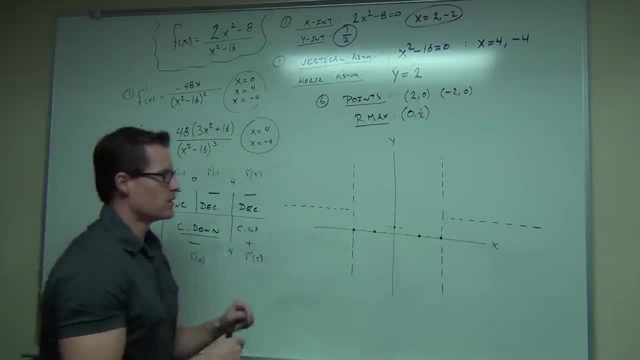 It says you are increasing all the way to zero. You're increasing all the way. So, from negative 4, that's where we're really looking- From negative infinity, to negative 4, you're increasing. Can this be increasing? No, No. 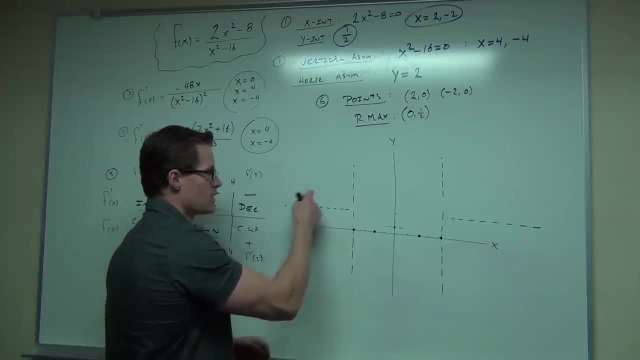 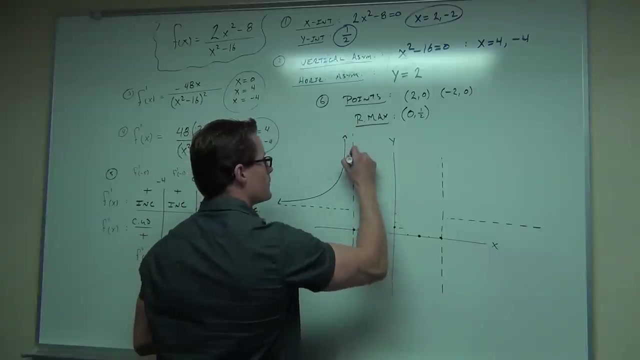 That was a mistake. That would be decreasing. Increasing says this way. So to fit this on a graph: if you have a horizontal asymptote and a vertical asymptote, that's the only way it can be. That's it Now. what about this section? 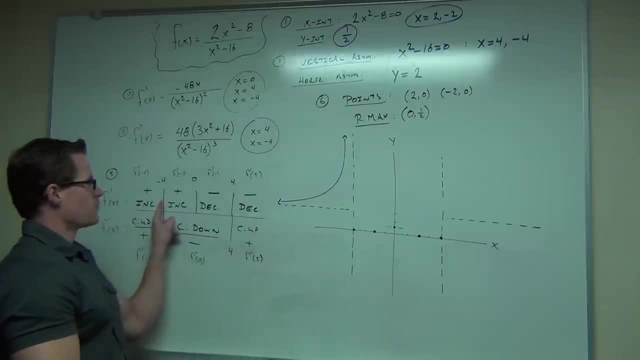 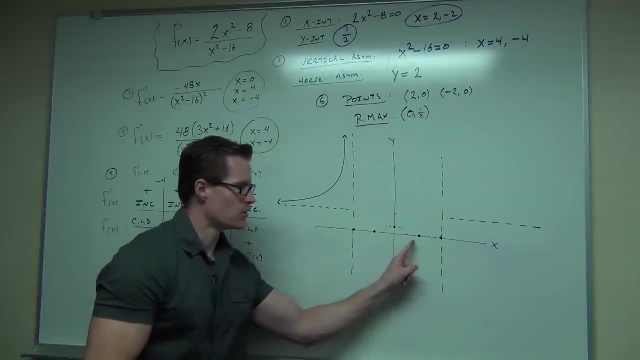 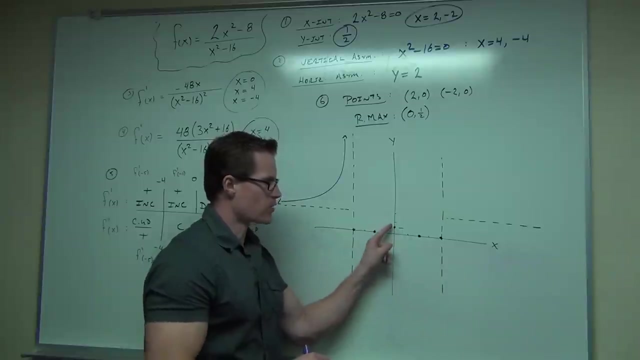 This section says you're increasing from negative 4 to zero. You're increasing from negative 4 to zero And then you're decreasing from zero to 4.. Well, what's the only way that you can increase and then decrease and have one relative maximum and touch these two points? 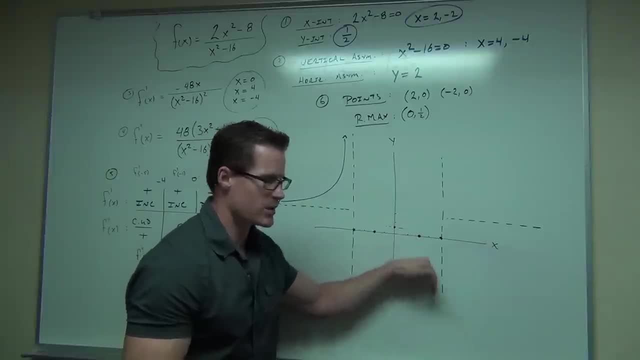 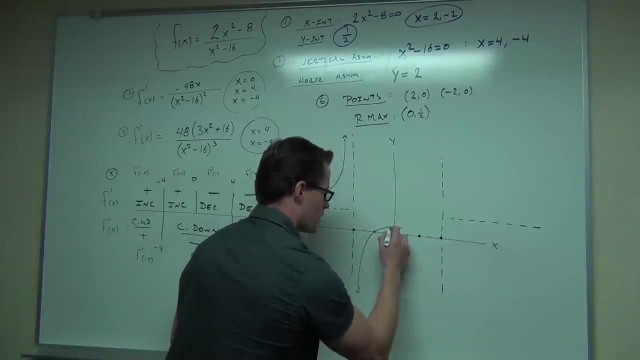 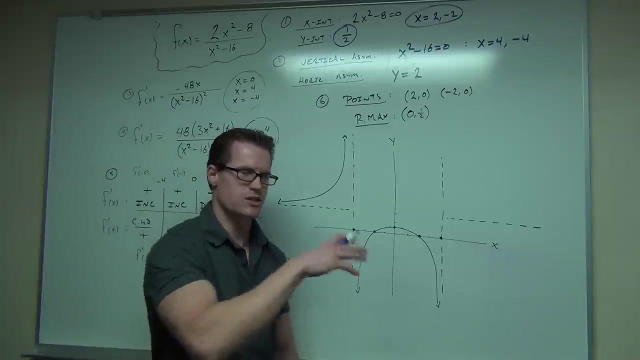 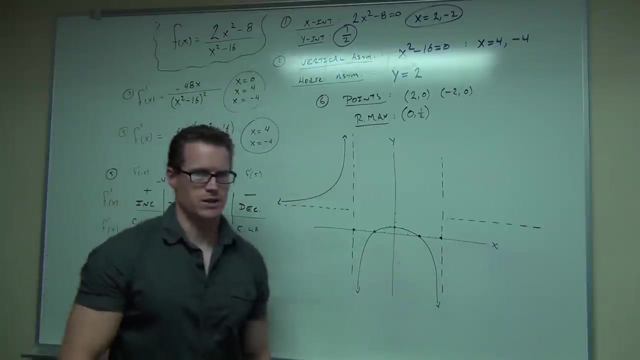 The only way it could possibly look is going up and coming down. That's it. I'll talk about concavity in a minute minute. just want you to see the idea of fitting your graph to asymptotes first. now, after positive 4, it says you're decreasing, decreasing, mind you like this? 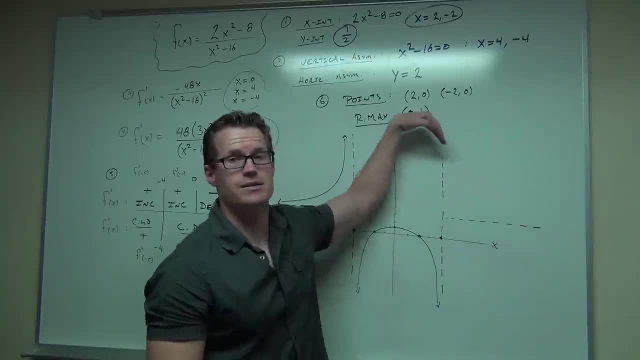 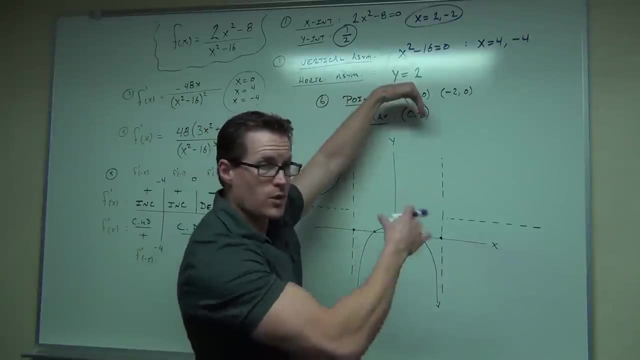 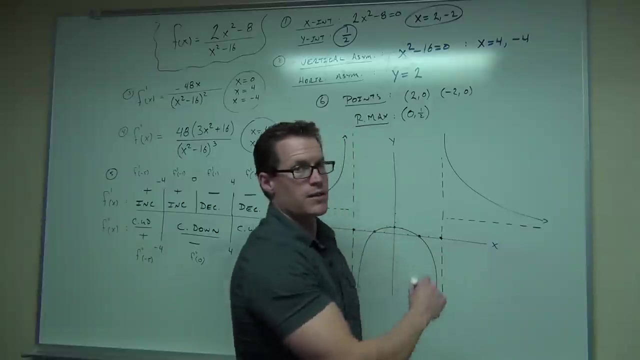 now that would be increasing like this: yes, that is decreasing. there's no relative max, no relative min. that means you're decreasing throughout, means you have to go from left to right downward. the only way you're going to fit this asymptote- and this asymptote is with a picture like that. 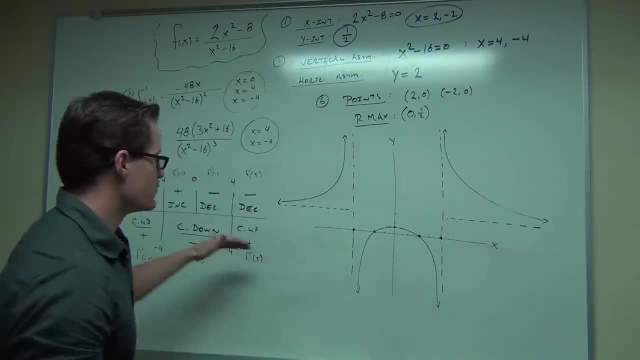 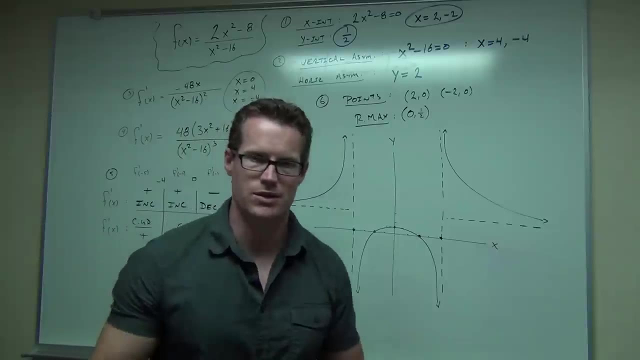 now I have gone ahead and done the second derivative for you and I gave you the table as well. if you want to go that far, that's fine. in fact, most times you really should. I'm just trying to get you to think outside the box here. but if you, 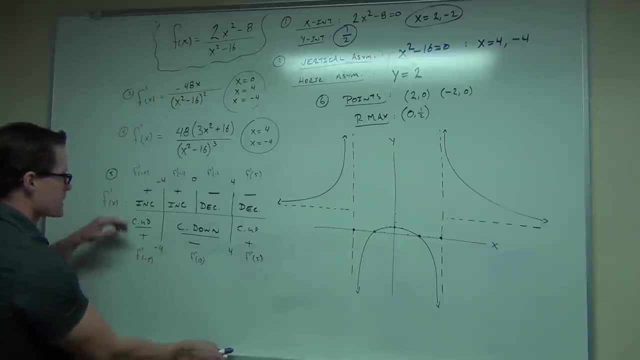 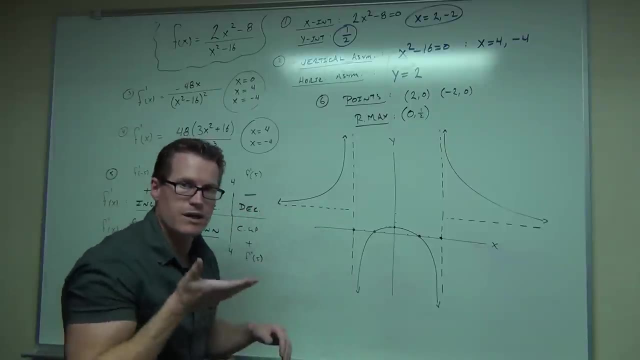 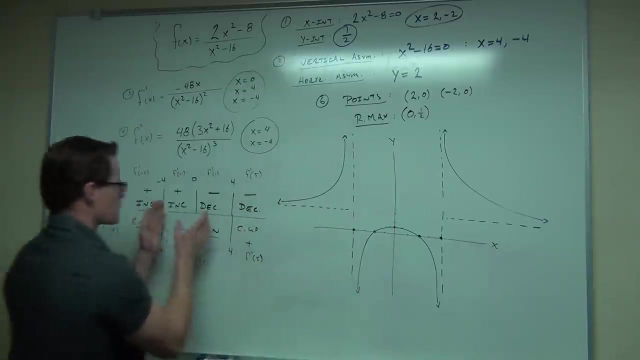 if you compare the concavity with this, let's see if it works. it says you're increasing and your concave up all the way from negative infinity to negative 4. increasing and concave up looks like this: that's what we have. increasing concave up then on this interval from negative 4 to 0. that's here says you're. 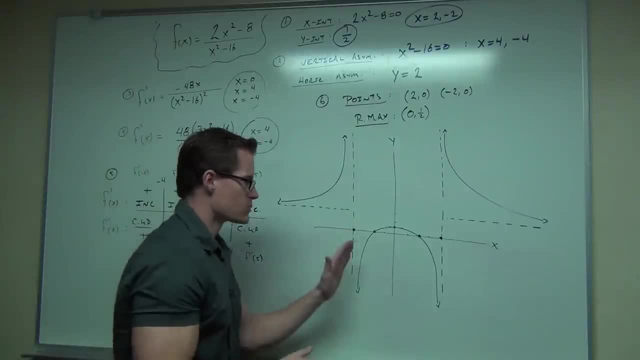 increasing, but you're concave down. well, look at that: if you have these asymptotes increasing, concave down. that's exactly what we did and we fit it to our points: negative: 2, 0 and 0, 1 half. we had to do that from 0 to 4. you're. 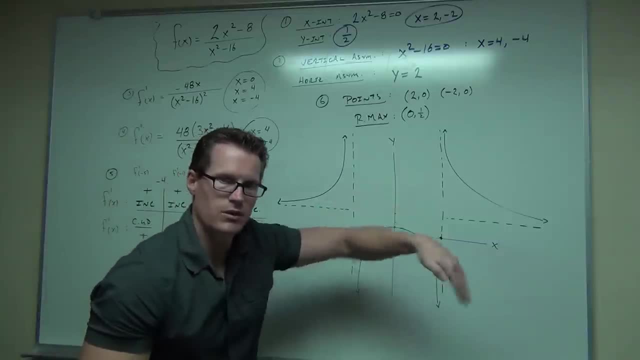 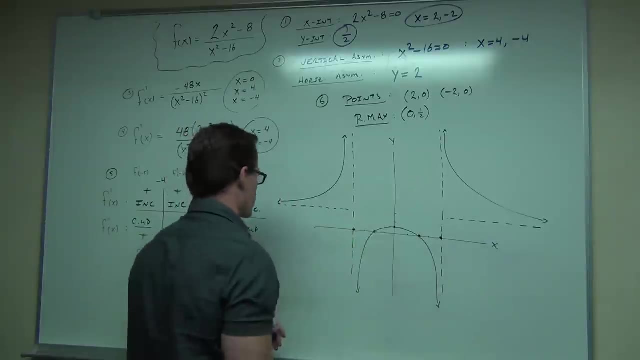 decreasing and you're concave down. decreasing concave down looks like this: so from here we're decreasing 0 to 4, you're decreasing and you're concave down: 0 to 4 and concave down. hey, that works. last section: from 4 onwards we're. 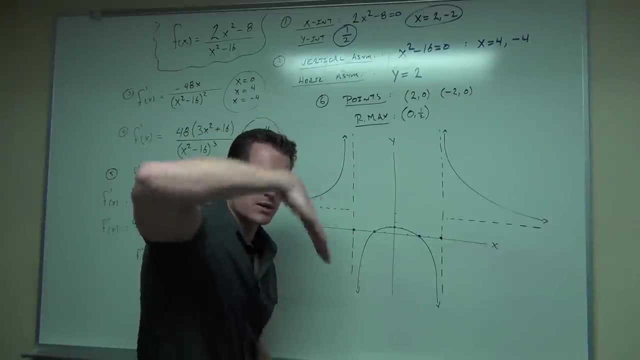 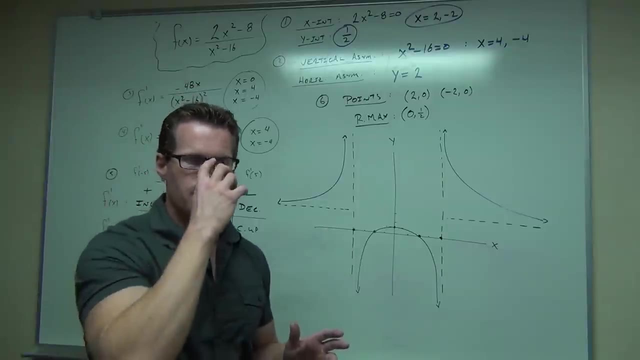 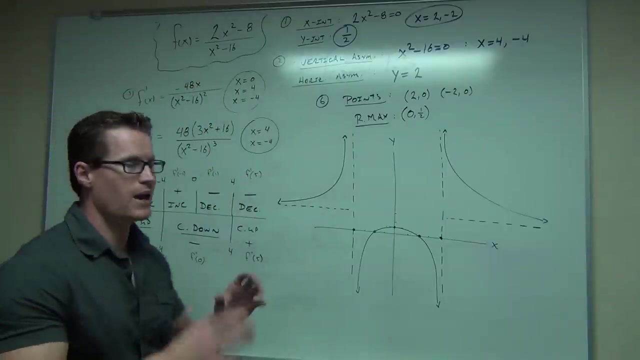 decreasing and we're concave up, decreasing concave up. looks like that decreasing concave. we got it. that's our graph. do all seven steps, you have your picture. but sometimes, with these rational function, if you, if you have those asymptotes handy, you can sometimes take your first derivative and just look. 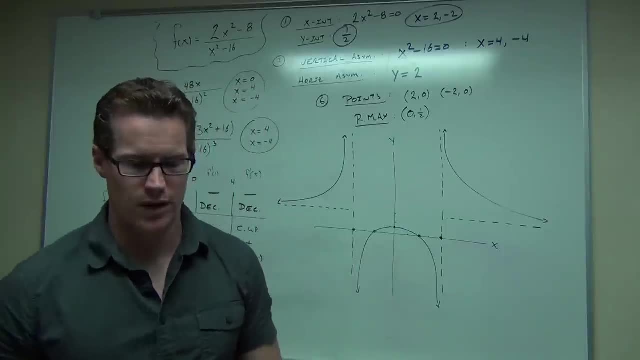 at that graph and put it in the right places, and the concavity does work out for you. 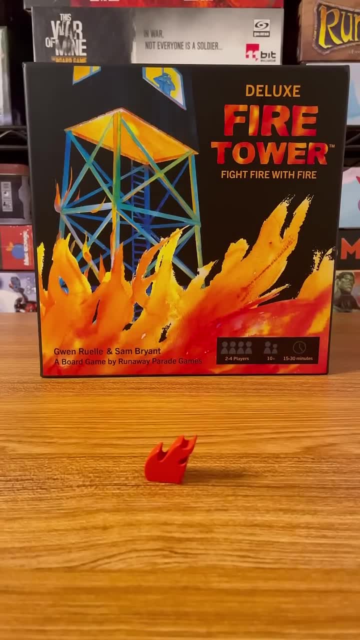 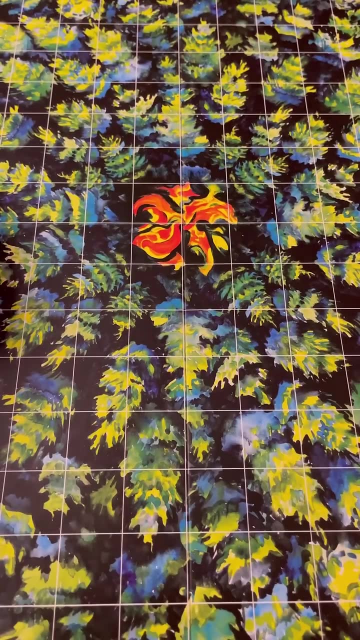 This intense game is Fire Tower. It's a game where you try to be the last one alive. You and your friends have woken up in the forest and are each trapped inside a tower. However, a fire has just started and only one of you can make it out alive. Your goal is to burn down the 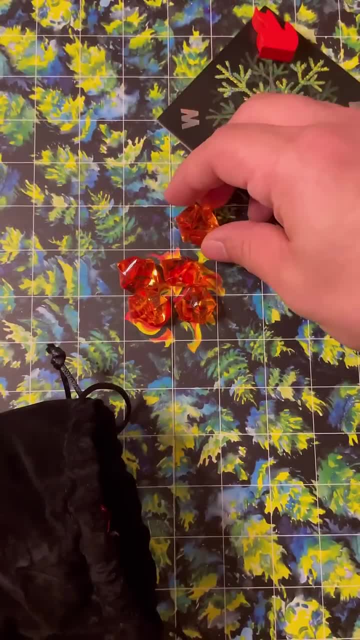 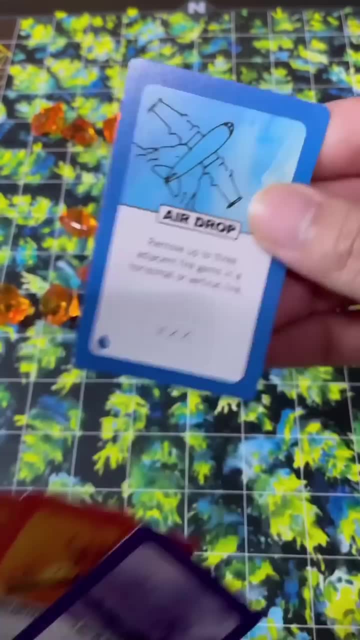 other towers and be the last one standing. Every single turn that goes by, you'll have to expand the fire in the direction that the wind is blowing As the forest becomes engulfed. you'll be able to play cards to increase your chances of survival. You'll be able to change the direction. 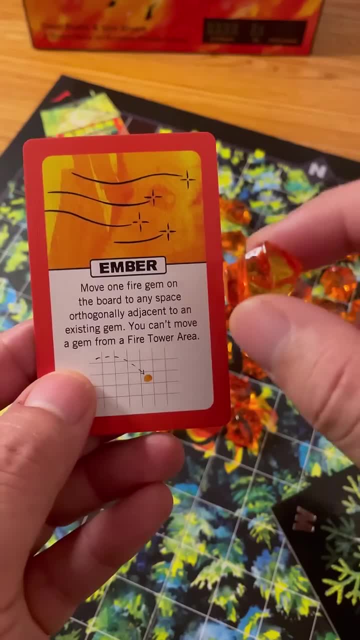 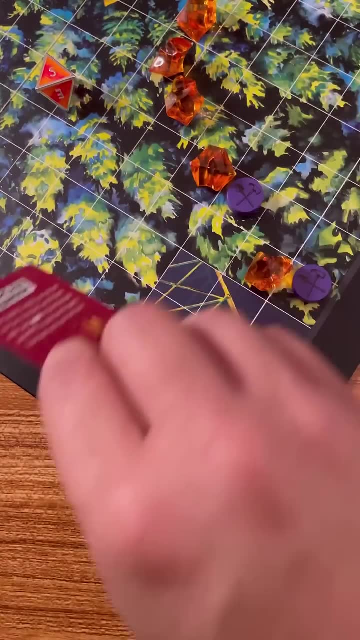 of the wind and push the fire towards your friend, Or shoot a ball of ember and start a fire in a new area. You might even get lucky enough to find items that will slow down your tower from burning. Eventually, the fire will reach your tower. If it ever hits the top, then you'll be 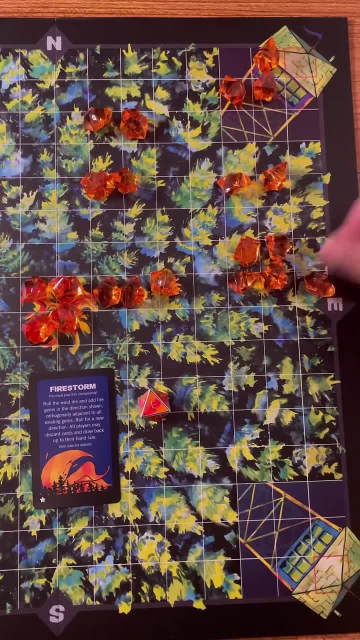 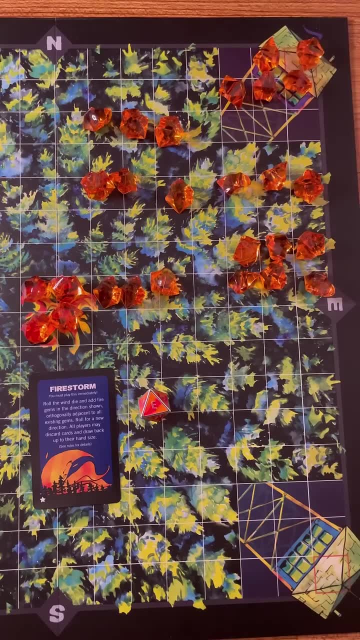 burned to a crisp. Everything sounds simple until the firestorm appears. Whenever the firestorm is drawing, every single flame in the forest will spread out, And from now on, every single time a tower falls, it'll happen again. Now, whoever's tower remains standing will be the winner. 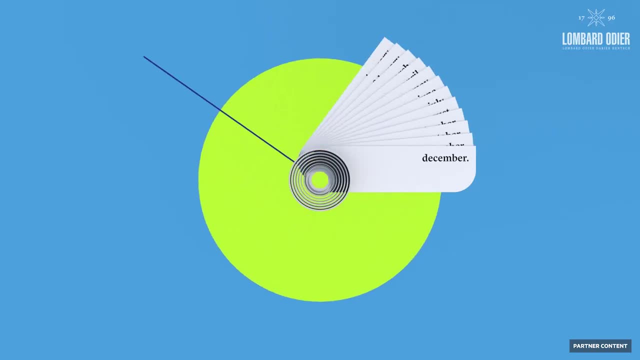 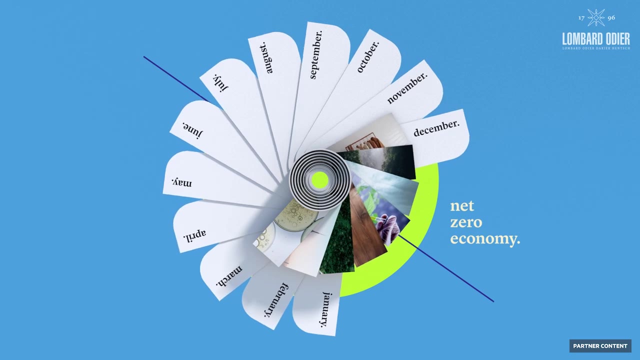 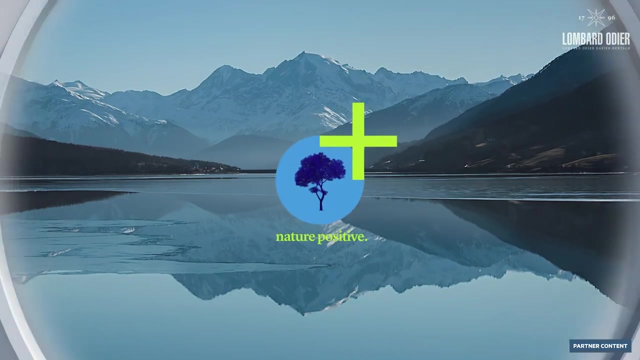 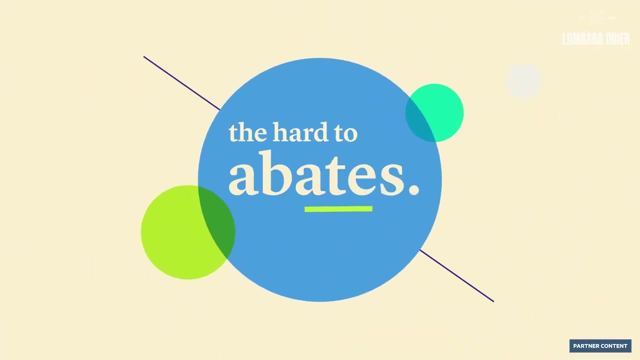 2022 is the year to achieve a net-zero economy, To find solutions and policies in the sustainability space, Ideas that will truly move the goalposts of how we can create a nature-positive future. We believe that it is precisely in the high-emitting sectors where some of the most important work